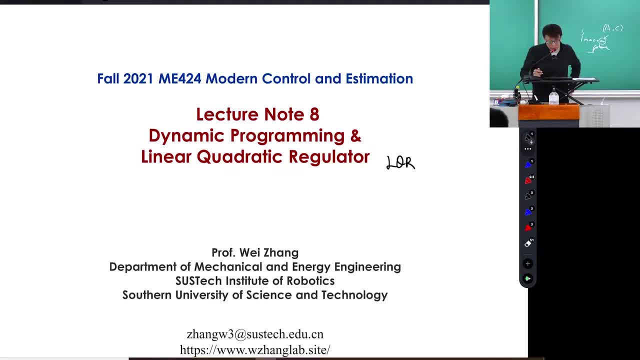 So it won't be that deep, but at least you know what's going on and how to use it, so on and so forth. Okay, And it has been used a lot in robotics, especially recent years. Okay, If you read a lot of any, 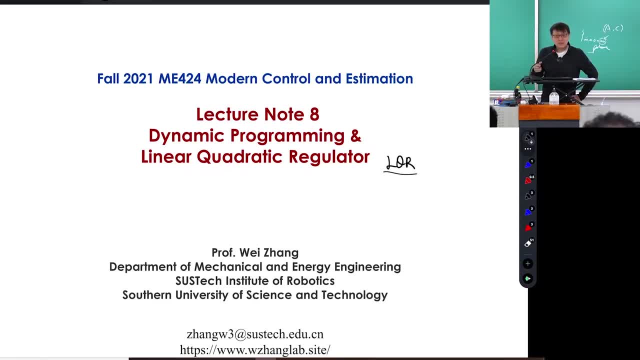 kind of papers talking about control of different robots. I think they all kind of involve LQR or its advanced version like MPC Okay, So it's a- I think the kind of concept extend to model predictive control. So if I have time I can give one lecture on model predictive. 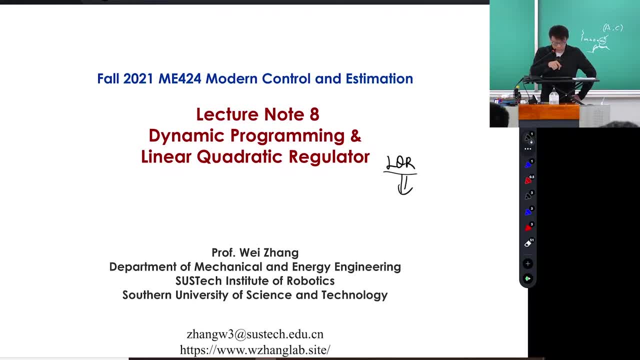 control. You will see the connection between these two. Okay, And also to really understand LQR, again, it's similar to the combat future. It's just a few lines of code, a few equations. The key is that: how do you make sure you understand? 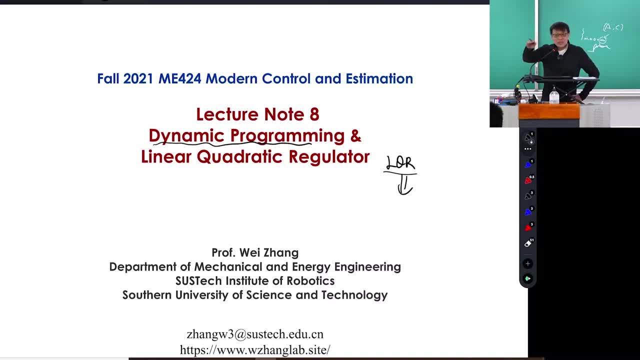 what's going on. So that's why, when you see different variations, for example, like at the beginning of the last lecture, I told you that we doesn't need to assume linearity with respect to control. Okay, That's a common feature, But it's also similar to the command. 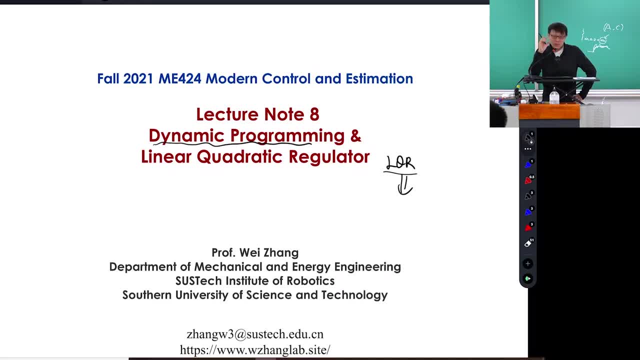 control right. So if you know what's going on truly, you can easily do those extensions. But if you don't know, then you have to match the formulas, okay. So I have to teach you optimal control and dynamic programming to the level. 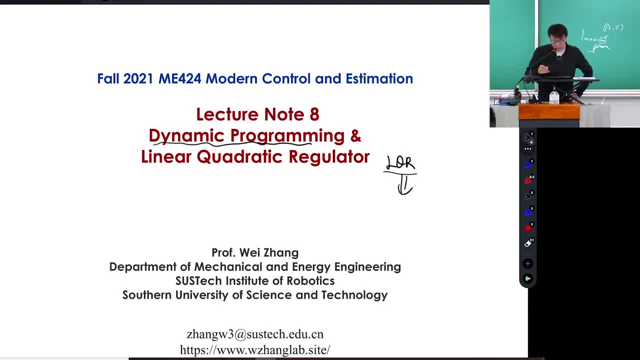 that's sufficient to cover linear quadratic arbitrator, And dynamic programming is my favorite. I have a lot of favorite. This is one of them, okay, And so I will make sure you understand this all right. So today, let's get started. 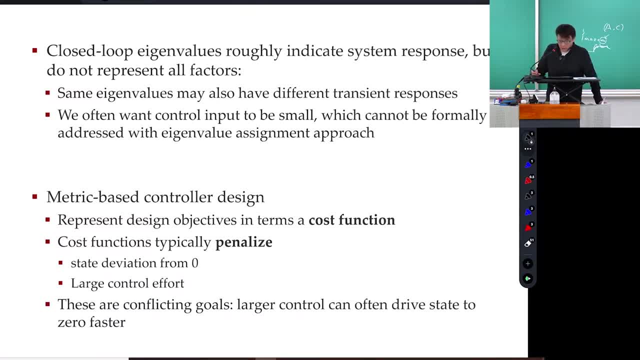 with some kind of quick short introduction So far. I mean, our coverage so far is involves pole placement or angle value, assignment to design feedback, control laws, And then we talk about common filtering. Okay, that's the two main things that we cover so far. 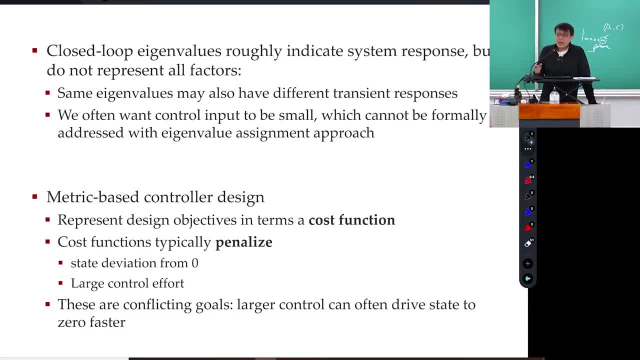 Okay, when we design controllers, we care about what, As I mentioned before, you always think about your design and the control gain is trying to move the angle values of your closed-loop system, because your angle values determines your system behavior. Okay, but my first sentence is going to violate. 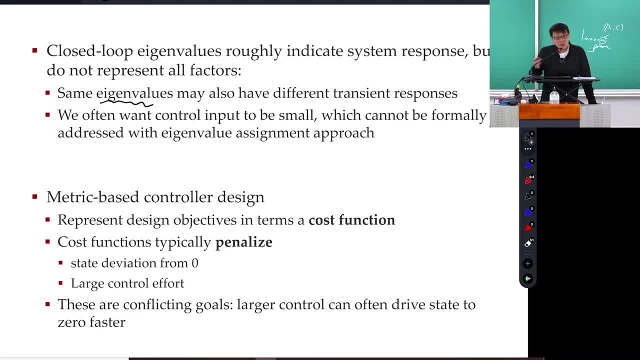 that assumption a little bit. So angle value does not fully determine the transient, It is mostly for asymptotic. So whether the system's stable or not and how fast it converts roughly can be captured by angle value. But it cannot. It cannot fully determine that. 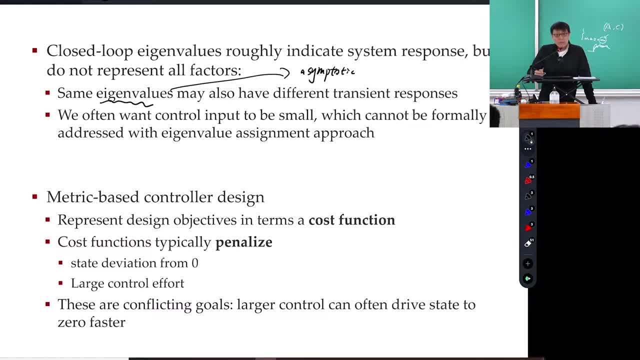 because there's other terms affect the convergence as well. But whether it converts or not, that's determined by angle value. So it only determines the asymptotic behavior. Okay, you cannot arbitrarily kind of control the transient And also what's a good angle value. 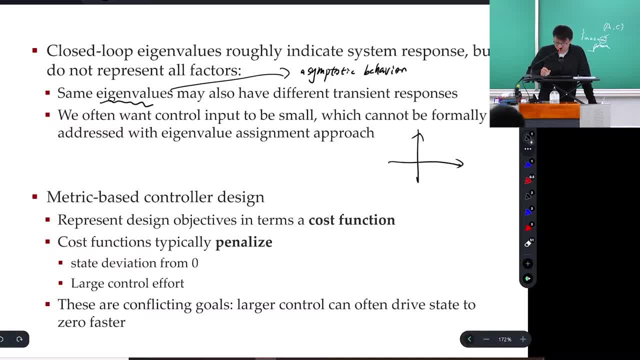 What are good angle values you think, Based on our discussion before? somehow in this great time we need to. how, Okay, I have the angle value in here, here, here, Inside unicircle, But somehow it's in there. 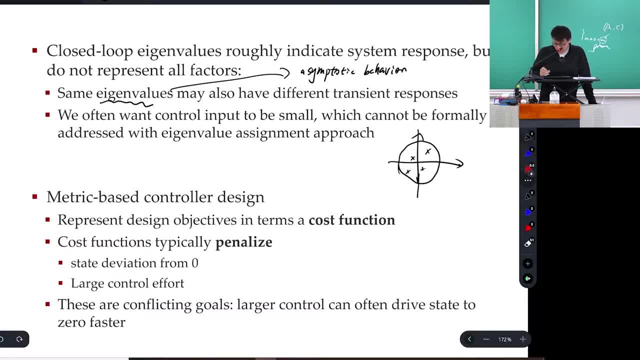 You may not know what's the best angle values, Which one is good? These four. If you think the smaller the better, then I will just choose angle value to be zero or arbitrarily close to zero. Is that okay? Nobody, do this right. 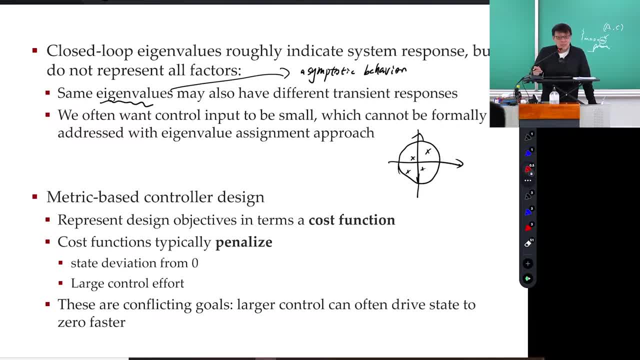 And you have arbitrary large control actions oftentimes. So we never formally see the word formally right. We have a hand waving way to discuss. okay, I cannot put angle value too small because that will cause some bigger control or large control effort. 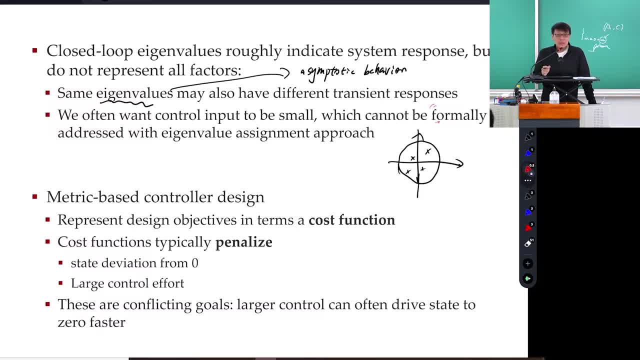 But we never formally address this trade off. okay, There's a trade off: How fast you want the system to converge and how large you can suffer, or you can tolerate Your control magnitude. No things can be done or can be formally addressed. 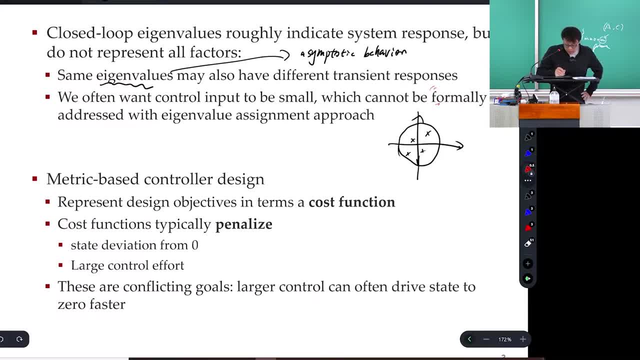 in the framework of optimal control. okay, So this is. you can think about this as metric based controller design, So it's not only stable or not. You want somehow a criteria to tell you what are the best. So the cost function. 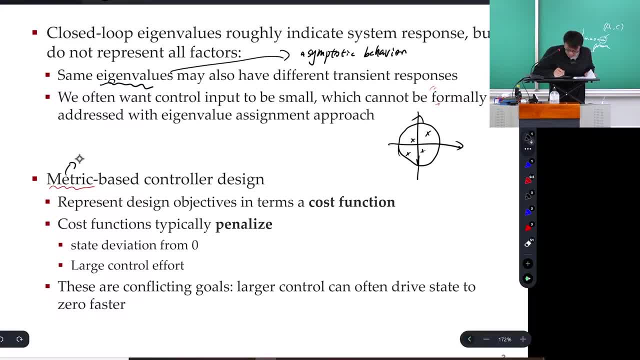 the metric. I think we can also call this optimization based. Okay, You may not realize. okay, there are only three tools that we keep using throughout this semester, maybe your entire life if you stay in this major. okay, It's two, three things, right. 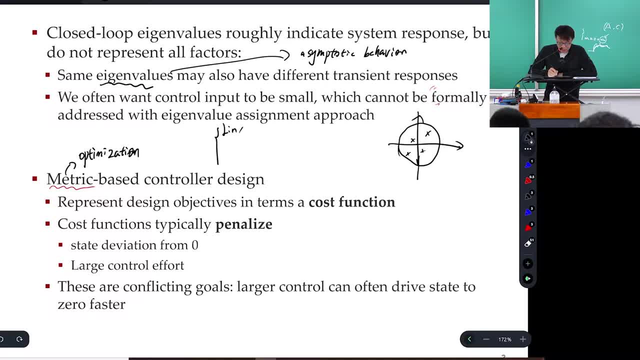 I mean the most important key thing, that my favorite right linear algebra. But how often do we need less? What I mean by less is you use a number to let you realize if there is probability. the other one that you may not realize is optimization. 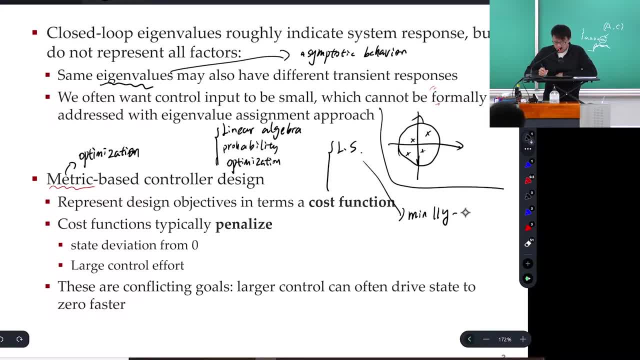 Okay, If you view the topics we cover so far, least square Least, square right. So estimate some unknowns and we're trying to minimize the deviation from our observation, From the model predicted output to the observation. Okay, and for common filter that we just finished. 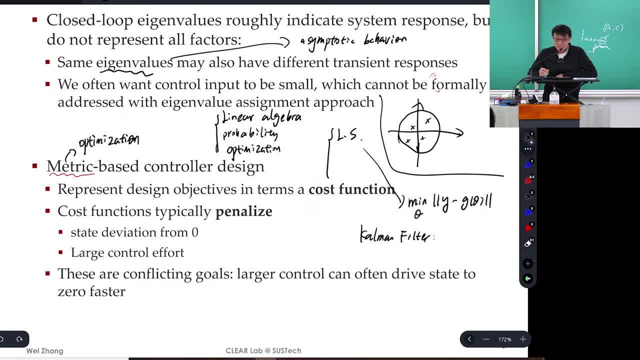 Filter. we are trying to optimize what Minimized minima. okay, X minus The best estimate, Given the given. something I want to: I optimize the best, the minimum, the mean squared error. that's what I want to minimize, right, all of this transform to Optimization. essentially, you are dealing with optimization either with deterministic models or deter, or probabilistic models. 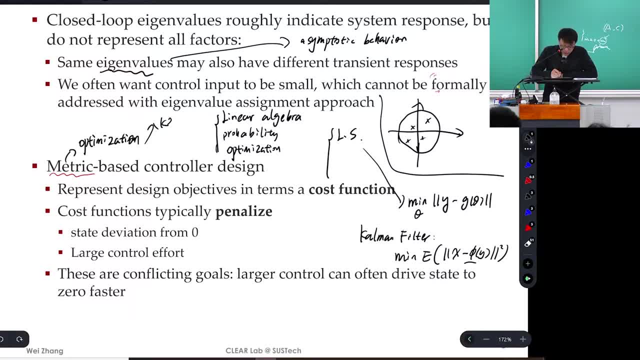 That's the key. This is the key not only for this class, for modern, not control more than engineering. What does engineering do? Find the solution to real-world problem right. you may design Your kind of robot, maybe mechanical design that doesn't need kind of medicine. but you should first ask: what is a good design? 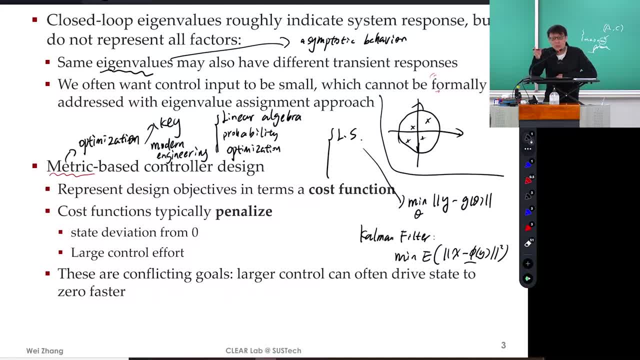 how do you quantify a design is good or bad? if you have that sense and you can optimize it, all right, Whatever it is on your design controller. You are designing mechanical parts. your motor and Your design have some parameters. you often want to optimize over these parameters. 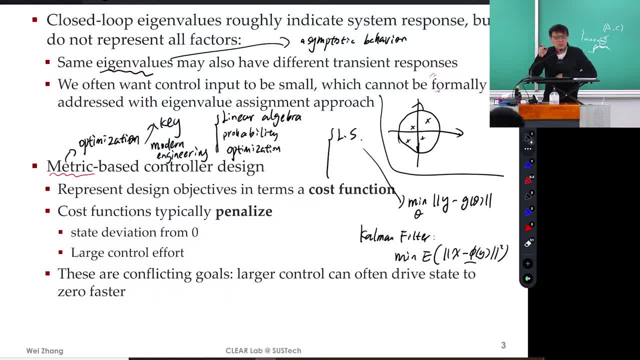 according to certain cost criteria that you before you may just just in your mind you, I think this will be good. Think about how you design Yuntian, how you design a mechanical. do mechanical design Cause functions? in your mind, You have your own kind of prediction. 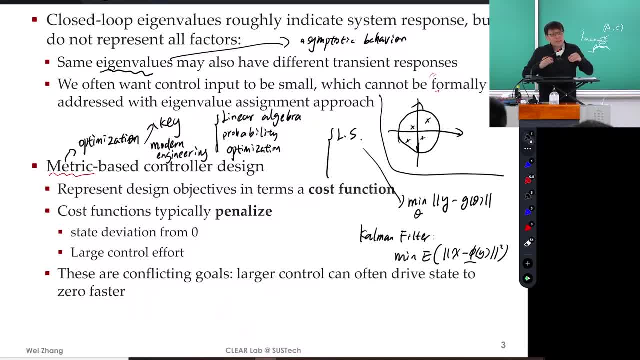 If I make this the thickness of this part, I mean there's a lot of parameter. you need to make decisions right And these decisions in your mind you think, oh, that will lead to a good performance. I have some constraints. 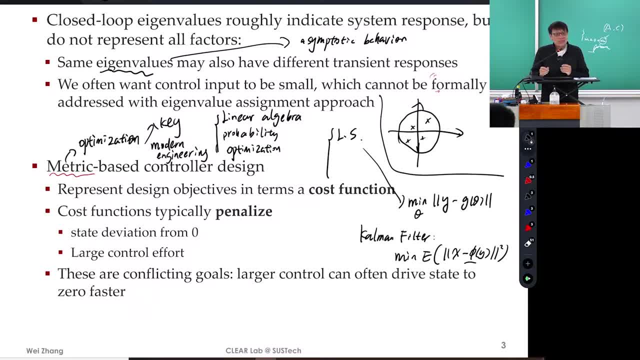 I need to make sure the force right You need to provide. You have somehow your own kind of cost function in your mind. You just didn't explicitly write that down. So what you're doing is optimization. Okay, So machine learning is also optimization. 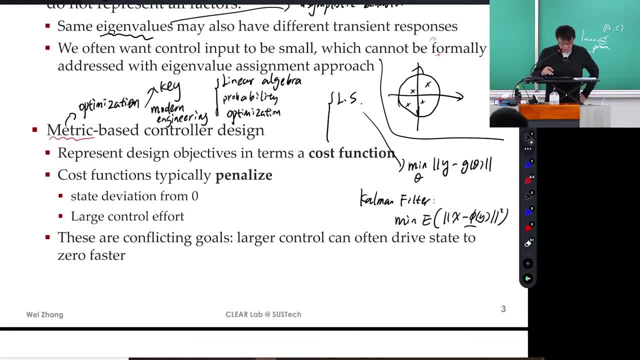 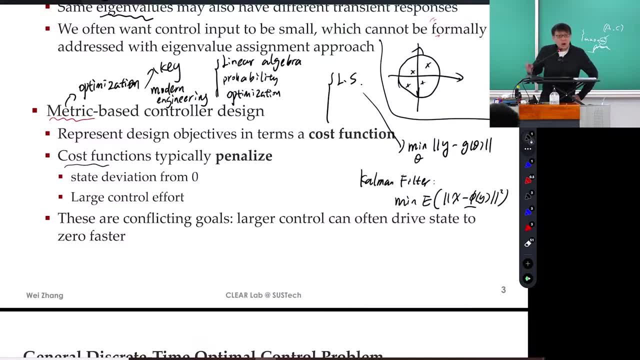 You know that right, It's nothing but optimization. So match the data, So cost function typically, how do we optimize over control laws? Okay, controllers And cost function. we use cost function right. We have to make sure we have a criteria. 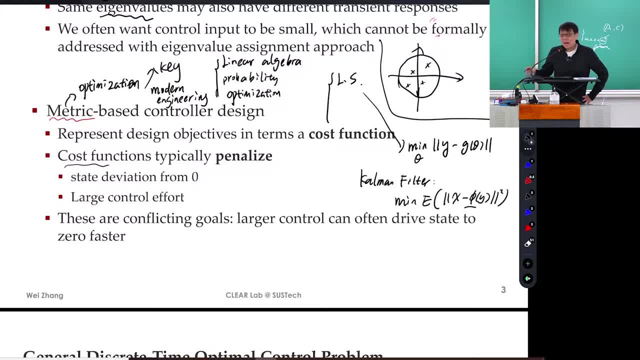 to determine what is a good controller, what is a bad controller, And we can use cost function. Cost function can deviate, can penalize your state deviation from your desired locations or positions or penalize large control effort. That's also possible. 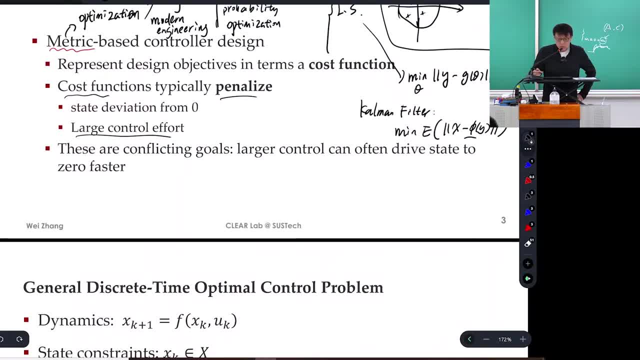 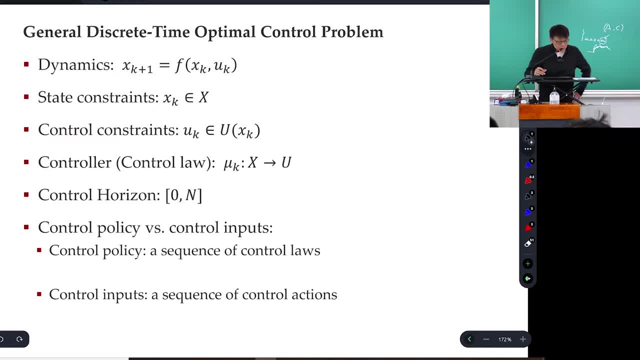 So, whatever you like, you can use. So whatever you like, you can use. So whatever you like you can, your desired behavior is, you can penalize deviation from that desired behavior. So now let's give some terminologies, Okay. 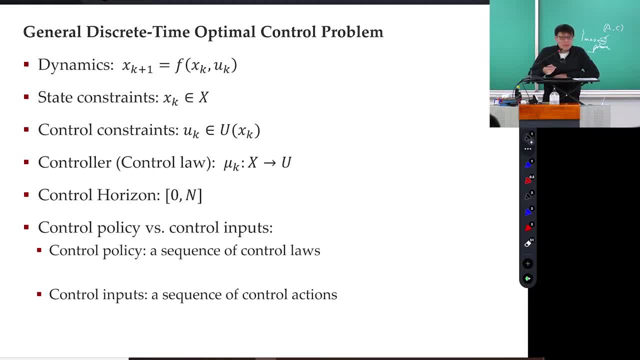 The optimal control port that we are dealing with, I'm trying to introduce, is very general. okay, We can do nonlinear dynamics. It could be like robots- whatever robot you feel like you want to study, And you have to be able to write this down. 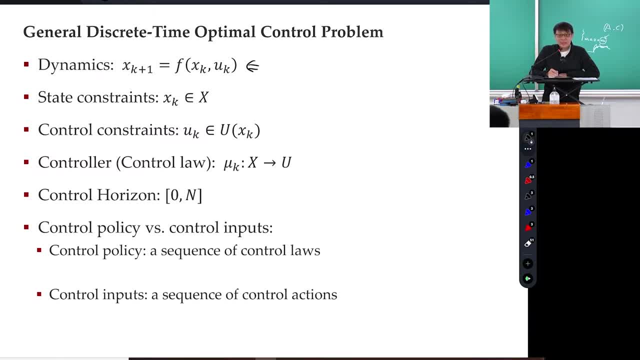 as a dynamical system. This could be nonlinear- okay, And oftentimes you may have state and control constraints. In other words, when you design a controller, you need to make sure your system satisfies some behavior okay or do not violate some kind of constraints. 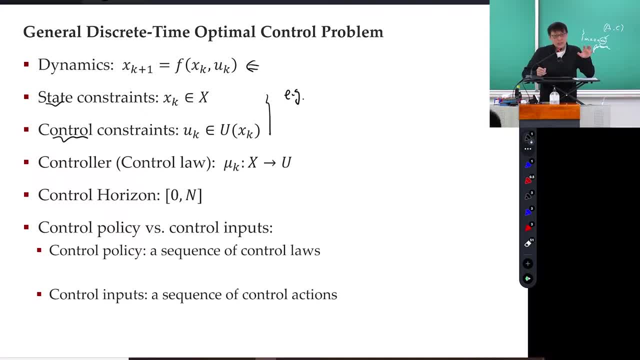 So I will give you example. Suppose you are trying to design your motor controller, So for example, motor control. Suppose okay, And this state constraint could be: say, my temperature is lines of 80 degrees, I don't want to go over too high. 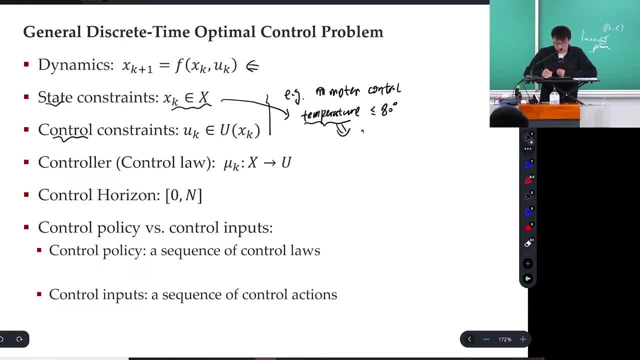 All right, And the temperature typically is a function of your state. Okay, This is the T. It's a function of your state. okay, X, K At any given time, your state, somehow it should be a state of function. 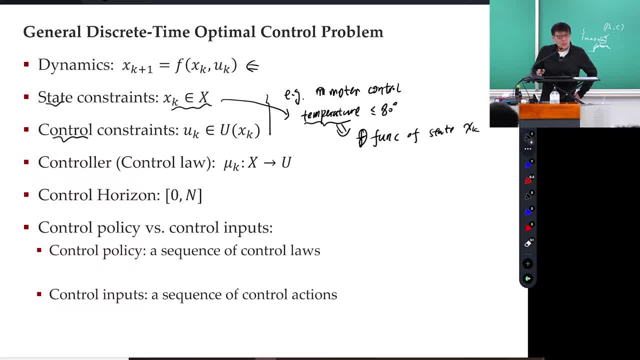 So state of function should be less than 80 degree. that impose a constraint on the state You want the desired controller to respect or to meet that constraint And this one. so control also has constraint, For example, the torque, the maximum torque I can give. 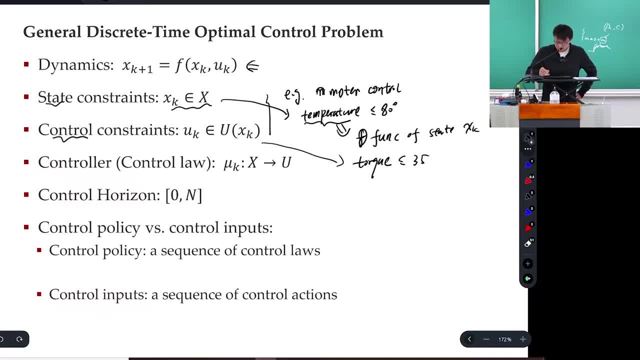 is 35 Newton meter, for example. That will be. it's already pretty good. all right, 35 Newton meter. suppose That will be your control constraint. That make sense. For our previous design procedure we didn't consider any constraint yet. 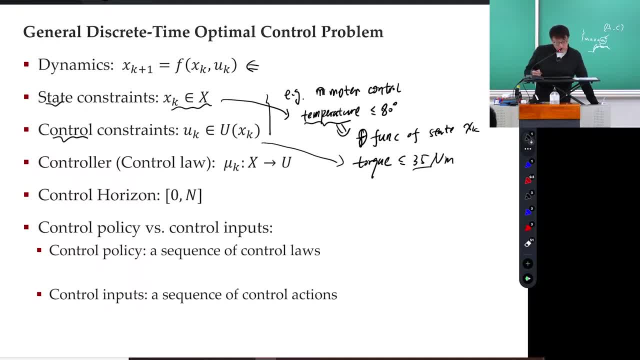 but optimal control can allow you to do it. Okay, another term I want to somehow you get familiar with is control law. If you don't like the word law, you can think about that as controller. But what does controller mean? You have a controller. 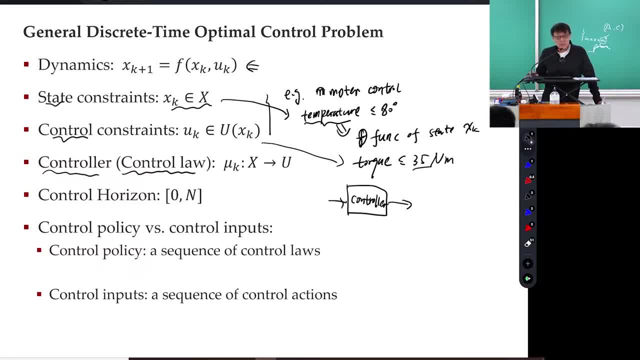 You always think about controller from diagram view. Controller in your function or in your system is nothing but a function. Take measurement or state and gives you what I think a good control action should be. at this time It's a mapping from state to control action, right. 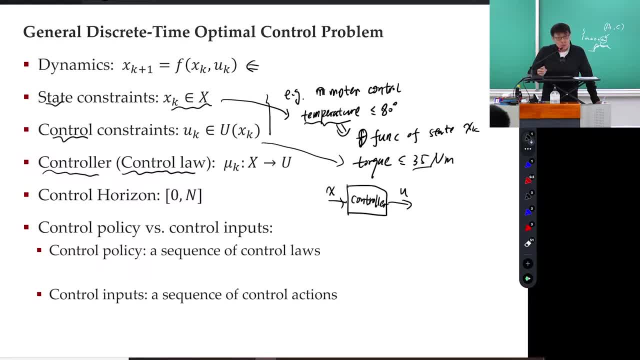 So controller or control law, it's a function. It's a function of the state, And the value of the control law is the action you should take at this time, at this particular state, And for optimal control problem you often need so-called control horizon. 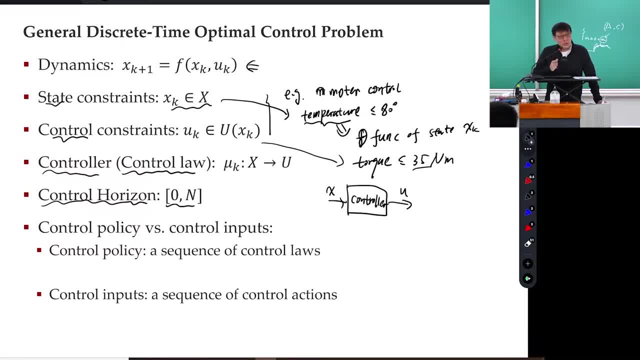 And this is a discrete time. we'll say zero: one, two, three, four, five, up to time n. This is the horizon. If n go to infinity, then we will have zero to infinity. This is called infinite. 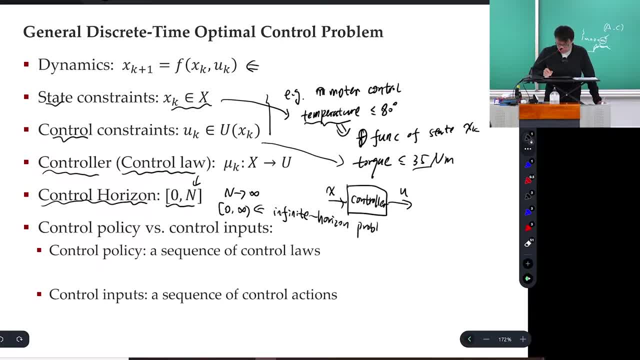 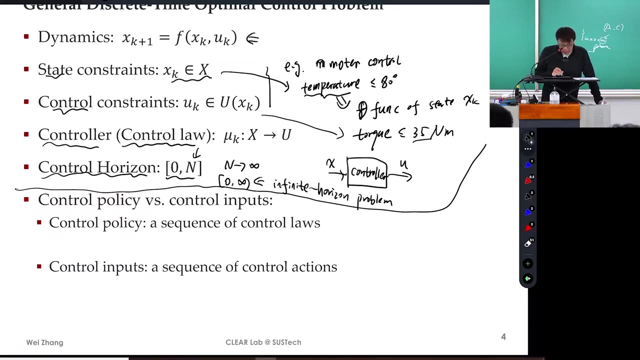 Infinite horizon problem. You consider all the future behaviors. You not only look at 10 steps. So infinite horizon problem, That's the terminology I want you to know, And there's a few things as well. That's control policy. That's where you do learning. 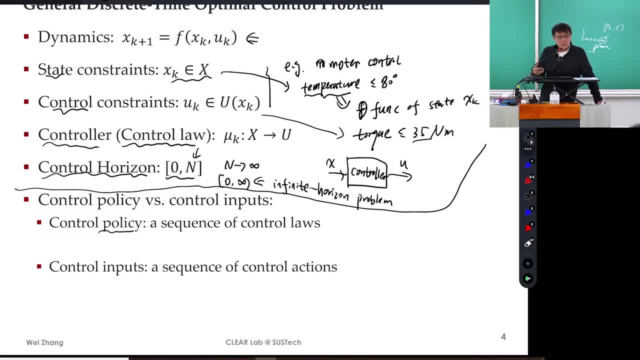 It's always reinforcement learning That's also trying to solve this problem. trying to solve reinforcement learning is trying to solve an optimal control problem. Well, if you want to talk to the CS students, then they're trying to solve a Markov decision. 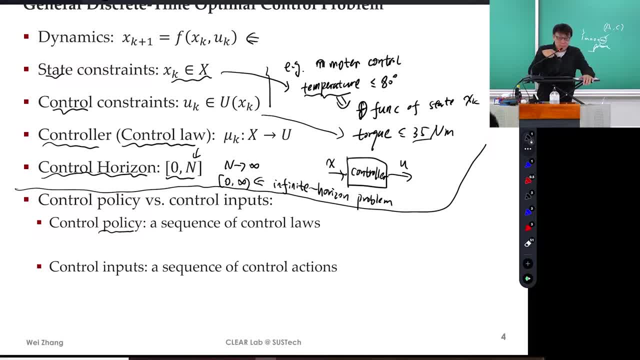 problem, which is an optimal control problem for a stochastic system. alright, That's roughly, it's that Policy. I would say pi. It's a sequence of control laws. let's say a sequence of functions, alright. And the control input sequence is a sequence. let's say u equal to u0,, u1, u n minus 1,. 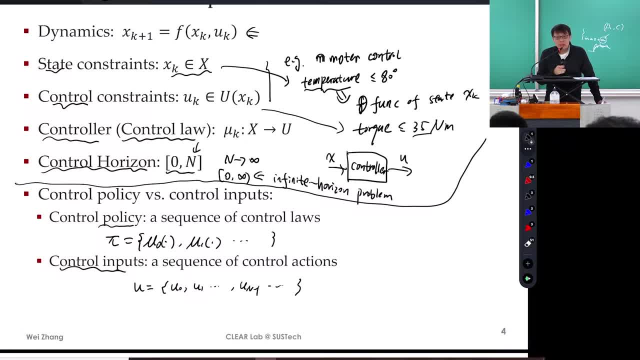 something like that. That's a sequence of numbers or vectors: control action. This is sequence of functions For control law, for example. Yeah, For example, this guy could be mu1, x is a function of state. could be k1 times x, right. 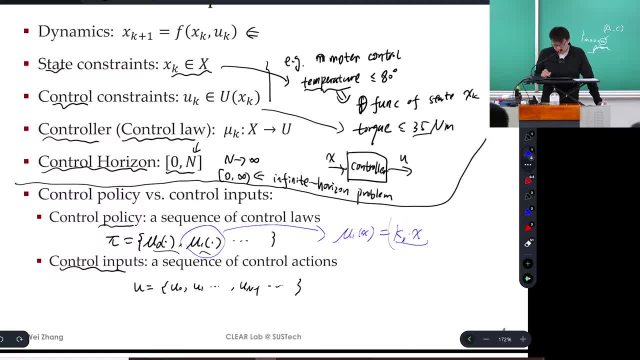 The gain times. Is this a function? Yes, Yes, right. It's a linear function of the state. It's a linear control law. I can have nonlinear control law, right? This is only an example. I could have this. 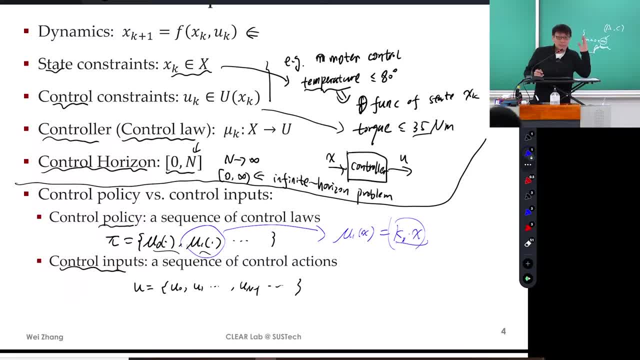 It's just a function of state And policies can be viewed as a sequence of- Yeah, As a sequence of control laws. That means your control law can change over time, If I Let's say, if the control law doesn't change so any given time. I'm just 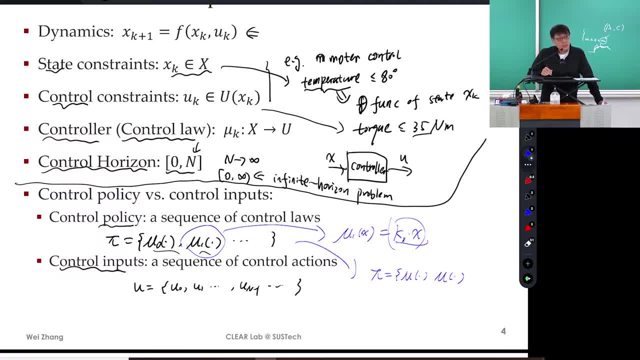 This block doesn't change over time. Your controller doesn't depend on time. then I can apply the same control law all the time. This is typically called stationary policy, Okay. Okay, So you can use this to do more than what you need, but those terminology will help. 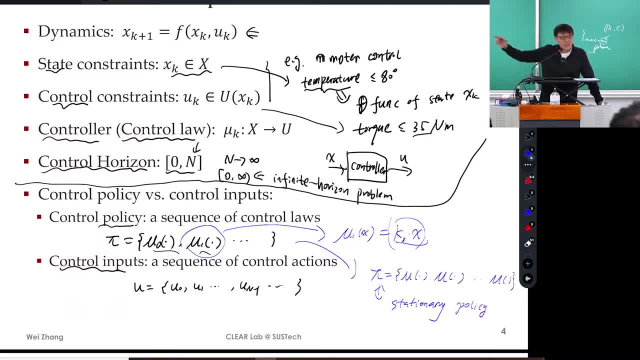 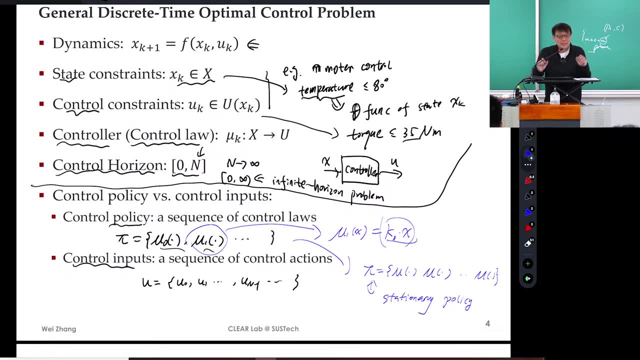 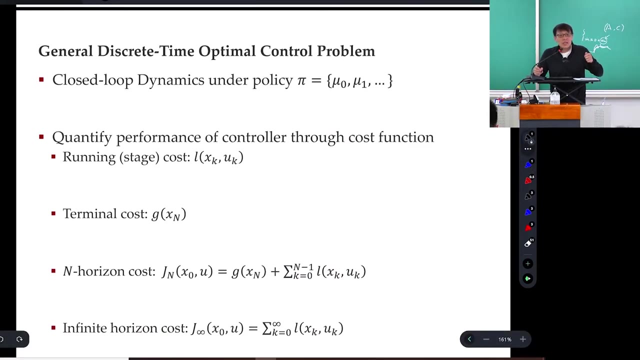 you to connect what I teach you to other kind of materials, online or from other class. Okay, That's all terminologies. Any questions? so far, It's abstract, right? You need to see examples, Okay, Okay, One thing that I call a lot. I somehow refer to a lot of closed loop, right. 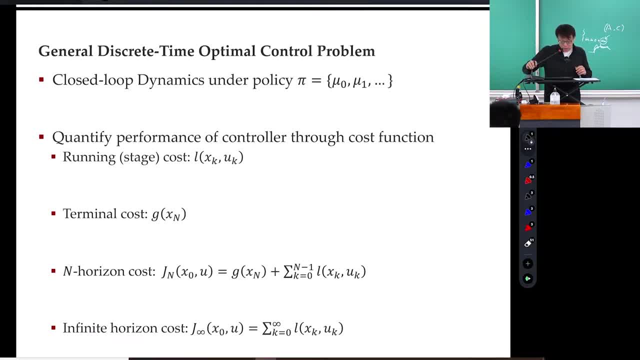 I explain a lot as well. And in the controller design we have closed loop. You plug in this control law. That's your controller. right Controller determines control And this is your system. Suppose we can measure out the state, The behavior of this closed loop, behavior will be my closed loop dynamics. 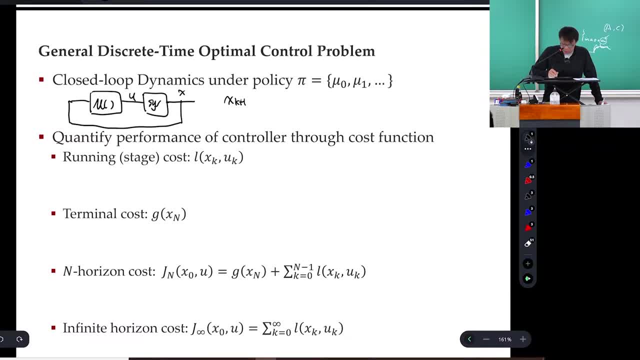 Right, So if I have my open loop, it's like this Open loop depends on what control actions I gave you. Control is undetermined, yet undetermined, undetermined, undetermined. okay, It's not determined, not specified yet. 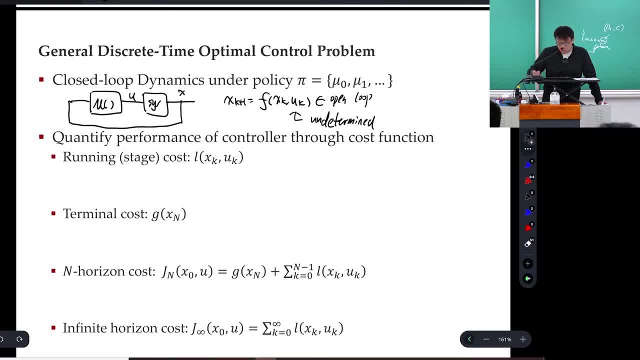 This is open loop, Okay, Okay, Okay, If I plug in my control law, right, If I consider this behavior, then the closed loop dynamics will be xk plus 1, equal to f, xk, mu of xk, right. 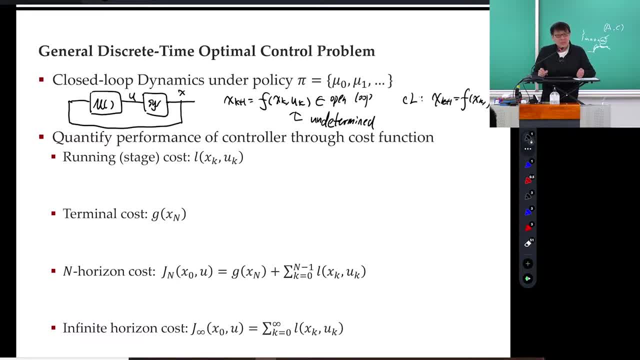 You plug in your control, So your control already determined if your state is given. So this will be my closed loop dynamics. Okay, It only depends on. Only depends on. Only depends on State. X, Okay, X Only depends on state. 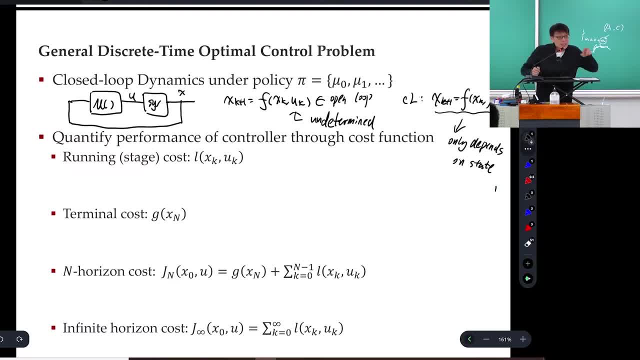 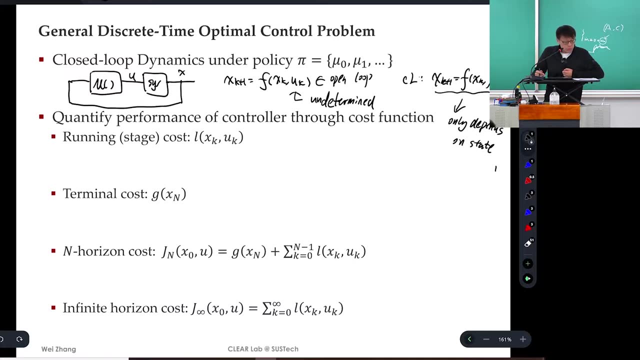 The state keeps changing, so you have a closed loop dynamics. That's terminology. Some you may know before, some you don't. That's fine, Let's get more exercise. You will get familiar to most of them. Okay, that you want to make sure. you want to quantify performance through cost function. 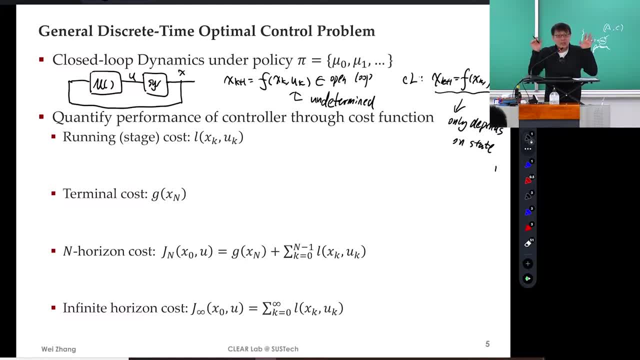 Okay, don't argue if you don't have a criteria. I like PID, I like MPC, I like fuzzy control, I like neural network control, I like adaptive control, I like this method, I like that method. Those arguments don't make sense unless all of us agree upon a cost function. 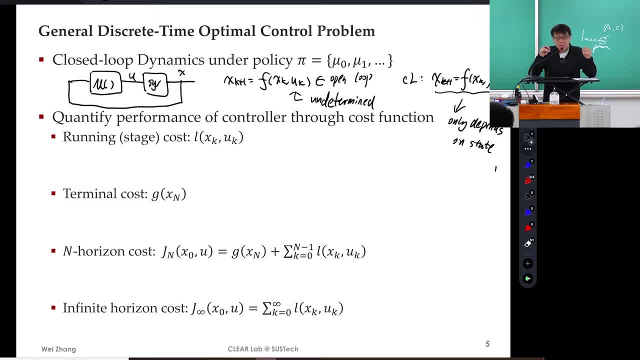 So what do you mean by good? You think this is better? right, This is good. but you have to specify. what do you mean by good, Otherwise it's just nonsense. right, You have to agree upon something. If your goodness, if your good is different from my kind of performance, then magic, then. 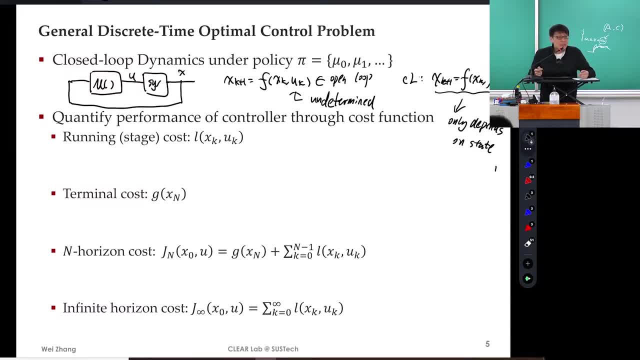 we. of course we will have different answers. If we agree upon a cost function or common performance, If we agree upon an index function, that means I just want the shortest path to that door And if you think okay, you think that's a good metric, so the shortest path to that, 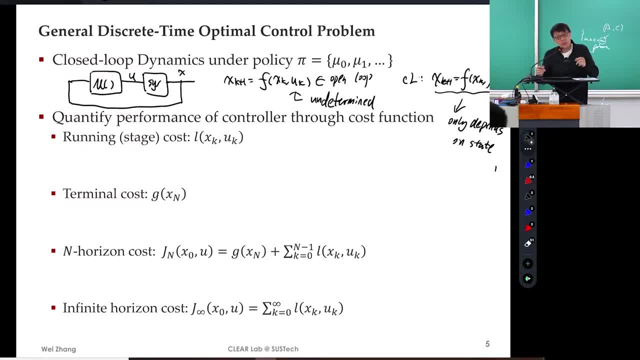 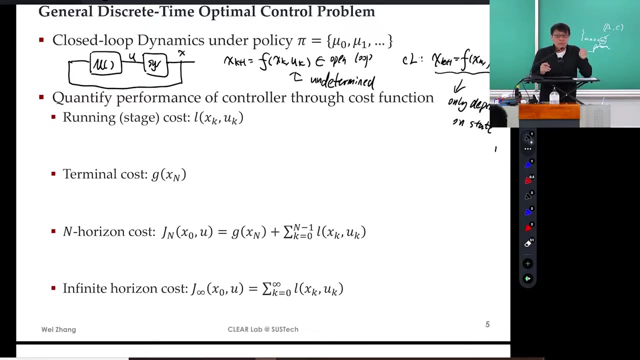 door, then we can find our solution, and our solution should agree. all right, If you want to say I want the shortest path, but the other one say I want the minimum energy, okay, That would be different, okay, So let's. so the key is that for not only optimal control, for, as I mentioned, modern 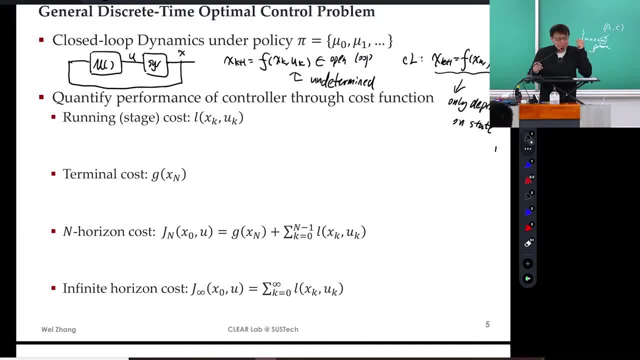 engineering is to really kind of encode. your objective means what you want to do to a cost function And then you solve optimization problem. okay, that's it. So let's see how we can quantify good performance or bad performance For optimal control problem. so typically there's two kind of ways to define, to encode. 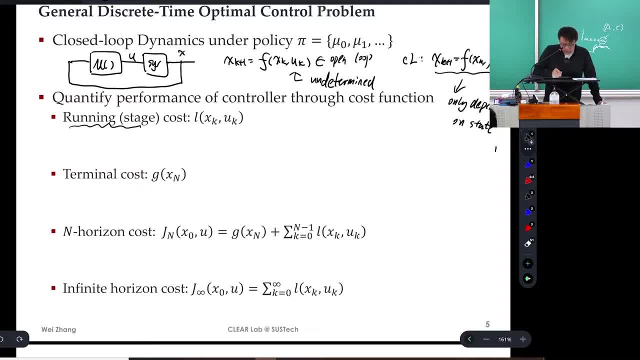 your objective through either so-called stage cost. cost means running cost or terminal cost is two things. okay, These are both functions of state and the running cost also is a function of the control action, So we can penalize. So this cost is introduced. to penalize cost means you want to make it small, right? 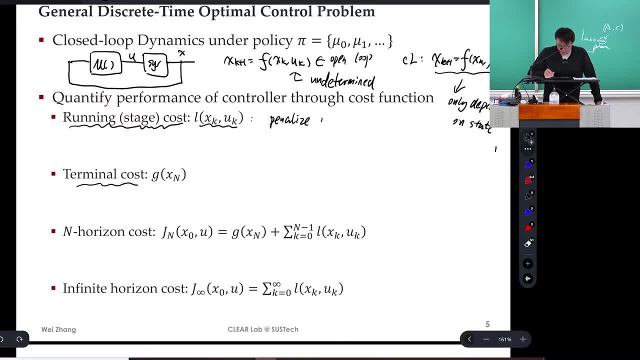 So it used to penalize undesired behavior. okay, behavior. What do I mean by that? For example, if my desired penalize undesired behavior, you have to have some desired behavior First. okay, suppose my desired state. I want my state to stay close to desired state. 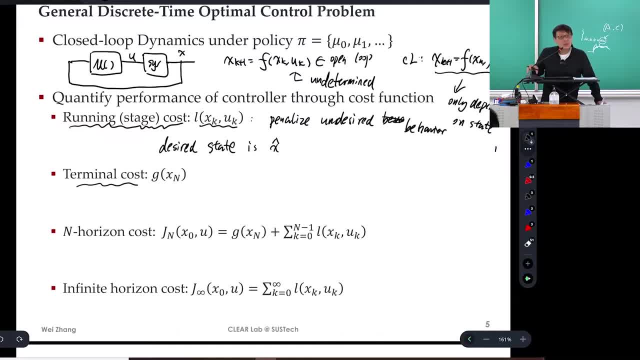 is, let's say, X hat, stay close to that X hat, Then my and also small control effort, small energy, Then my cost function is a function of state and the control could be X minus X hat squared plus U squared. That's one case, one possibility, okay. 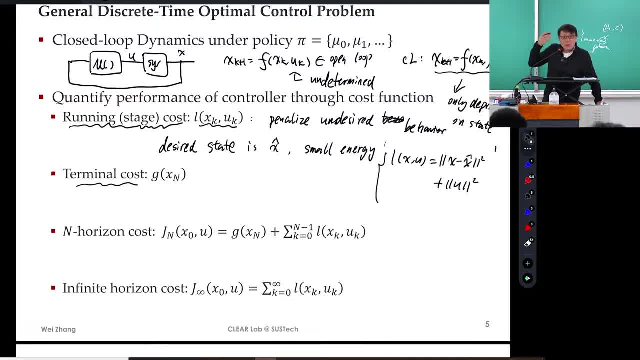 What does this cost function do is somehow encode your objective. okay, I want to stay close to that state and I want to minimize my control effort. Okay, All right, If you want to say I want to stay away from this as far as possible, this is some bomb. 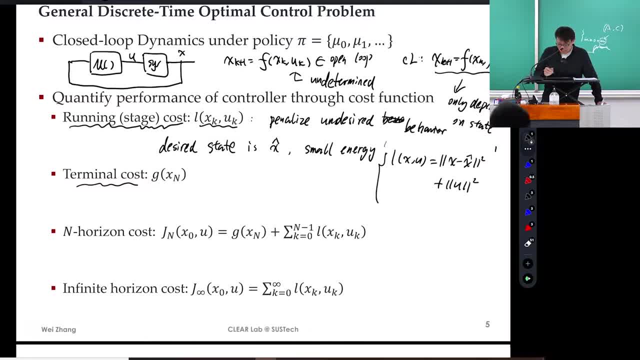 location or dangerous location, then it will be different. You can use one over it to encode that objective. So whatever objective you have, you have to make sure you can write it down. quantify them as a cost function. okay, Terminal state is just at the end. 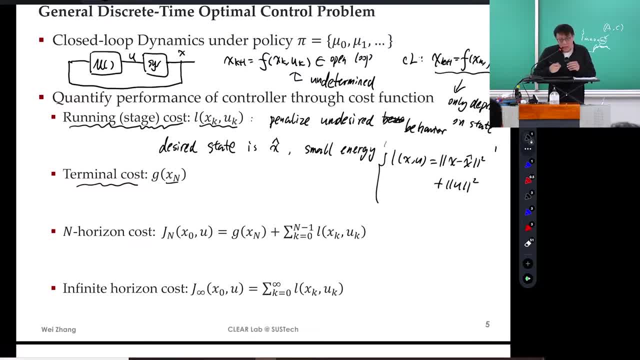 End of the game. you want to make sure you have the choice to specify, to penalize your deviation from your desired state. So this could be, for example, could be also deviation from this. maybe three Cost function is not given right. 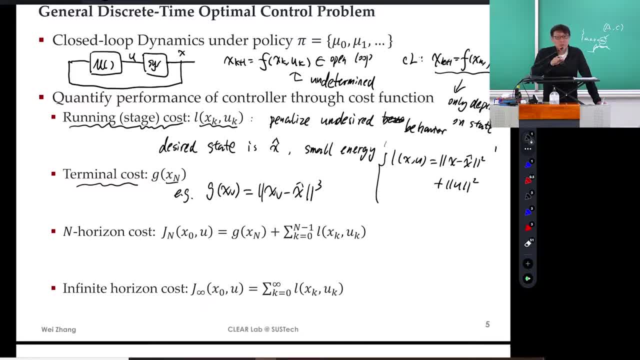 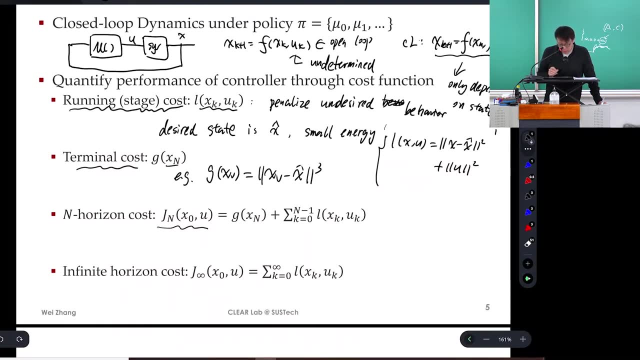 It's whatever best explains your objective. It's your choice. Okay, There's no kind of a good choice for everything cost And nHorizonCost function is so you want to select your control sequence to minimize the cost, which is summation of the running cost plus the terminal cost. 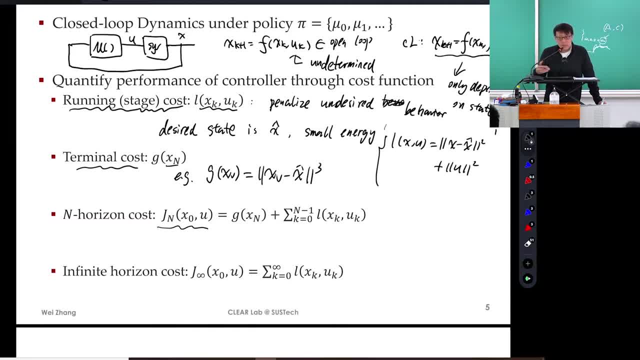 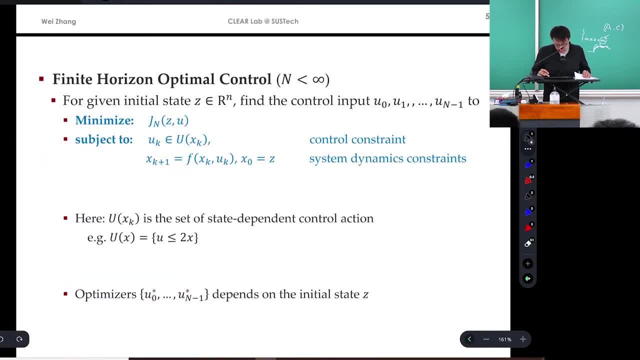 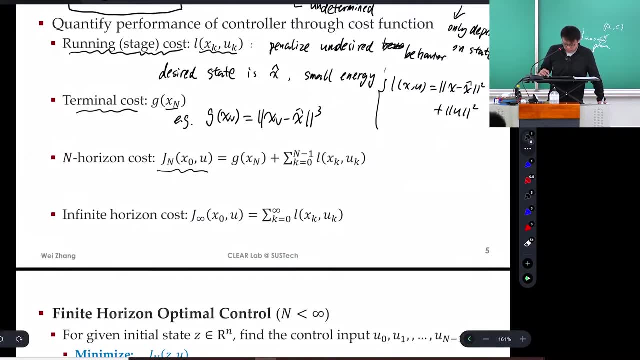 That's a standard formulation for optimal. If you minimize this, it will be standard formulation for optimal control problem Okay, All right, Okay, So now let's look at the general formulation. So our goal is: let's see, okay. 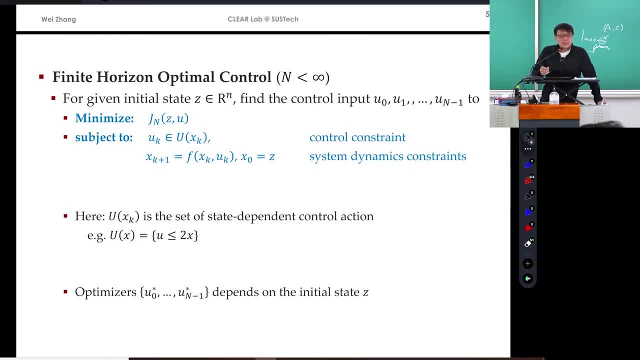 So design your controller can be viewed as: select the best control action to minimize your cost function. This is a cost function, right? So it's summation of running cost plus g of terminal cost. Okay, That's the standard formulation And I want to say all the control problem can be transformed into optimal control problem. 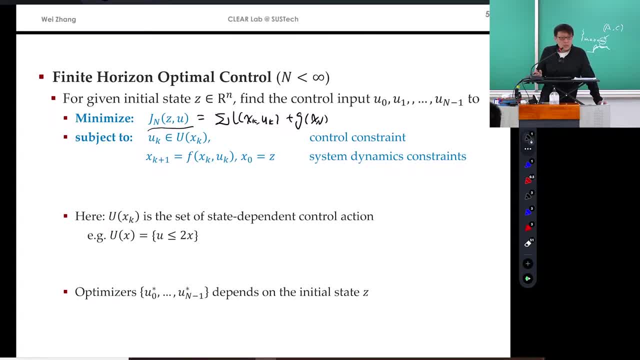 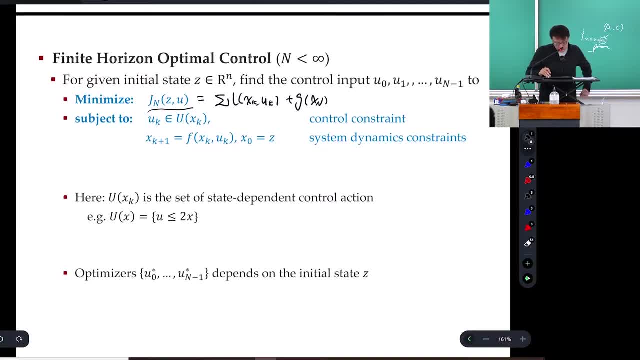 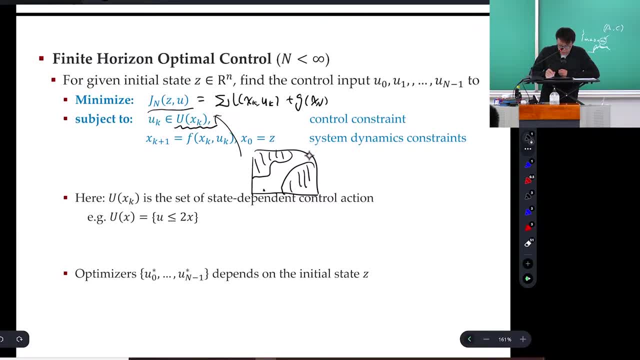 Those are obstacles. You want to from here to go here. all right, That's your goal. You want to find the path from the initial state to the final state And at any given location your control constraints are different. For example, I can tell you: suppose this is my A, then locally my control can move. 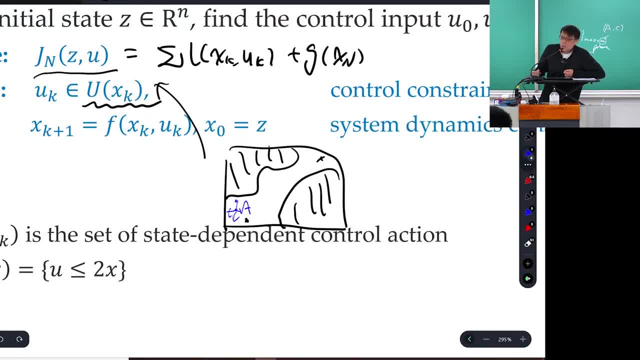 anywhere. Let me zoom in. okay, I can move anywhere, But if I'm here, this might be The control. action I can take is only Okay. It doesn't allow me to move away from the obstacle. There's some action that's not allowed. 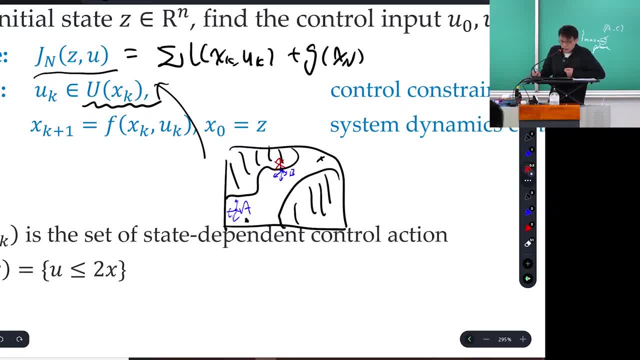 For example, going here is not allowed. okay, So if you specify your control action, the constraint you have is state-dependent. in general, It depends on where you are. the available control action you can take is different. Okay, If you have this. 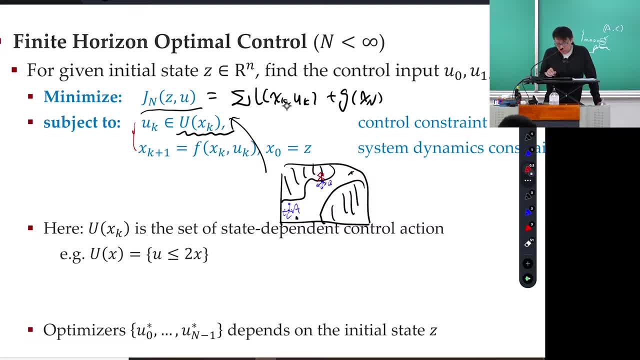 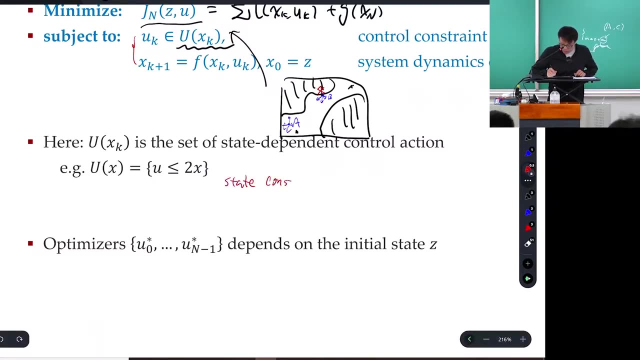 Okay, You want to find the control sequence to minimize this cost function subject to those dynamic constraints and also control constraints. I want to also mention state constraint can be transformed. can be transformed to state-dependent control constraint. Okay, What do I mean by this? 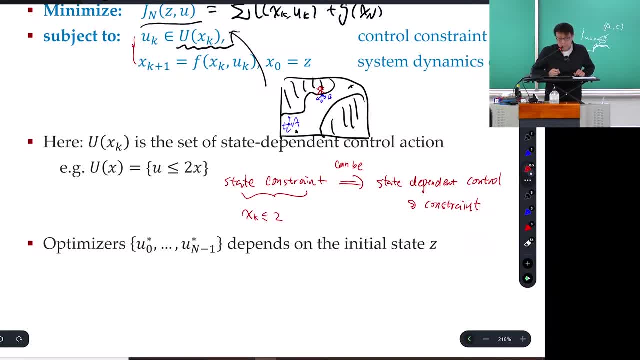 State constraint, for example, XK less than two. That's my state constraint, right, Then that's imposed. That tells me, because I know my XK equals to XK minus one, I suppose. okay, plus two of UK minus one. 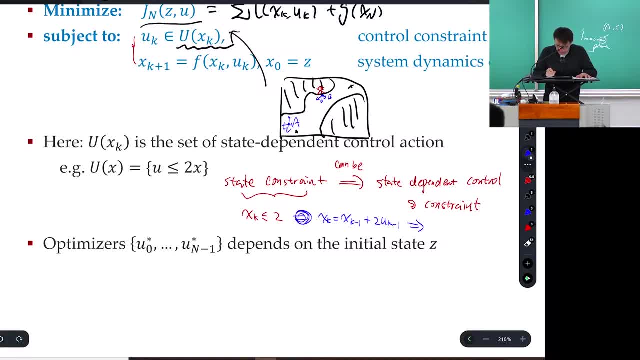 Suppose that's my model. That tells me, let's say, suppose This is assumed, Okay, This two thing tells me that my UK minus one should be what Less than two minus X divided by two XK, right, Sorry, XK minus one, okay. 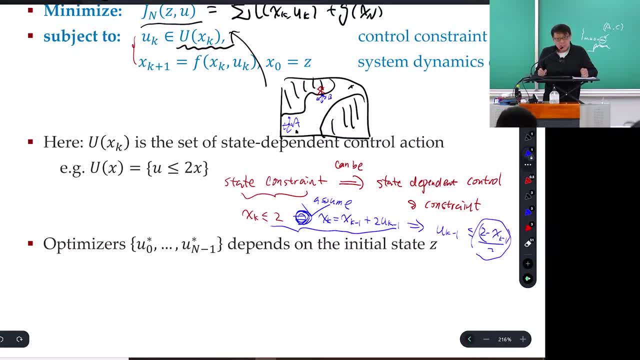 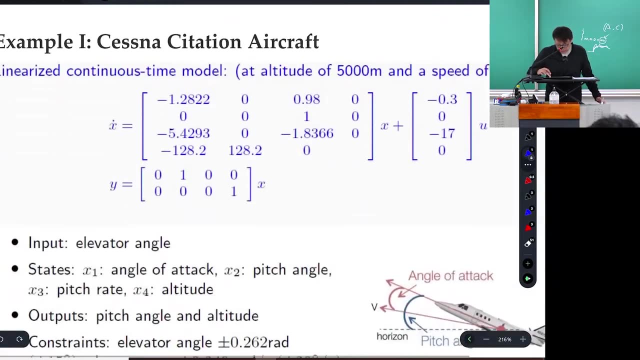 So that's my. So this is a function of state. So you control constraint depend on the state Now, So state constraint can be transformed into control constraint. Those are pretty abstract. Let's look at example. I think that's the best way to see how this works. 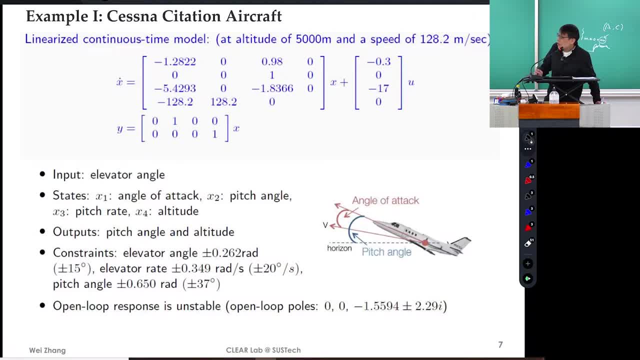 Okay, Suppose this is an aircraft example, This is a real kind of example, right? So this is how they design controller for aircraft early days And this is the linearized model of the aircraft dynamics at a particular attitude: 5,000. 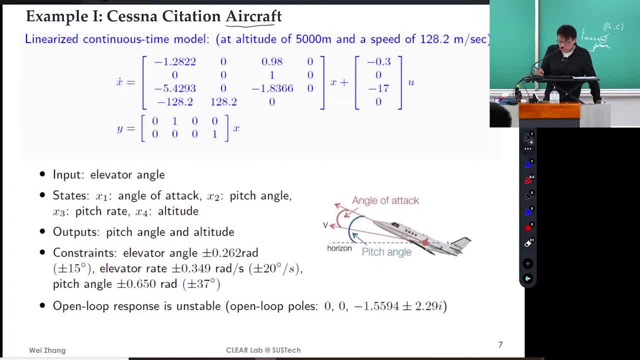 meters and at airspeed of 120 meter per second. And this is my state, is First state is angle of attack. Where is the angle of attack? This thing? it's angle of attack And the second one is a pitch. 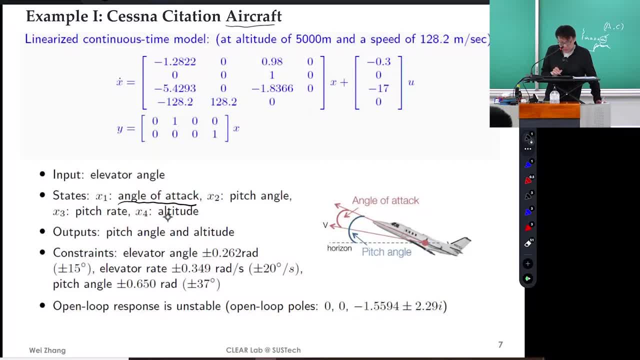 And the third one is a pitch rate, And the fourth one is altitude. It's how high you're flying. Okay, Those are for state. This is attitude minus 5,000.. Okay, This is deviation from your desired altitude. It's not a true altitude. 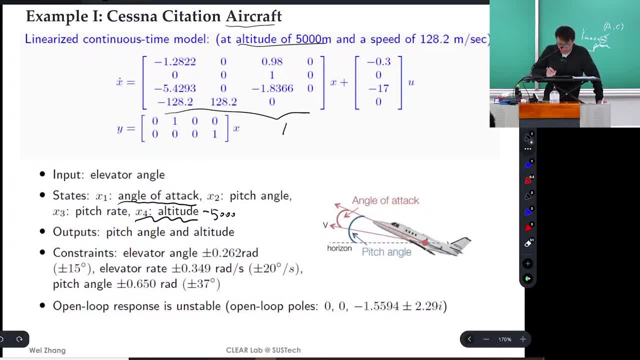 Right Given these dynamics. this is my A matrix. This is my B. This is continue time. This is my C. That's a linearized model. Okay, Our goal here is to stabilize it, Make To make X convert to zero. 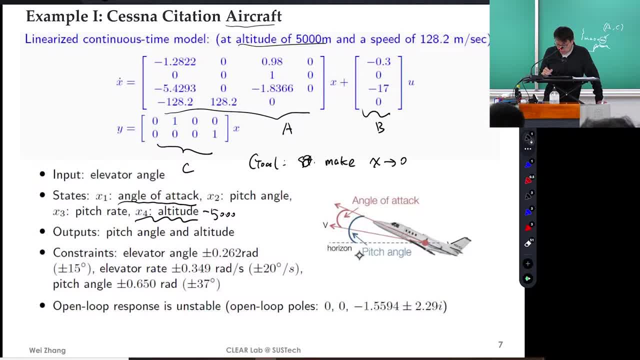 You want to make sure you fly with zero angle of attack, zero pitch angle And at this particular 5,000 meter, that means X4 also need to be zero. Okay, So our goal is try to make sure everything goes to zero. 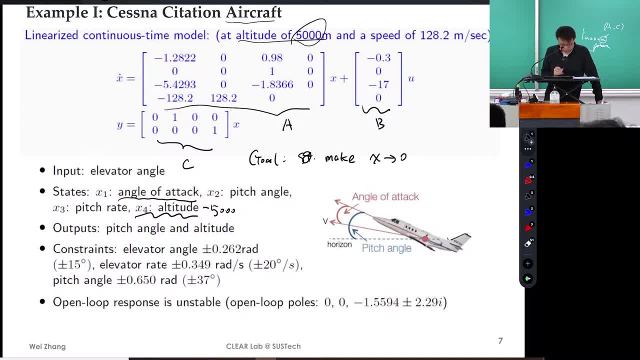 That's stabilization problem, But I have some constraints here. Right, I have. The pitch angle cannot be bigger or equal. So elevator angle is the control. by the way, You know the elevator angle And elevator range. that means the change of the angle cannot be too fast. 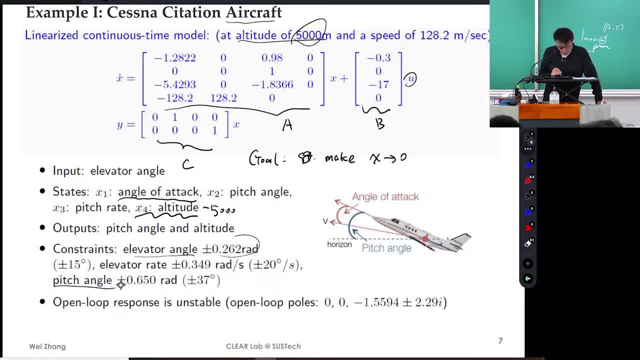 And the pitch angle. that's a state constraint. I cannot have a too large pitch angle, Otherwise I will crash Right, You will lose your control. You specify this objective, Okay, Okay, So is this the optimal control problem? 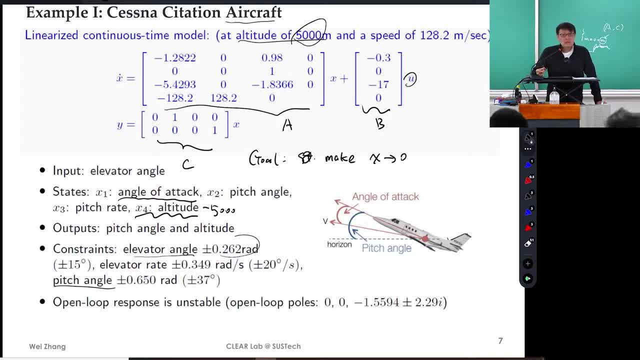 Yes, It's Okay. So, whatever problem is our superficially imposed things, right, It's our belief. As I mentioned, you can view all the control problem as optimal control problem, All Including this one. Right, You don't have to. 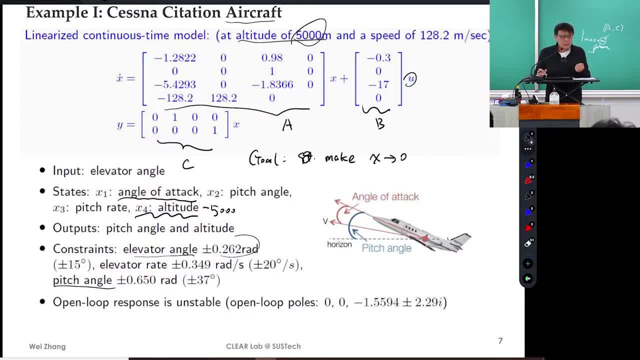 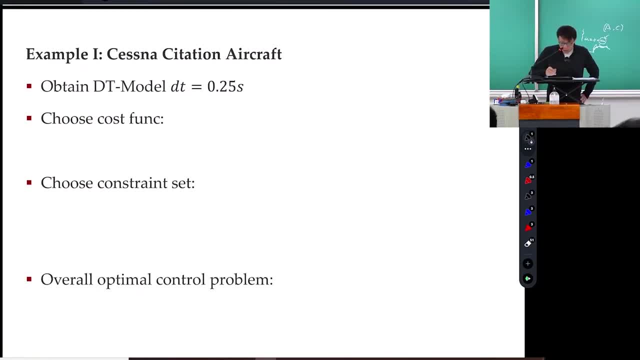 You can just say: I want to design a pole placement problem. Okay, That's fine, We can do this as optimal control problem. Let's see how we can do it. The DT model: Let's do discrete time Right. So I have A, B, C, D now. 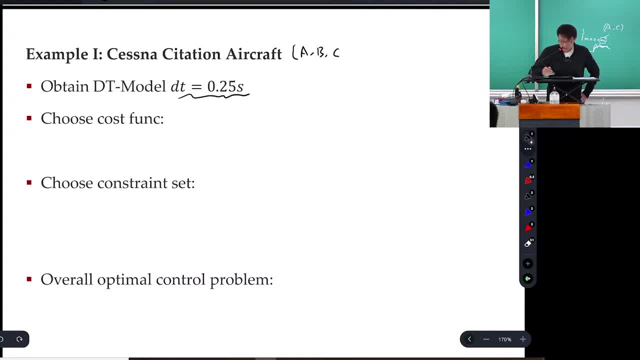 Do I have D? I don't Right. So then I can have XK plus one equal to AXKADXK, plus BDUK And YK equal to CDXK, With discrete addition step: 0.25 seconds. Okay. 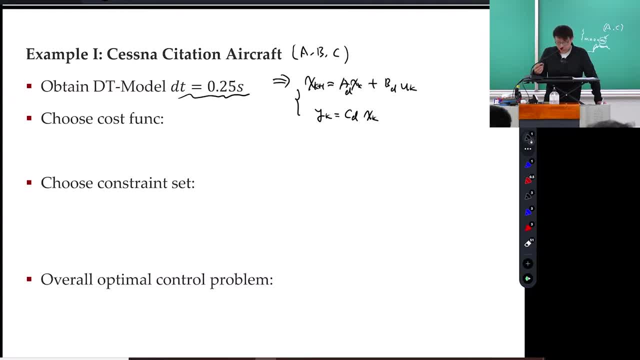 We can do it. I will show you similar examples, maybe later. Okay, We can have discrete time model, that we are studying discrete time model. We have been studying discrete time model for the entire semester. Then we can choose cost function. What would be a good cost function for this example? 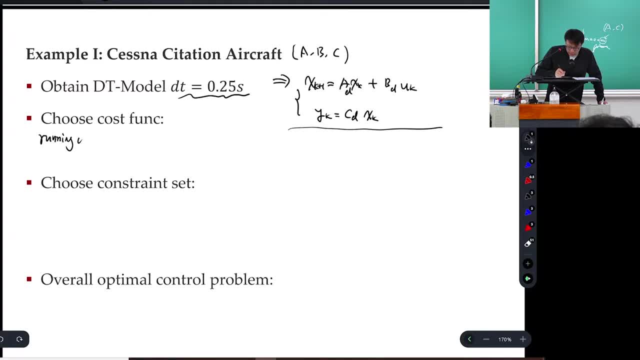 There's two things right: Running cost. There's no unique way to specify them. As long as they reflect what you want, then it's fine. Cost function would be XKUK, The running cost. I will see squared plus UK squared. 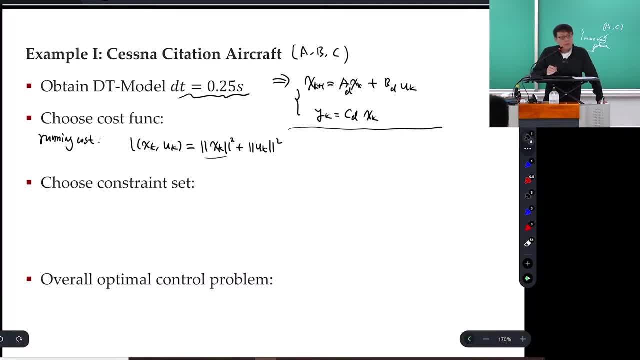 Okay, I want the minimum effort And I want the XK to be small, As small as possible. Okay, This cost will be imposed or be accumulated over its time. Whenever you have a non-zero state, your cost will increase. Okay. 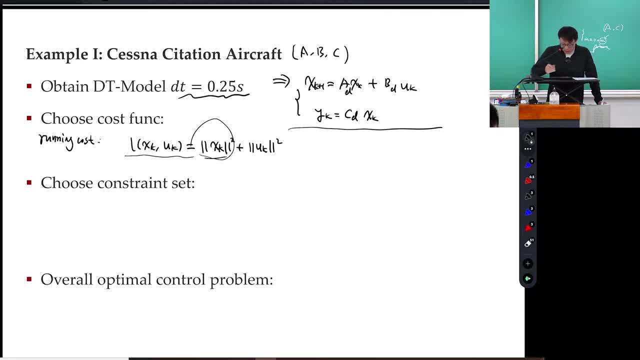 You want to minimize it. Also, we can have a running cost, a terminal cost, which is G of XN. I can also say: this is my squared, Okay. So maybe Xiaohan wants something else. right Could be he wants. this cost will be 100 XK squared plus UK squared. 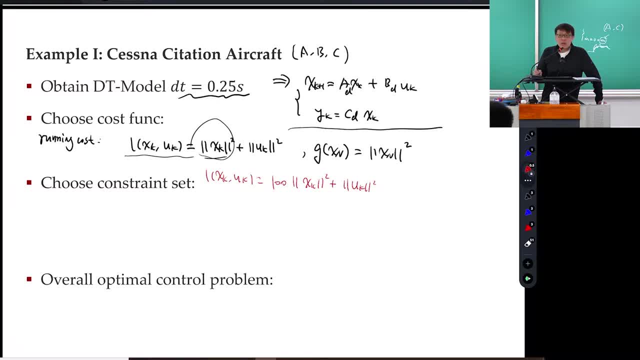 Is this okay? Whatever cost is okay. right, It really matters whether that reflects what you want. This cost differs from this cost. What's the difference? What's the difference? Panel lights more about state deviation And you care less about your control energy. 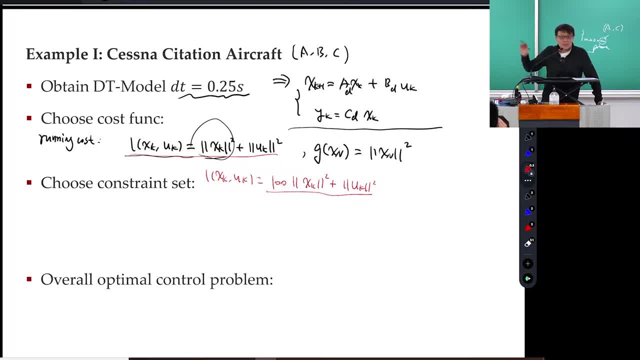 So you don't care about how much gas I waste, How much fuel I wasted, So I just care about my state deviation. So then you may, as a result you may- have a control trajectory that convert to zero faster. 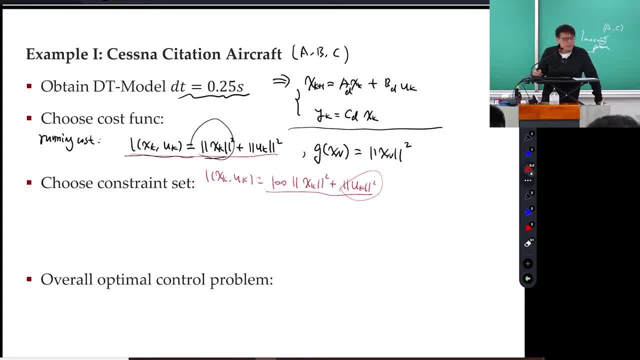 But may have a larger control effort. Okay, You can. by designing your cost, you are telling the system what you really want. Okay, And also you can choose constraint set. In this case, for example, the state constraint- Well, okay. 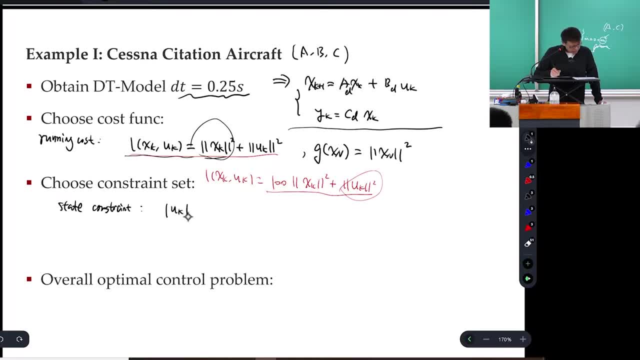 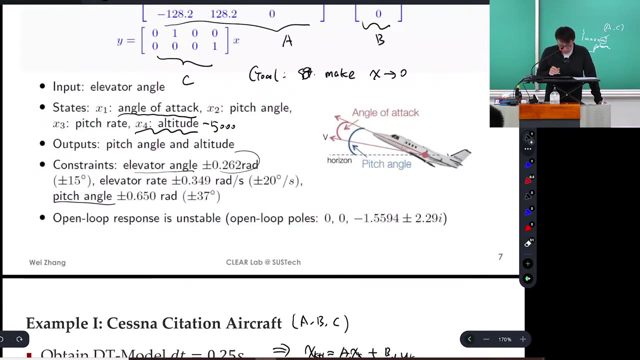 Let me write it down: UK, that's not state control constraint as well. UK is less than 0.26.. And my second state, SK of 2, should be less than 0.65.. Right, What is it? 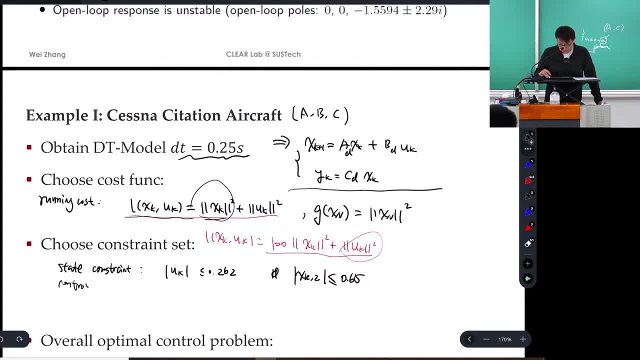 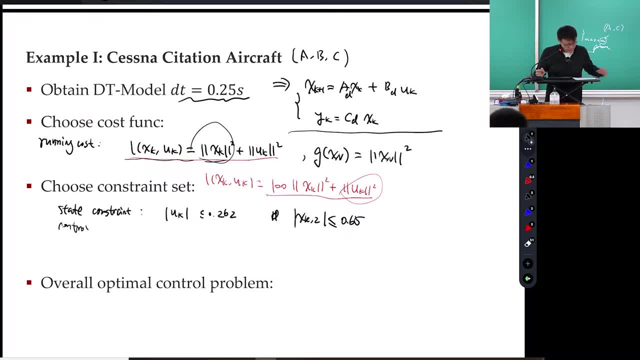 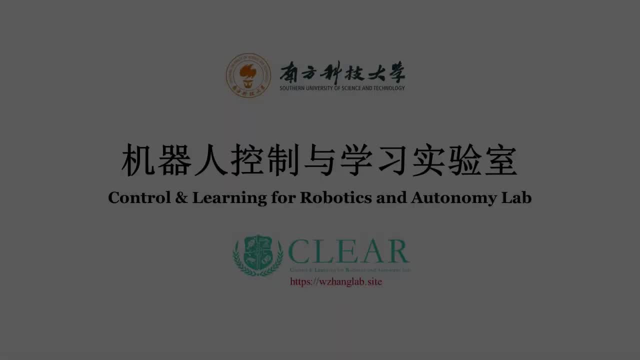 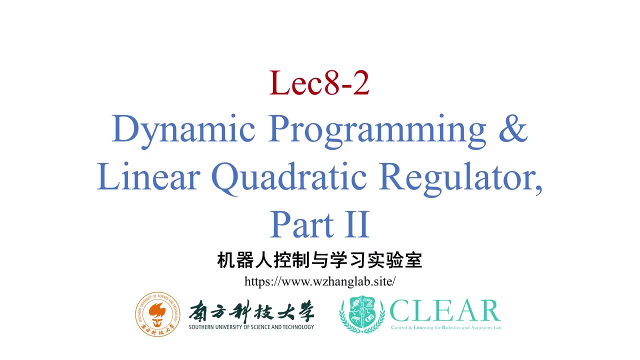 Is this guy? The pitch angle is the second state Right, So I will not. I will do this next time. Okay, Let's take a break. Oh, I forgot the quiz again. All right, Let's get started. 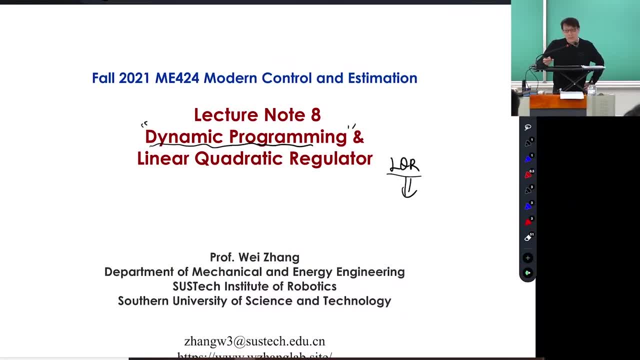 It's the last lecture, which is lecture note 6.. Not last lecture, I think it will be. hopefully it will be lecture 9.. Today we are going to finish lecture note 8, hopefully Okay. This lecture is about optimal control. 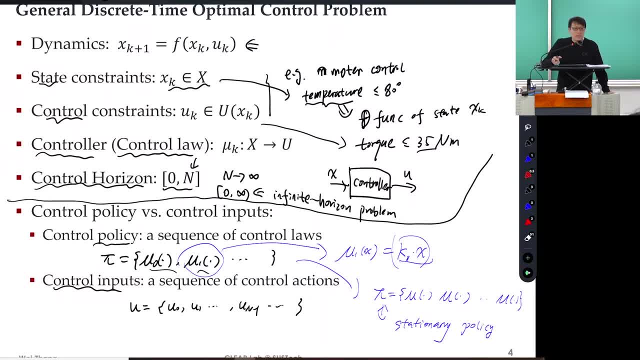 So far we have learned how to design what Control based on pole placement. Okay, If we don't know the state, we can use observer. If the system dynamic has uncertainty, we should use common filter to observe the state. Once you have the state, you can do state feedback control. 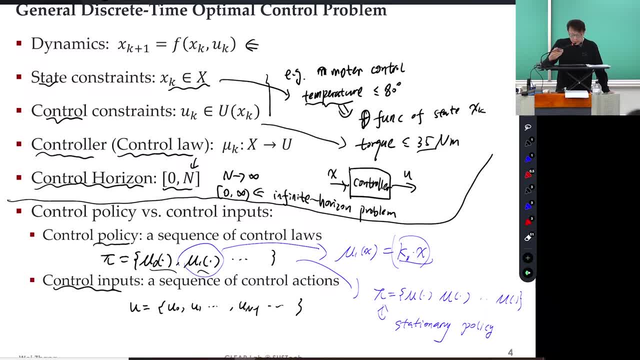 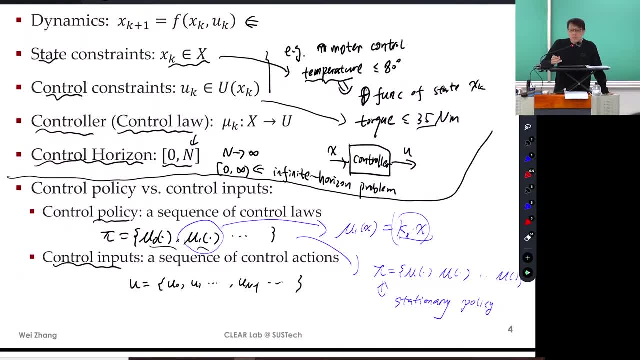 Right And based on pole placement, because that affects the closed loop dynamics. The last time we started talking about optimal control- And that's, I think it will be a unified view for almost all the control design problems- Some problem by nature is optimal control problem. 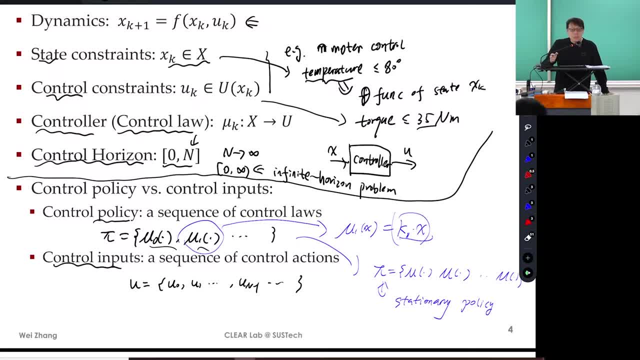 Some of them may not look like an optimal control problem to start with, But you can think of them or reverse, engineer them to become optimal control problem, And so I think this. As I mentioned last time, almost all the control problems can be stated or formulated. 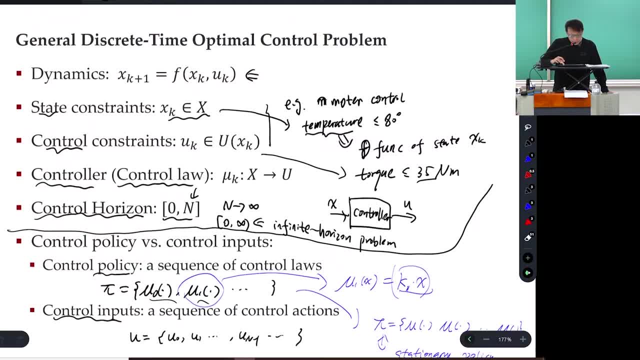 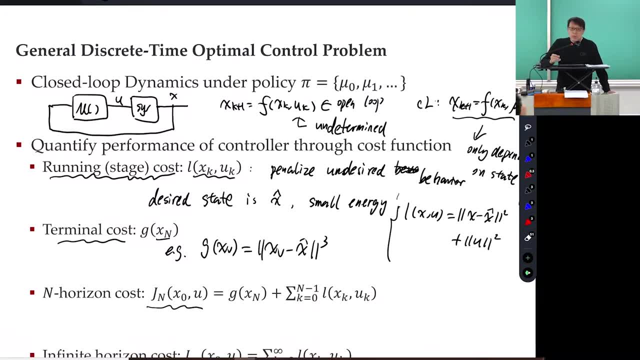 as an optimal control problem. Okay, Now we start talking about the formulation. I think the key is that you should know your objective. So, whatever your control design objective- I mean Whatever your objective is, it doesn't matter what it is. 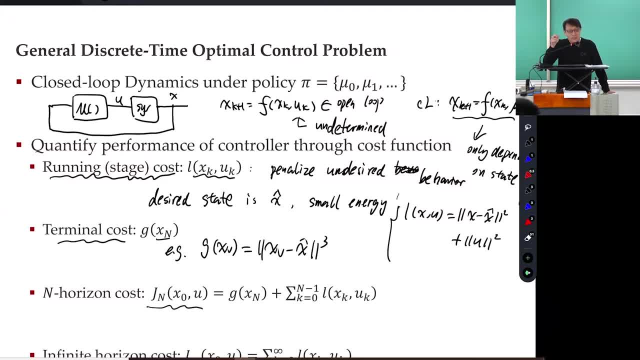 You should be able to convert that into a cost function. Okay, You want to stabilize it. You want to make it more stable. You want to make the transient less oscillatory. You want to reduce the percent overshoot. You want to track faster. 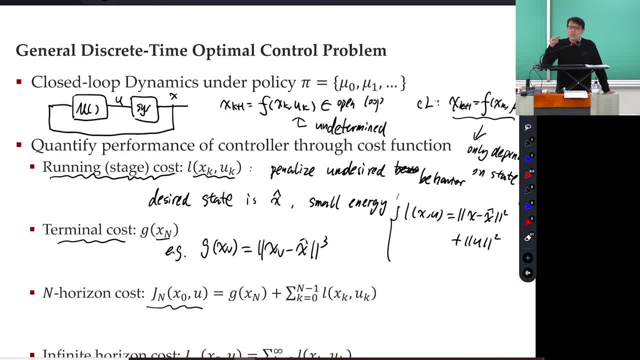 All of these things should be able to convert it to a cost function. Once all of us agree on a cost function, then we can design a control to minimize the cost, In other words, to optimize the performance, The performance that you care. 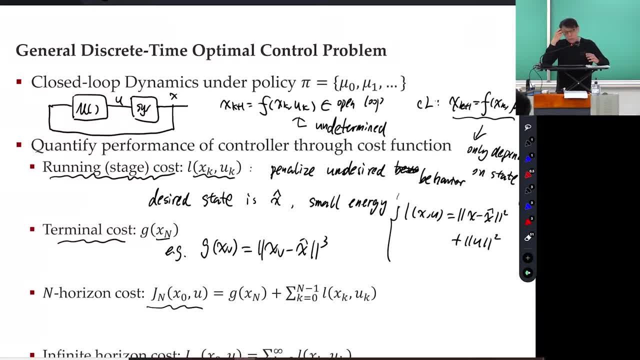 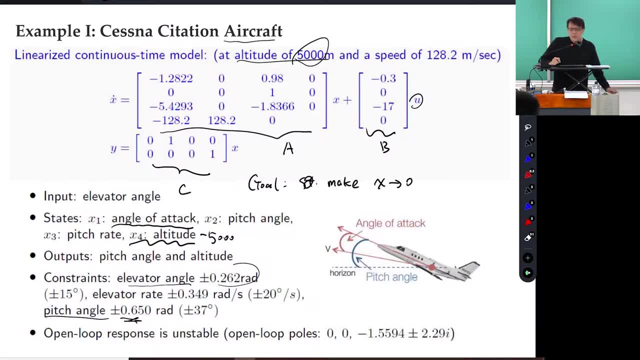 And that becomes, And how to do this. This is basically the topic for optimal control. We started talking about this last time And we started talking about this example- I think right- And as the first example When you see engineering problem. 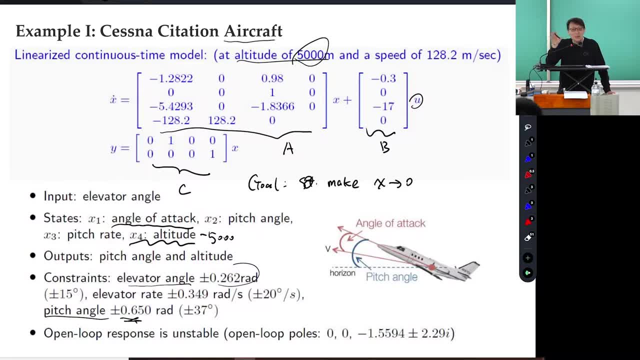 I don't think they will have optimal control problem statement for you. Unless you're in the exam Right Or homework, I will tell you okay to solve this optimal control problem. In reality, you were given the problem described by plain English. 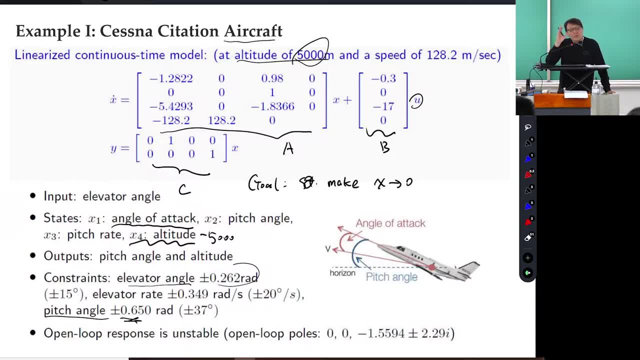 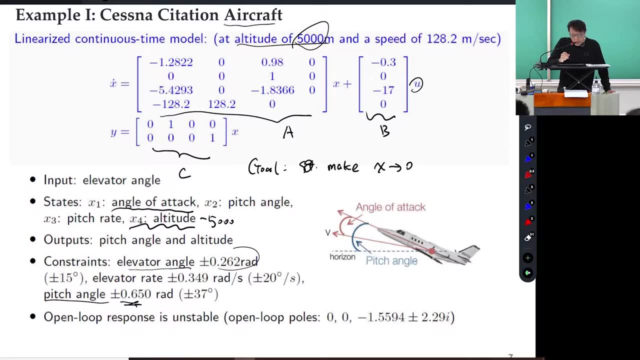 Or Chinese, Whatever, Okay, And you should be able to convert what you want to do into a kind of cost function. Right, This is the example. We start talking about this. Last time we talked about this is the model for an aircraft. 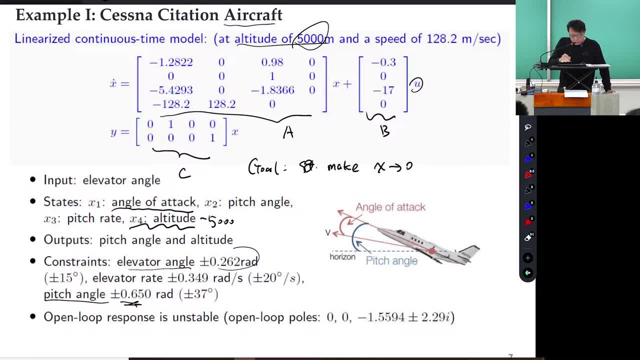 This is kind of a real aircraft And those parameters are, I would say, practical. It's not exact But it's practical: Hold on, And this is a continuous time system And we linearize it around certain operating point. Now here I want to emphasize that this state is deviation from desired state. 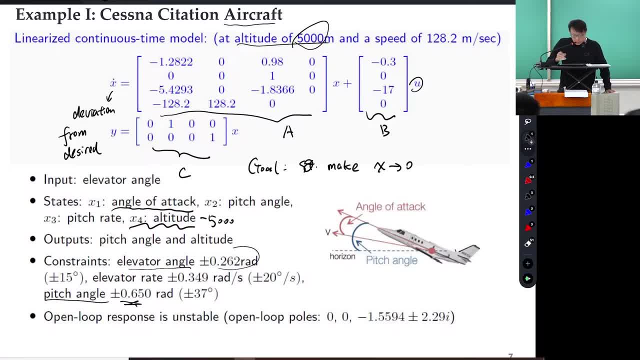 Okay, So we want that to be zero. For example, when I say X1 is angle of attack, that means deviation from your desired angle of attack. That desire may be zero or maybe not, I don't care. We only care about the difference. 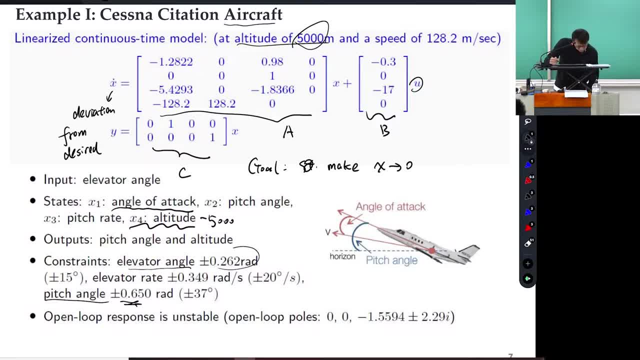 Or deviation from the desired, And altitude means deviation from desired. Here is the linearization point: It's 5,000 meters. So that's the deviation from 5,000 meters. Okay, There's a piece angle and piece rate. 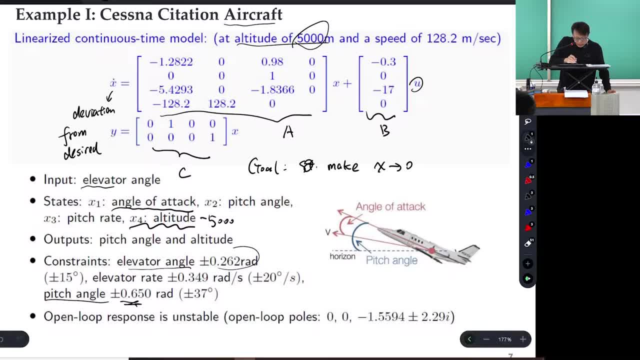 Those are four states And the only one input is the elevator angle. Okay, And the angle can be controlled, But it also has some constraints. The elevator angle cannot be larger than certain degrees And also the change, the rate to change. it also should be less than certain speed. 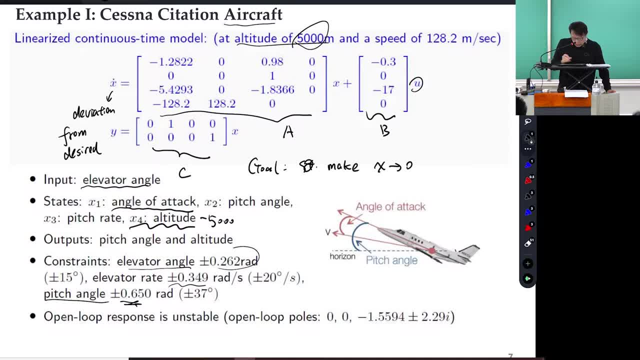 Okay, So that's the statement. And the system is unstable. Open loop unstable. It means that if you don't control the elevator angle, you crash Right. It's not. It's like the mobile robot on the ground is stable. 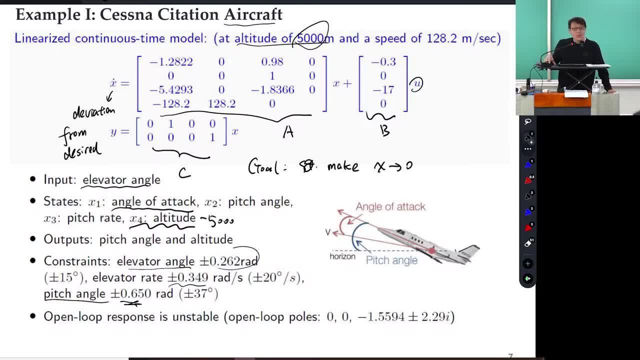 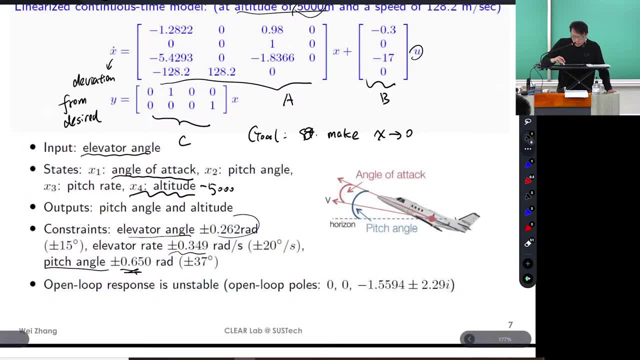 If you don't control it, it stays there. But this system, if you don't control it, it will fall, It will crash. So that's called open loop, unstable. So our goal- I didn't say our goal- 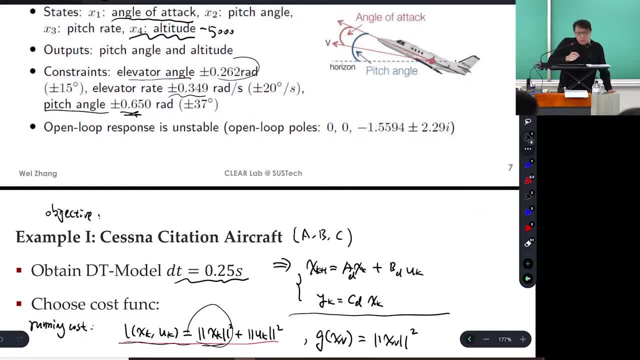 Our objective, roughly speaking, is to regulate Right, To drive X to zero with small energy. Let me not use energy. energy, A small control effort, Loosely speaking. Okay, If I don't need to apply any control to achieve this goal, then that will be better. 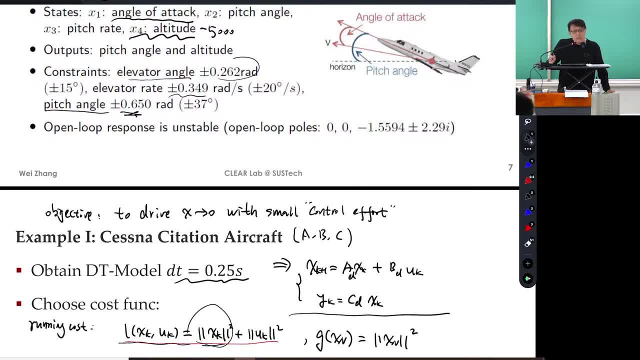 Okay, I want to use the minimum or smallest control effort to drive my state to desired Okay. To zero means to desired value. Okay, If you push away or have some disturbance, you deviate from your desired values, then you want to move back to it. 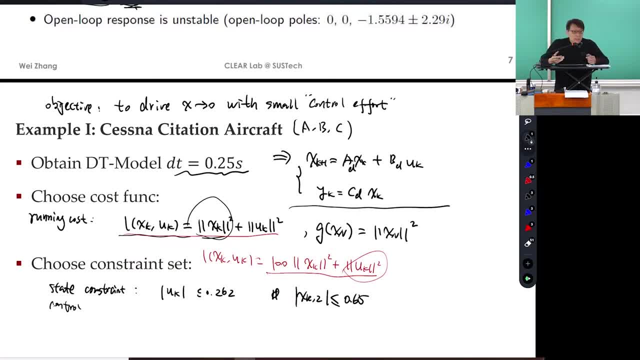 Okay, So that's the goal. It's not an optimal control problem, Right, But we can. What we can define is we can formulate this problem as different ways. In particular, the optimal control formulation can be given as follows: Right. 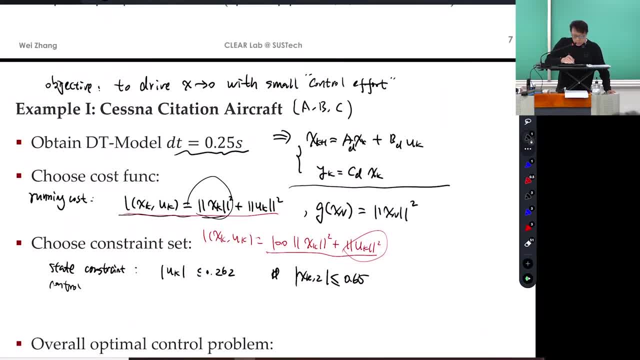 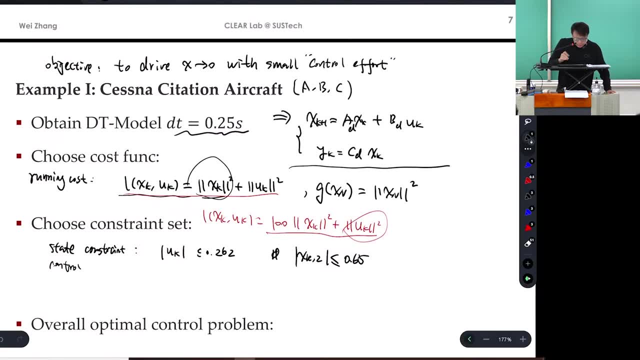 Since we're dealing with most of the time, it's the discrete time model, let's choose a discretization time step, which is .25 seconds. Okay, And now we need to choose cost function, As I mentioned last time. cost function. 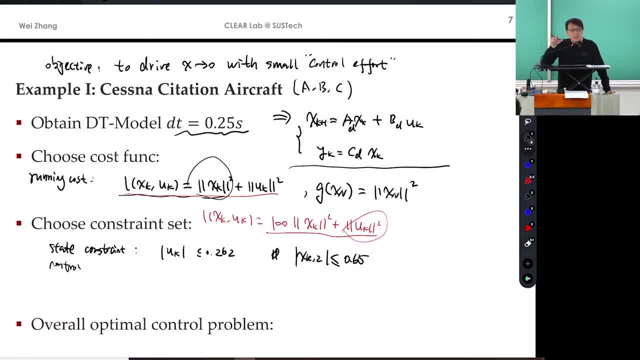 Cost function has two parts. One is called Terminal cost, Right. The other one is called running cost. Running cost is the penalization each time Okay, And terminal cost is only penalized the final state. Suppose you have a final time, finite time horizon. 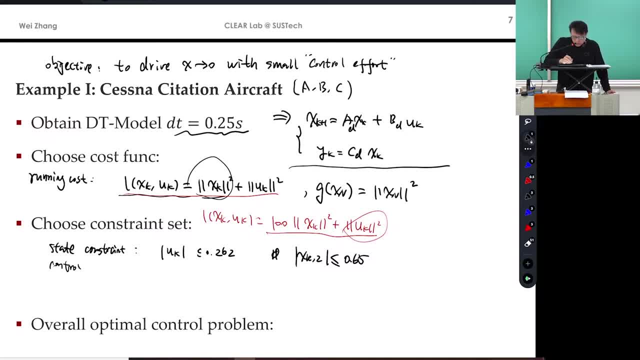 Okay. In this case the running cost is, I put it- like a quadratic function, like a norm of the vector. Can we come up with other running costs? Are you okay with it? I'm fine with any kind of running cost that loosely reflects my goal. 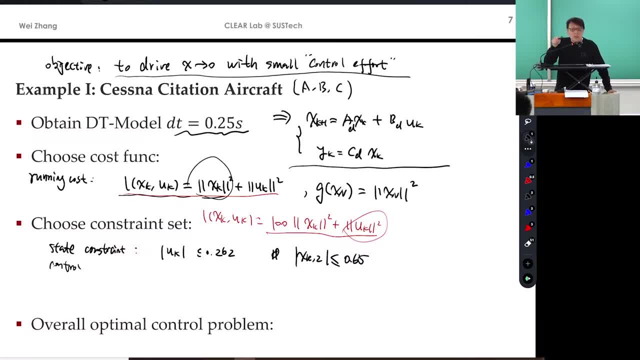 Okay. But if you have a more concrete goal- so, for example, you know the price of your gas gasoline Right- And you want to minimize the gas cost, That has to have a more concrete metric: 最小花你的油钱。. 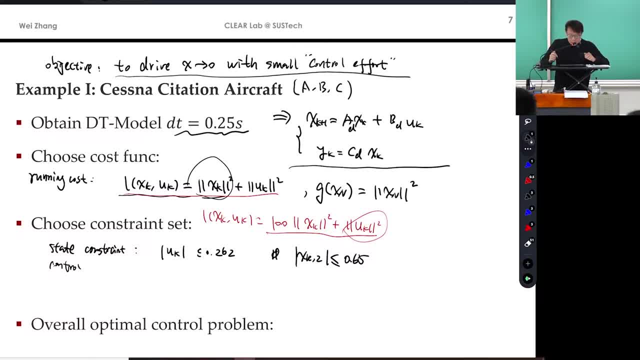 Okay, that's fine. That has a concrete number for the cost For this case. we just say: okay, we want these two to be small. Each time you are non-zero, I penalize it. Okay, So the terminal cost here is also. 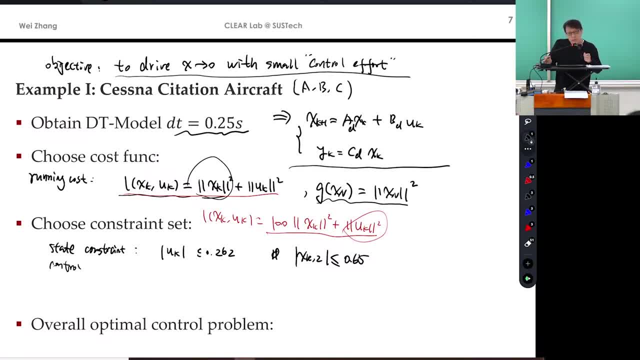 We don't have a specific terminal goal. We want it to be zero. But if it's not zero, it's okay. If you deviate a little bit from zero, it's okay, But we want it to be as close to zero as possible. 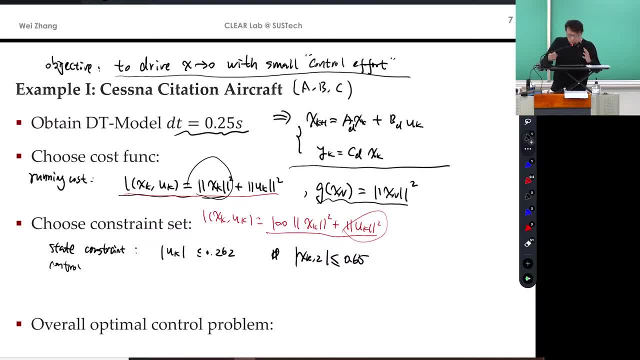 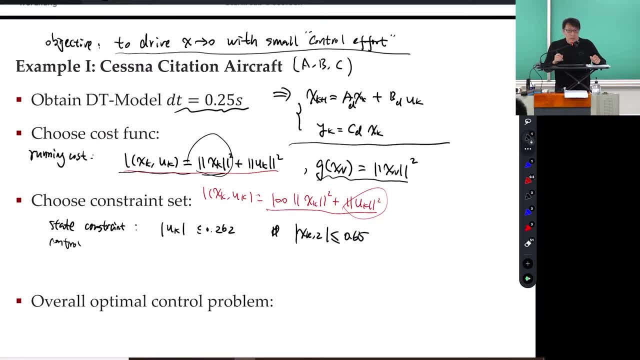 Right, So let's also put this one. You can put 100 or whatever that roughly reflects this goal, And then I can. Another important thing is that not only the cost, okay, you also have restrictions, constraints. You cannot do arbitrary things. 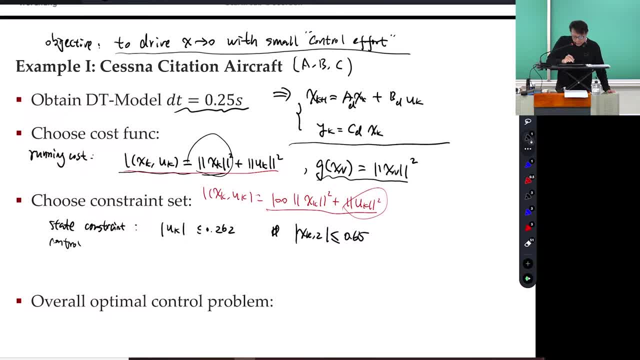 Right. So the constraint here is, first of all, the magnitude of the control action. The action is an elevated angle. The angle cannot be larger or smaller, Larger than this 0.26.. And also this: What is this? 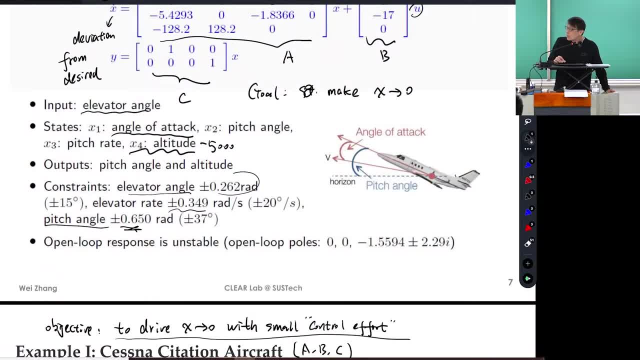 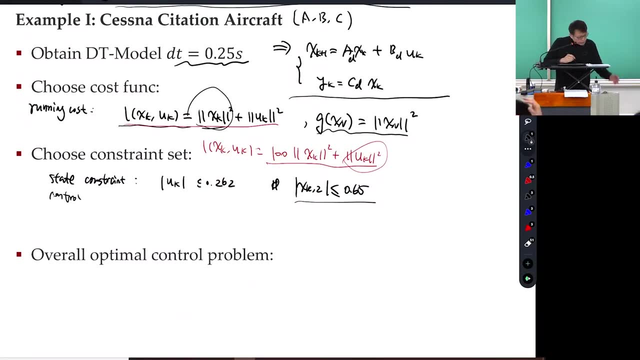 The pitch angle cannot be too large. Any questions. If the pitch angle is too large, then that's somehow valid. That's my assumption, that maybe my linearization model will be invalid. Okay, So that also should be considered. And what other constraints I have? 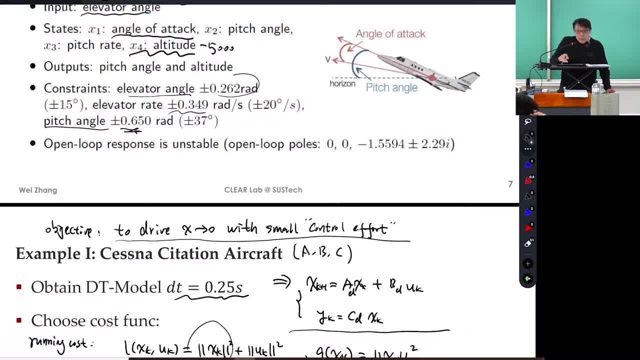 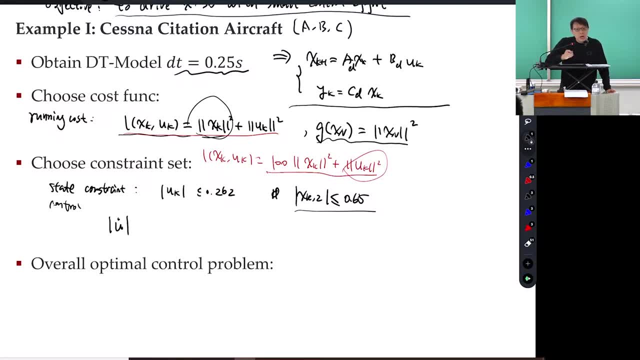 For example, I have this one right Elevator rate. What does this mean? U dot Right, U dot. The change of U cannot be too fast, Otherwise the lower level controller cannot accomplish this Right. So this is less than 0.349.. 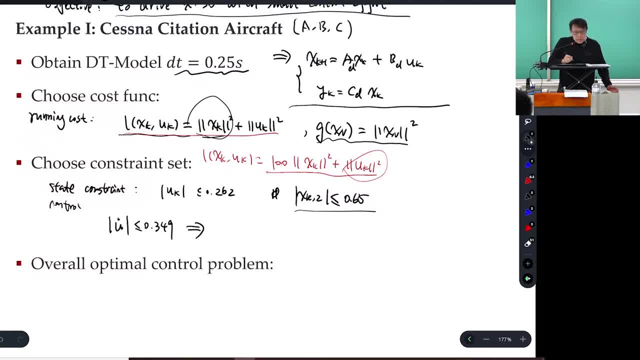 But this is a continuous time model. But what does this mean? I can formulate this as a U minus U minus 1, less than or equal to 0.349 times delta T. Okay, That roughly reflects what I want. It's constraint. 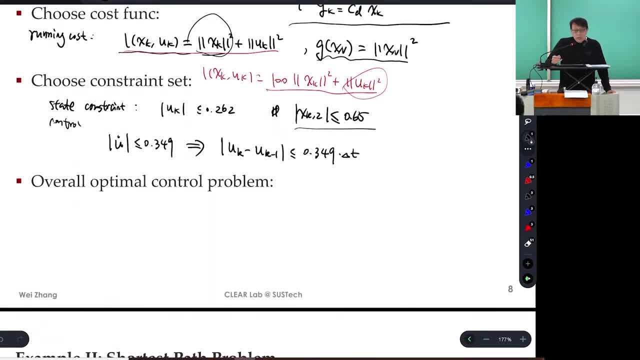 It's constraint on the control. All right, So now we have our objective. If you purely have objective, that doesn't mean anything. Right, You have to know your boundaries, What you can do, Okay, Your control actions. That means the constraint. 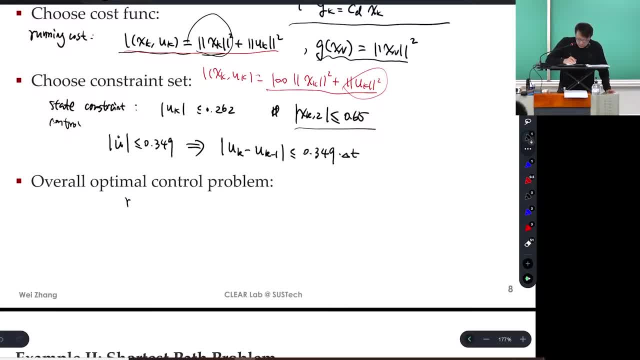 So, overall, the optimal control problem is the following: So minimize summation of from k equal to 0 to n minus 1.. L, X, K, U, K, That's the summation of random cost. Each time you'll penalize deviation from your desired state. 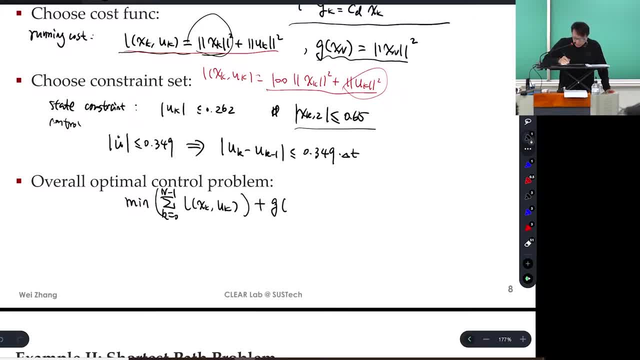 Okay, And then plus a terminal cost which only penalizes the last state. Okay, Added the final step. So in the subject 2, I need to consider constraints. First of all the dynamical system constraints: The x and the k are not freely changeable. 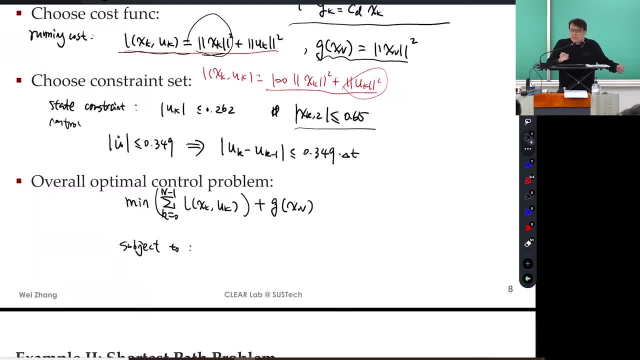 They're not free. You cannot arbitrary pick x, k and the u k. They are. They need to satisfy the dynamical system equations, which is, in this case, is linear Right. So k plus 1 equal to ax k. 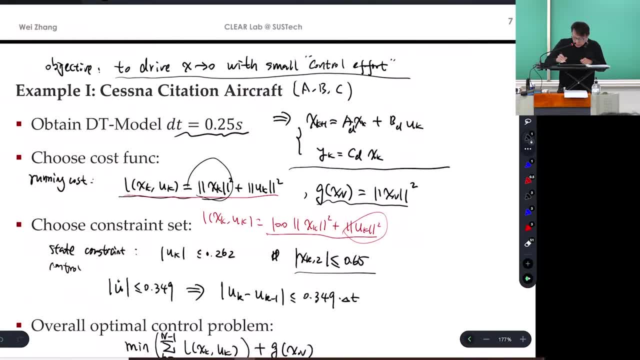 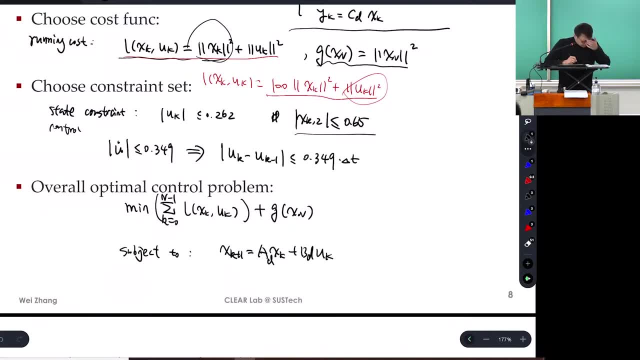 I said it's ad right Discrete time. Did I say that This is ad bd, Right? So this ad plus bd u k. This is my relation between x k u k and x k plus 1.. 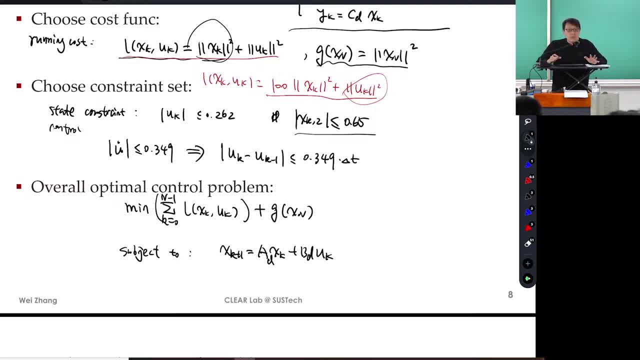 That can be viewed as a constraint for an optimization problem. So these three variables need to satisfy this condition. Okay, And also I know u k has to be less than equal to 0.262.. And the second coordinate of x, k. 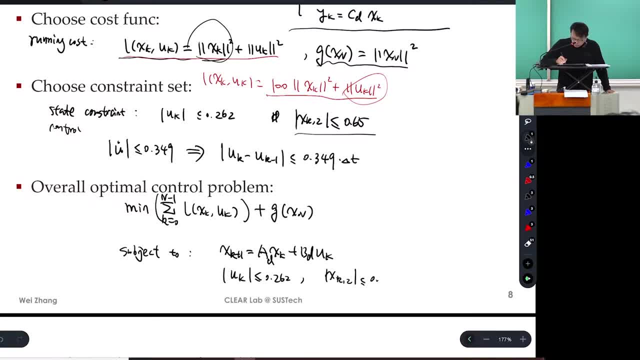 The second coordinate of x k should be less than equal to 0.65.. And also, my u k minus u k minus 1 should be less than 394 delta t, Delta t, here is what, 25.. Right. 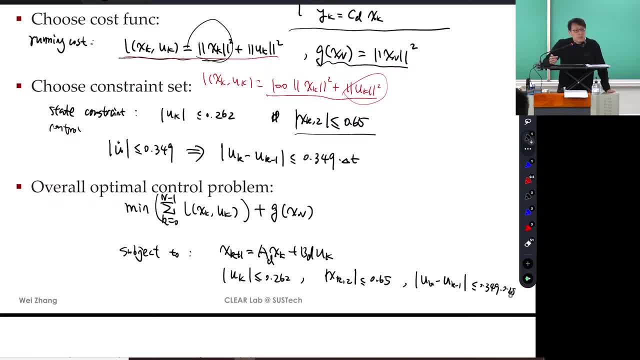 0.25.. So I can just write it down. Is this an optimization problem? Do you know what an optimization problem is? Minimize fx subject to x satisfied certain conditions. That's an optimization problem. This is an optimization problem. 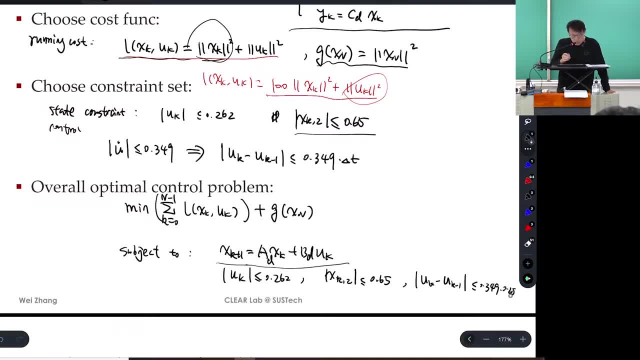 But it has a sequential nature, It has this dynamical system involved, So it also can be viewed as an optimal control problem. I want to ask you: what is the optimization variable? What do I mean by optimization variable? What are you trying to tune, to select? 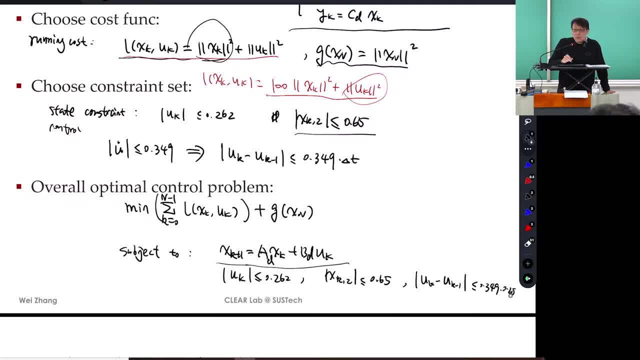 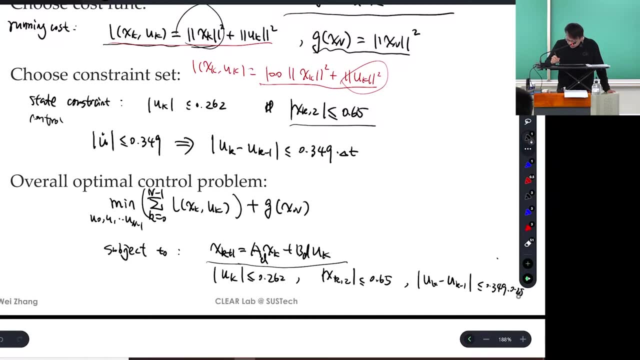 X and u, Only u right. So u0, u1, all the way to u and minus 1.. You have this number of u's, This is less. What is it? So? you cannot see it. So this is: 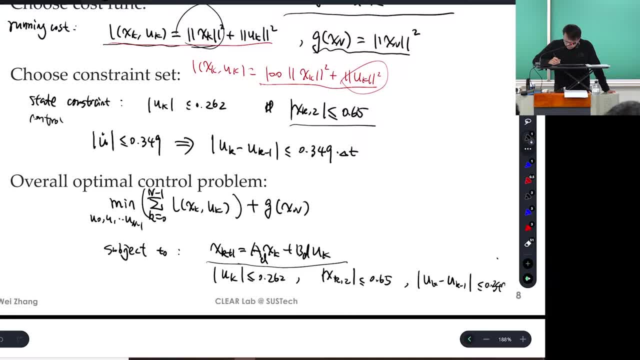 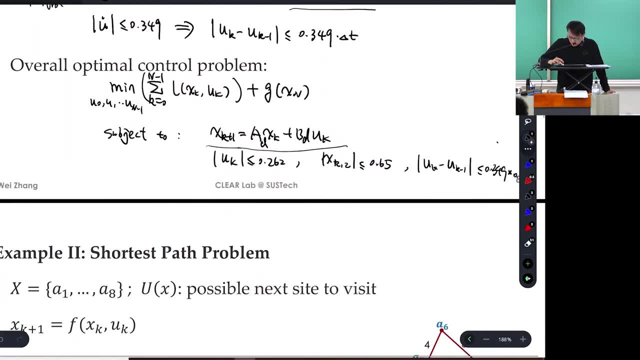 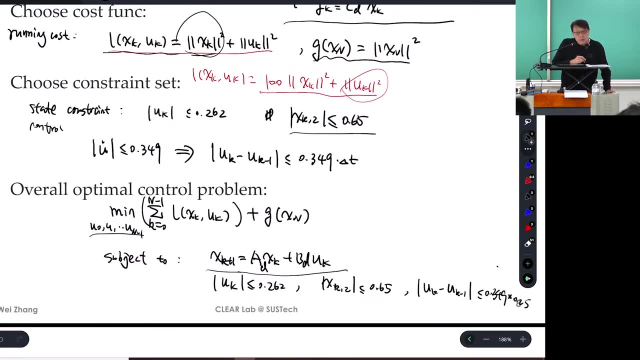 3 times 0.25.. Okay, Only you can see from here. All right, So those are the optimization variables. Once they are determined, then x, k are determined, But you need to start from a x0.. Right. 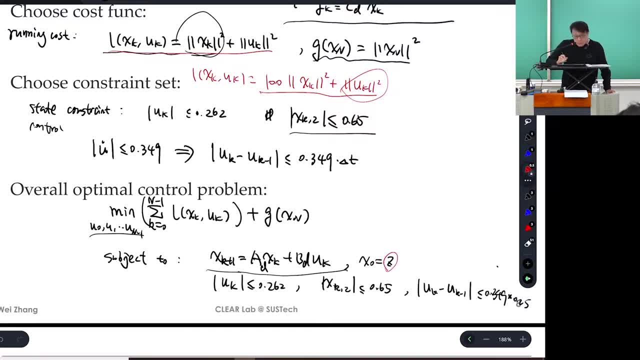 x0 needs to be given. Suppose I call x0.. A, z, Okay, So, So the solution of this, So this thing, It depends on z. only So this problem. Of course, if I optimize over u, I pick the best one. 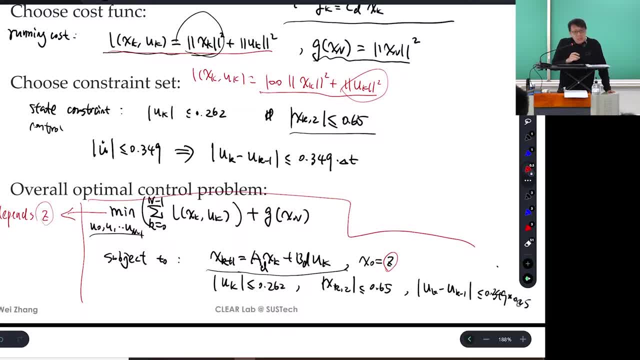 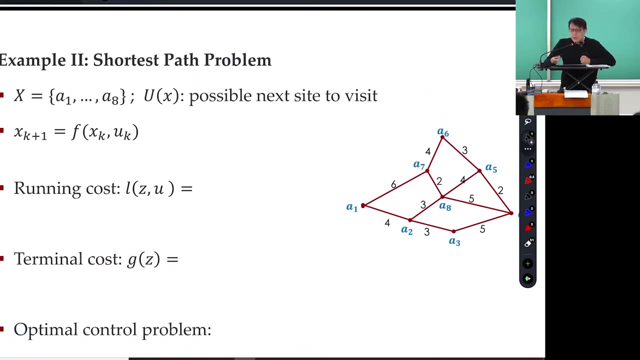 Right, That's my optimizer And the whole problem somehow is parameterized by my initial state. If I change my initial state, this optimization problem changes. Okay, The optimal solution will also change accordingly. All right, That's enough. Let's look at another example that you may not view as an optimal control problem, but 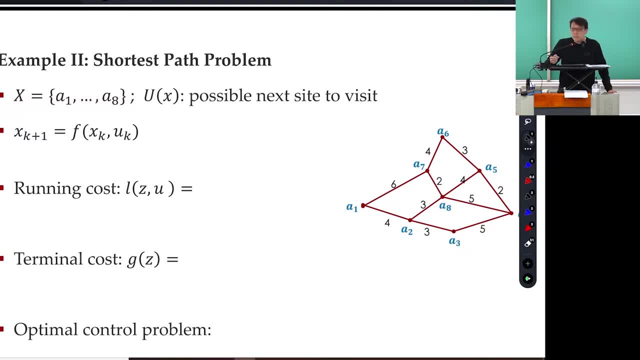 it essentially is: It's a shortest path problem, Or when you're booking tickets, it's also So airfare problem. So what's the optimal cost to go from Shenzhen to Guangzhou? Guangzhou is too short. 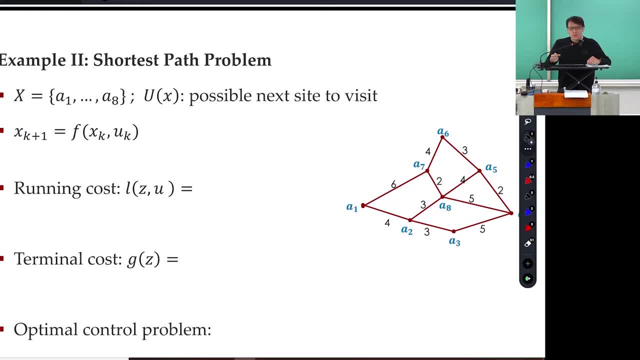 No, So let's go to the US. We cannot go there, All right, So you need to take multiple, You need to take transit Right. Then you need to find the best path, Right, Okay, Or you drive your car. 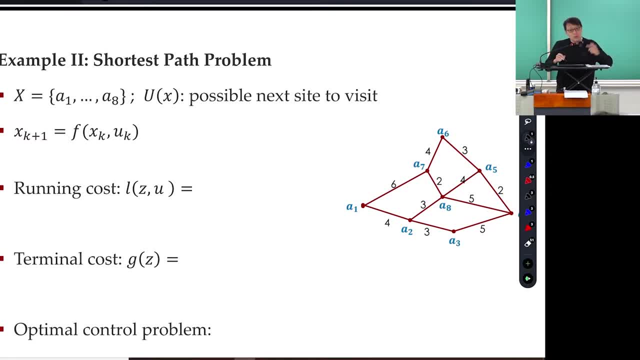 What's your best Kind of path from Shenzhen to Beijing, for example? That's somehow this kind of routing problem or path planning problem, Right? So suppose that we are given this figure, this graph, and I think this is. 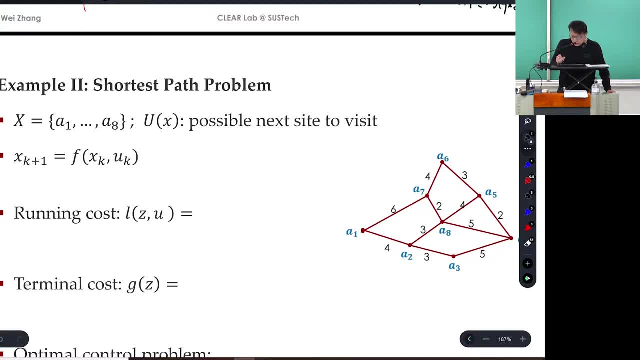 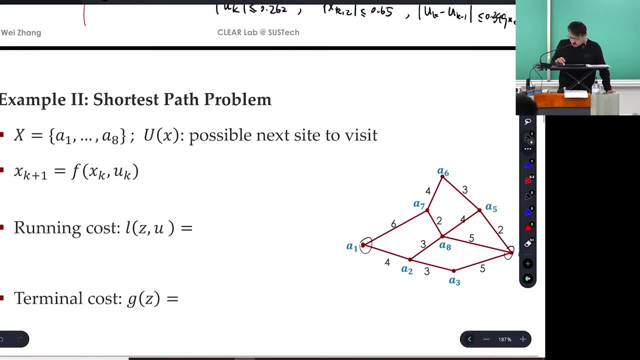 The meaning is kind of apparent. So those are the cities. Okay, I want to visit, Suppose I start from A1.. I want to get to A4.. Here is A4. You cannot see it. I don't know how to move this guys. 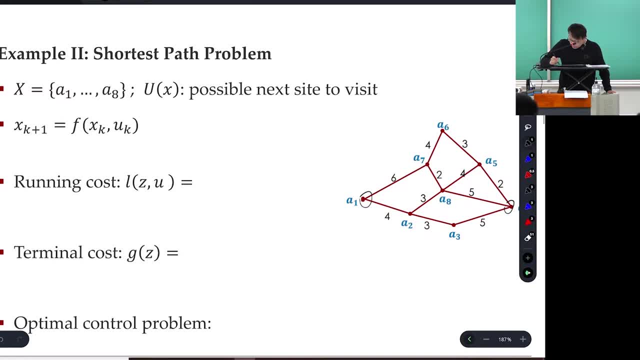 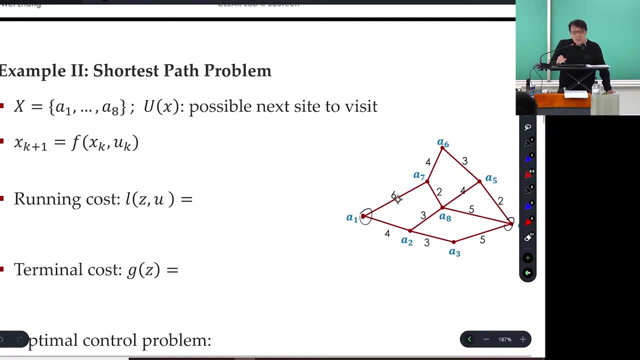 Okay, So I can't move this. Anyway, that's fine. So this is A4.. So it's the number, it means the length, Okay, Between the two cities. let's say that The length Okay. 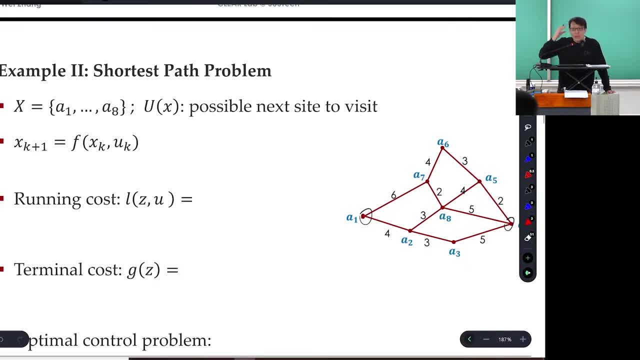 So I want to find the best, shortest path, And in your brain, when you do this, you will just enumerate all the possible paths, possible paths, and you will find it. I think this is easy enough. You can do it by inspection, without writing things down. But let's consider a 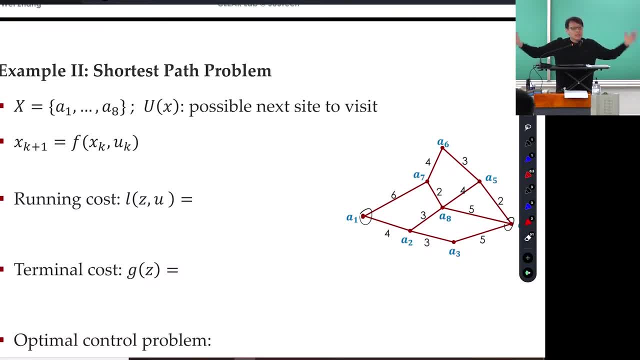 formal way to consider. Suppose you have a big- okay, a thousand by a thousand cities network, right, So then it's hard for you to do it. Then you have to program your computer to do it. and how to formalize it There are different. 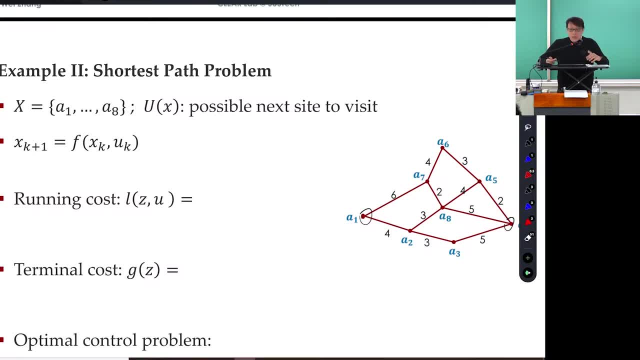 ways and there's a pure CS ways- Okay, computer scientist ways, And what I'm talking about here is not the most efficient, but it's more general framework. Let's think about them as a state-space dynamical system. Can you think that way? What's your state? Let's think about the state now, As I mentioned, 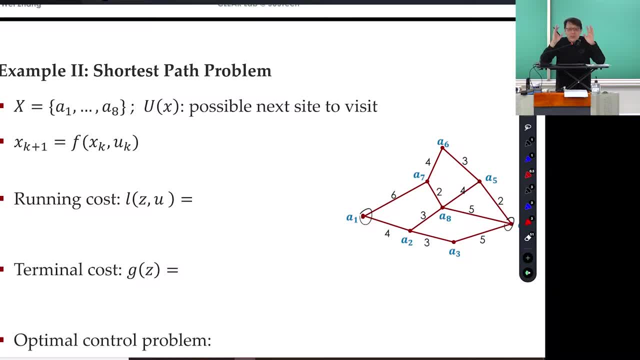 there's no one tell you what are. the state is Okay, those are models, and all models are wrong, sometimes right. So it's really reflect what you want or not. There's different ways to view the same problem, In particular this problem. we can view it different ways. 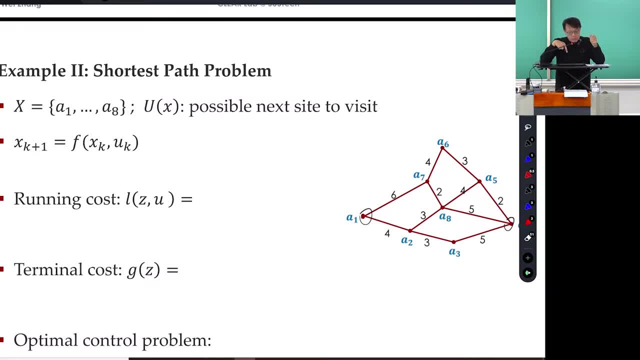 but let's consider a state space approach. okay, I think that's very general. The state space is all the cities. Suppose we have eight cities, right, That's the state space. Previously our x, typically in Rn or in R right. 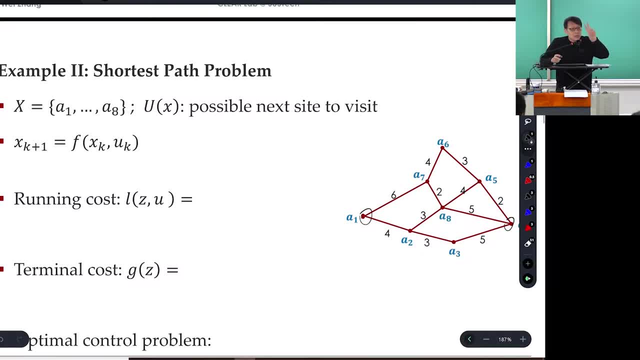 It's a continuous variable, but here x can take values, eight values, That's fine, right. Each value represent one city. You can think that way, right. And then I have a constraint set. I think this notation I explained last time. 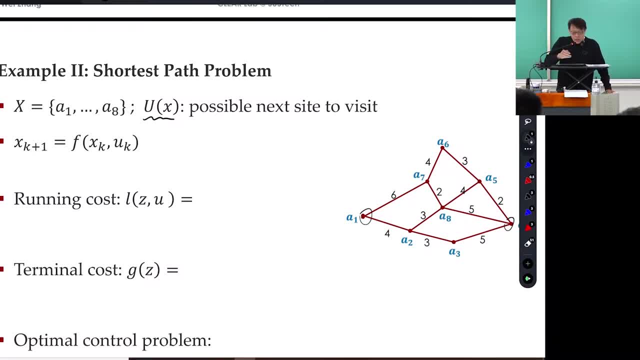 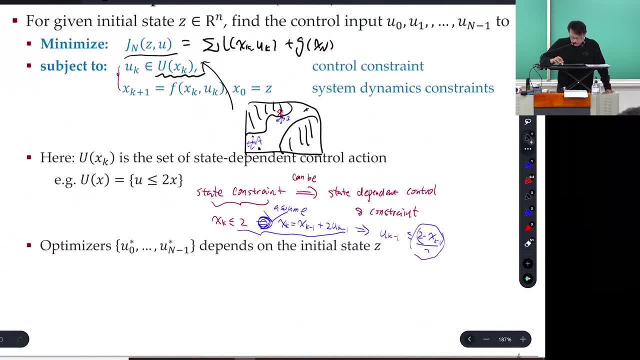 This is available- control action you can take when you are at state x, right, And this thing can be the constraint, can be state dependent, as I have the figure last time, right, You remember, If you are here, your control action. 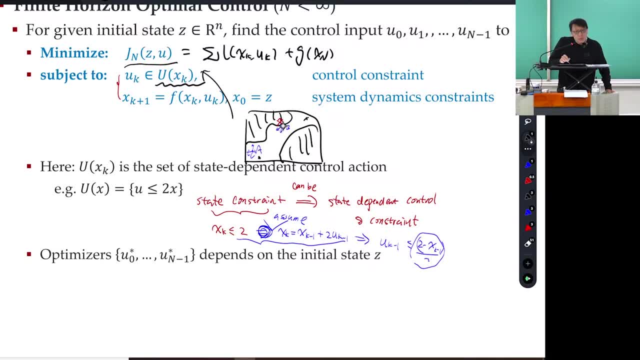 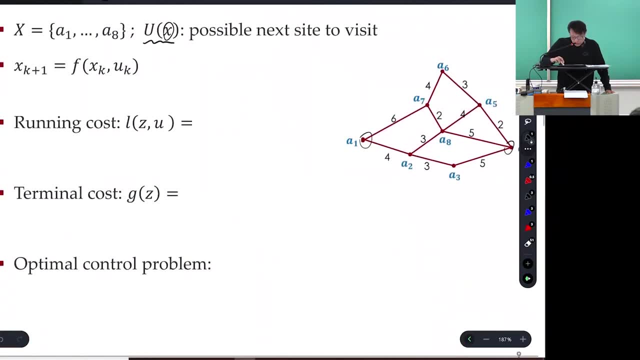 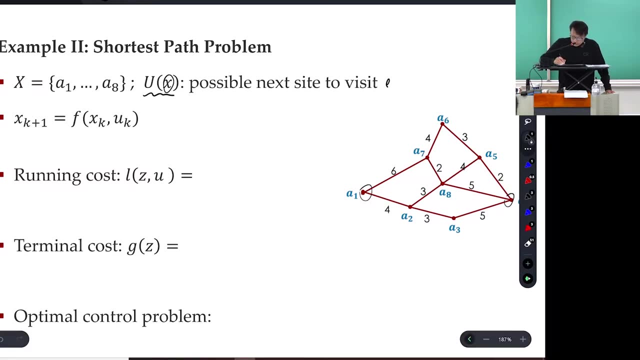 suppose you can move different locations, different direction, versus you are here at the B location, your control action available for you. it's different. Here is the same thing. I will say: this guy is a possible next site to visit. For example, I will say U of, let's say, A7.. 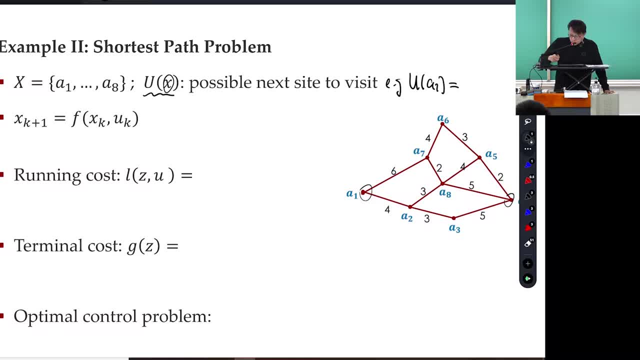 What do you think it is? U of A7, it means, by definition, U of A7 equals U of A7.. How many action I can take at the U7, A7?? Three right, Suppose I can move back okay. 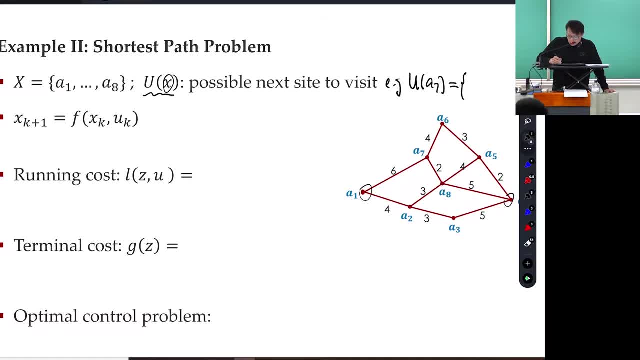 I can go back to A1, I can go to A8, I can go to A6.. So it's A1, A8, A6.. Okay, that's my control action. Although it's discrete, it's still a set. 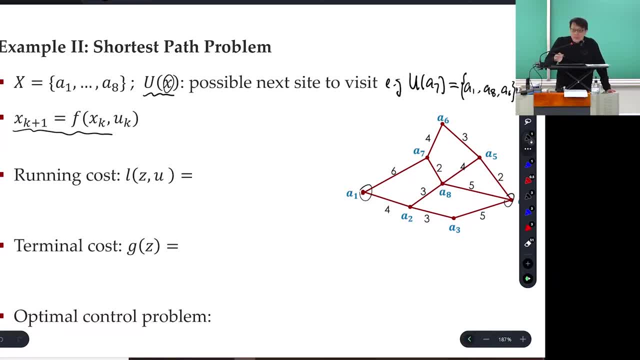 Okay, my dynamical system in discrete time is nothing but state update equation. So, given the current state, given the control action, you specify what the next state is. In this case it's nonlinear, right Of course. it's discrete even. 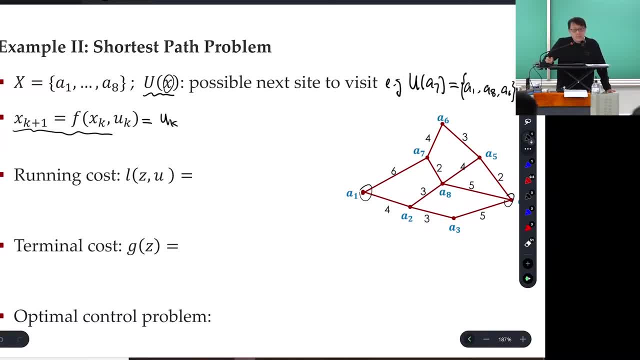 So what is it? It's nothing but U of K, So I can directly control my next state. It's a trivial dynamics, So it's time. you select where you want to go, but you can directly control where you can go. So this is nothing but the. this is directly the next. 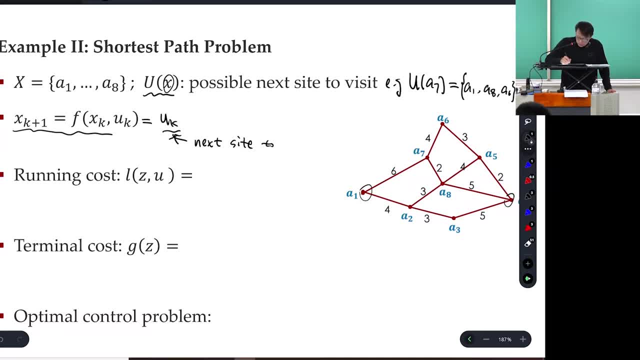 directly state the next set to visit right, Next set to visit Right, and then we can specify depending on our objective. we can specify cost functions. If we want to minimize the total travel time or length, then the running cost is that if you go from 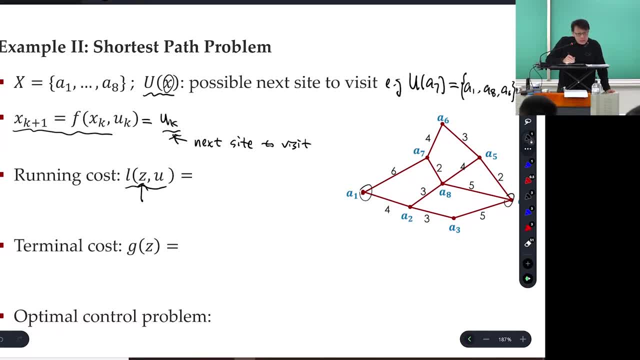 meaning running cost means what It's: the function of the state and the function of the action you take at this state. All right, so I will say this can be viewed as: In this case, it can be viewed as defined as length. 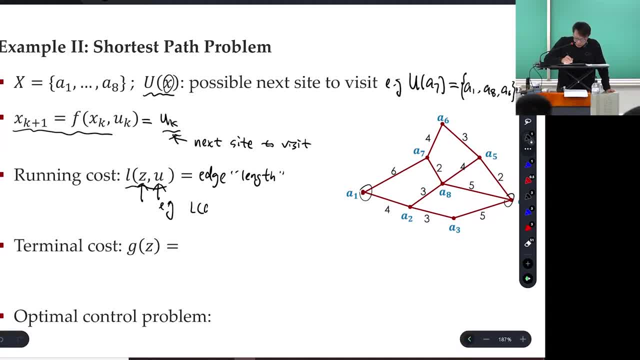 What do I mean by that is, for example, I will say L A1.. U can be A7, right, U is the next one. I want to visit XA1, U equal to A7,. let's say U equal to A7.. 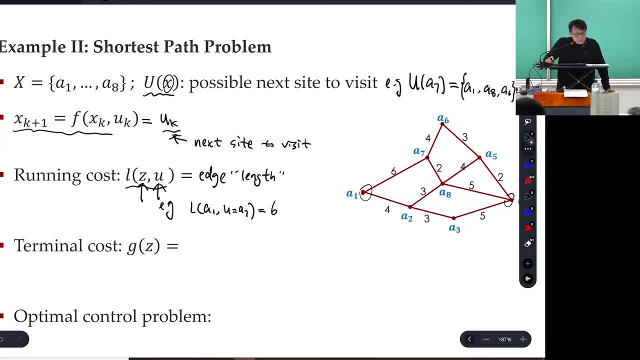 Then this will be this the length. it will be six. It's all notations, right? Any questions A1, A7, equal to six, I will say I'll, let's say A2, I can go A3, right. 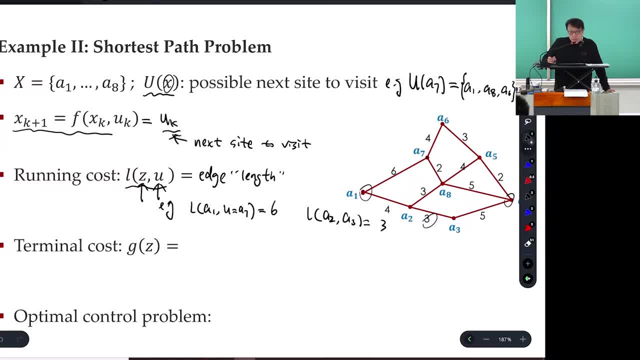 A3, that will be three. It's this length. What about terminal cost? in this case? Do I care where FNL is? Well, I can define either way. I can soft penalize or I can do a little bit extreme in this case. 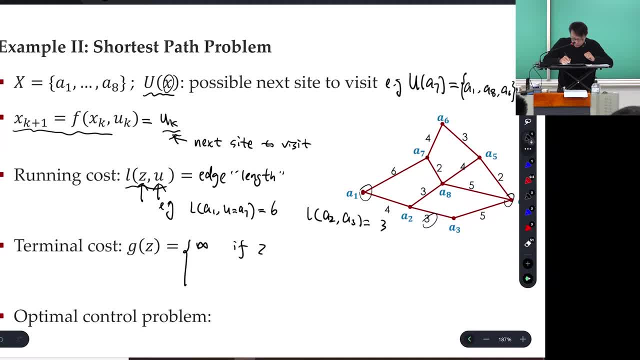 I will say Z, infinity, if Z is not my goal. If I want to go to Beijing, then I eventually go to Shanghai. that means my cost is infinity. Right, and that So that's. if not A4, suppose our goal is to. 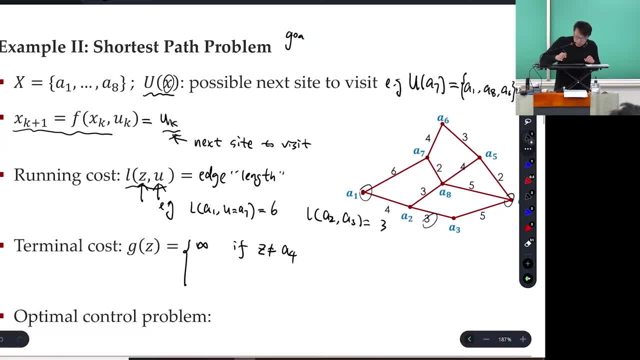 so our goal is to suppose I need to specify our goal- okay, Start from A1,, go to A4 with minimum minimum cost or whatever the distance. So then, if I'm already the final state is A4, why I use Z? 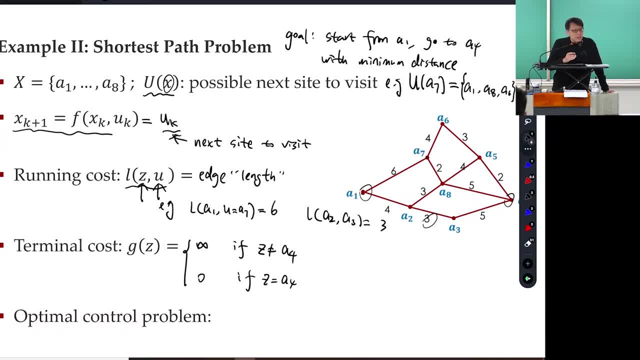 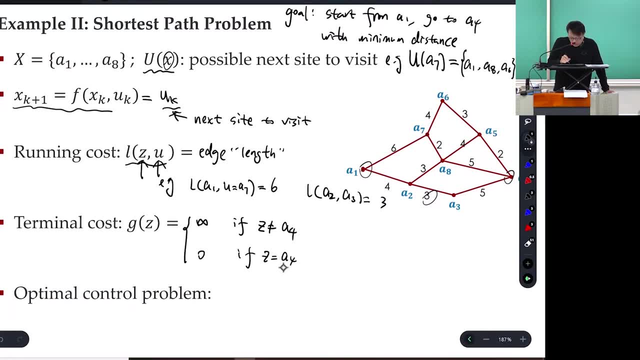 Z is a dummy variable. okay, It's a some function. Function is mapped input to output. Here I just use Z to denote a generic state. So if A4,, then it's zero. So if I'm here, then I don't penalize you. Okay. So then, because you know I've been doing this, there's zero. So all of these, you know, output and output. I'm doing nothing here And I'm still in the same, So I'll just use X to ignore it. 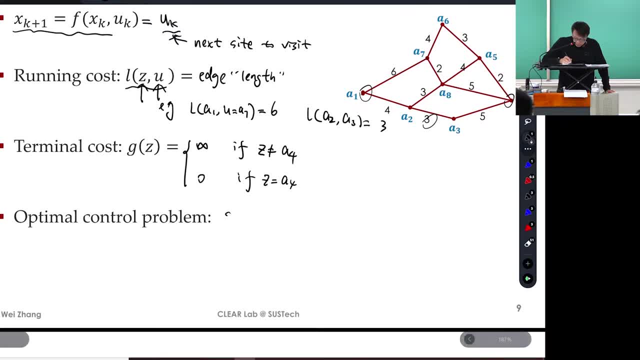 Okay. so then the problem becomes, let's say, sort is path, sort is path A1 to A4 problem Can be formulated as the following: Minimize I'll summation k from 0 to n minus 1,. 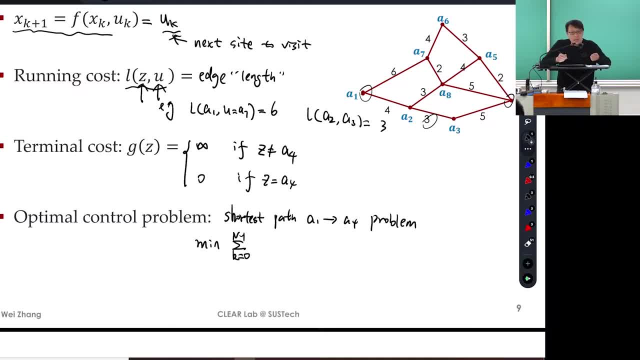 depending on how many times I want to give you right. If I gave you one step, of course you cannot go there. Your cost is always infinity, So. but so n is specified as time horizon. I allow you to solve this problem. 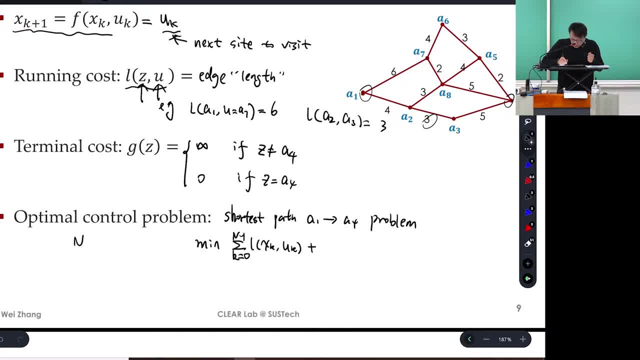 And this is xk uk plus g of xn, subject to xk plus 1, equal to. in this case it's fxk uk and uk belong to capital U of xk. That's it So, since the n is here. 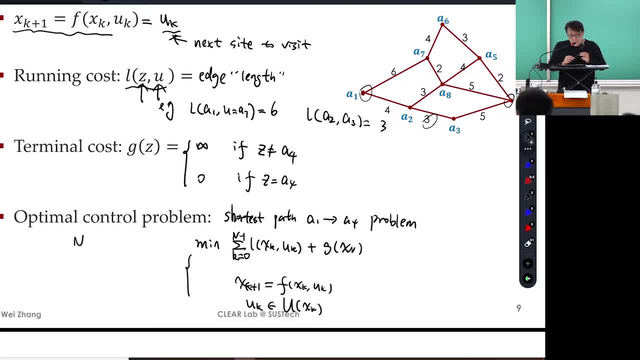 I think that the control action we can take, this should include the state in the same city. Yeah, no, Why? Because No n can be 4 or 5, or 7, yeah, It's given. So if n, maybe n equals to 4,. 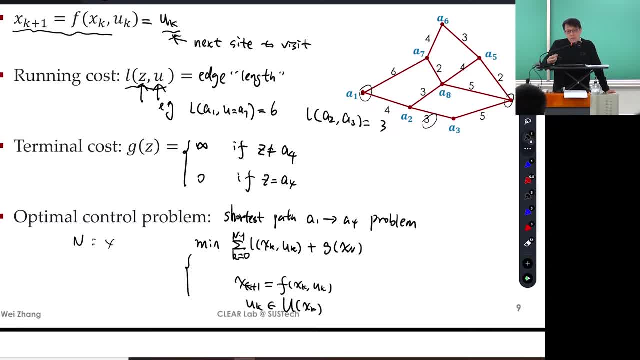 I have one of the shortest paths and then n equals to 5, I come: Yeah, sure, sure, yes. of course, If you're given more than, let's say, the minimum path, it's from, let's say, two steps: 1, 2, 3.. 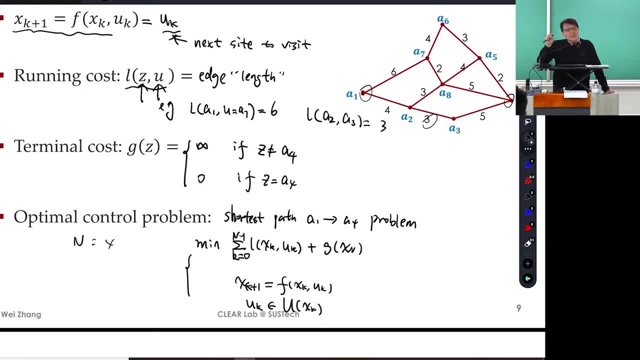 Suppose it's three steps, okay, And if I give you more than 4, then you will just stay. you will go there and stay there, Or you stay at the beginning to the end, right, It's fine, Constraint set okay. this is my general notation. 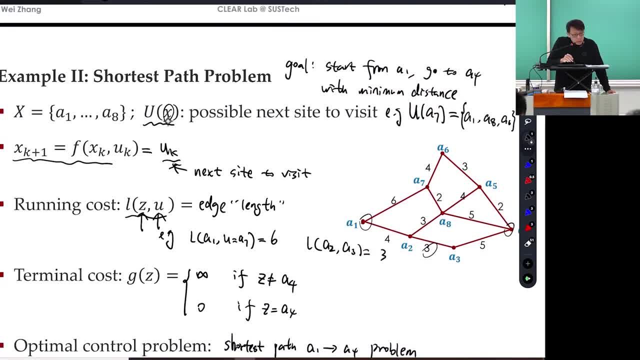 Constraint is just the at any given location, the place. It's just this example, right? Do you understand this example? If you are at A7, that's your current state- The control action you can take is three. If you can either go A1, or A8, or A6. 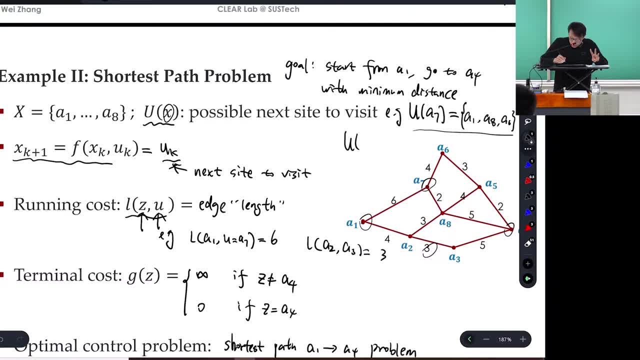 Okay, But if you are here, let's say, if you are A2,, let's say, if you're A6, then your control action you can take is A7, and A5.. Okay, It's different right At different location. 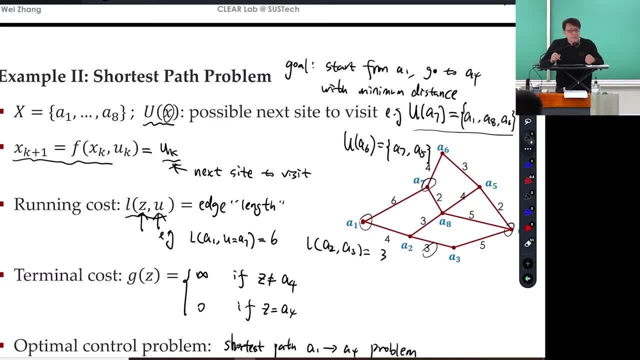 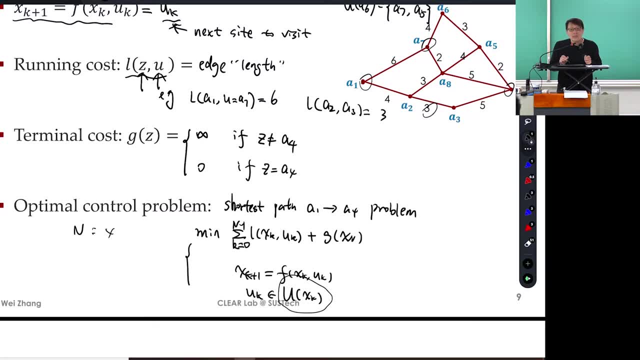 the next location you can visit are different. Okay, So the reason I'm writing this. you can see this is the same formulation almost from the previous one, Although previous one. I write down the more explicit formula. It's the same almost. 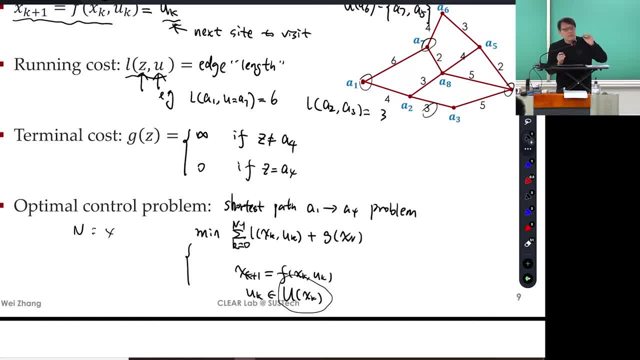 That means most of the problem, although from the beginning it looks like a completely different problem. But eventually I can all convert them to this general form. So now I can focus on this general form to study how to solve this kind of problem. 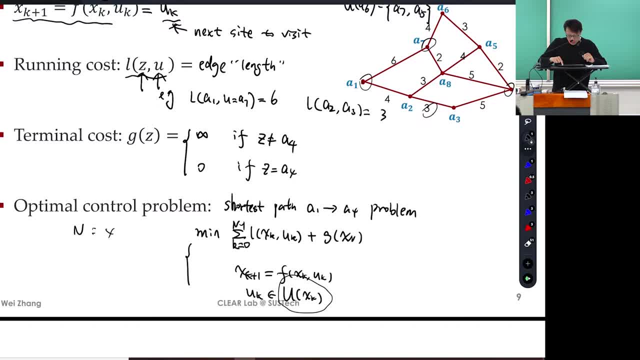 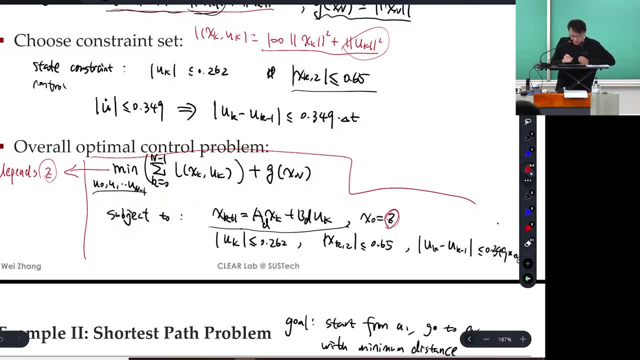 Then I can solve a wide range of problems. If you look at this equation, it's the same cost function. It just have different meaning. in this case, right, But exactly here all these things can be viewed as u- k belong to u of x- k. 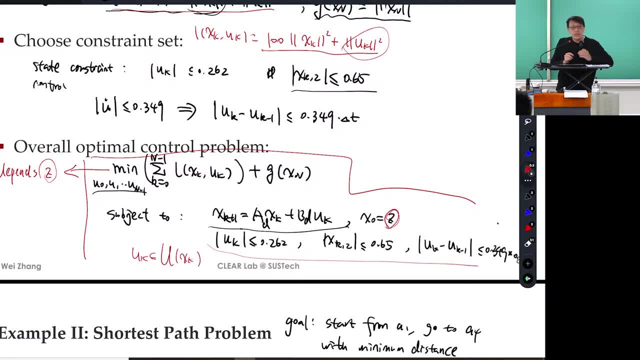 Okay, It's just. at any given time, your contraction available to you is different. You need to specify that constraint side. That's the case, right? It's the same kind of mathematical formula. Of course, the variable means different things. 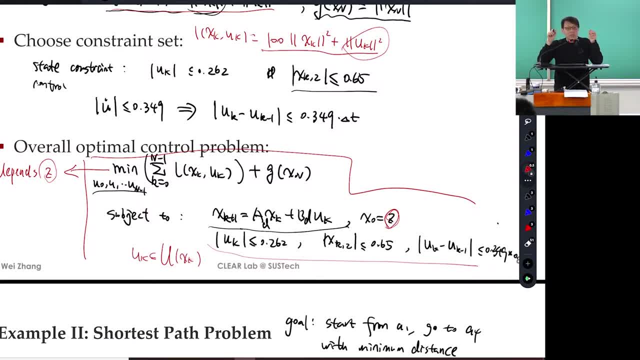 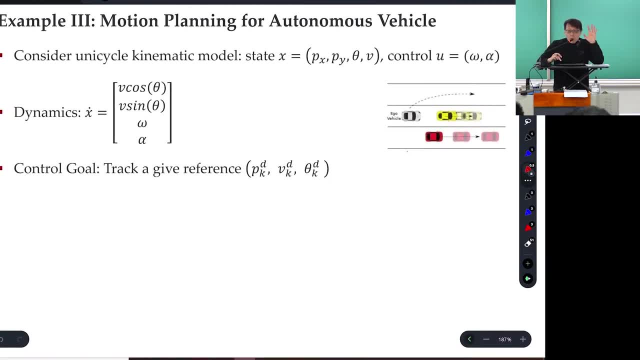 in different application right. So that's the generality of the optimal control formulation. I'll give you one more example. Then I think you need to have a concrete understanding of the optimal control formulation, So I'll give you one more example. 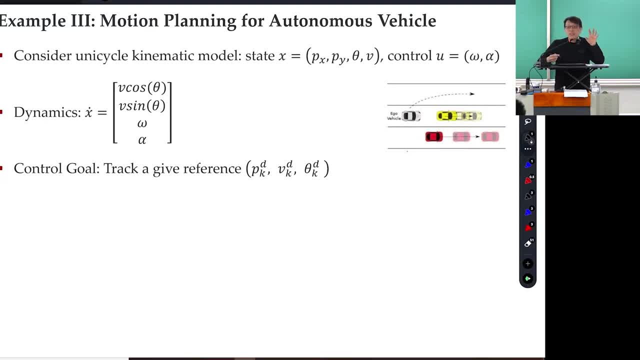 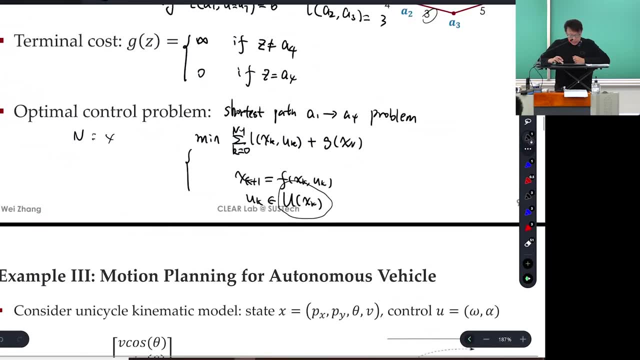 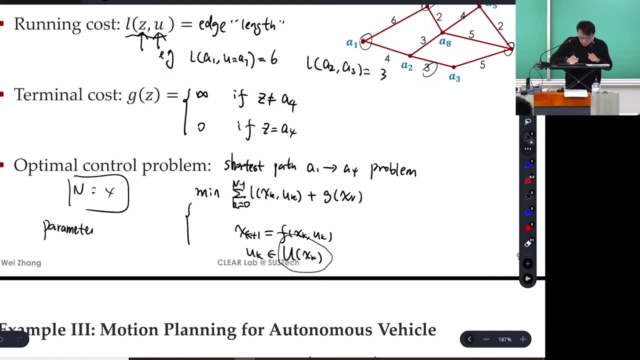 I think you need to have a concrete understanding of the optimal control formulation, Okay, Of what these symbols mean. Yes, So why do you determine the value of k? Say that again: How would you determine the value of k? These are parameters of your control problem. 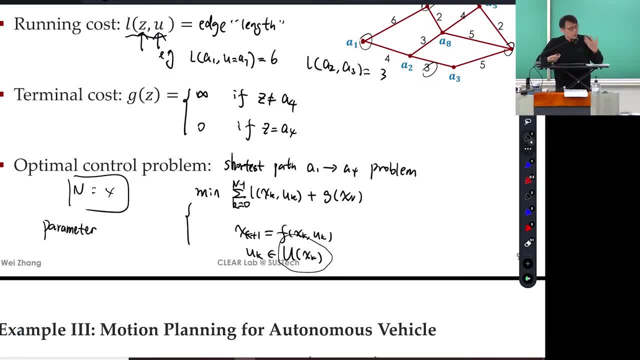 that you need to specify. There's no how. It's just formulate. It's depending on your problem, depending on your objective. In this case, I don't care how many steps, I just want to go there. So I can give any time, four or three. 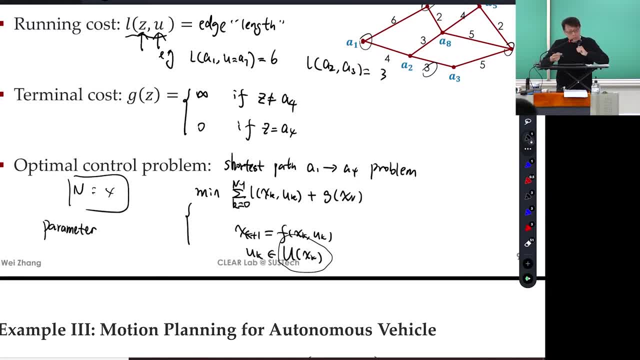 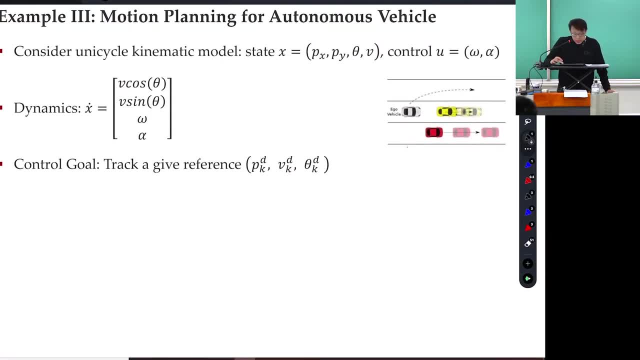 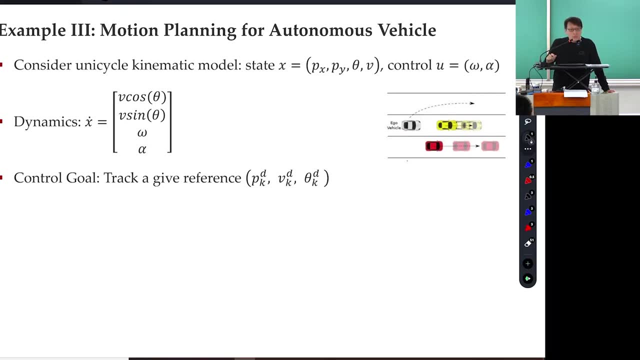 more than three is fine In this problem. Okay, So these are a parameter that you need to. you have freedom to define. The third problem is motion planning. a simple motion planning problem for autonomous or, let's say, a mobile robot. 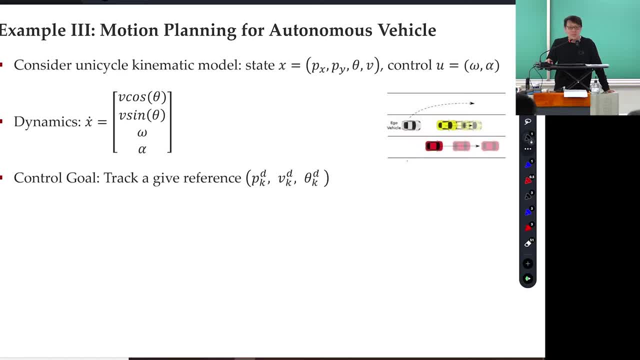 The fancy name is autonomous vehicle, but it's just a robot. had been studied 30 years. Okay, Let's consider any kind of a mobile robot or autonomous vehicle. It have a model. Let's use a simple kinematic or so-called unicycle kinematic model. 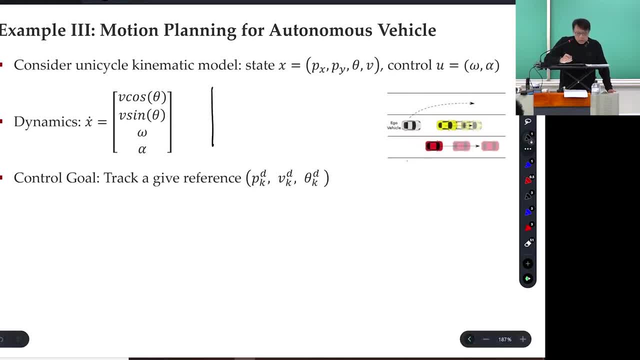 And the state has the following, And this is often used, by the way, for a mobile robot. I mean, you may find them useful not only for understanding this formulation, but also understanding your mobile robot problems. Suppose this is my location. 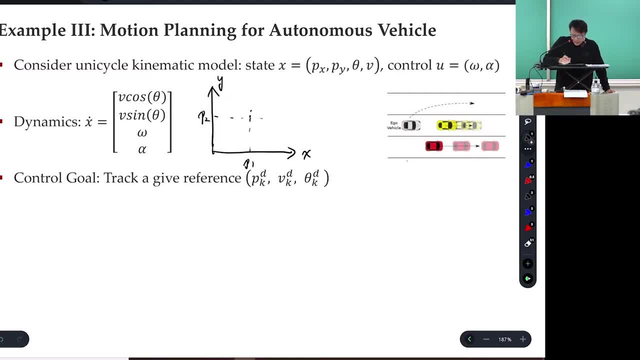 This is my P1.. This is my P2.. Okay, I have a car. that's a robot. Okay, The robot has. well, I can consider many things. I can model a robot as a bicycle model or as a point mass. 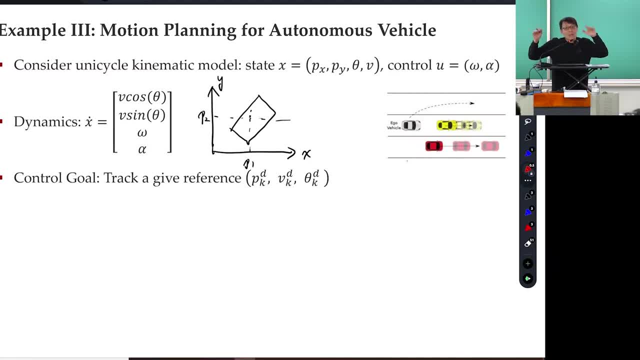 as a bicycle model, as a unicycle model, as a dynamic unicycle model that you consider forces, But in this case the kinematic. we don't consider forces, We only consider the kinematic information. That includes the location and not their velocity. 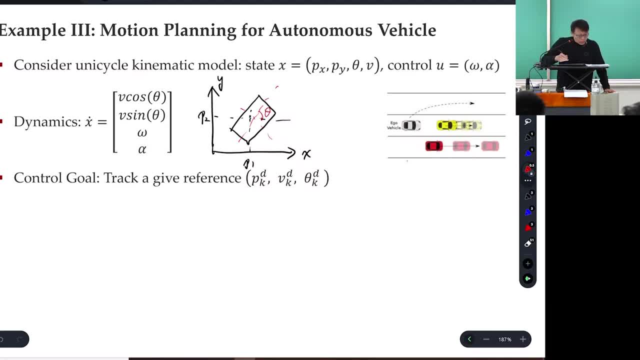 So here is, let's call it theta. This is the heading angle. It's a. this is the velocity. Okay, This is the heading angle. Okay, This is the heading angle That can be controlled, by the way, Right. 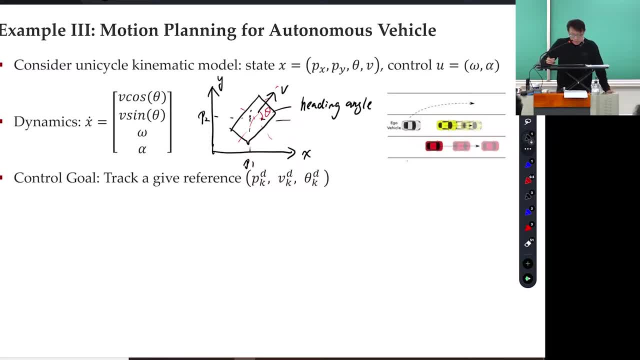 You can control in different ways. Let's abstract it. You can control it. So the state are four. You can planar, you can change X position, the Y position. Also you have theta and you have velocity And in this case, 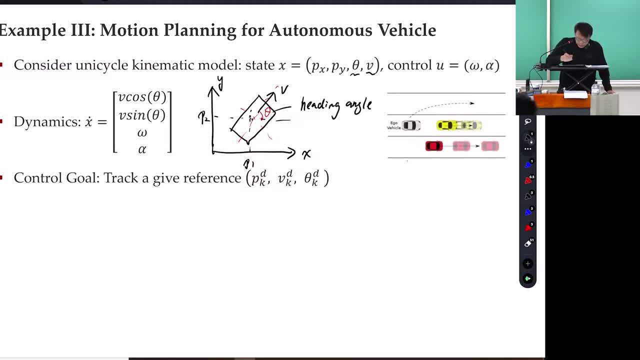 velocity can be changed as well. So I want to specify my notation here: X dot equal to V times cosine theta. So this is X dot. All right, You can. you can use simple psychometrics, You can find it out: V change equal to V times cosine theta. 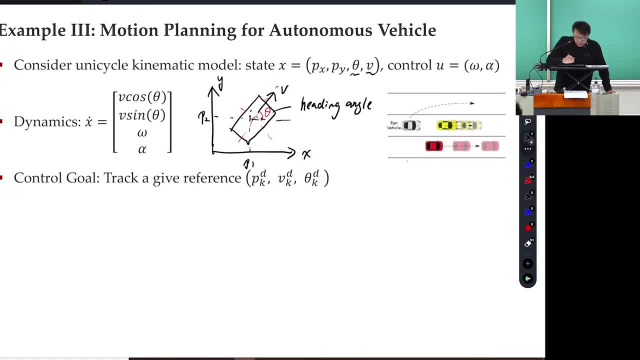 along the X direction, And this is sine theta. And of course, this is my what P X dot, This is my P Y dot, Right. The third one is theta dot. Okay, This is theta dot. Last one is how fast you change your heading angle. 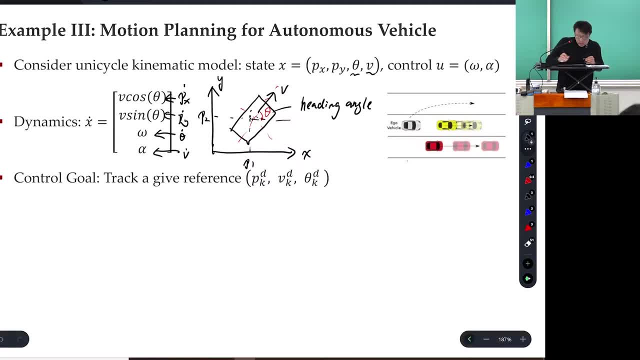 And this last one is the V dot, So how you can also accelerate Any questions. That's a model that describe your location. There's different ways to view this. This is one model that has been used quite a bit. Let's use the simplest model. 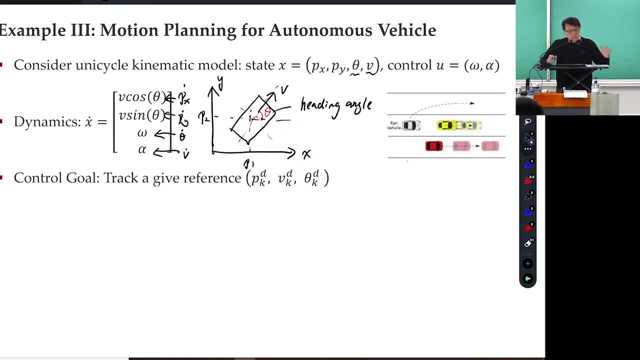 Okay, Unicycle model. You can consider steering angle. that would be also slip angle. There's a lot of different things that you can consider. The more details you have, the more accurate. suppose the model is cracked, then the more accurate. 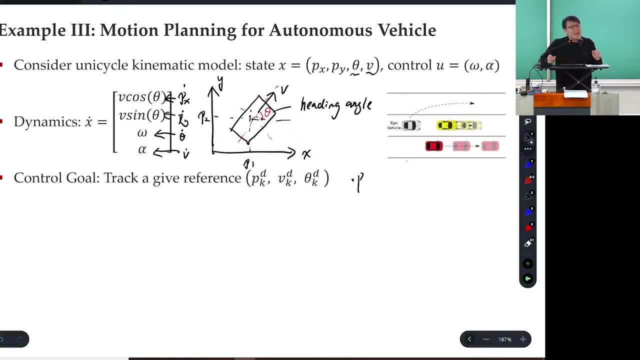 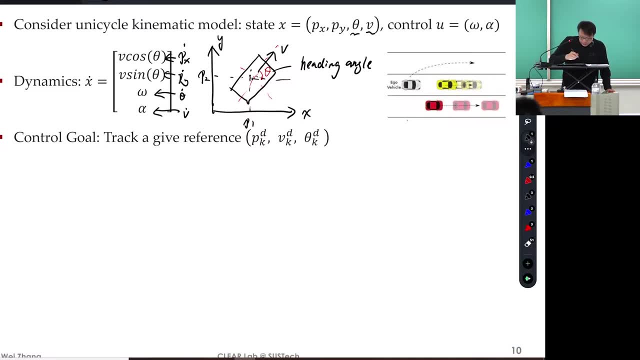 But here is it's roughly. I can also consider point math, That's fine, But here is the unicycle model. Okay, My question is the following: Our goal is, given a reference, PD, VD, QD, theta D. 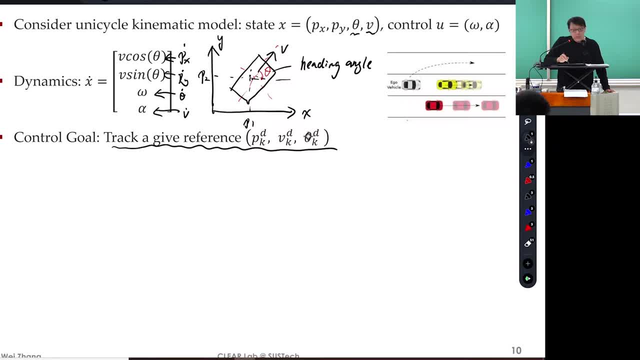 What are they? So the position reference and the velocity reference and also maybe heading angle reference. Okay, Suppose I gave that That's specified typically. Let me give a comment. Those are those are typically given by planning problem. This problem is tracking control. 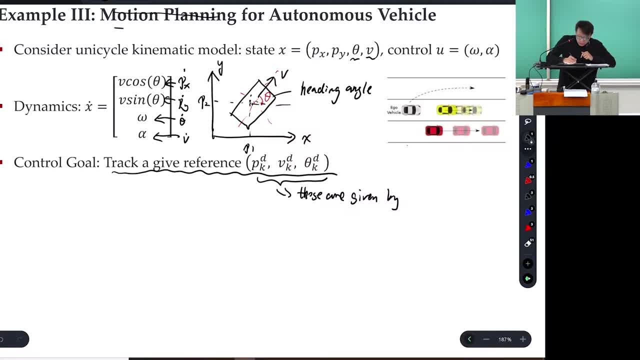 Okay, I shouldn't call it motion planning. This should be called tracking control. Okay, So given by planning algorithm, For example, if suppose your vision tells you these are the the lane and you want to stay in the center line of the lane? 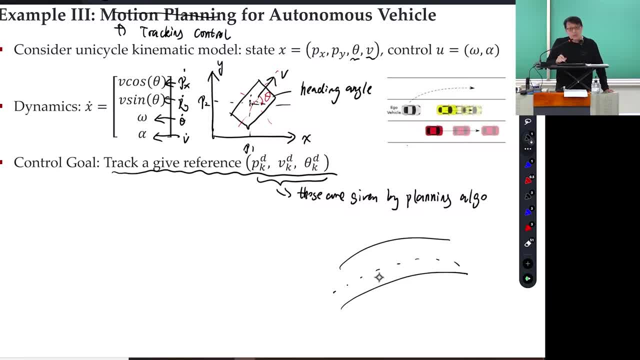 typically, And those are typically specified as the polynomials. Okay, You want to specify your desired polynomial Roughly And you want to track that. You want to stay in the center. That's your objective, So you can. you can find those. 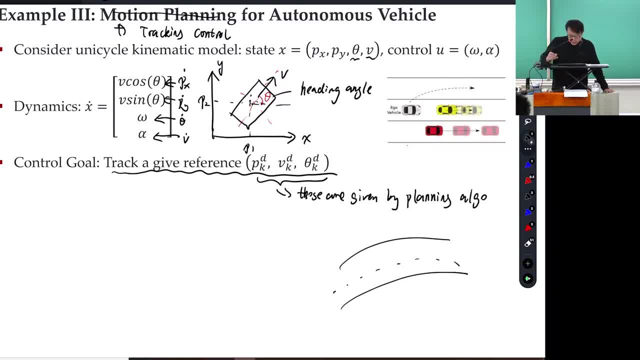 position and its velocity and heading angle changes. Okay, Let's assume they are given now And our problem is track. Problem is to track, Yes, track of given reference. So the first of all is this is continuous dynamics. I'm not sure whether you can see it. 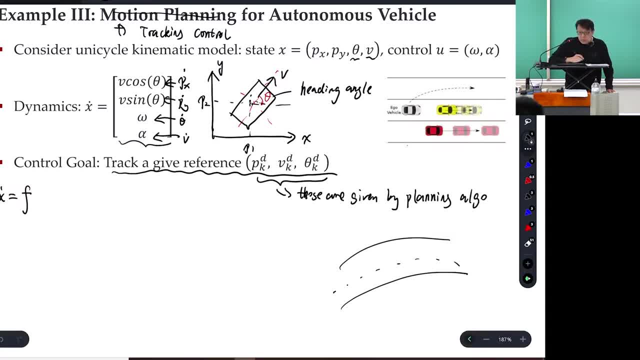 This is. this is my vector field. Okay, Let's view what. what are the controls here? The rate of the heading angle change, the heading angle change rate and also the acceleration. Okay, The velocity change rate is something I can control. 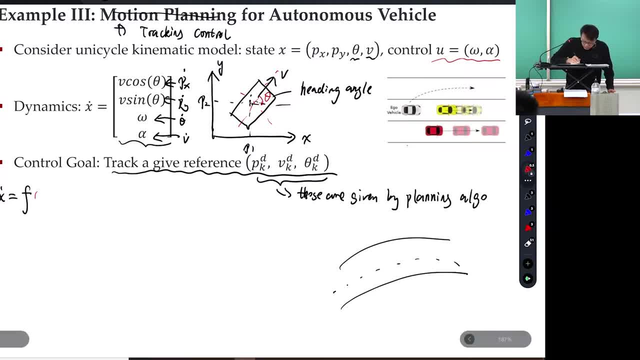 in this case, And so that will be my x and u. Assume you know this is my u1,, this is my u2.. Right, This is two u's. That means that's specified. Those are not state, Those are controls. 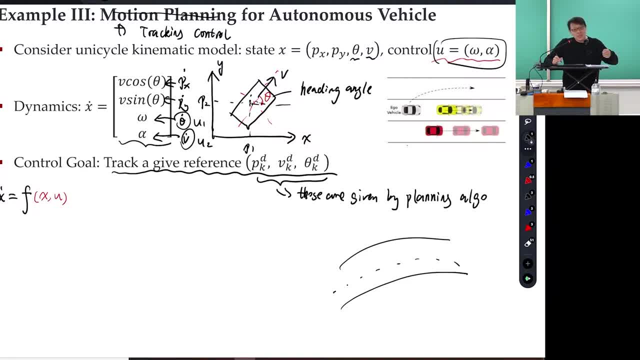 Okay, Your control directly control the velocity of certain state. So then that will be my. well, we want a discretized model that will be xk plus, one equal to xk plus. if you use Euler discretization, that will be xk. 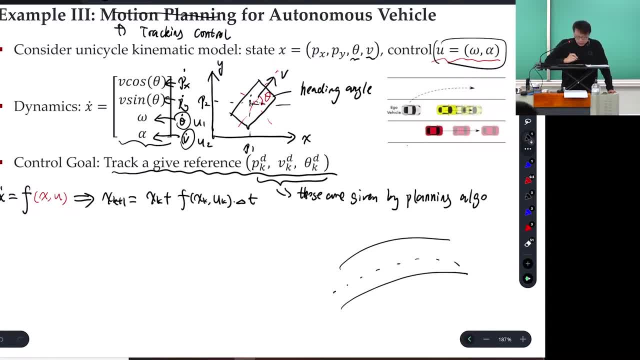 uk times: delta, t, Right, And this whole thing is my f? xk uk. This is called d the discrete time, Are you with me? You have a continuous vector field. you can discretize with sampling time. Then you have a discrete time thing. 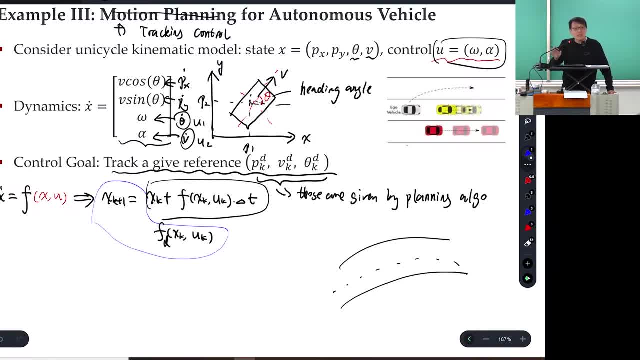 Mathematically. mathematically, this model has the same representation as a previous shortest path problem on discrete graph. You see, it's all the same thing. That's why the framework is powerful. It depends on how you view the meaning of different state. 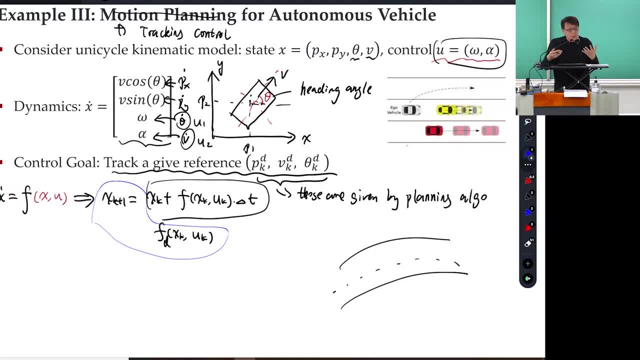 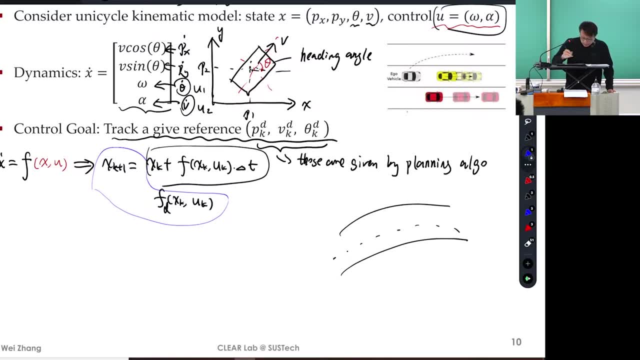 and the control. They will represent different problems, But mathematically they have the same representation. Okay, That's the beauty. We want to track this problem. how to formulate? There's a thousand ways you can formulate that. For example: 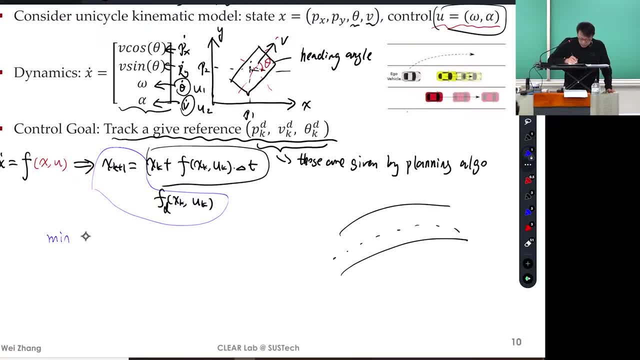 I will throw out one formulation, For example. you can say: I want to minimize running cost. Suppose my running cost is zero and minus one. Suppose my running cost will be pk minus pkd. You want to follow your desire, Right? You want to minimize that? 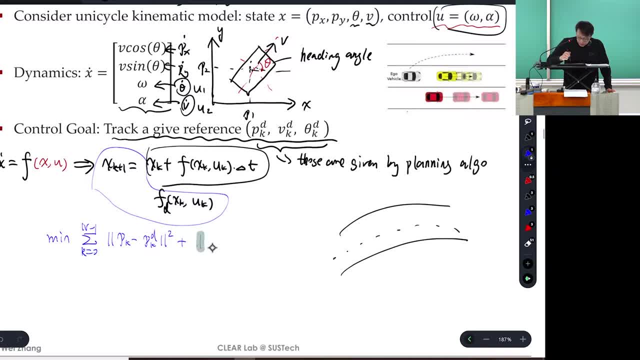 Plus, let's use a maybe. I think control is not that important. I will say times alpha k. Alpha k is my control Right. So it's alpha k is my u k of one. Alpha is two Right. Alpha is two. 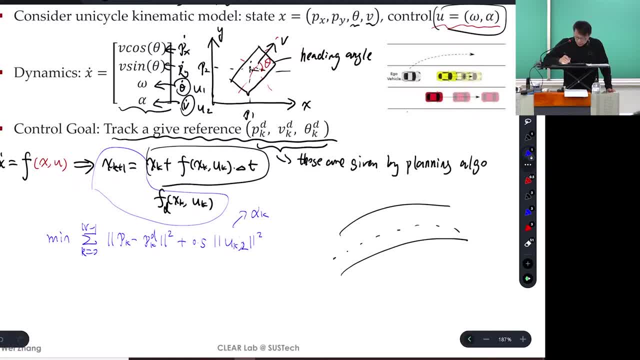 u k of two. That means alpha k Right And plus. suppose I also want the change rate to be not too big. Let's say this is a two times u k of one, u k of one sub index, one squared. This means I don't want. 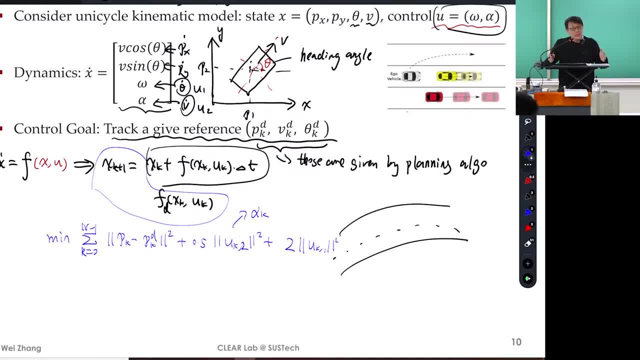 the change rate of the turning to be big. Right Acceleration can be a little big because I penalize the changing rate of the, the heading angle to be larger than others. Okay, The cost function And also I want to penalize. 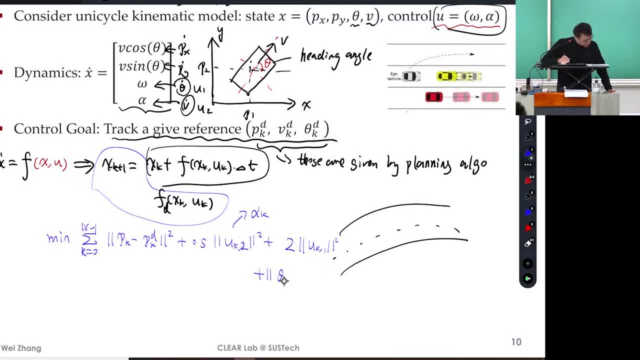 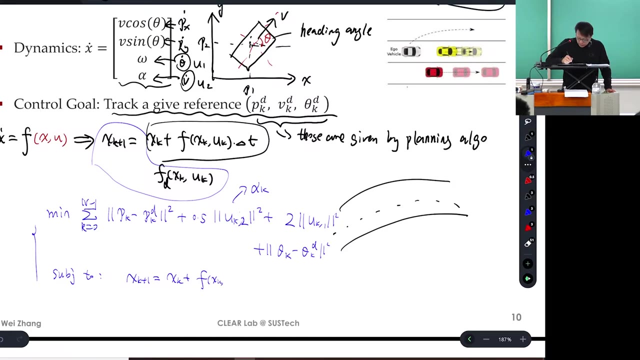 deviation from my theta k. Theta k minus theta k d squared Well, there could be also terminal cost as well, But subject to subject to. let's say i x k plus one equal to i x k plus i f x k, u k. 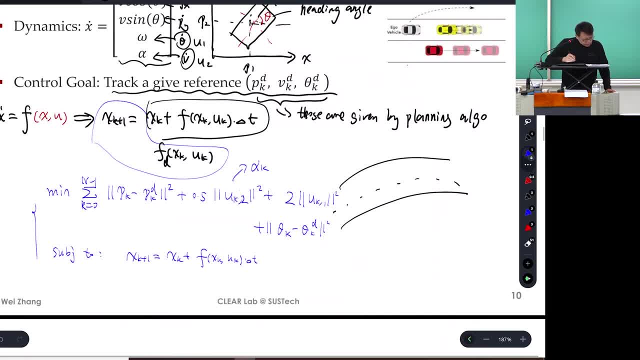 delta t, which is my discrete time update equation, And also u k belong to u. You need to specify what contraction you can take, For example. for example, you need to respect turning radius limit There's. I mean, I don't want. 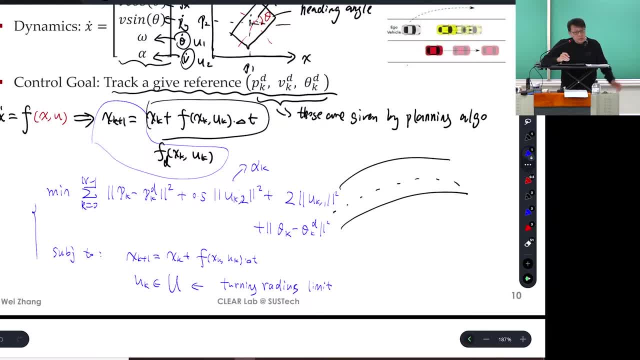 to write down everything completely. in this case You know roughly. you need to consider a lot of things: how fast you can change, For example, the acceleration cannot be too big, Things like that. And also you also want to specify what contraction. 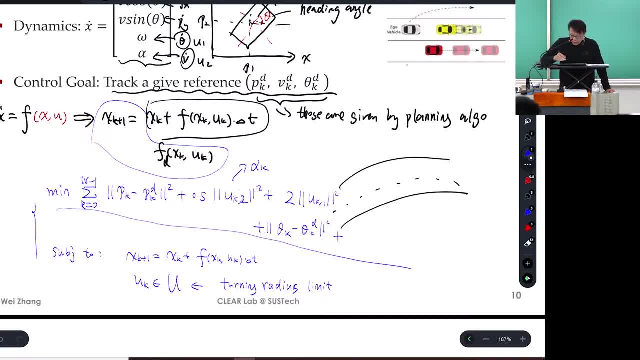 you can take to maybe be safe. For example, I can put that in the cost I want to, plus 100 times my distance to obstacle. Okay, Suppose that's my current position. t k, You see what I mean. This is a function. 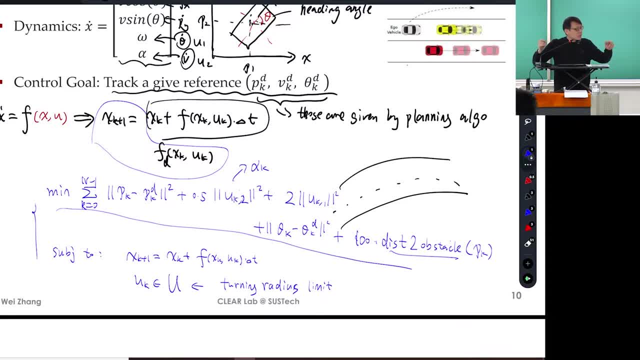 that how far you're away from the wall or some obstacle And you can calculate based on how close you are to that obstacle. you can calculate number: The larger the number is, the safer you are. But you have too many obstacles. You need to. 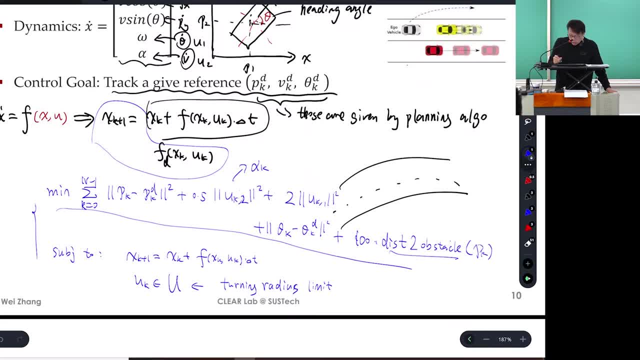 penalize them. Okay, that depends on the current state as well. So all these things- I will circle these out, Okay? So all of them are in my formulation here. all of them are running cost. You see what I mean. 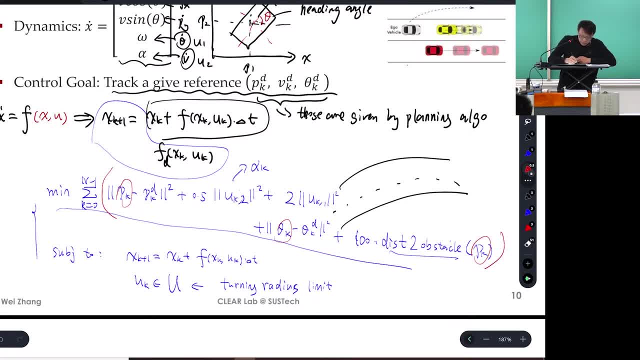 All of these whole thing is a running cost. That means it depends on x, k and the u k only At any given time. the terminal cost depends on the final state. I can keep adding things. That depends on your boss. He may. 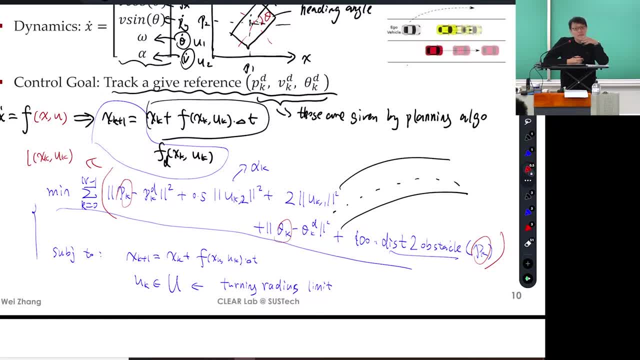 care more about comfort, care more about other things. You need to put that into your cost functions. There's some tuning into this whole problem. I hope that's enough formulations And I can just assure you that all the problems you care or you 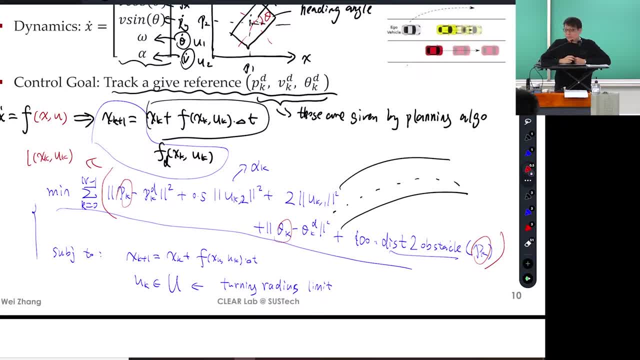 want to solve can be formulated as an optimal control problem. Let me repeat All the control problems you're trying to solve. well, maybe each of you will give you a homework. You can try to challenge me by writing down a problem that you. 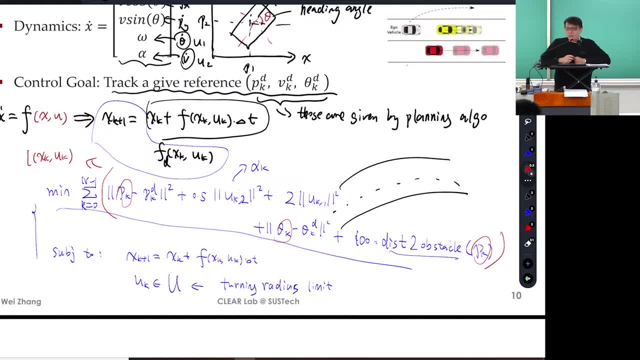 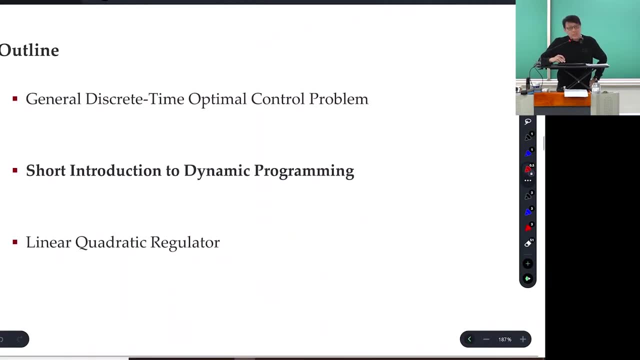 think you want to solve, but they cannot be formulated as an optimal control problem. Send it to me and I can tell you the answer. Okay, that's the formulation. That's already a big deal. Okay, you can formulate these linear packages. 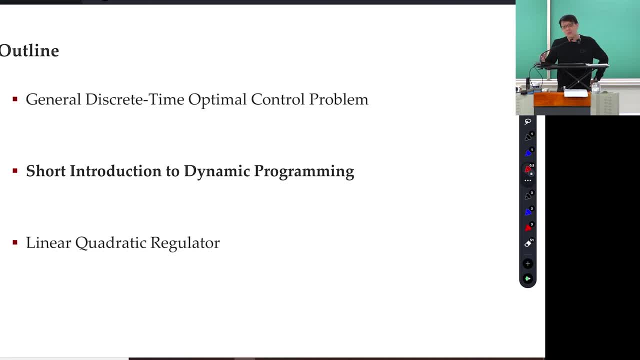 that can help you solve optimal control problems. You know I don't like you to just introduce dynamic programming. How many of you know dynamic programming? I think everyone right. No, You know that Xiao Han 知道, 知道. 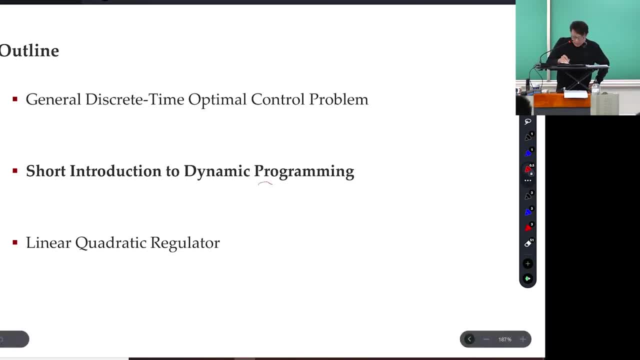 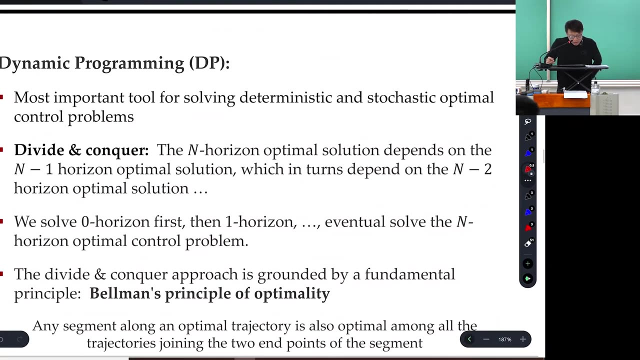 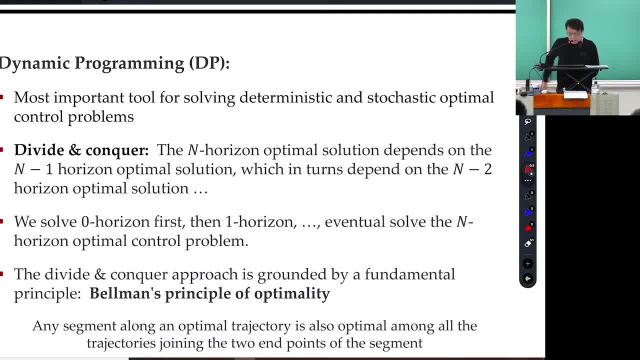 是 我, 我 是, 我是, 我是 了. 这是 你, 是 你, á 是 Ö, 是, 就是, 是, 是, 是, 했는데, 是, 是 真的, 是 reinforcement learning or Q learning or DQN. 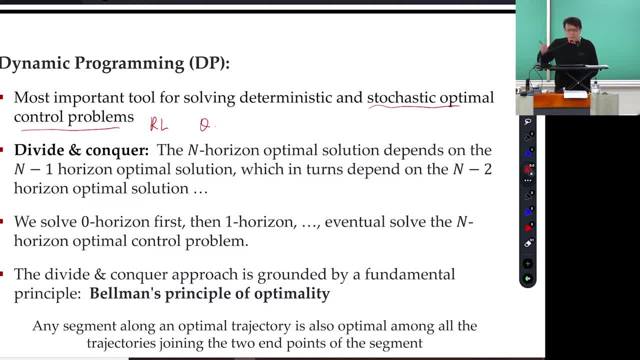 AlphaGo they are solving. what Optimal control problem. You can find their running cost. You can find their terminal cost, Exactly So. AlphaGo is similar to our road network problem. I mean based on abstraction, but of course it's hard to solve. 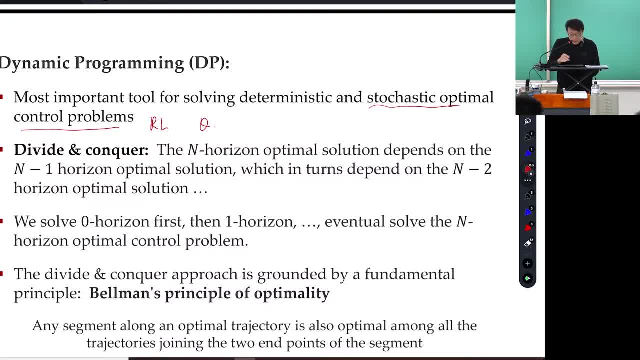 So divide and conquer. So the key idea- I think it's this L-Horizontal Optimal Control Problem- can depend on minus one optimal control solution, which in turn depends on minus two. So let's keep it like that. 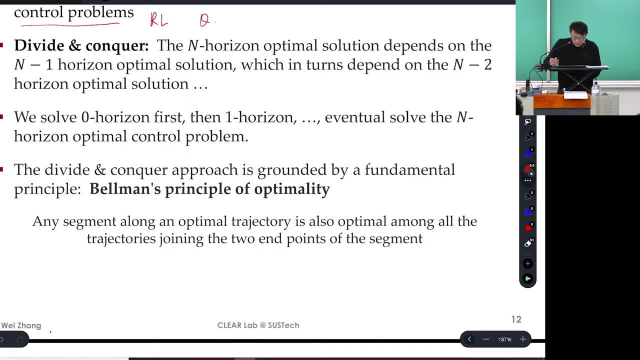 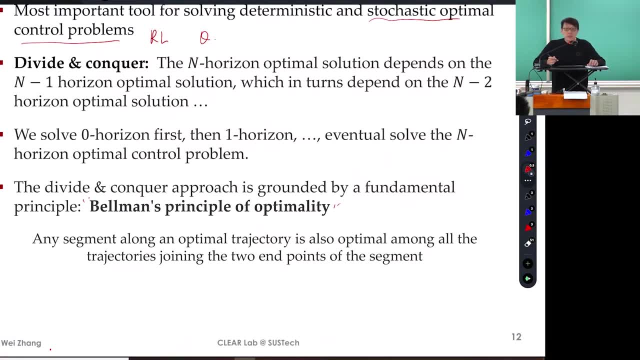 Backward induction. we'll see how this works. I do want to emphasize this is all the thing. the dynamic programming, they're different views. Okay, You may learn it from, I think, most of CS theory class with teeth of dynamic programming. 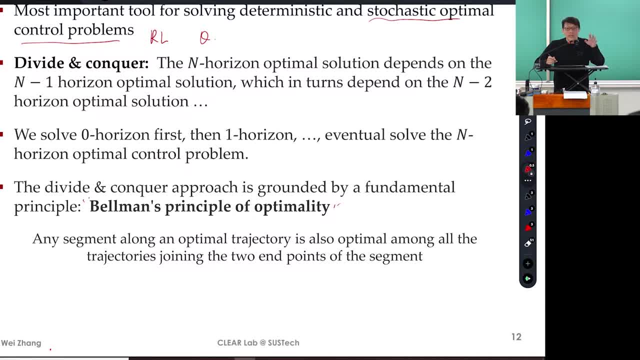 How many of you have learned dynamic programming from other class- Algorithm design, Algorithm design, Really, We have this class. Yes In CS, Yes In CS. okay, So typically CS would cover this, but it will cover it differently typically. 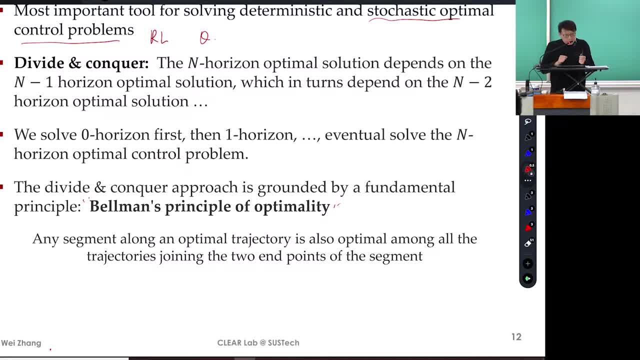 They care more about implementations. Okay, They will learn things that are in different flavor, but in nature, mathematical nature, they are the same. Okay, I want to mention that. well, it's all. so the DP, dynamic programming. 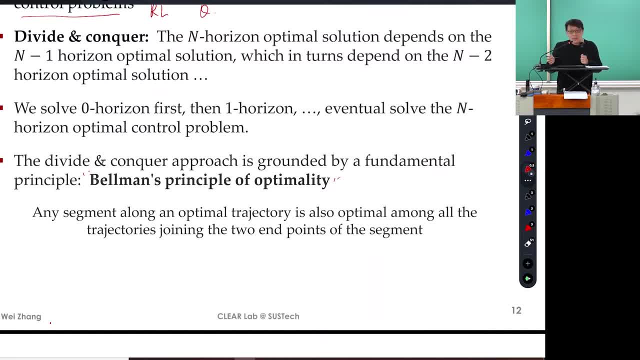 is based on Bauman's principle of optimality. So this means: how do you know something is optimal or not? So typically, when we do least square, we take derivative, make it equal to zero. That quantifies or specifies something is optimal. 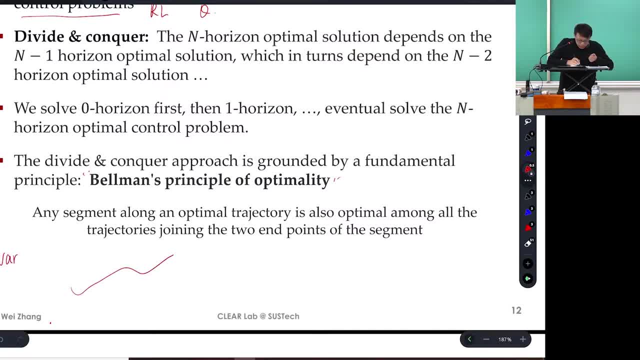 Right, But that is called variational. variational, And that means that you must beat the optimality condition Options you condition. What do I mean by that? So, if this is your trajectory, if you perturb a little bit, 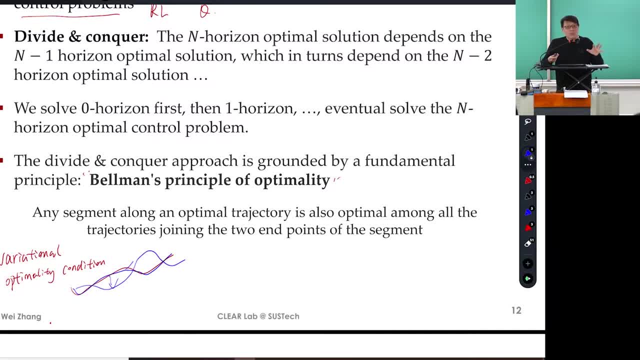 if you bring this, it won't be optimal. Okay, That means infinitesimal perturbation will be zero. It cannot improve the cost. That means your typically the gradient equal to zero, things like that optimality. But in Bauman's principle it's a completely different way to specify. 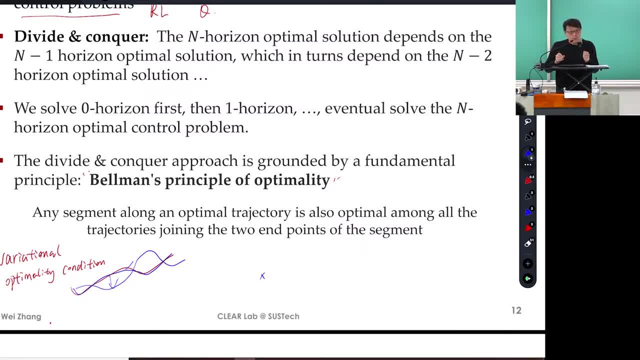 optimality. It's a different way to think. something is optimal or not. You need to remember. So, for example, what does this mean? Any segment among optimal trajectories is also optimal among all trajectories joining the two end points of the segment. I'm not sure whether That's my summary, by the way, If you don't, 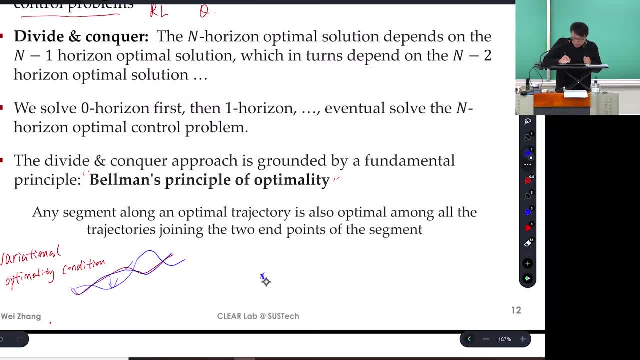 understand, I can explain. So suppose, from here to here. this is my optimal, This is my optimal path. okay, Then I ask you a different problem. I ask you: what is the optimal path from here to here? It will be exactly the same path, You see. 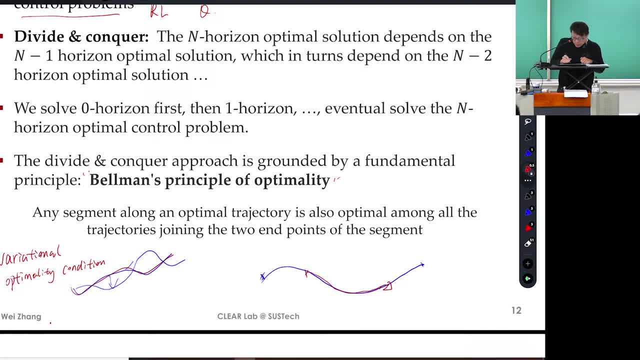 what I mean. Let me repeat: Suppose this blue line is optimal from A to B And I ask you, And this C and the D are on the optimal path. I'm asking you: what's the optimal path? from C to D? Of course you should follow this path. What else, So what? 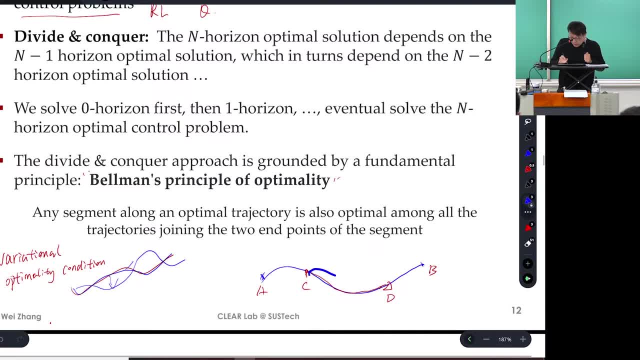 happens. if not, If there's other, better paths, let's say this is a better one, then my optimal path will be the same. My optimal path would also take this right. That's roughly the same. That's roughly the meaning of Bellman's principle of optimality. Any portion of the optimal path has to be. 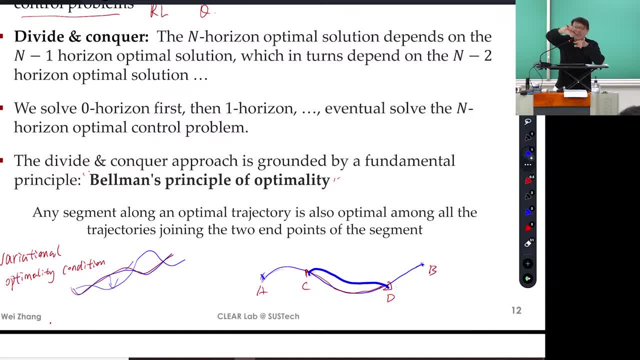 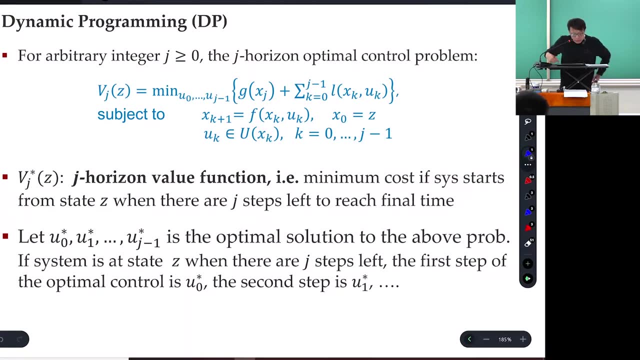 optimal. Otherwise, you will replace that portion with other things, with a better one. I don't think you need to fully understand what it is, Just keep that in mind. That will be okay. All right, So let's jump into dynamic programming. So, in order to solve. our goal is to solve. 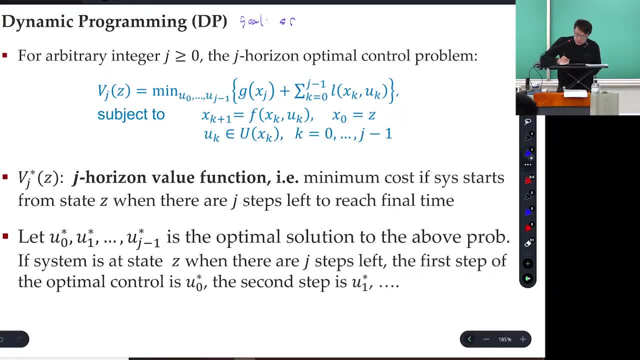 So goal: solve n-horizontal optimal control problem. okay, OC optimal control problem. And we start by defining a sequence of optimal control problems with varying horizon. One is, It means J can be zero or zero horizon one, horizon two, horizon three, horizon up to. 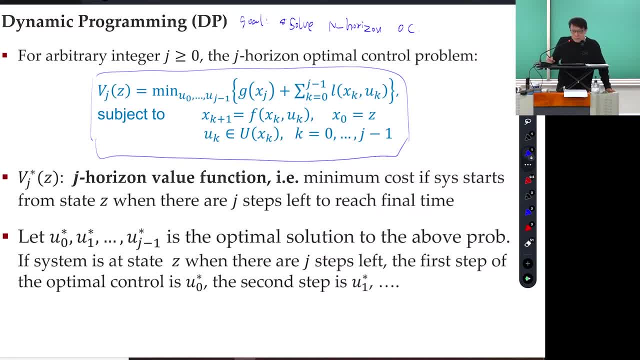 n horizon. Is that okay? I just replace n with J, right, But my goal is to solve n problems, n-horizontal problems. But I start from the zero-horizontal problem, because the smaller the horizon size is, the simpler the problem is right. So that's roughly the case. So 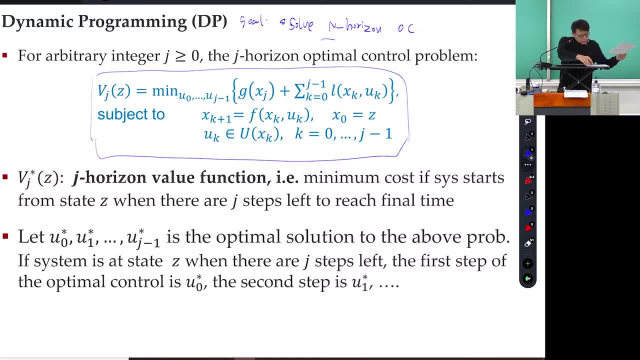 there's a few kind of- I will call it- terminologies I have to ask you to know And you have to know it. I think that's very important. One is called value function or cost to go. Have you heard about this? It's called a value function. So what does this mean? It's. 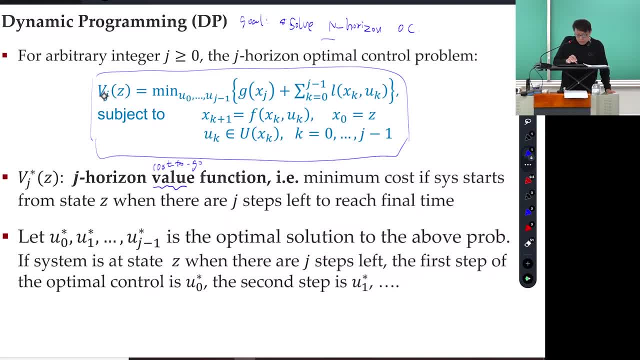 What does this mean? VJ of z means Means the optimal cost, The optimal cost for the all n-horizontal optimal control problem. So if you have, Let's say if you have, I just want to say: minimize x squared plus one over x, suppose. 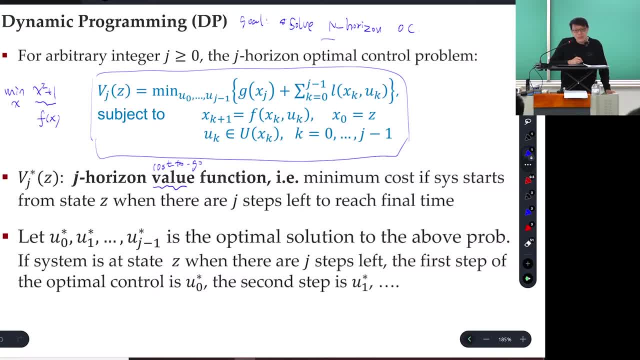 right, And this is my f Right, And so the minimum value would be 1.. No matter what x is, it will be 1.. So minimum value- this is the value function- will be 1.. Okay, The optimal. 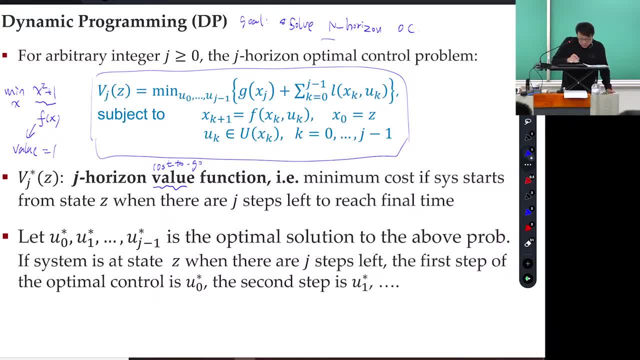 cost it can achieve is 1.. So this means the optimal cost. You solve this optimal control problem. you will have a cost. The cost could be number 1 or 2 or 3, and that number is called the value of the problem. Why it's called the value function? Because the problem changes. 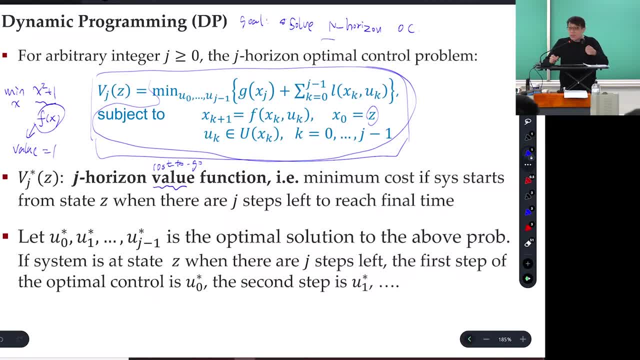 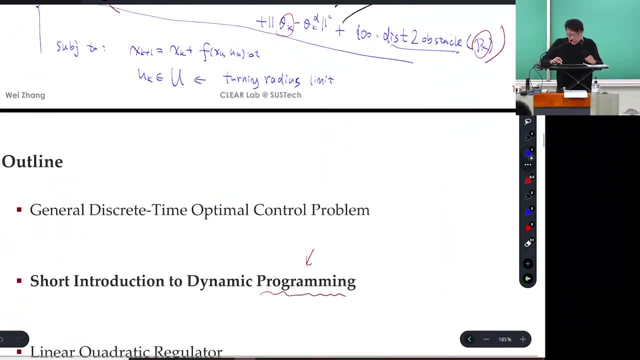 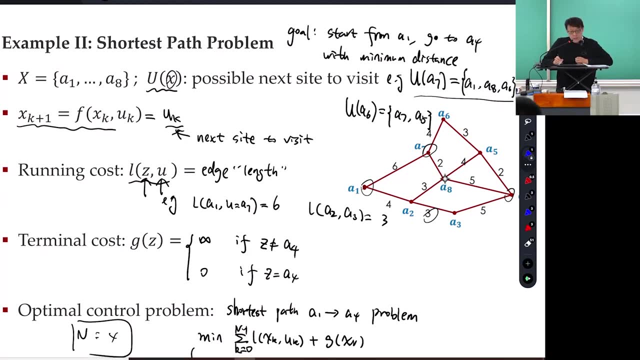 When the initial state changes. As I mentioned, this problem depends on the initial state. Okay, The optimal cost. I can just Let me finish by this: The optimal cost, if I start, initial state is a2,, a8, or a3, or a1,, the optimal cost will be different. The optimal. 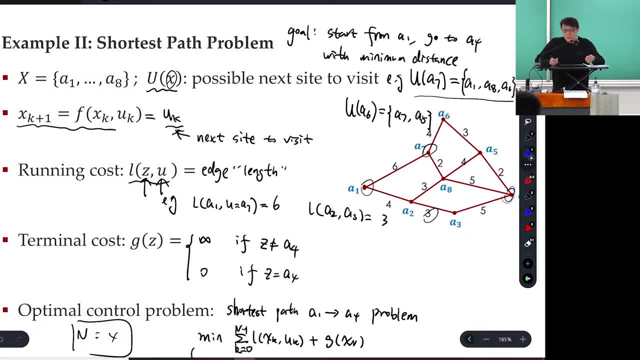 cost will be completely different. If I start from here, the optimal cost will be zero. If I start from a1, the optimal cost will be something. 8 will be something. Overall, the optimal cost has a. It's become a function of where I start, So that function is called. 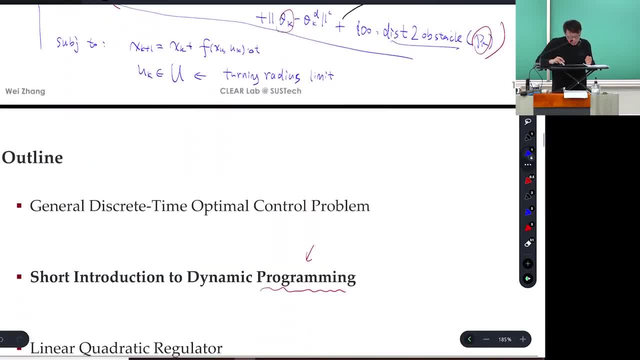 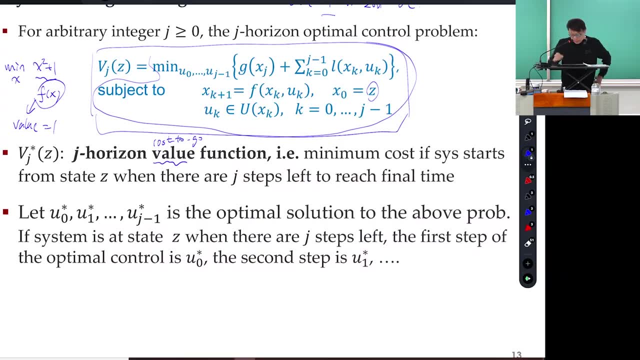 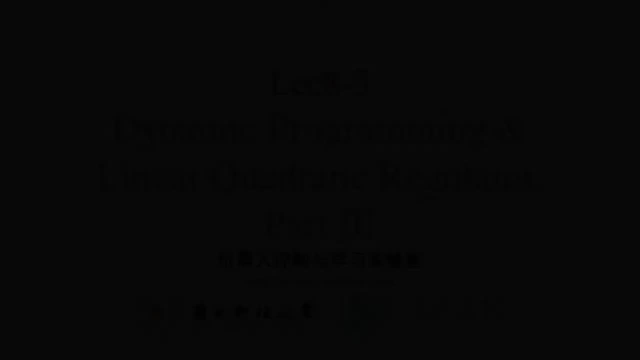 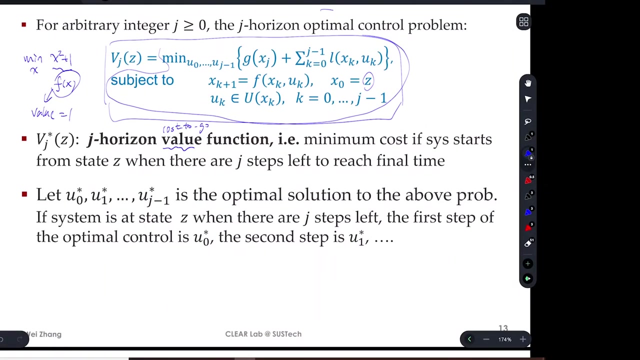 optimal value function. It's called a value function In this lecture we will call it v star. All right, Let's take a break. Okay, Let's continue Again. I want to emphasize: the value function here is the optimal cost. 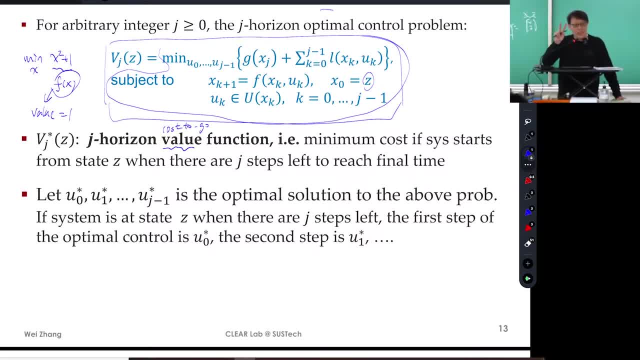 of the problem. And the problem depends on two things. One is where you'll start, What's the initial state before and also how many time horizon you were you gave to this problem, which is J. so this meaning, the true meaning, or or a complete statement of this meaning. 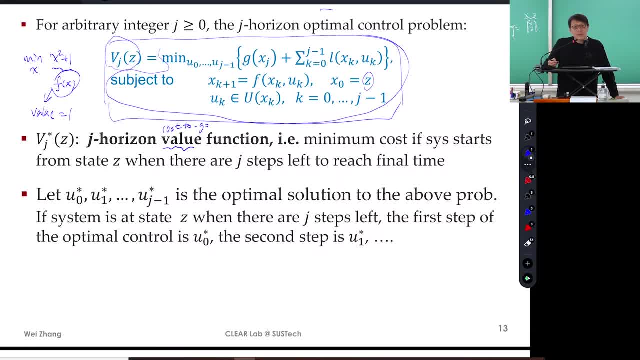 is the optimal cost. if there are J steps left and then you stay at the Z. you know this is J and this is Z. okay, if you're currently at Z and you have J step to go, then this is the optimal cost to finish the rest of the horizon. okay. 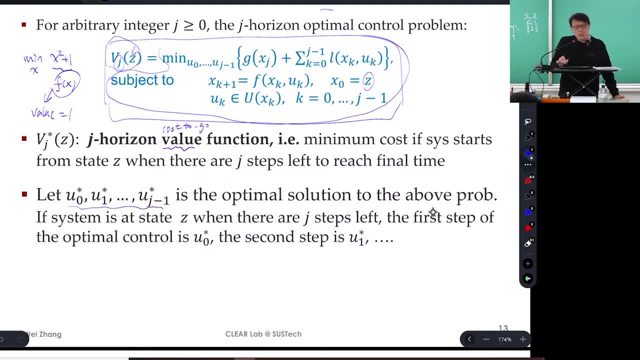 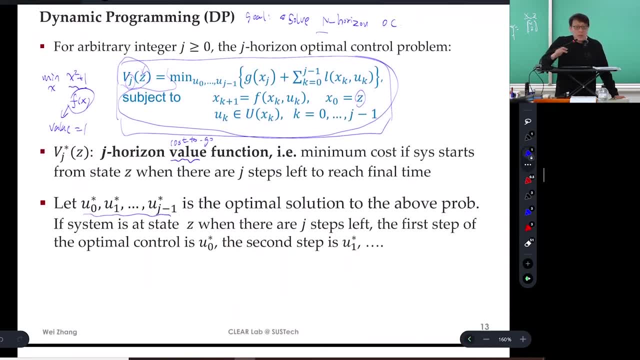 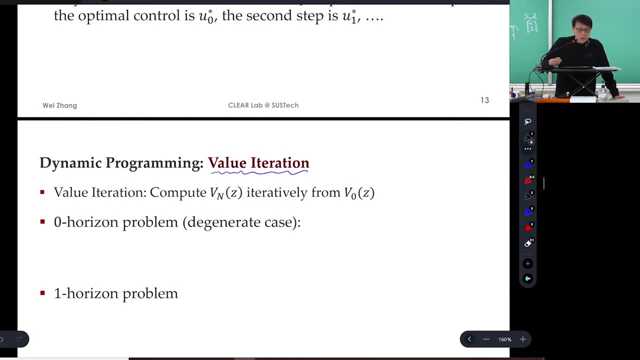 and these are the solution, optimal solution to the above problem, and let's. there are different ways to do dynamic programming. one way is called value iteration. I think this is the only way we are going to learn and it's the most popular way that you are going to code as well. 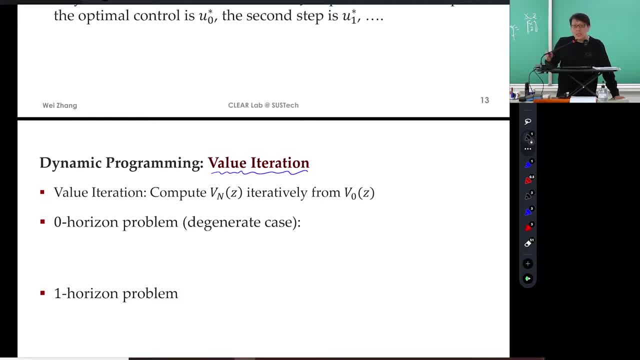 what is value? iteration is just you completely compute the value function for all, zero horizon to one horizon up to an horizon. okay, let's start from the. it's like a recursive. you have a starting point. the starting point is an equal, or the horizon size equal to what J, equal to zero. so what do you think is? 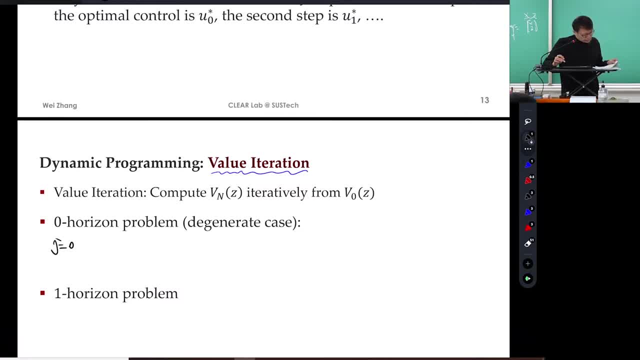 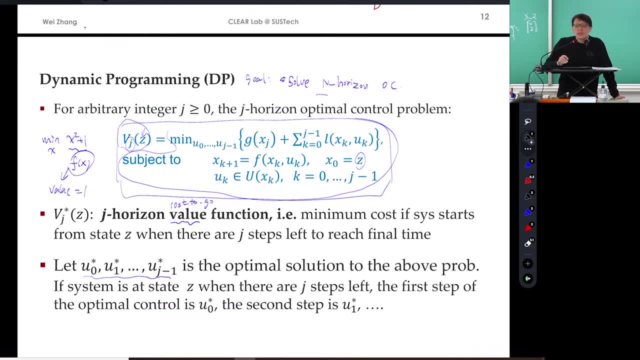 a J horizon problem is. let's look at this problem. I'm not sure whether you can, you can understand. when J equal to zero, what are the optimization variables? these are the generic terms. okay, the generic terms. when J equal to zero, you have a user up to you minus one. do you have anything? you don't, because 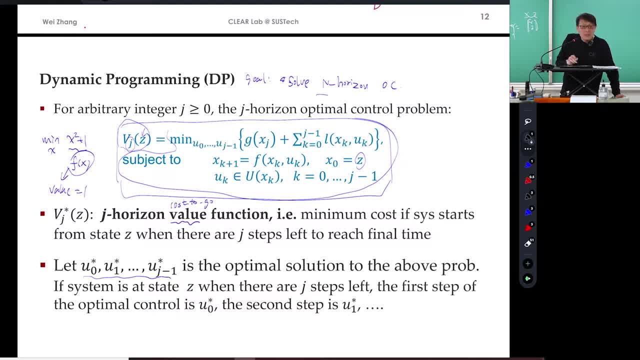 you don't have any index. satisfy the indexing rule, which is from 0 to day minus 1. so there's a no controls, right? what about this submission? there's nothing, right? you have only have one horizon. there's no running cost. the starting time is the end time. okay, see, but you have G of X. J equal to 1 is X- 0. 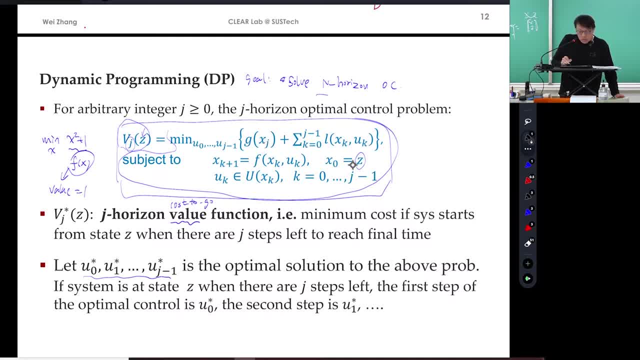 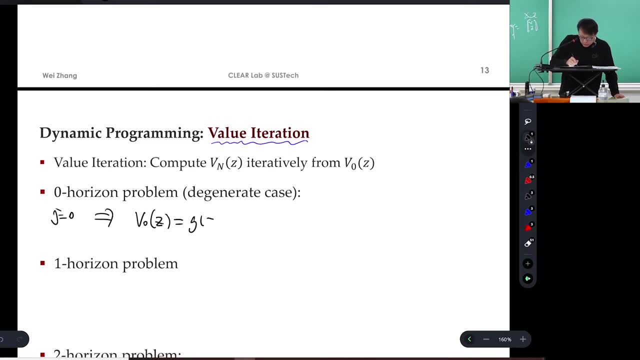 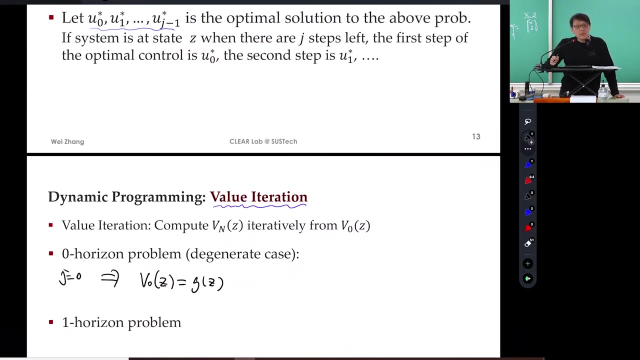 right. So x zero is z. You don't have any. all the other constraints are satisfied. they don't appear anywhere. So when j equal to zero, we can say v. zero of z, equal to g of z. That make sense, The optimal cost to go. if only zero steps. 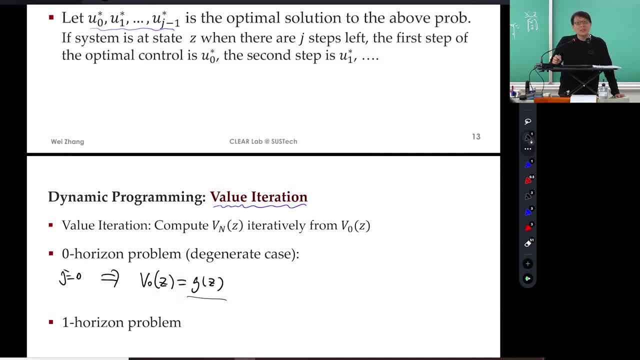 is the terminal cost, Because at the beginning you're already at the terminal time, right? So that's roughly the meaning. okay, So v zero of z equal to g of z, So we don't need to compute, we can directly write it down. 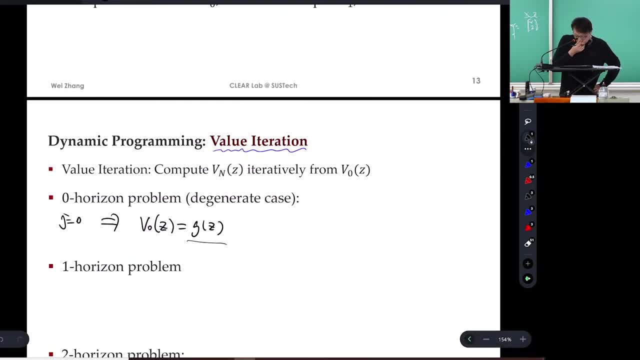 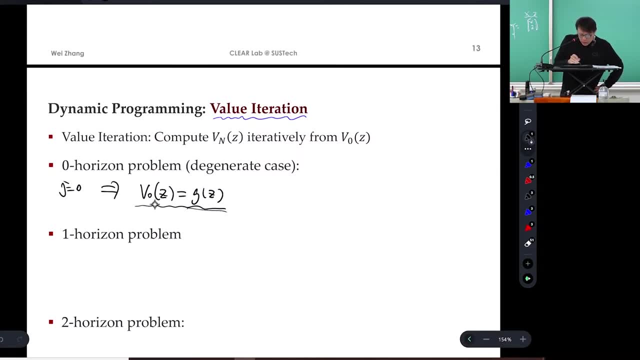 if we are already determined the terminal cost. Okay, let me jump a few steps. Let's just say it's recursive, right? So now we know how to start. When there are only zero horizon, then we have terminal cost. is the value function? 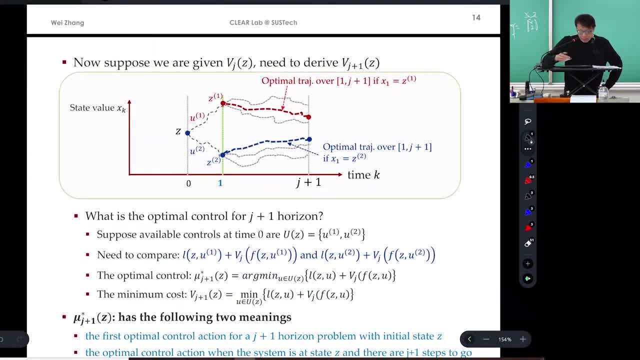 What about suppose? now let's directly jump to here. okay, Suppose we have v, j of z, Suppose we know the cost function or value function, j, horizon, value function, how can we compute the j plus one horizon, the optimal control cost? 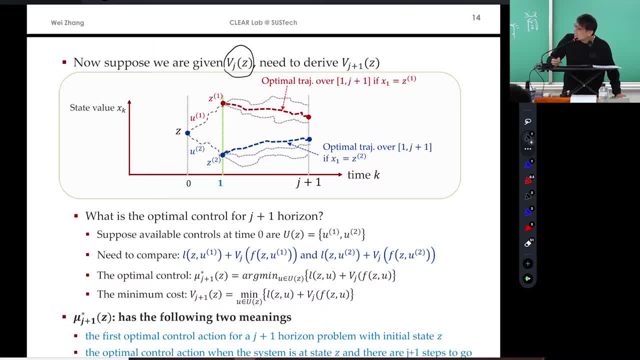 And the fundamental cost is j. That's what you need to go to, so we'll use that. now Let's look at this figure. Let's just look at this figure. I know you don't like dual vision. let's look at the figure. 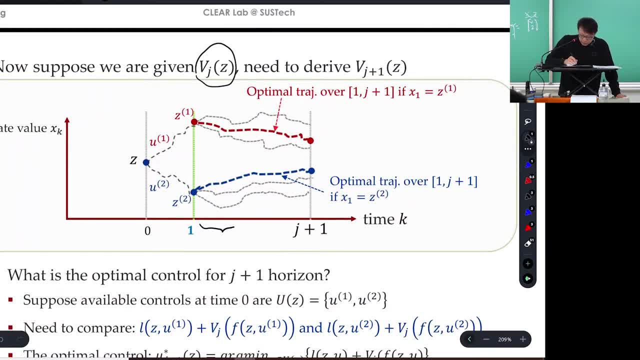 I'm giving you a problem. Suppose this is my j horizon problem. right Now I'm considering j plus one horizon, My horizon. I'm going to call it j, All right, so let me compute size increase by one. Suppose I have to solve the j-horizontal problem. it means what? 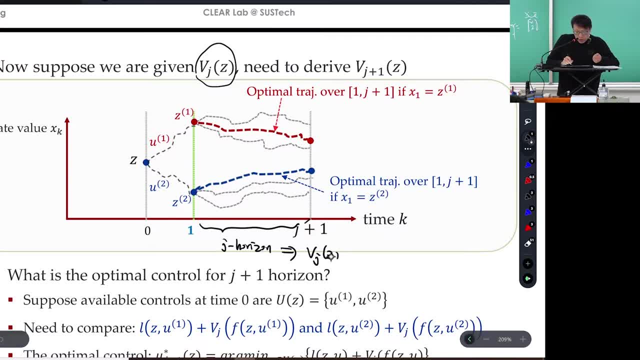 I know this thing. that's what I've given right. J of z. What do I mean by that? I already solved it. I know the optimal cost. If I have j steps, my initial state is z. That's already solved. 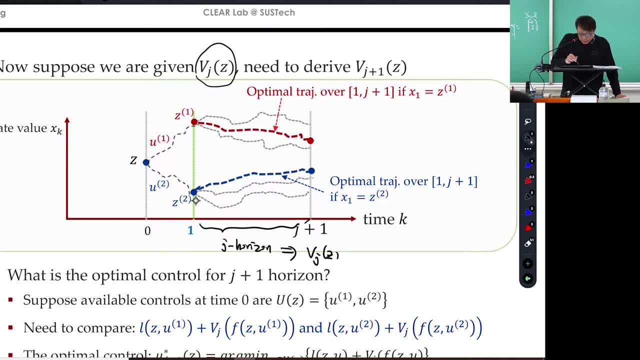 And suppose: well, the z can be different. right, The z can be different. Suppose there's a 2z possible, z of 1, z of 2.. That's two different states. If you start from here, I know the optimal path is this. 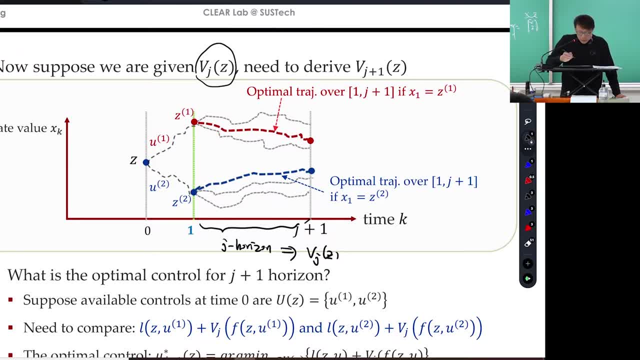 If you start from here, the optimal path is this. That's from the figure. Now I'm going to give this figure some number. Suppose this is 20, this is 100, okay, That's the optimal path. Has 20 cost. 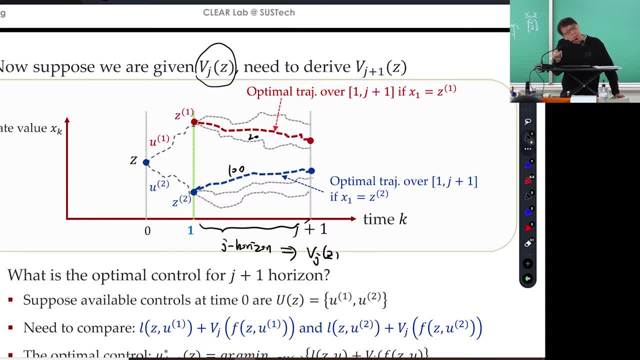 Okay, this guy, But this guy optimal path, although it's optimal, but it's still pretty big. it's 100.. Because the initial state is different. Are you with me? So these two guys, which one is a good initial state? 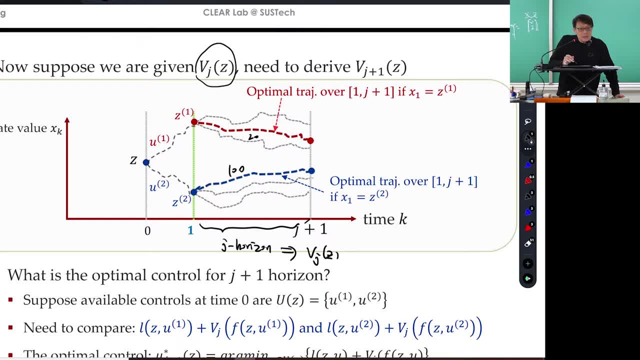 Z1.. Z1, right. Z1 is a good initial state. Z2 is a not so good initial state for a j-horizontal problem. Now I'm going to consider j plus 1 horizon, So suppose I start from here. I start from this: Z, capital Z. 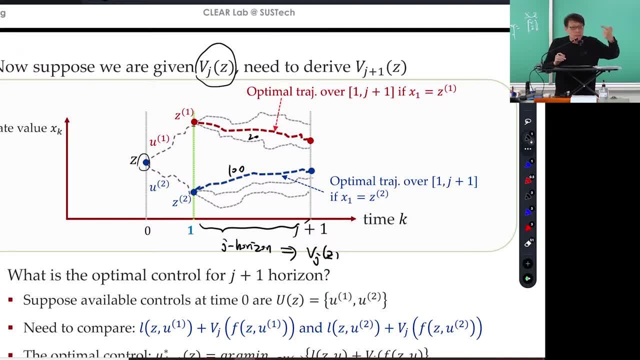 I have two choice. suppose, At any given state you have different control actions available for you to make decision. Suppose at this z I have two choice: One is u1, the other one's u2.. Which one is optimal? 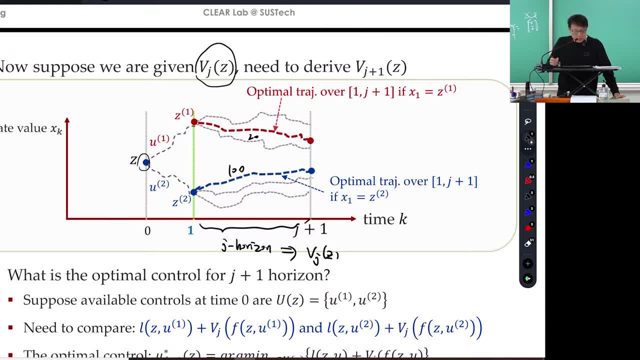 u1 and u2.. Well, that doesn't mean no, I don't think so. right, It depends on what number I gave you, Right, It's hard to beat. You know that It depends. No, I don't think so. 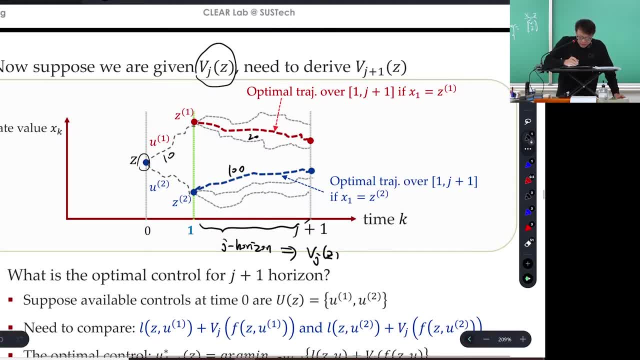 It could be this guy. This step is a hundred, This step is one, Okay, so take this one step May give you a hundred, Okay, and take this step will give you one. and overall, after this step, Which one you should take. there's different paths as well. You should definitely take this right. That's Bellman's principle of optimality. 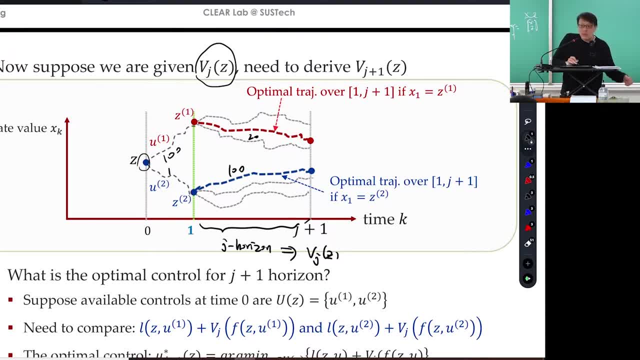 I already solved this problem. I don't need to resolve it again. I know from z2.. This is my shortest path, so what would be my V J plus one of the in this figure? What's the cost number, Depending on which path I take, right suppose about which one is better. This is: total cost is 120. 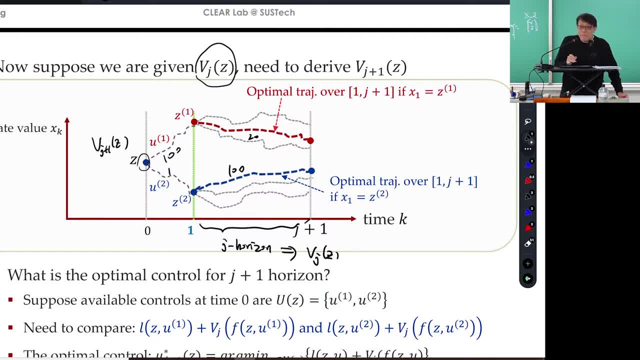 This total cost is of 101.. Which one is better? This path is better, so the cost would be 101. this is my value function, Right? this is my value function. so you should take down here. Well, that depend on as I mentioned to you in 10, that's this depend on my number, right suppose? 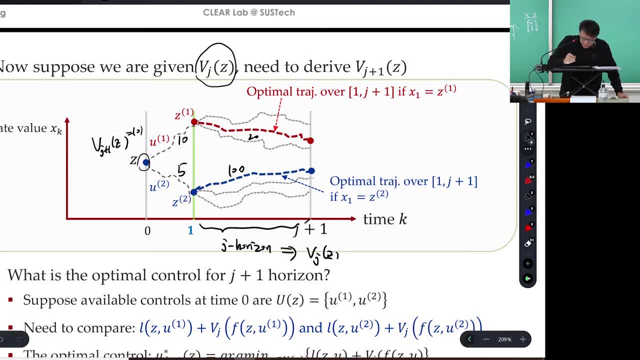 Suppose my number is like I'm going to test you, This is the five, this is ten, This is the 5 I'm going to take. I take 1 and this is the one. What's my optimal decision? What's my? u here is zero, This is a time zero, and 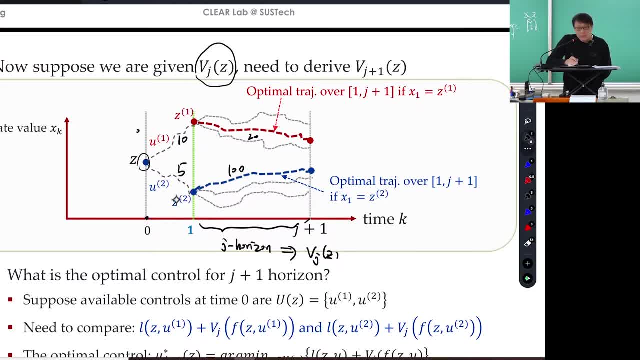 J plus my horizon time zero. so, as we take action, which action has to take, If I only look at this one step, cause this is running cost, then I should take this guy Right. I should take 5, because that's give me my most, the smallest running cost. but taking this step will cause me to a very, very bad initial. 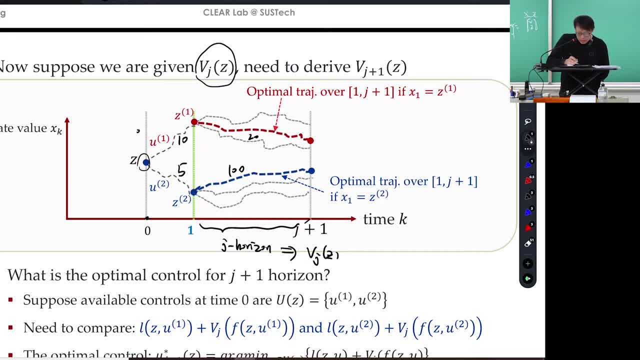 state for the j-horizontal problem, All of these particular steps. I save some cost, but later I have a larger cost to go. Okay. So if I consider not just one step, this is called greedy right: You only consider the next step. If you consider today's happiness, 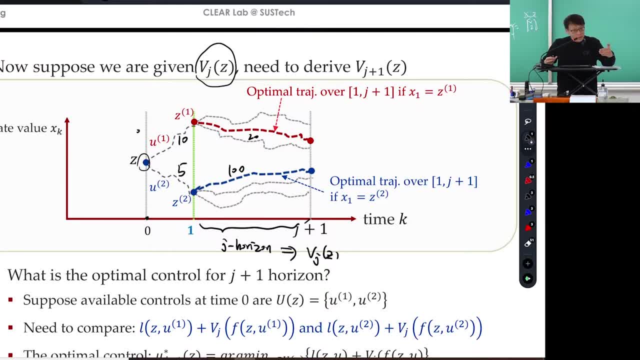 you will play games Right. If you consider the happiness after finals, you will study Right. Okay, That's the use of the. consider what, Use the consider, use the plan, use the think. if you play games, you will enter a worse state. 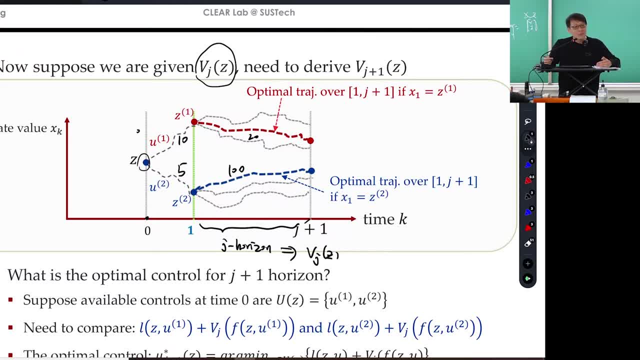 Later on you'll have more time need to spend for a class and the GPAs. Your entire life depends on your everyday's running cost- what decisions you make, Right, Of course, today's happiness is also important. Okay, So I hope that's fine. So, in this particular number, 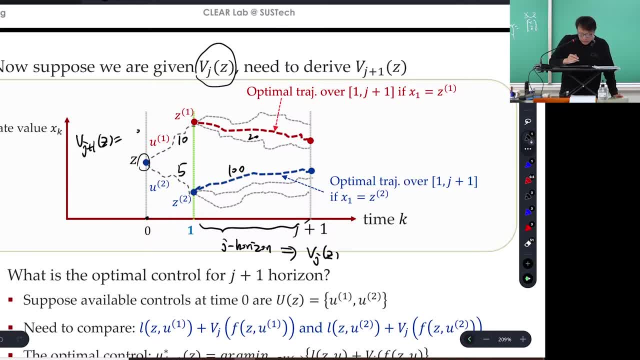 let's write down. let's give you one more case. What is the optimal value function for, say plus one, with this initial state, In this case number 30, right, So it's 30.. Because I go, you should go here All of the 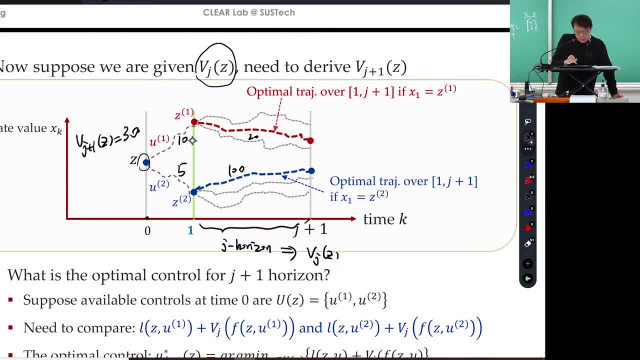 first, today I'm going to suffer a little bit, but later I'm going to have a really small cost. So overall it's 30. So you know how to make decision now. What do you need to compare The running cost? just one step. 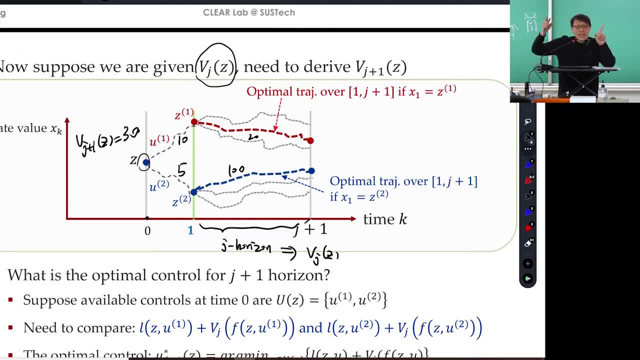 Plus the future cost of the next J cost. J step cost, optimal cost. Does this matter? Does this two curve matter? Maybe I have a lot of other curves. It doesn't matter anymore because I already sort out those things are not the optimal ones, I don't need to worry. 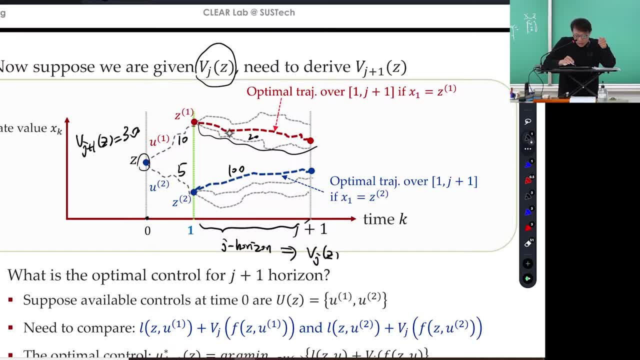 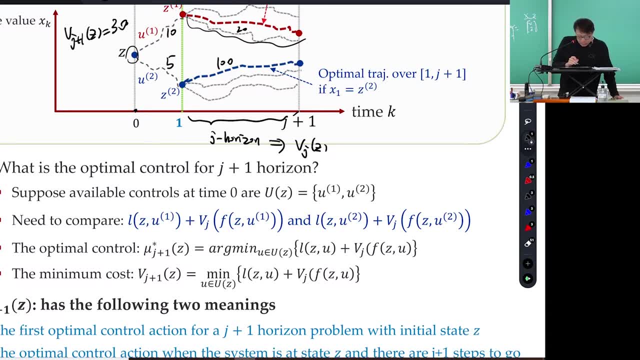 about them anymore. Okay, I only care about start from this. What's my optimal cost? Okay, I think that's the figure By the equation. that's the following: Okay, So available at time: zero if J plus one cost. 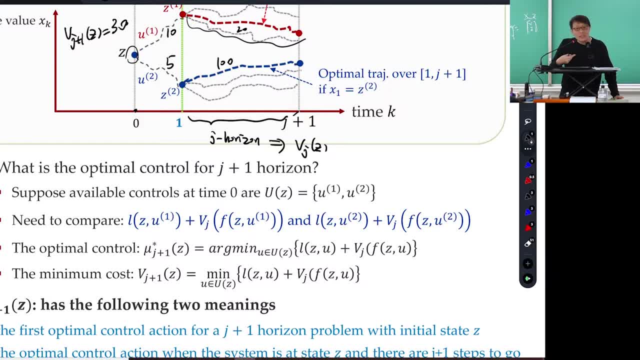 is U1, U2.. And what we did is mathematically what we're doing. What we're doing is comparing the sum of running cost plus the future cost, the future cost, the future optimal cost. If I apply this step, then I will be at a different location. 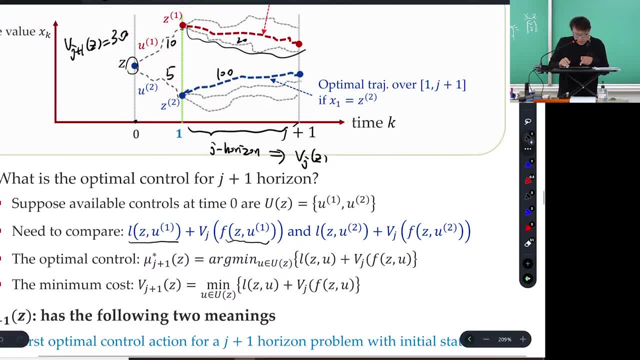 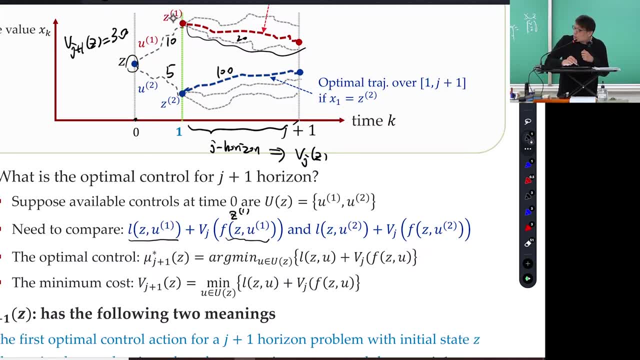 So this means I have Z of U1 is nothing but the Z of one. If I use U1, I will enter here This is right Z1.. If I use U2, the next step- I will be here Where I am. next step is super. 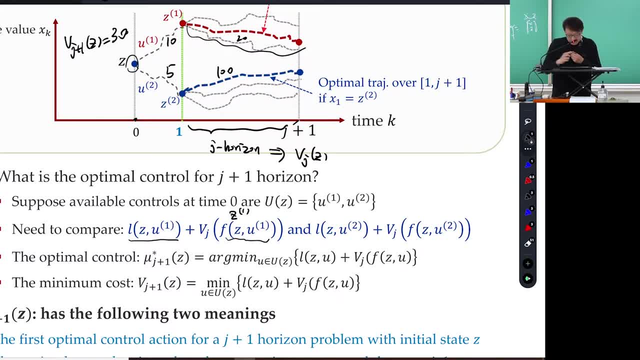 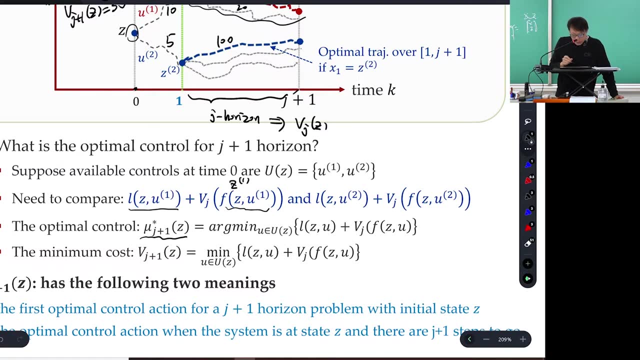 important because that determines my future cost. So I need to compare these two numbers. I pick the small one. That's my optimal decision At this stage. Okay, So mathematically my optimal decision is what It's whichever these two, So U1 or U2, depending on which one, I am right. And it's argmin. What does argmin? 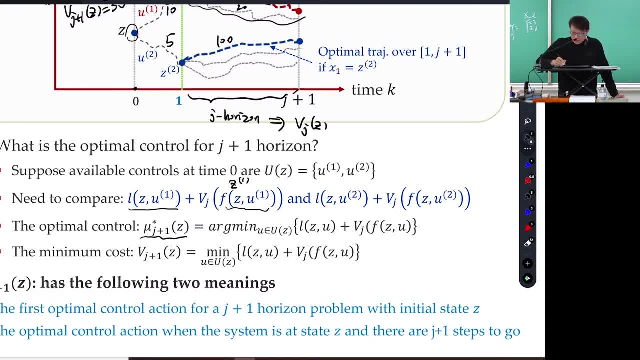 mean. So the mean of X2 plus one is one right Argmin of X1 plus two is what One Right It'szeigt Zero. That base value is now zero. It's the minimizer minimizes this cost. The minimizer means X equal to zero. That's zero. 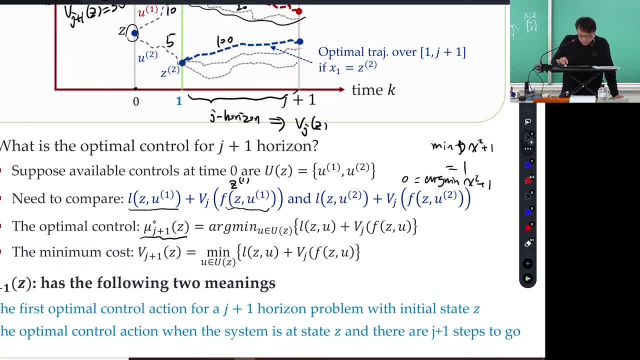 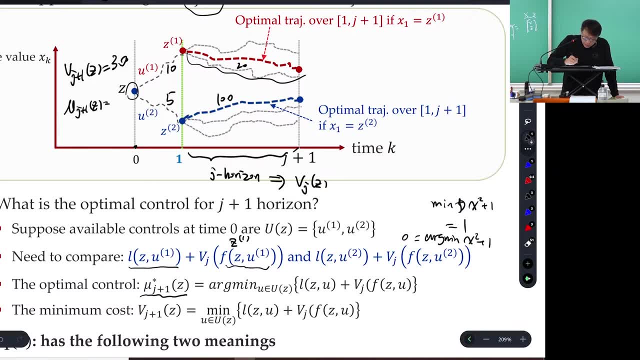 it's the minimizer In this case. if I look at this number- In this case U plus one of Z equal to what U of one- I should go up Yes, Right, Right In this case, That is correct. 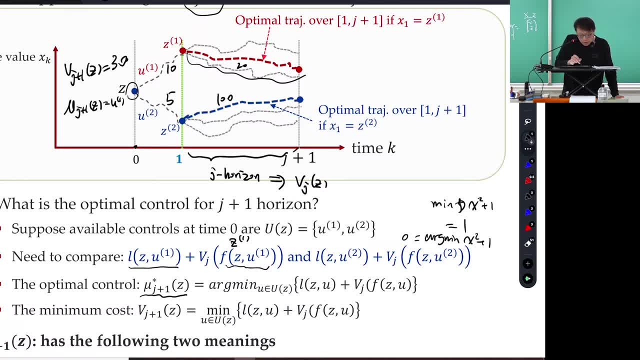 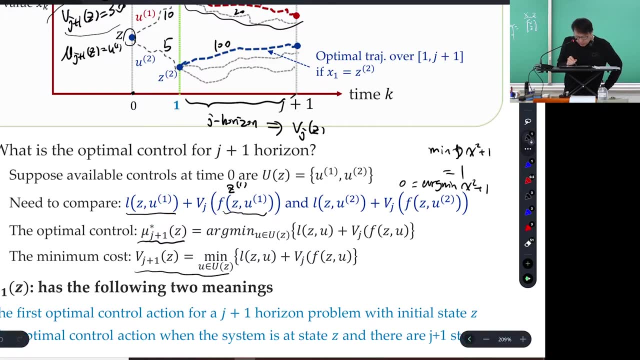 At this step I should go up. Do you see what I mean? At least step I should go up. That's optimal cost. that's my optimal decision at this time and the overall optimal cost is this, running plus the future. so the minimum cost is nothing, but i minimize over all the possible contractors. 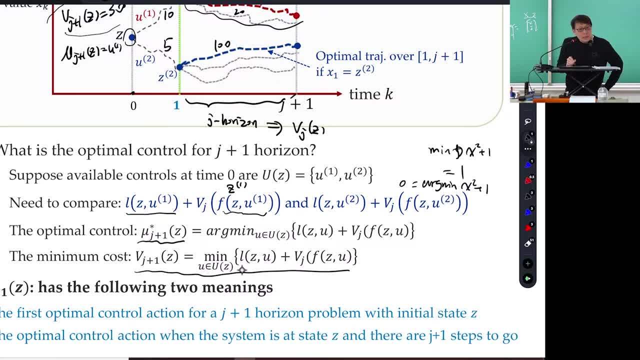 i have at this stage, okay, and what i compare? the running cost, just immediate satisfaction, right. today's happiness plus the future suffer the future cost, right, but you take the optimal you, you only care about optimal ones, right. so you don't study today and you assume tomorrow. 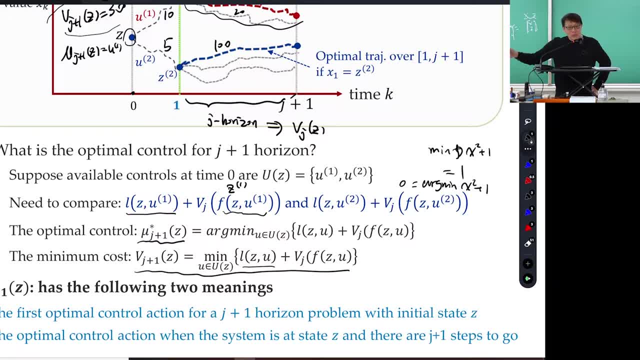 you study in the optimal way into the next, until the final. that's your cost, right, versus your study today. i mean, well, anyway, i know you don't like study, um, it depends, right. uh, so i don't like study for the exams, i like to study to understand things. 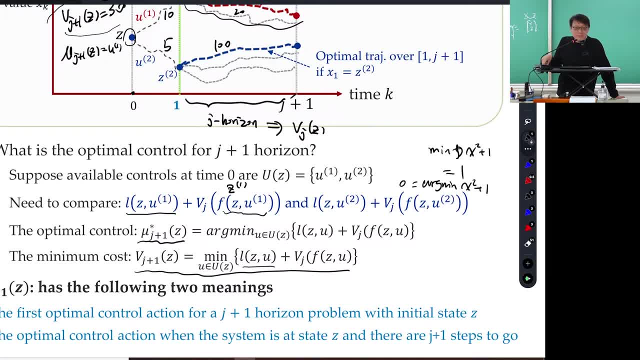 i think everyone has its own curiosity. okay, we like to study to you. you can google all the time to satisfy your curiosity. maybe that's about pop stars, maybe that's about some kind of knowledge, but that's fine, that's curiosity. we like to study to satisfy our curiosity. 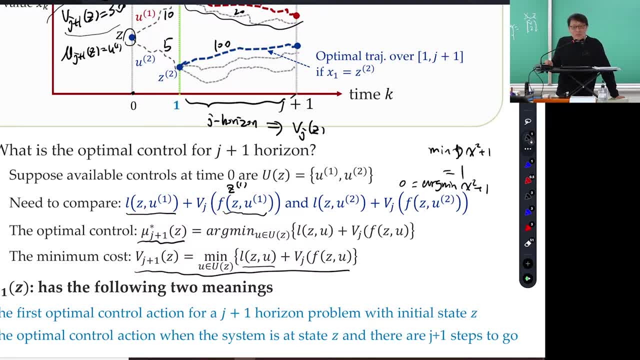 but we don't like to study for some kind of exam. but sometimes this is the way we learn right: you have to have some pressure to learn, um, i think so this equation. does anyone- i mean does everyone- understand this equation? now, vj plus one z, equal to mean. 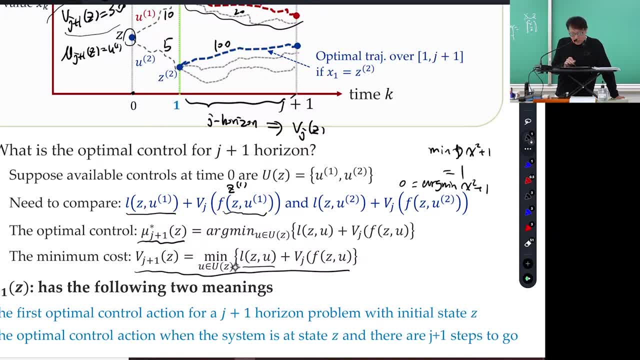 of a value control mean over the other possible contractions and how, what kind of control, what kind of metric i determine which controls we use? is running cost plus future optimal cost? your current decision will affect your what your next state will depend on whether you are in a better or worse position for the future cost. 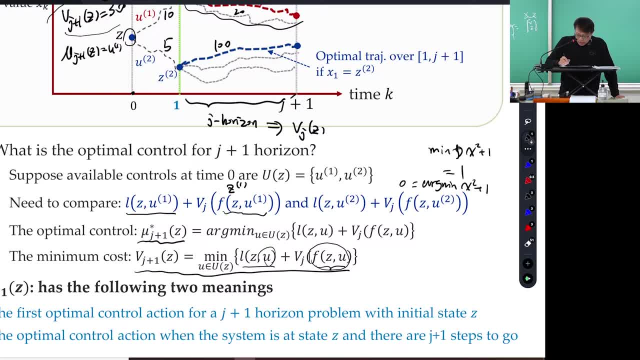 a future remaining decision problem. okay, okay, and this, this particular equation is called bellman. okay, it's bellman equation. another: it's not a biome equation, it's former recursion, or whatever. okay, uh, this value iterations, you, you well, anyway, so value, it's just called this. 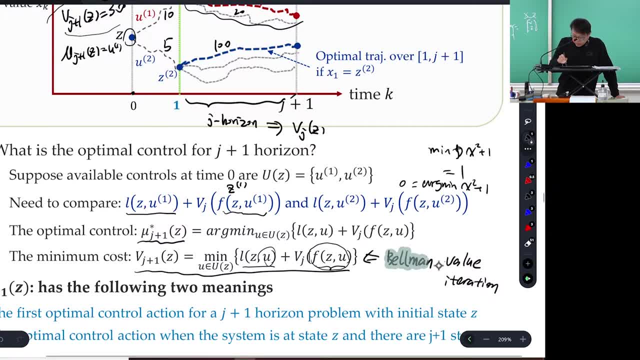 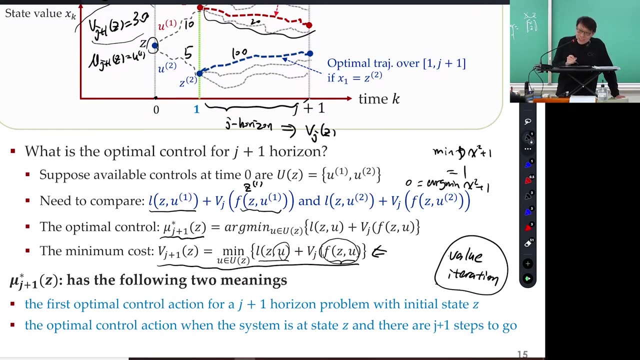 is just value iteration- sorry, it's not filming equation- value iteration- that's exactly value iteration. we already learned about iteration and these two has different meanings. we all know this guy's meaning. right, if you currently have type at state z and you have z plus by horizon to go, 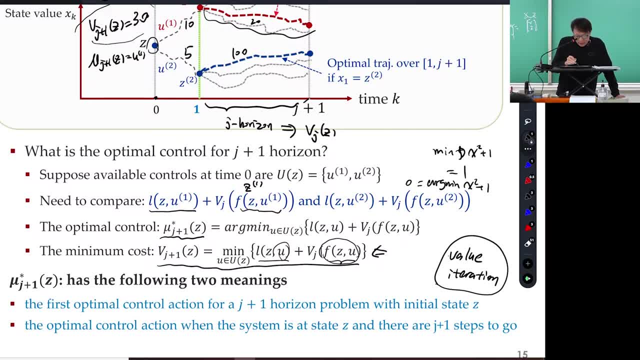 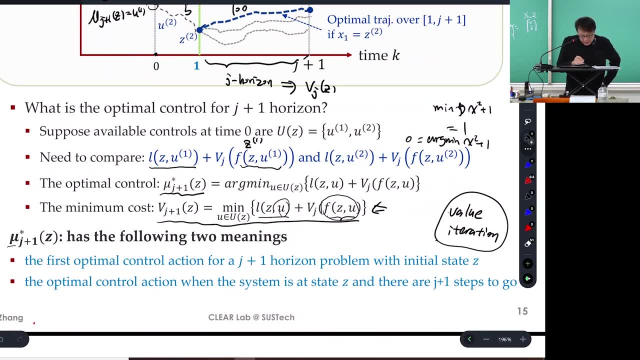 then that's my best cost i can have and this guy is the corresponding by a best control action i need to take. okay, so i need to explain a little bit this guy. it may be confusing for some of you. this is mu, not you. you know mu and the? u different right mu. here is a function. 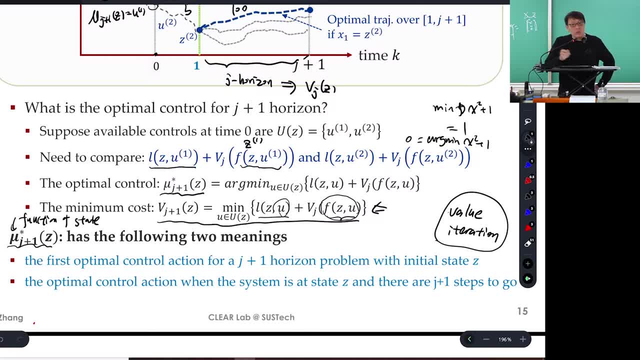 of state, which we call control law or controller. okay, versus the control action. that's the particular number. the controller will will. will will output, right? this is a control law. it depends on. this is optimal controller? okay, it's a function of state. it depends on where you are. 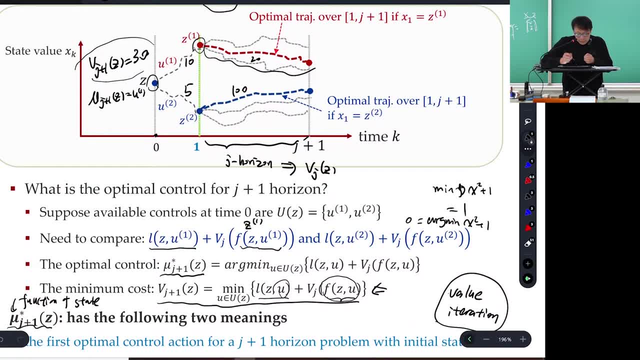 it depends on where you are. for example, if i'm here, this guy, this path will be my optimal control, all right. and if i'm here with this part will open, my optimal control depend on where i am and also depend on where how many steps i have. 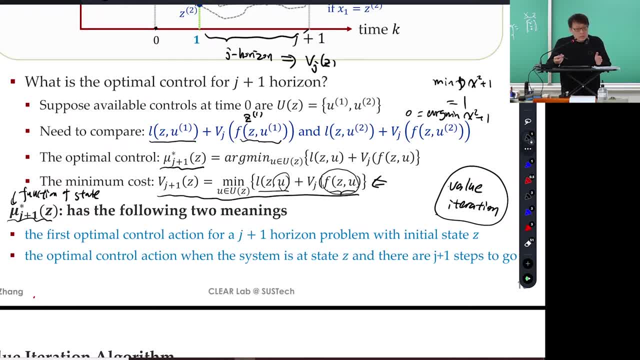 okay. so if tomorrow is the final exam and you didn't learn anything yet, maybe the optimal control for you is to play games. right, your gpa will be the same, right so. but if your final exam is 10 days away, then your opt-in decision today maybe, maybe, still play games. 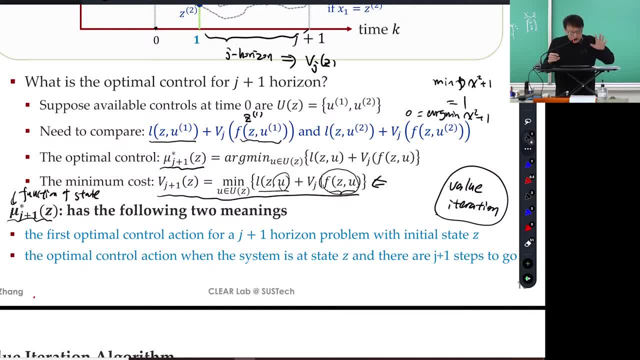 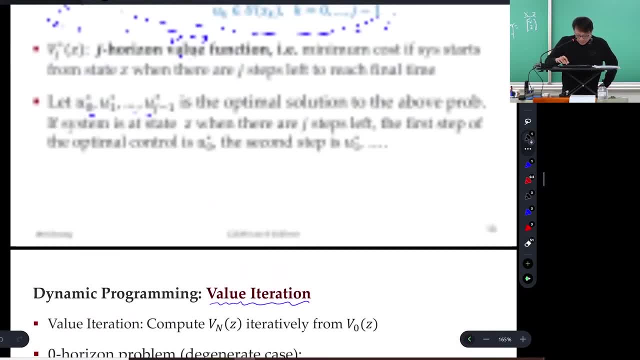 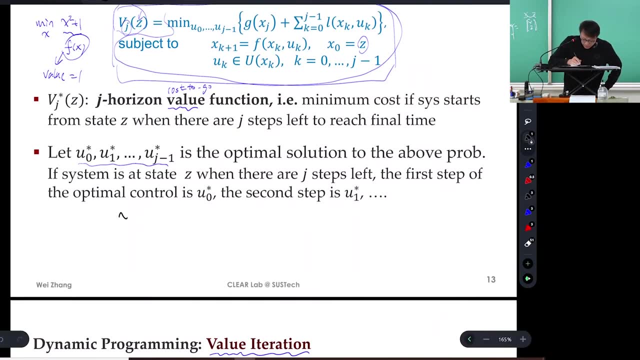 but maybe study a little bit that will be different. right, the time horizon depends. it also decides, determines the optimal action you need to take. i'm going to test you with: uh, these are control actions right to solve this problem. but i'm going to test you my notation now. okay, so this guy is a initial state. 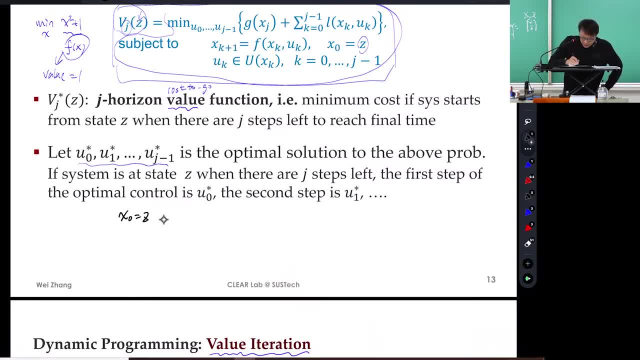 x0 equal to z, suppose. right, uh, then i take the optimal contractions. so that would be my u star, u0 star. if i apply u0 star, i will be at x, one star, which is f, x, X, zero, U, zero star, If I apply my optimal contraction. 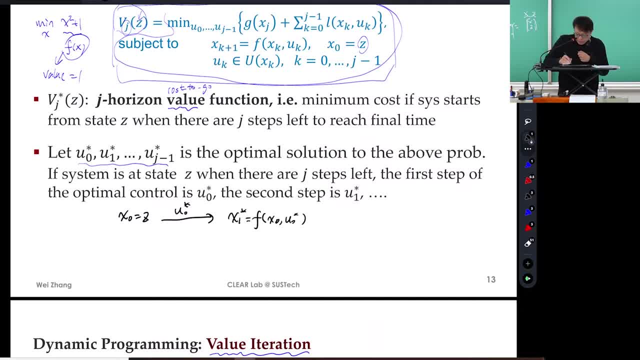 that will be my optimal state next time. Then I will apply U one, star, that's my optimal control at that time. right Then that will be optimal two. so dot, dot, dot. Eventually I will be at optimal X and star. That's my optimal trajectory. 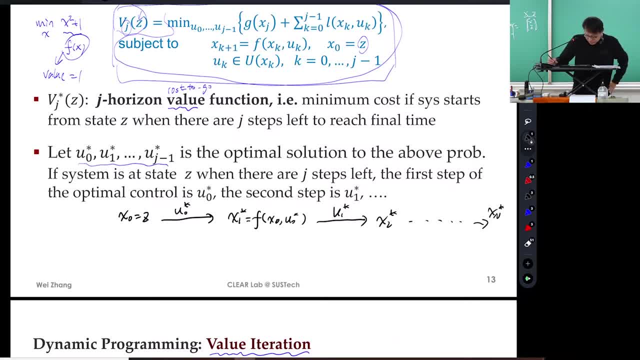 the system state trajectory: okay. So now I'm going to ask you to change the notation now a little bit. Suppose this is N-horizontal: okay, J equal to N. right, That's N-horizontal problem. I'm asking you: this is the control action I take, right. 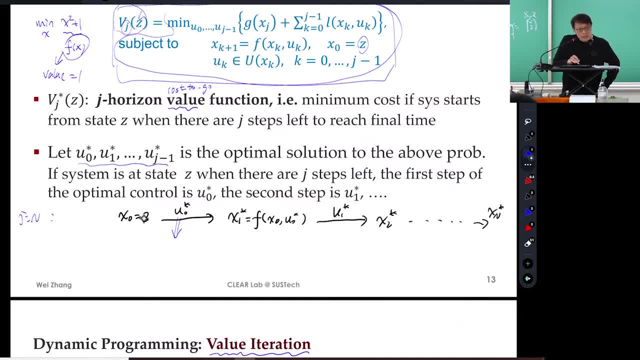 If I have N steps left, I'm currently at Z. So U zero star. eventually by my next notation will be this of Z star. okay, So this is the control law. okay, If I have N steps left, I'm currently at Z. 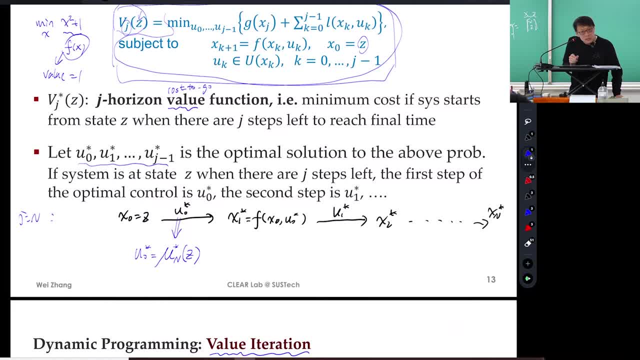 That's the contraction I should take. okay, That's a play game or not? That's this guy, And this guy means play games. This is a law, okay, The law depends on how many days you have. okay, The law depends on how many days you have, okay. 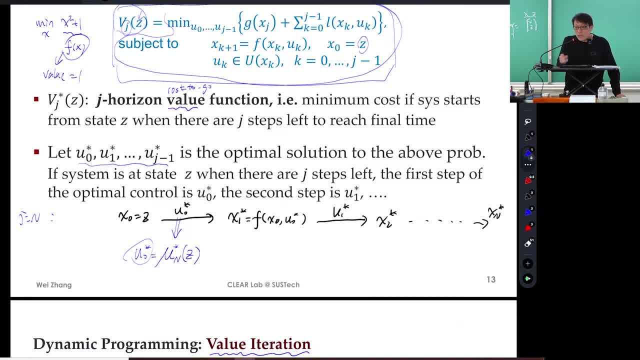 The law depends on how many days you have and also depend on your readiness for you to take exam. If you're just missing a little bit, you will still study. If you didn't learn anything yet, you will just give up, Right? 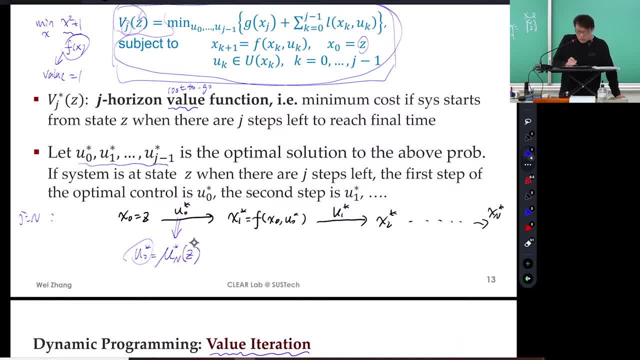 So that depends on how many days you have, depending on your readiness, depending on where you are. Now I'm going to ask you: what is this? How many steps I have left? 10 minus one, n minus one optimal contraction where you are. 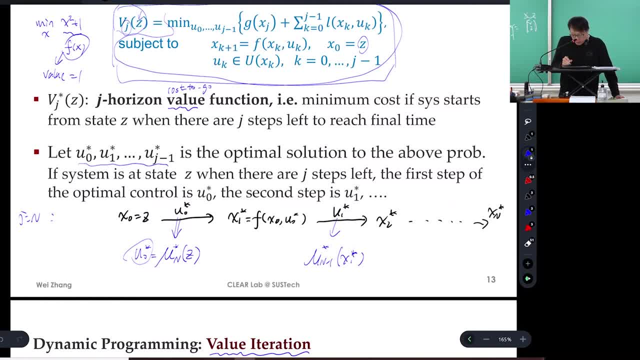 X one star. Okay, So this is u one star. The second, this is the second step. you take that optimal one, but it's equal to the optimal control decision. you should apply it if you have n minus one step left, but you are at x one star. 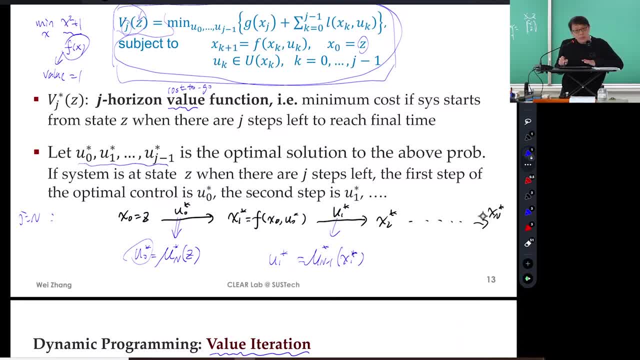 Okay, This sequence was determined by solving an n-horizontal optimal control problem But, as I mentioned, Bellman's Principle of Optimality. if I look at this n-1-horizontal problem, this will become my first step to take. okay, You see what I mean. 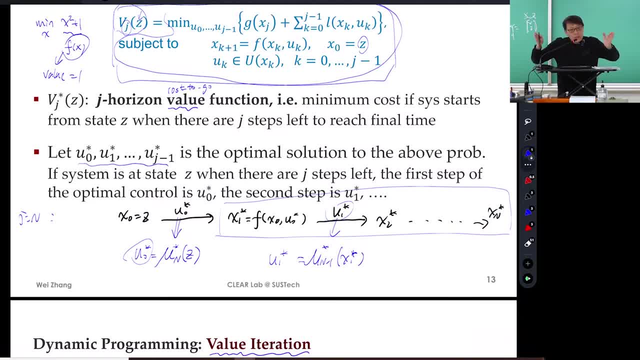 If this is my- I only consider this problem- then this will be my first step to take and this x1 star will be my initial state for a j-plus-one problem, n-minus-one problem, And this guy will be the optimal control. 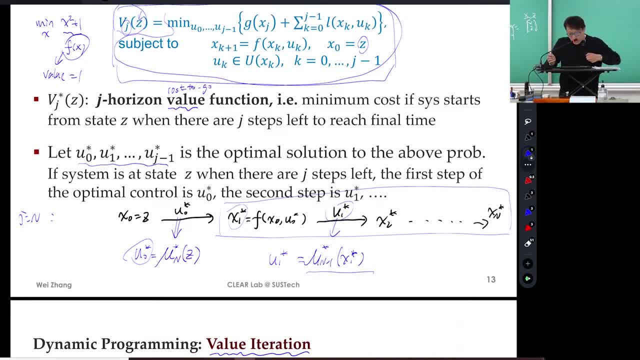 So this law is nothing but my notation. okay, It's nothing but the optimal control action I should take if I'm here and with n-minus-one step left. Huh, Say that again. Why is n-minus-one step left? Why is n-minus-one step left? 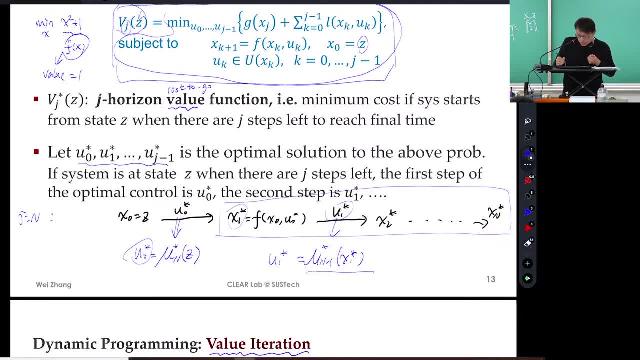 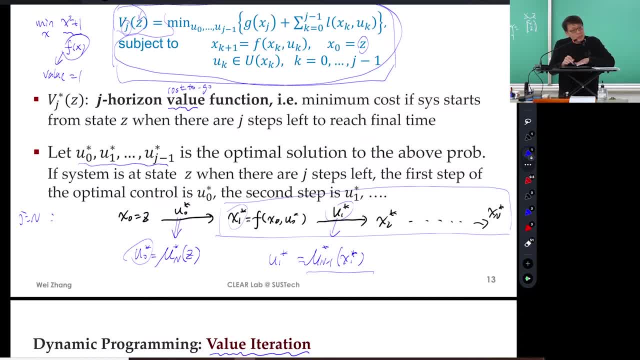 So okay, if you recount your starting point. so if I have j-plus-one problem, I'm currently at here. so time changes, right Time changes. This will be your x0 at time one. If you start your problem at time one, then x1 will be your x0. 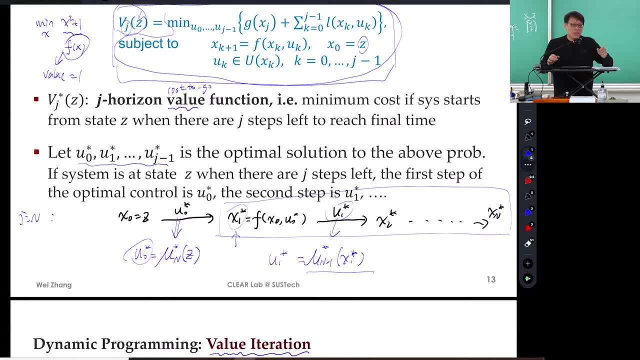 Okay, Let's do that anyway. x1 will be your initial state. okay, We already knew the optimal trajectory based on Fermi's law. Yeah, yeah, of course, yeah, So this will be your nj-horizontal, so that's why I called it z. 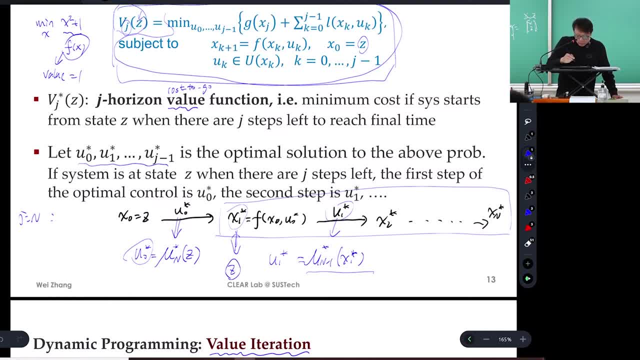 This is my z for a n-1 optimal control problem. okay, So that's a function, So I can start at any given time. All I need is that this function. You know, this is a function. This is a function of the initial state. 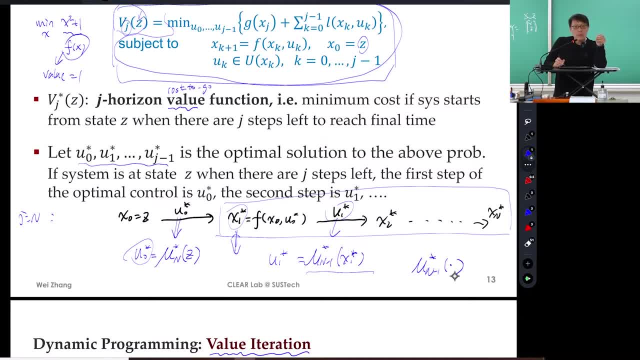 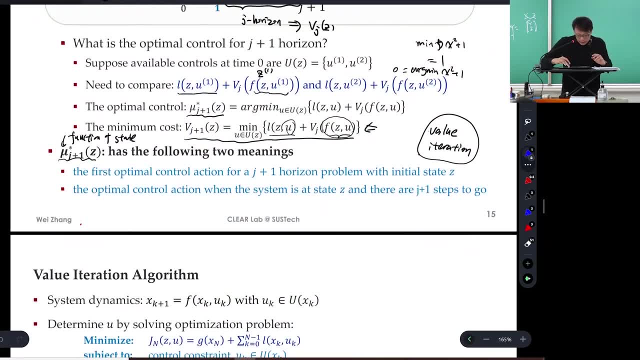 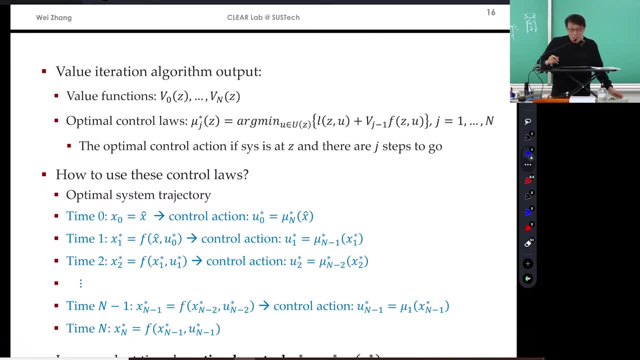 Depending on where you are and how many steps you have, this function will tell you the optimal contraction to take. all right, Let's look at an example. I think that will be. I don't think it's much better, but a little bit better, okay. 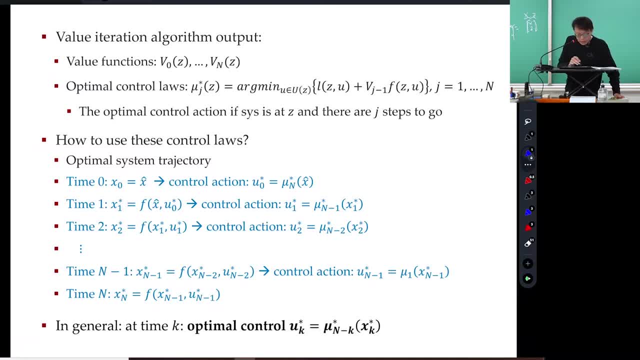 Here is some kind of summary. all right, So time 0, you're here, Control x and this is x0. But this is what? This is the optimal control x. If you plug a law, that's the optimal n-horizontal control law, okay. 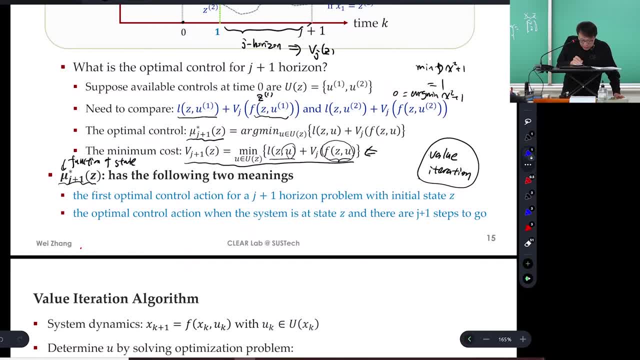 So I think I have an explanation here. That's this thing. What's the meaning? It's the first optimal contraction for a j-plus-1-horizontal problem with initial state z, Or it is optimal contraction when the system is at state z. 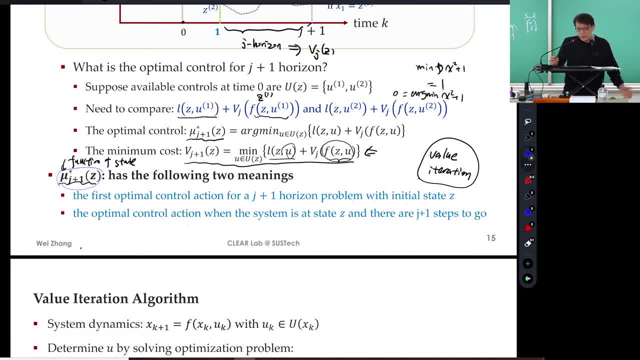 and there are j-plus-1 steps left for it to go. It will take some time for you to think. I think at least you have a rough, vague understanding, Maybe not complete, but that will take some after-class effort. Let's try to solve this. 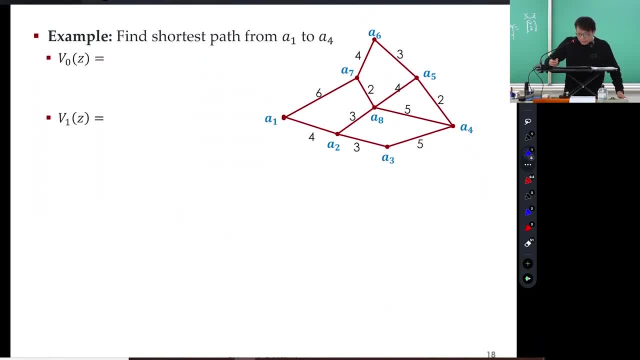 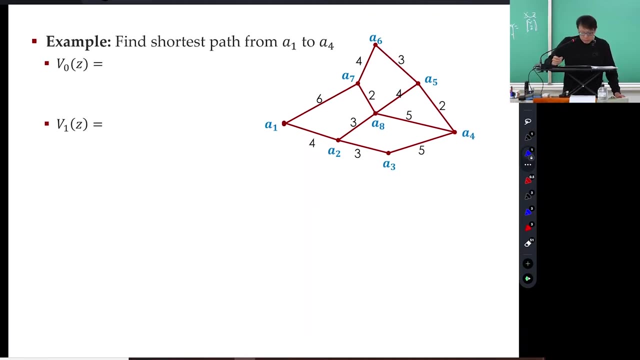 Let's try to solve this problem. all right, At least we solved some problem. This is the problem: the simplest problem, the shortest path problem. We can code. The coding will be few lines. okay, Now I'm asking you: based on my formulation, we start a value iteration, right? 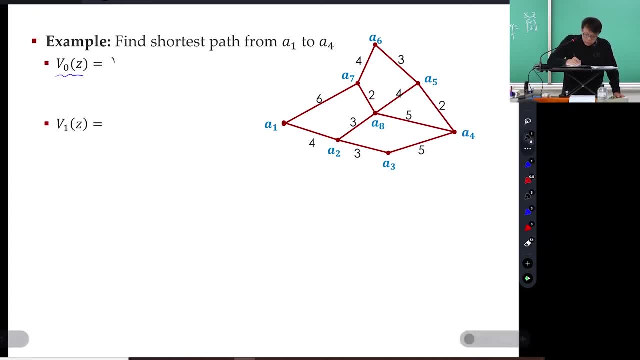 What is this? This will be my terminal cost, Which is suppose I want to go to A4, right, This will be zero if z equal to A4. It's infinity if z does not equal to A4.. Is this a function of z? 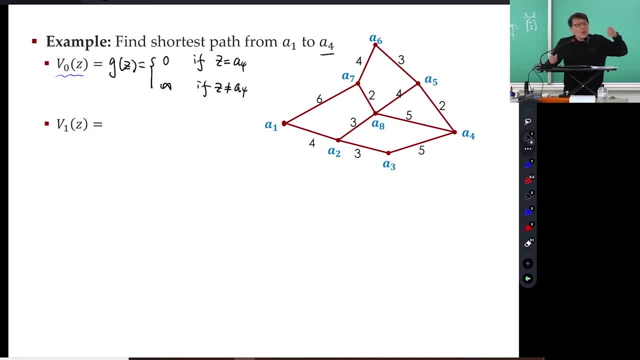 Of course It's a function of state. It really depends on where you ask for the optimal cost, Because the value function depends on the state. At different state you have different value function. Sorry, the value of the value function is different. 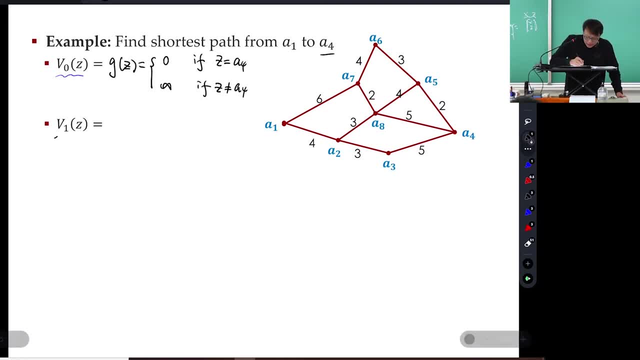 Okay, now let's look at Any questions. I have a question: If z does not equal to A4. It's infinity, Why? I just don't. Well, you can make it. You can say he thinks it's y. 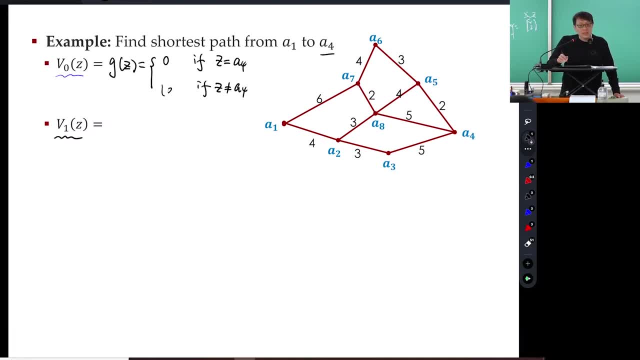 I can say it's 10.. If you didn't gather, I kind of gave you a fine: It's 10 bucks. But for me- I think I just want- That means you are not there, Or in my lab it's nan, whatever I. 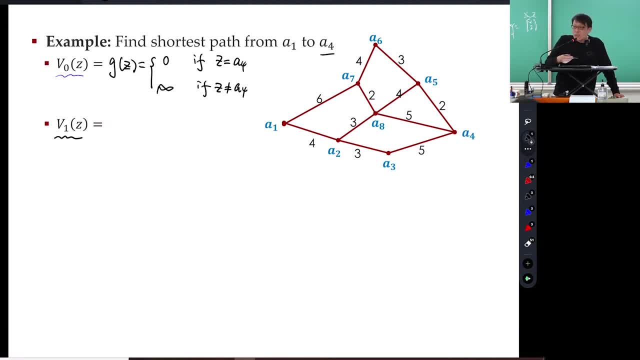 Whatever I want to, I just say: you didn't get there. That's a discrete thing. It's success or not. Success is zero. If you didn't success, you're dead. You're dead. That's infinity. That's my cost function. 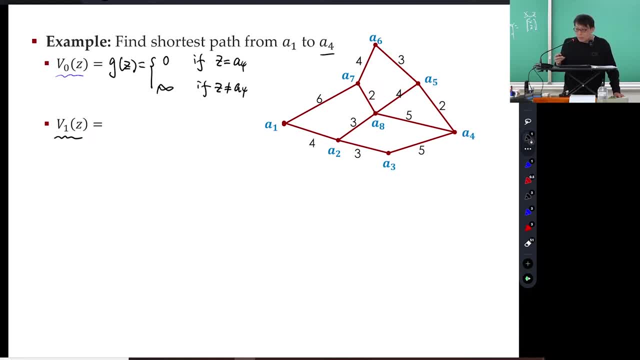 You can have a different cost function. Okay, Let's look at the. Let's work on a few steps. You will see why that's reflected. the shortest path problem- Okay, Let's. I don't think we need to redefine. We already formulated the problem at the beginning of today's lecture. 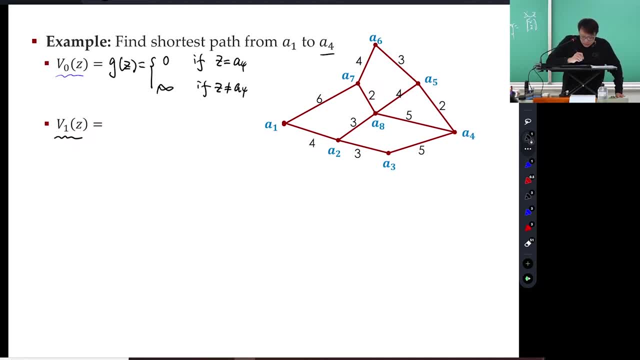 What about v1 of z? Okay, So we already know v0 of z. What about the value iteration formula? That means from u, from u of z the running cost plus v0 of fz of u. That's the value iteration formula. 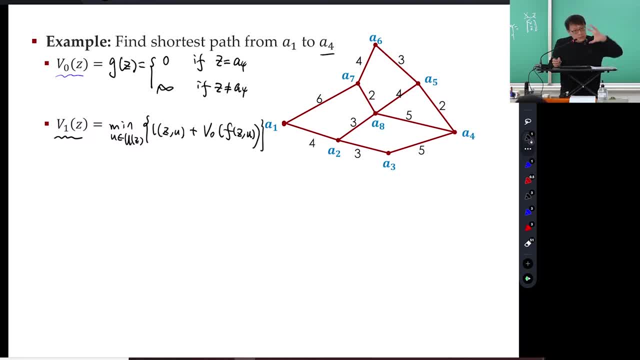 Let me repeat: This is the value iteration formula we just explained with that figure, Today's happiness. It will lead you to some state which is f, x, fz, u, And start from there. you take the optimum cost, But the horizon decreased by one. 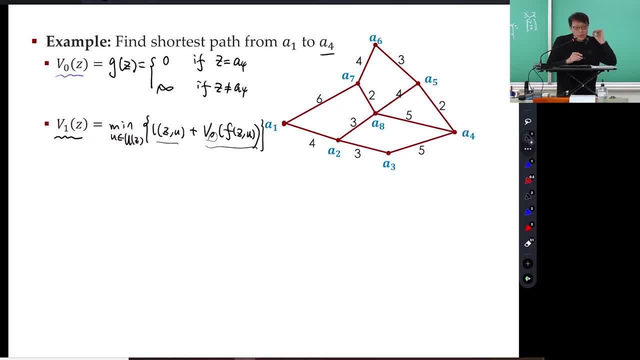 You have one day shorter time, Okay, So let's take, Let's look at an example. Let's say v1 of, Depending on what z I'm asking, right, Let's say v1 of a3.. What is it? 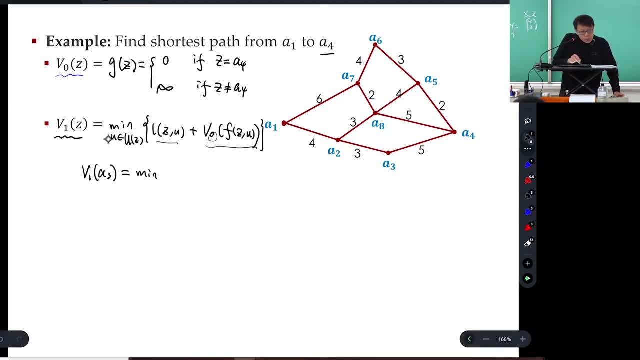 That's minimize over the possible contractions. I have A3.. Where is a3?? Here I have two actions to take. Right, So that will be. I need to compare two contractions. The first one is L a3.. 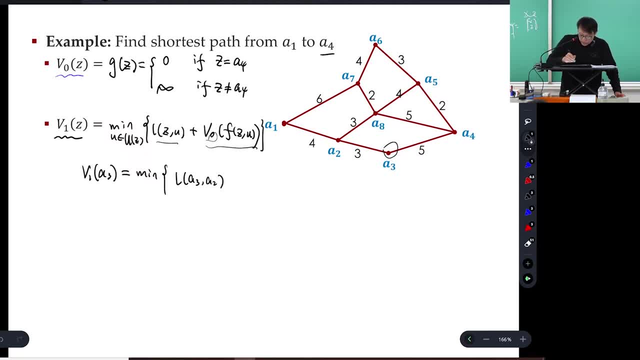 I go to a2.. Right, A3,, a2. Plus if I add a2.. But I only have one horizon left, But I try my best to start from there. That will be a2, right, That's f. 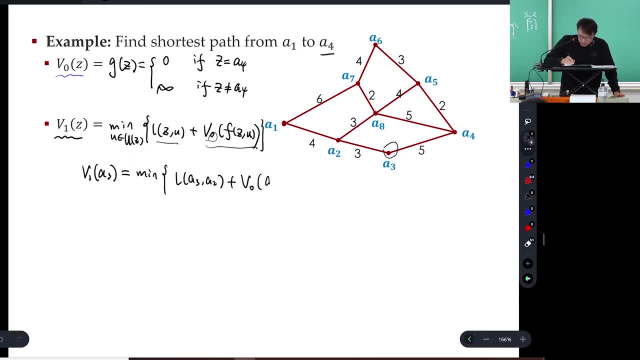 Next time will be a2.. In this case I will directly plug in a2.. Sorry, That's one action. Okay, The other action is a4.. I need to compare this guy: a3, a4 plus v0 of a4. 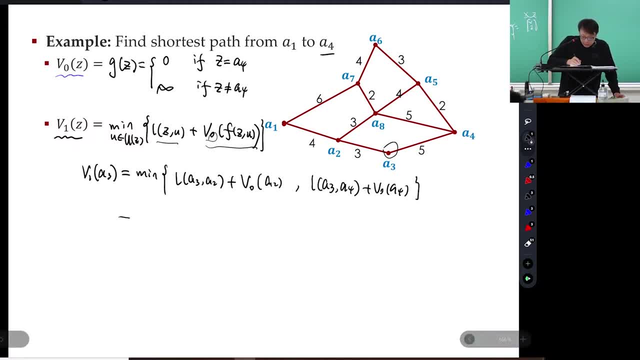 Okay, I need to compare this number, Two numbers. What are they? This guy is? This guy is a3 plus infinity. Why, this is infinity? You plug in this infinity. Okay, This guy is: This is a5. Okay. 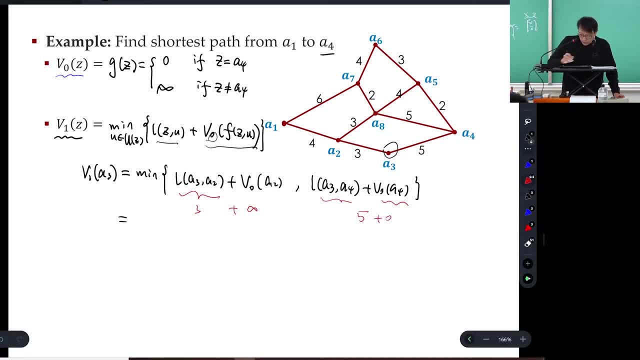 So 5 plus 0. So it's 5.. So overall I have 5.. Okay, And my mu1 star a3, what is it? Again, what does it mean If I'm at a3, I have one step to go. 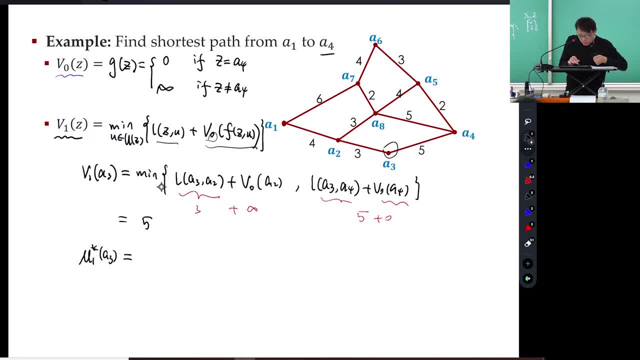 My optimal contraction is: This means I take a2.. This means I take a4.. So the optimal control is a4.. What does it mean? If I'm here, I have one step to go. I need to directly go to a4.. 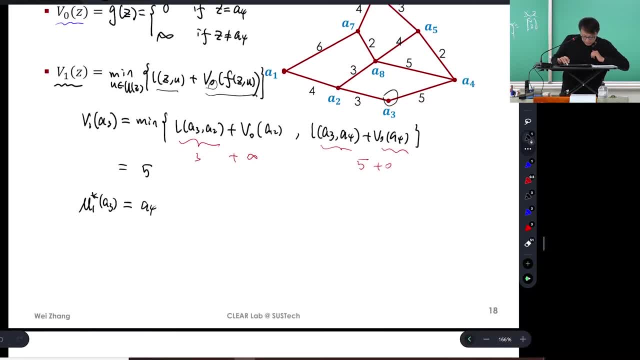 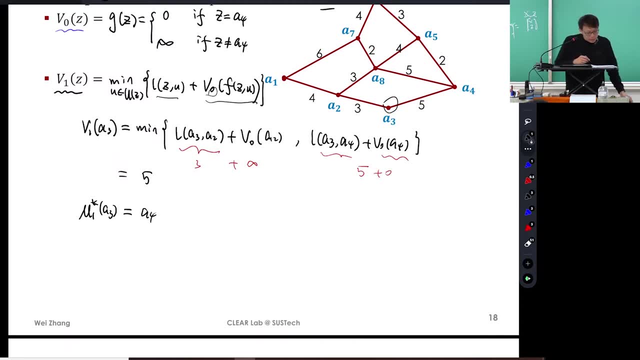 I need to directly go to a4,, of course, Okay, That's my optimal action, But the action depends on where I am and how many times, How much time I have. Let's see v1 of Let's see. 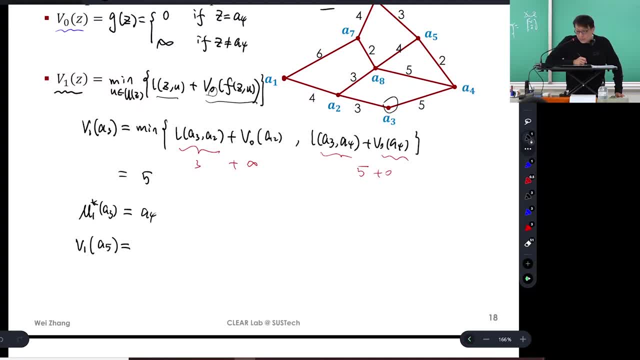 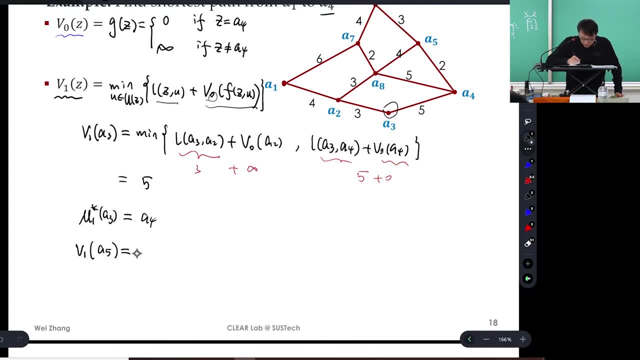 What about a5?? There's three, But I don't think Repeating this, you know this will be what- Two. Right, Because you should directly go here. This is two And a5 is two. a8. v of a8 is five. 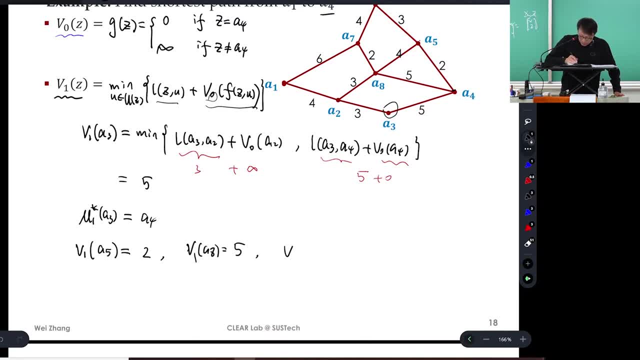 Right, And what about v? Well, sorry, v1.. What about v1 of a2?? v1 of a2? v1 of a2?? You have three choice. All of them will give you what Infinity, infinity, infinity. 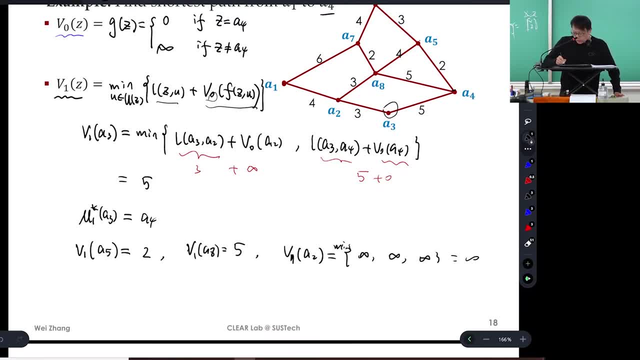 Three choice Mean over the three choice is still infinity. So what about v1 of mu1, of a2 star? What is it? Equally bad, Right, Equally bad. So I can randomly pick one Or I can. 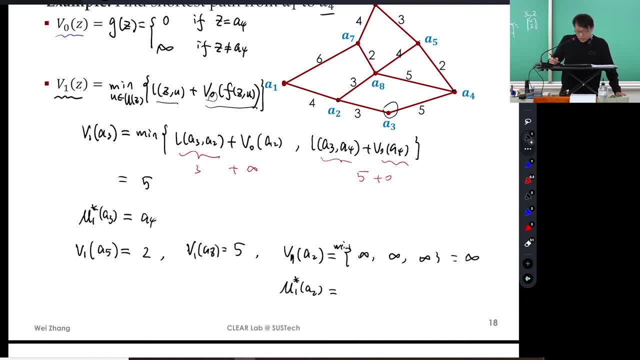 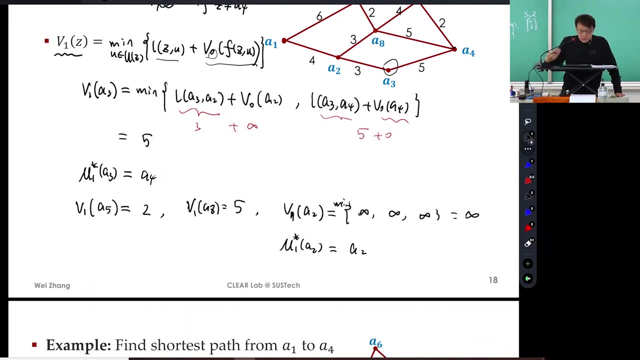 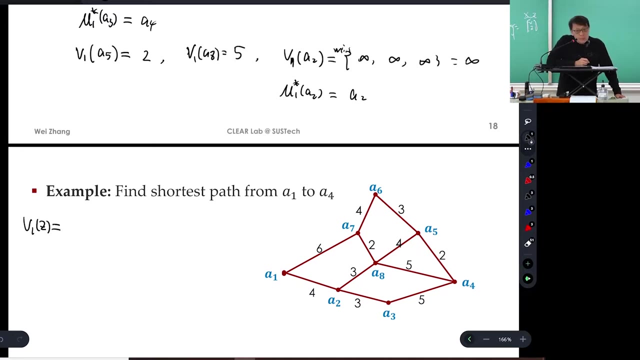 It's hopeless anyway. right, So I can pick any one. All right, I can pick. let's say I can just pick a3, a2 as well. Anyway, it will give me infinity according to my cost. So overall I will have v1 of z is a function. 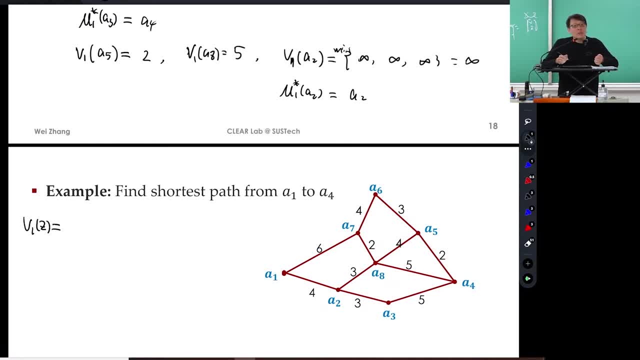 This function? what does function mean? You have to define its value for all the possible z. How many possible z? I have Eight, So, but it's 2 if z equal to a5.. It's 5 if z equal to a8. 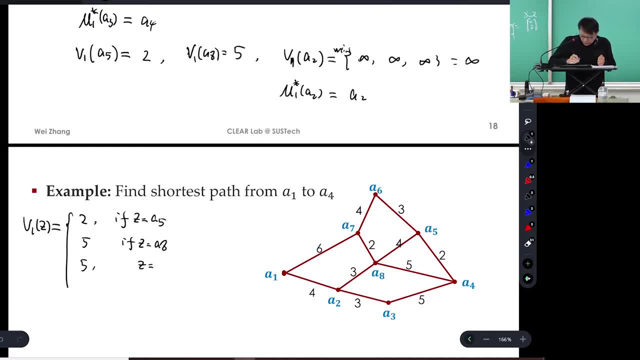 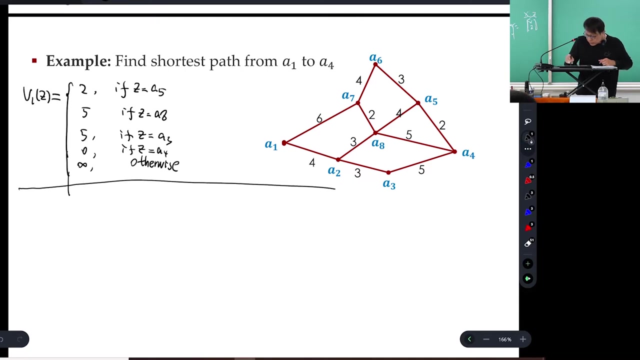 It's 5, again, if z equal to a3. Is infinity otherwise? Oh no, Sorry, Is 0. if z is a4, right. If only have this four finite values. all the others are infinity. The more important thing is the following: 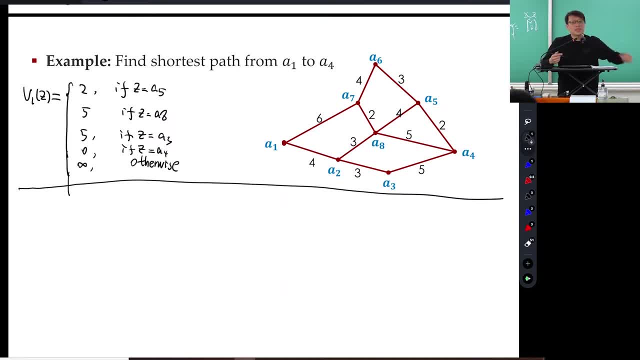 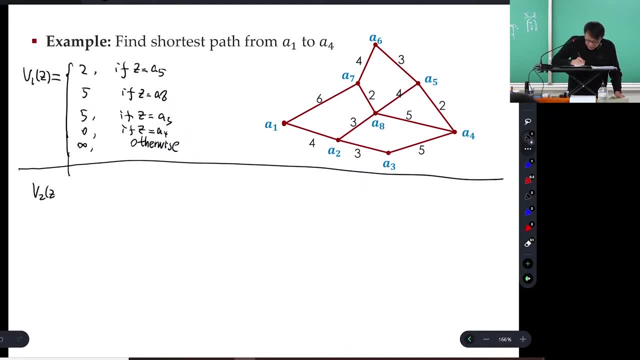 We have time for quiz, right? Have five minutes. Okay, that's good. v2 of z. Let's do one more right. v2 of z is minimize. You first write down the value iteration formula: Is u, belong to u of z? 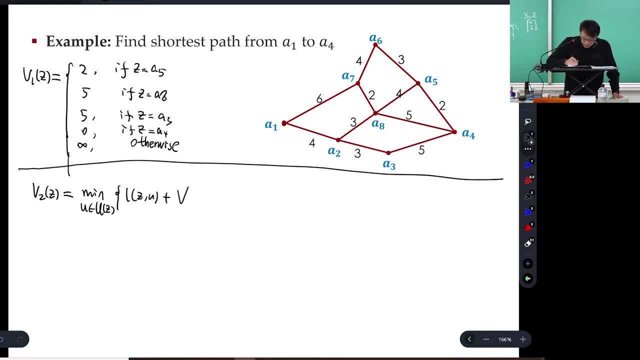 I own z of u plus v of what? 1. S of f? z of u, The running cost plus. if you take this contraction u, you will be at the next step, And after the next step you have only one horizon to go. 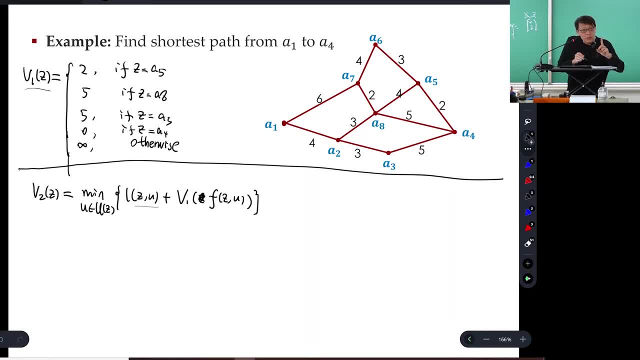 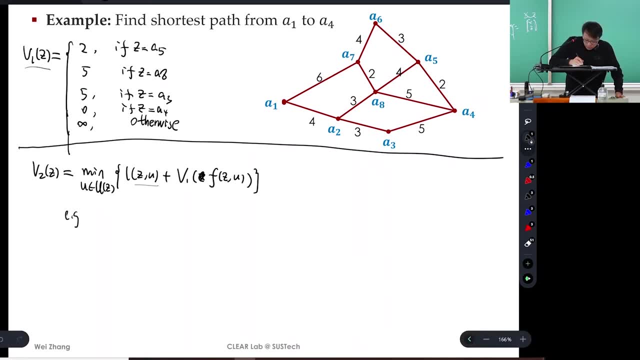 But you already compute everything you need for one horizon, So you can just do this. I wouldn't write everything. let's pick example v2 of a2. suppose you don't use your intuition, don't use your intelligence. think yourself is a computer. that's it right. you think yourself is a computer. what you need to? 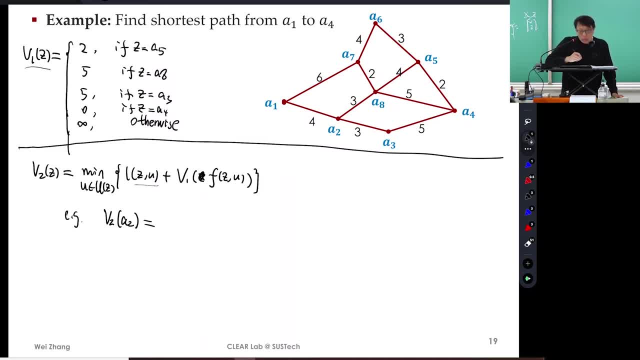 do is the same is this: minimize, you find out how many accent you have. so you mean of a to add a to how many action. you can take three, right? so you need to compare three numbers. okay, the first one: if you take to a1, that means that's a, I'll a to. 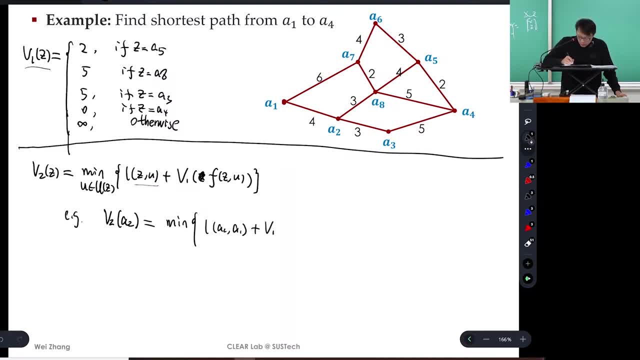 a1 plus v1 of a1. that's the first. I'll a2, a1 plus v1 of a1. that's the first. I'll a2 plus v1 of a1, that's the first. I'll a2, I'll a2, A3 plus v1, A3, of course if I stay at a2 as well, but well, maybe that's. 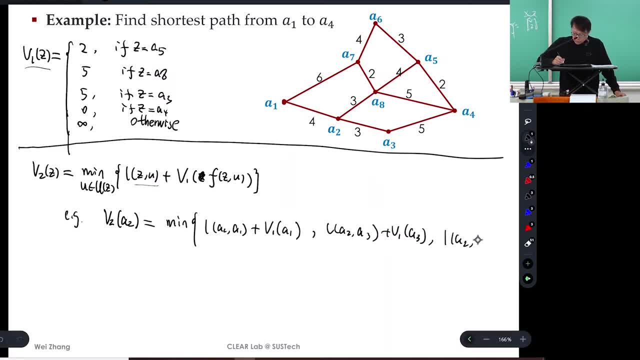 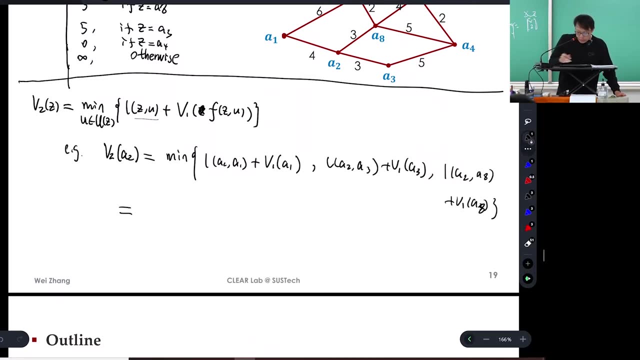 four. okay, I'll A2, A8 plus V1 of A8- A8. okay, let's just use v3, the other one. I don't think we need to. I mean this is fine. So what is it? This is a four plus. think of yourself as a computer. 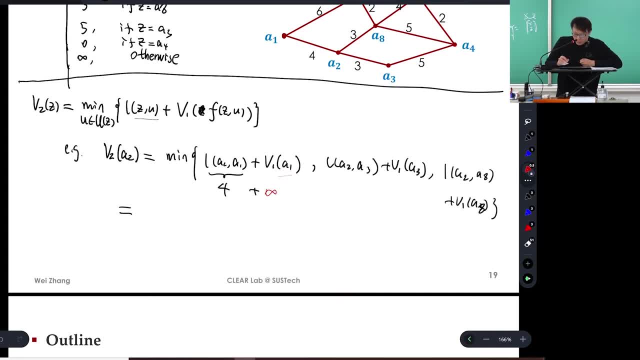 you don't know what RNAs, you have to compute them in order to know which one to take. This one is A3, A2, A3 is a three plus five. Now you have finite value, right. That's why you need to compute V1. 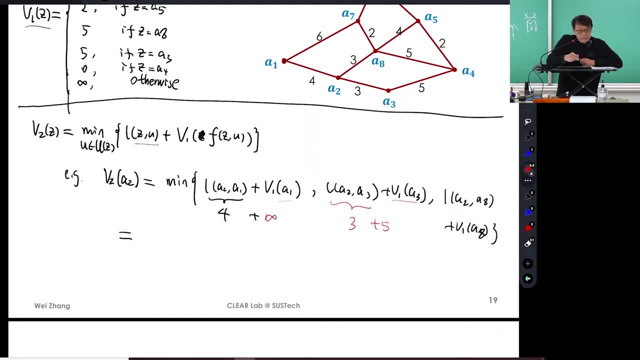 for all the possible Zs. You're going to use all of them. Well, not all of them at least. you don't know which one to use, so you have to compute all of them. And this guy is A3,, A8,, this is a three. 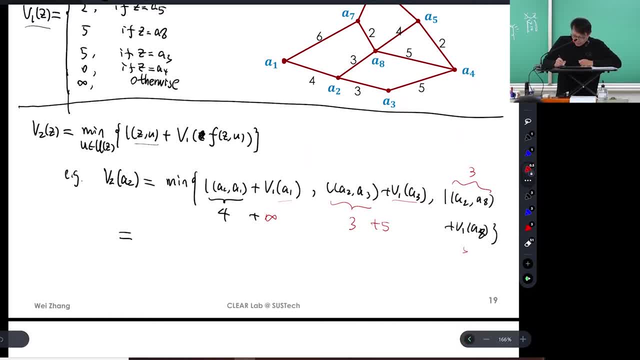 That number is really bad. Well, there are two of it. Those are five as well, so it's eight. So overall minimal is eight, The value of the function is eight and the mu two star A2 is which one? 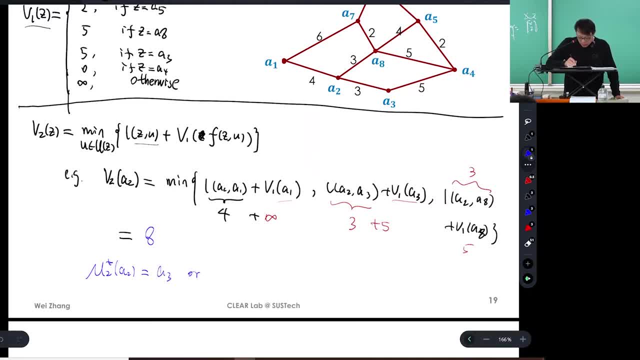 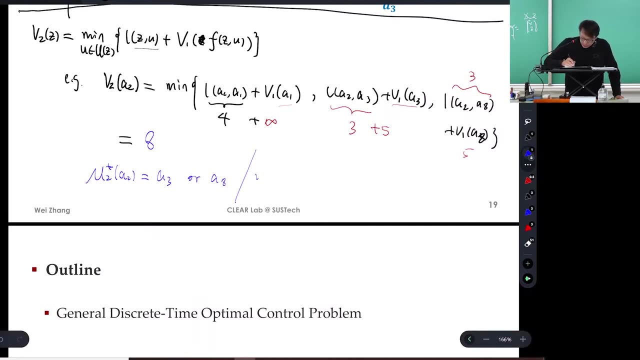 A3 or A8.. In this case they are the same, so I don't care, just pick one. So we will say that we need to huh. uh, we need to compute The computer. is that It reminds me to do a quiz? 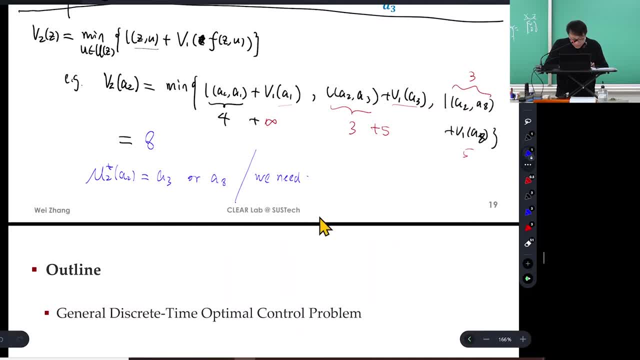 I can't do quiz anymore, so it's: Uh, I will say: you are right, We need to compute this for all the states V- Okay, not only this two, and then keep going like this. That's called a value region. 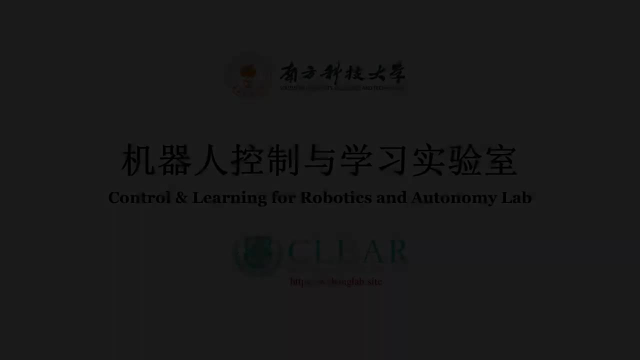 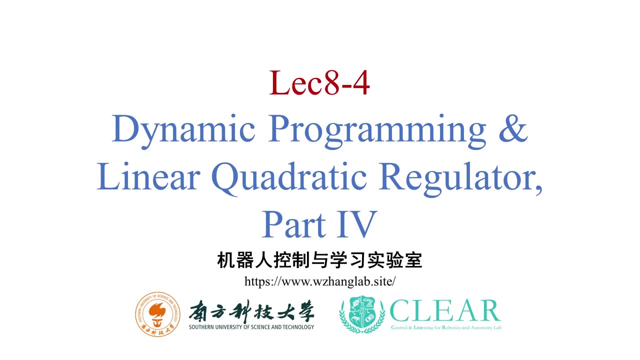 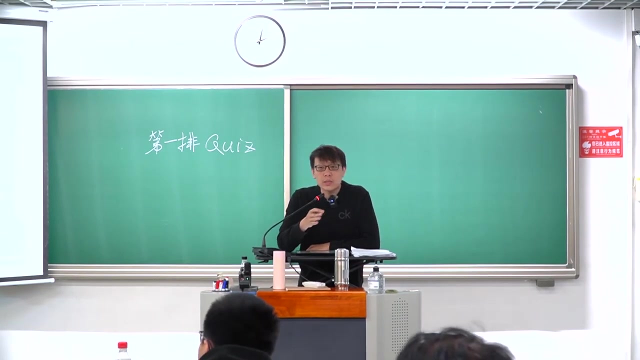 All right, that's. I think we've finished today's Uh, so I will de про guitar, but Chois they are already at a stop, so i would continue our discussion from last time about optimal control. as i mentioned before it, all the control problem can be viewed directly or indirectly as optimal control problem. 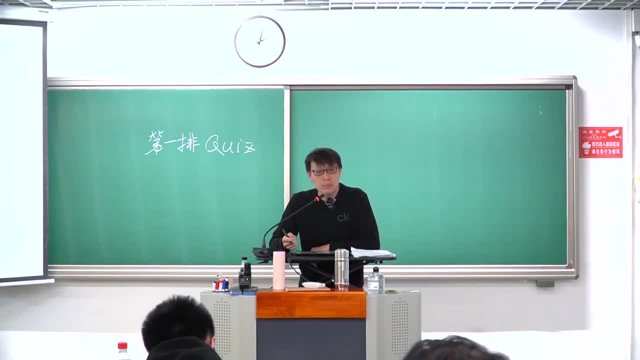 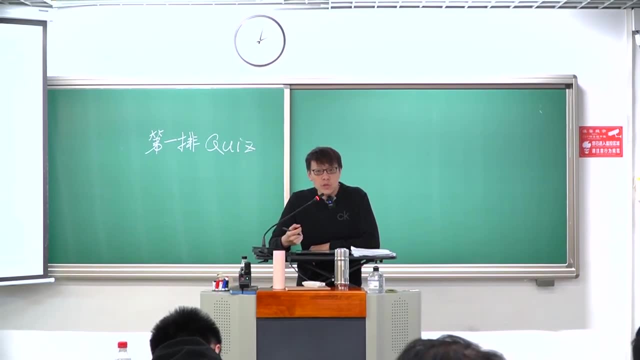 let me emphasize all the control problem. you can think of them as optimal control problem. so that's gave you a unified framework to think about all the decision or control problem in general. so that's why typically, optimal control is the most. uh, i like it the most, i don't know. 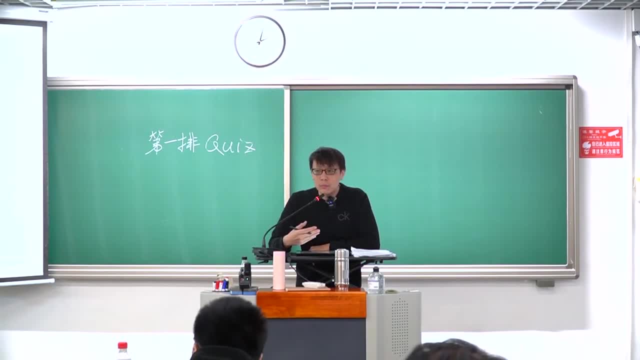 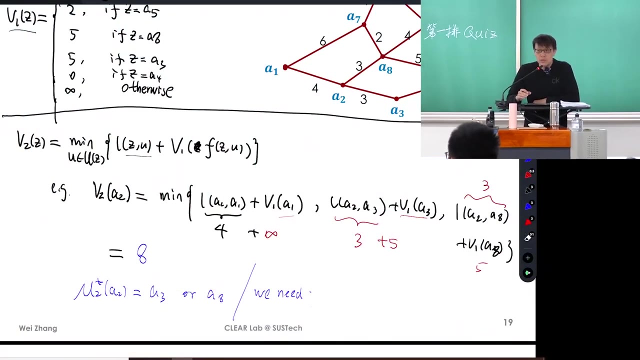 why there are other people and you will see any fancy robot from boston dynamics. all of them are based on optimal control and the model predictive control they are. they are related as well. okay, and the last two lectures we covered basic foundations for optimal control formulation and the dp dynamic programming. uh, let me briefly recall. uh, it's from last week, so 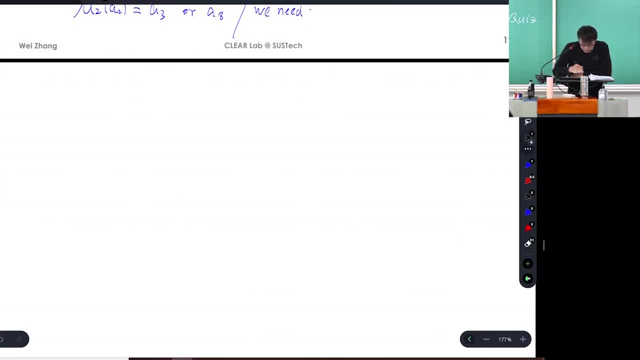 i have a lot of questions about the dp dynamic programming and the dp dynamic programming, uh, let me briefly recall: it's from last week, so i have it's from last week, so i have been awake. let's review or recall the formulation a little bit: optimal control. 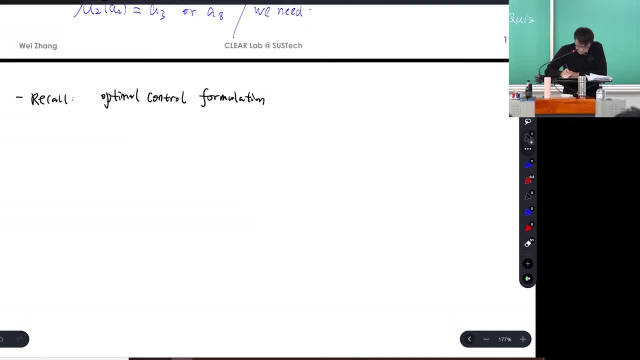 formulation. a lot of people like to see the diagram, like to see figure. okay, you have a system or plant. you want to design controllers to control it. that's all we're trying to do, okay. and the control means you need to send the input and you can measure the output. typically, 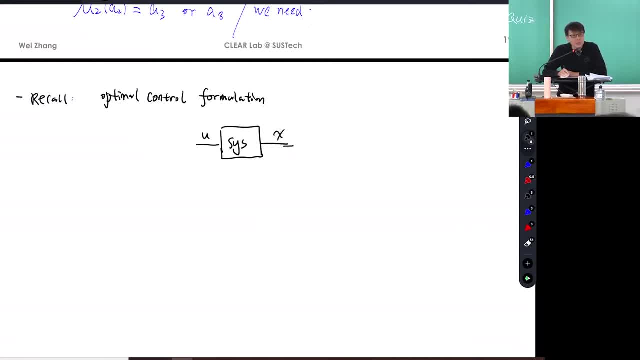 for optimum control. we assume we have the state. if you don't have state, you can do observer these control. we assume we have the state. if you don't have state, you can do observer these design to estimate state. okay, and that may be the output function that give you yk right and so. 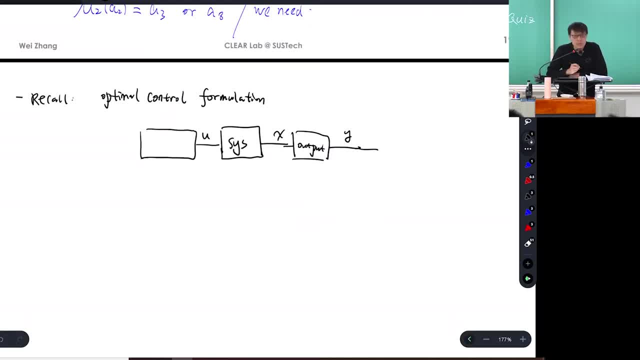 typically we will design a controller, oftentimes controller, and you may know, okay, there's a pid control, right? that's maybe all you know. we learned pole placement, right? maybe negative k times, x, something like that. okay, feedback going here. that means this part is called controller, okay. 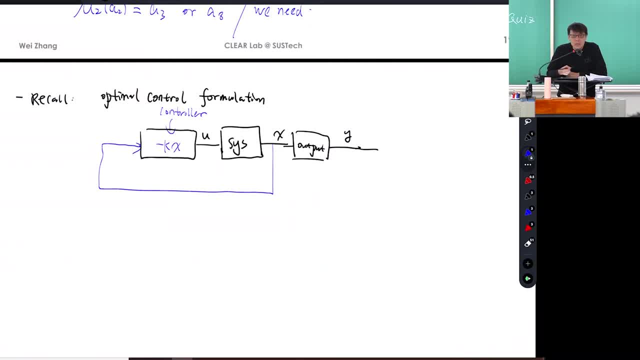 and at the beginning of this lecture i told you that a controller, if you think about mathematically, is nothing but a mapping from state to a control action. right, controller can be viewed as a function, however you want to define. you can. if you code, if you do coding right, your function could be 10 lines of code, or a thousand, or ten thousand. 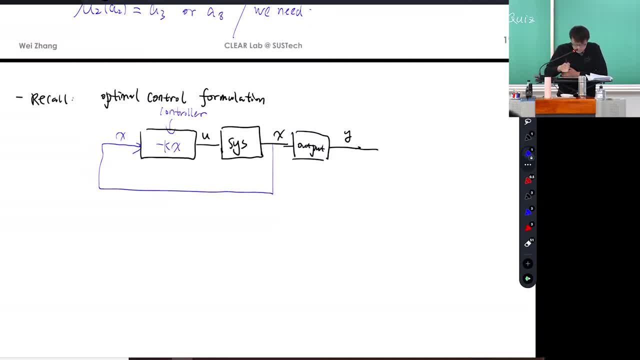 lines of code, depending how complicated that function is. okay, the optimal control. and this is our optimal controller, optimal controller. it's a controller, it's still a mapping from state to control input, but in determining the control input, this means the output of the controller is the control input to the plant. okay, if i want to determine this controller, uh, contraction. 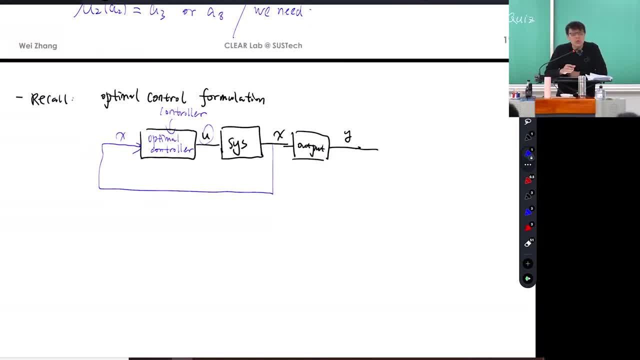 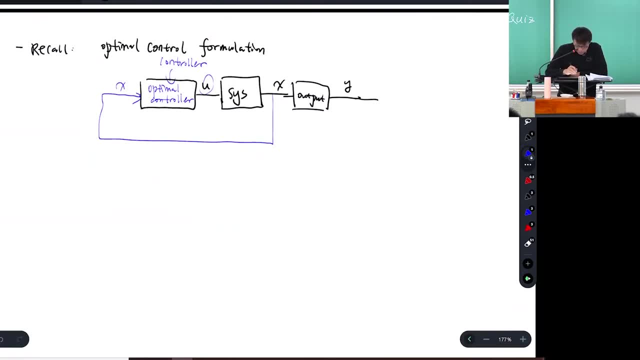 i want to solve a optimization problem or optimal control problem. in a way i want to minimize certain cost subject to project some constraints. if i want to have more details, let's say my system. this is my block system and in general i have too many colors. let me stick to black. in general i have a non-linear. 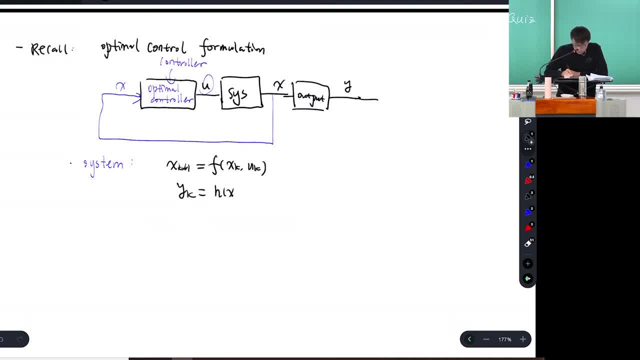 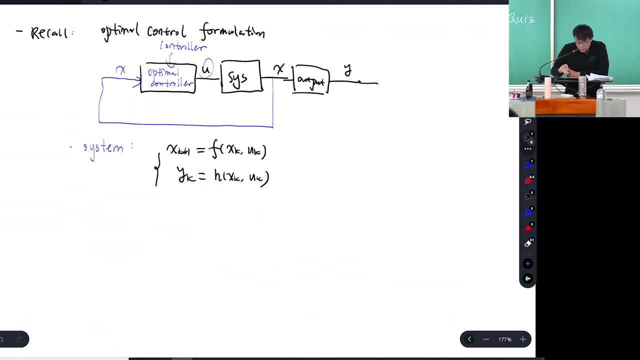 state update equation and may have an output equation like this: right, and we do not consider- uh, at least we do not consider- systematically about uncertainty. there's no noise like a common filter. this is just deterministic case. that's a system dynamics. okay, the optimal controller. part of this part, that's the optimal. 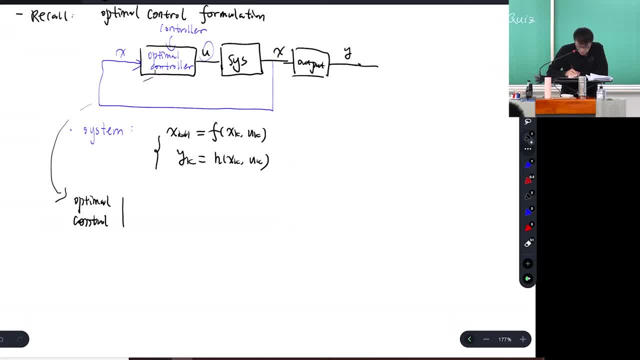 control part. the key idea is what is to use an optimal controller to control…. let's call it a TP is to encode your control objective. If you want to design a controller, you must have an objective. You may not know. your objective has a mathematical form. 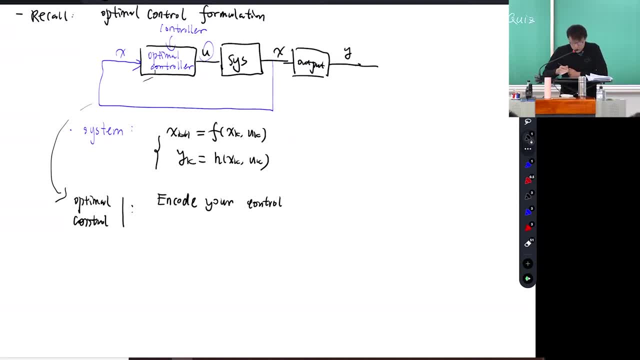 or can be written in a mathematical form, but you do have an objective form, a control objective. You want to encode your objective into a so-called cost function. In the learning community they like a reward In controller, they like cost. 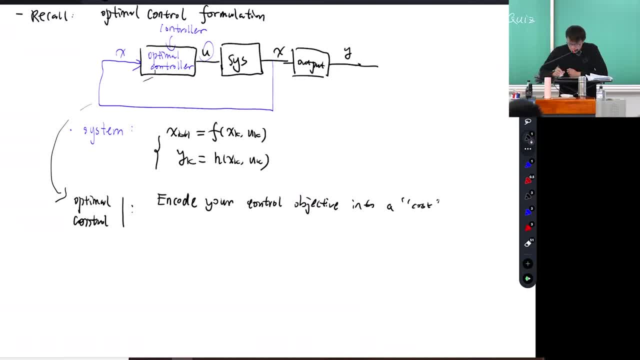 One is the negative of the other. So cost function in reinforcement learning. this will be reward. They want to maximize reward. We want to minimize cost. Then we find the optimal one Because we have a criteria. now we can determine what are the objectives. 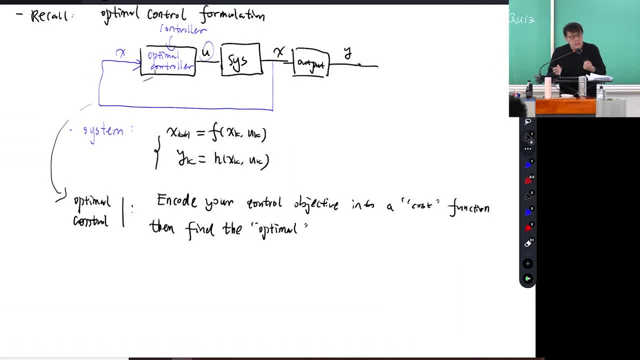 What are good, What are bad. In particular, we want to find the good among the good, which is the best or optimal one, So we want to have the optimal control u star. Typically, this will be u 0 star. u 1 star. 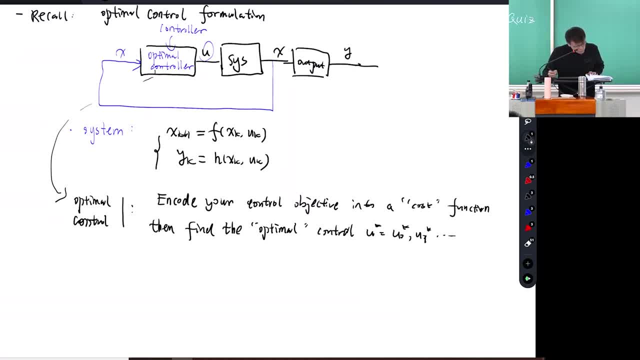 all the way to the future, depending on how long the control horizon is and to minimize the cost. OK, That's u 2 star. right. You translate your control design objective into a cost function. Then the design of a control becomes solving this cost. 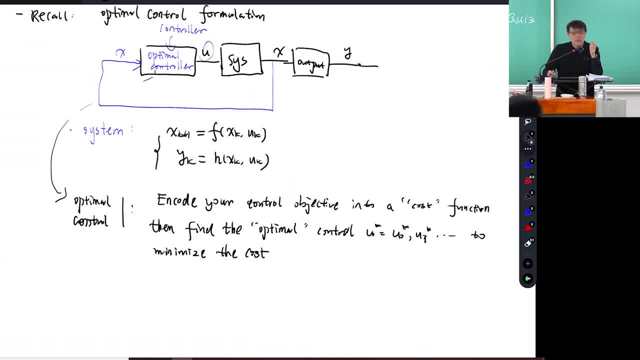 minimization problem. OK, Under what conditions? we can do this, Under no condition. All the control problems you have in mind can be formulated this way. You may not realize it, but I think that's very important. You have to know whatever you want. 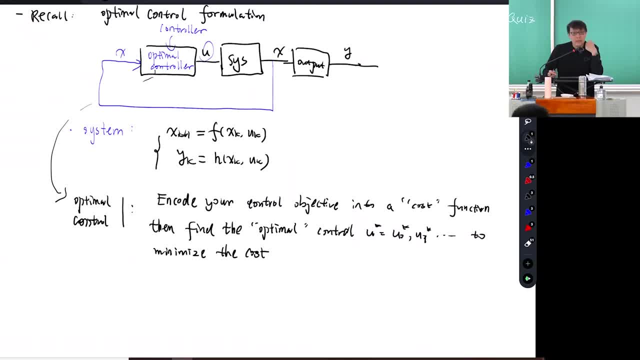 You say: I want my car to go from A to B without hitting the curb or obstacle. That can be formulated as optimal control problem. You minimize maybe the traveling time or fuel consumption and, subject to constraints that you stay away from the obstacle. 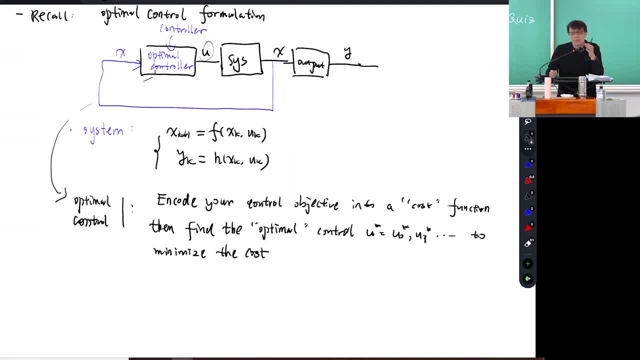 OK, As I mentioned before, if you don't believe this, you just come up with something you don't think You can write it down as a mathematical form, Then you send it to me, and I didn't receive an email yet. 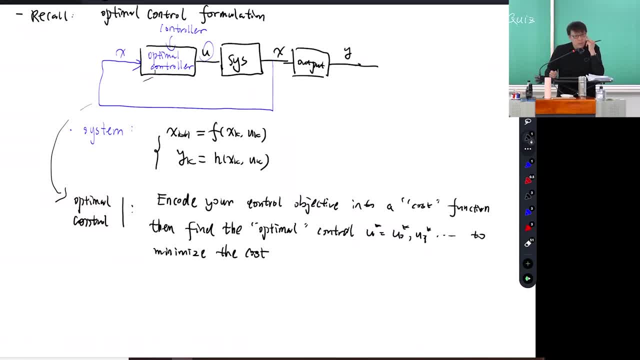 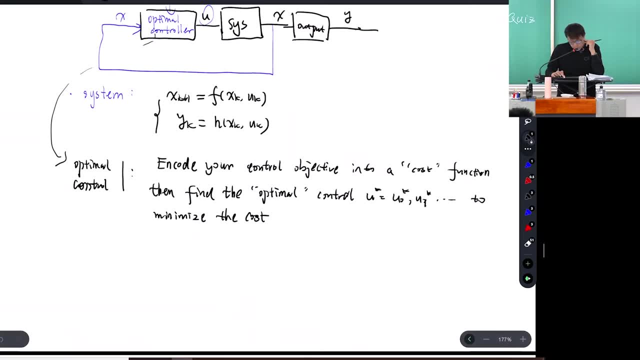 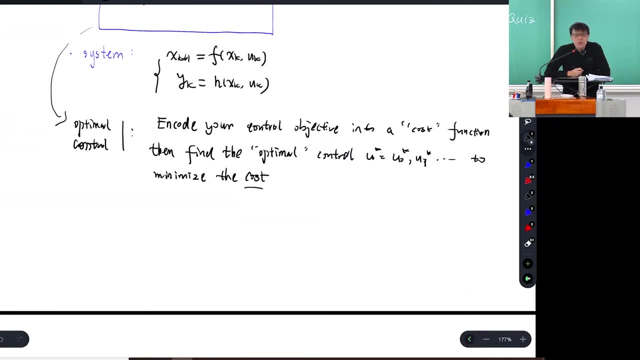 OK, So I can try to go through that with you. OK, So that's why it's so powerful. It's very important And typically that means Well, how do I represent my objectives through cost? And a general framework is the following: 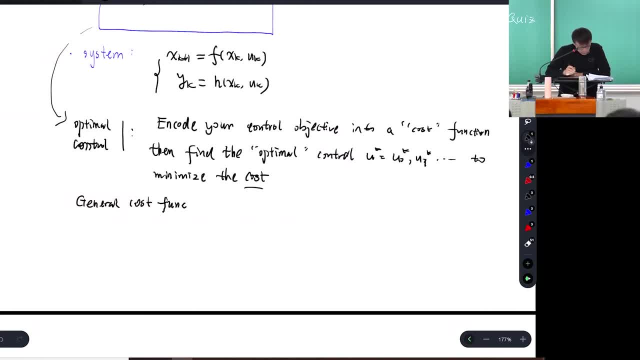 General cost function. structure cost function, which is J of terminal cost. J of cost Cost is function of the initial state and the control action or control sequence you want to take over a certain time. horizon: K from 0 to n minus 1.. 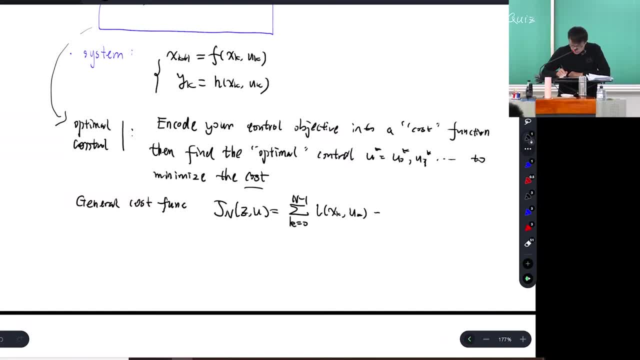 L, xk uk plus g of xn. This is called Terminal cost. Terminal cost- OK, That's the final cost, or terminal cost. When you are at the end of the control horizon. you have no life after that. 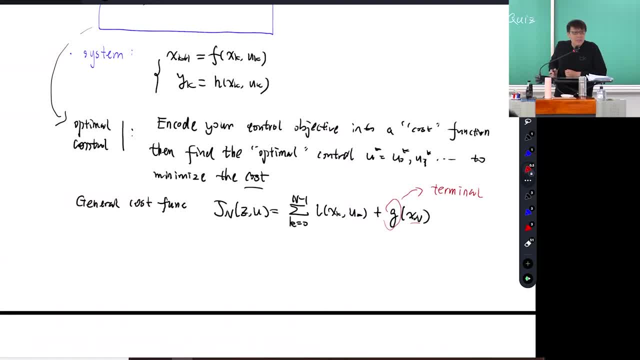 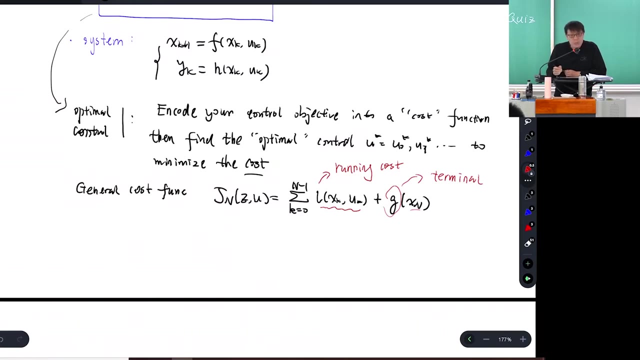 OK, And you evaluate how good or bad your life is at that state. OK, There's nothing you can do anymore. OK, And this IO is called Running cost. OK, So this, too, encodes all our objectives. 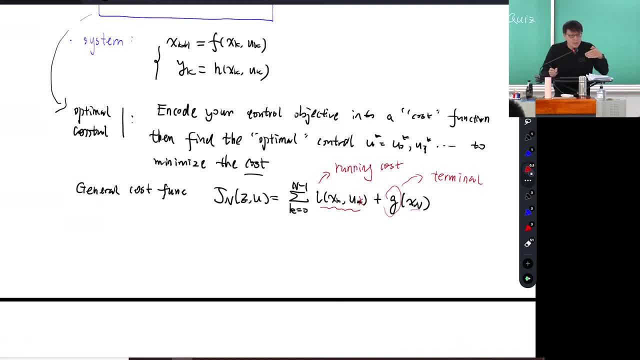 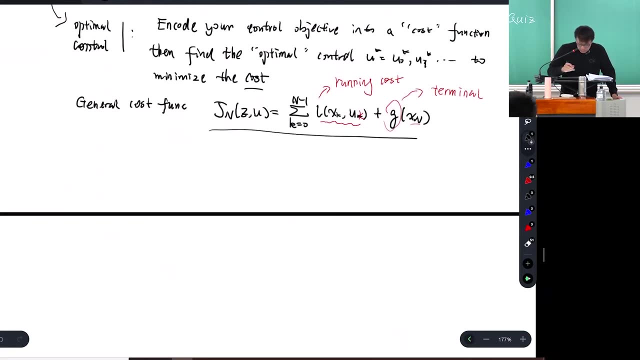 So for some control actions, you don't care about running cost, You don't care about each step where you are, You only care about you reach your final goal, which is your particular state in the state space. OK, So if I have this cost function, my optimum control problem. 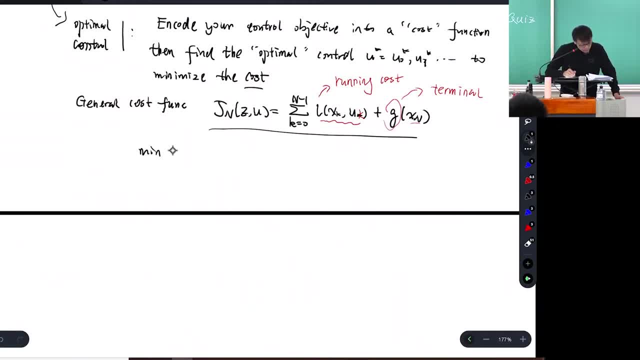 is what Try to minimize? what J of n, of z, of u Minimize over all the possible u. This, u is a sequence, It is class, Everything is a vector, Everything can be a sequence And this is a sequence. 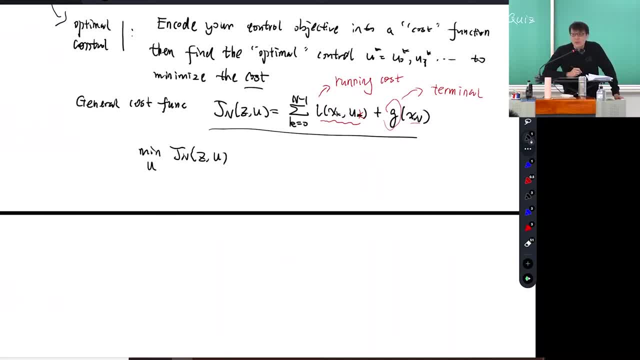 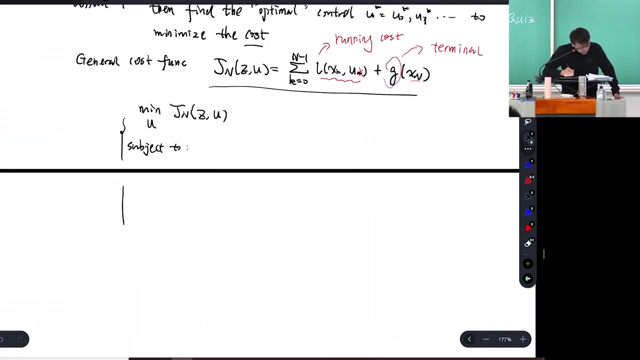 All right, And you are not free to select your control. Your control has to satisfy the so-called constraint. What kind of constraint you have subject to? Subject to, First of all, dynamics. Right, Let me Dynamics. So it's xk plus 1, equal to fxk uk. 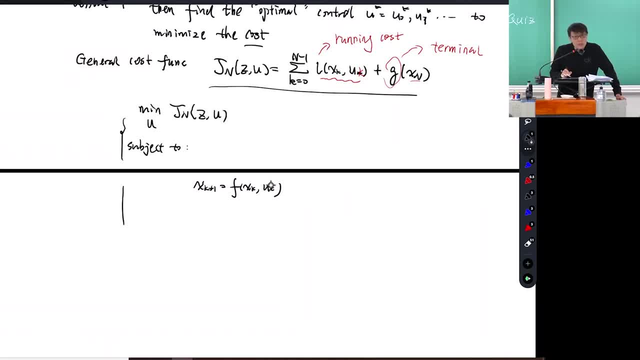 OK, Why we care about this? Because control actions determines, along with the initial state, determines the whole state trajectory. So if you determine your control, if you decide what the control is, then the entire control state trajectory is determined already And that will affect your cost. 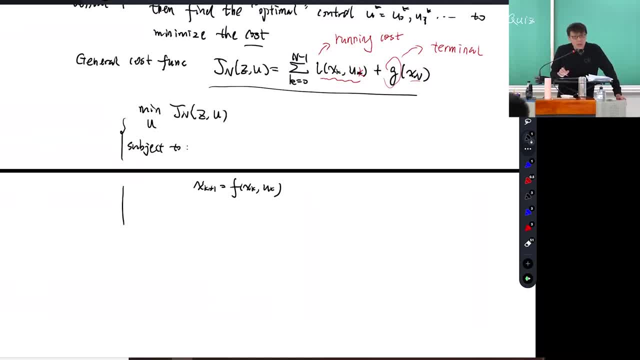 Because your cost function depends on the state as well as the control action. You can also have a control constraint, Like: the current cannot be too large, Your voltage cannot be too large, Things like that. As I mentioned, your control constraint can be state dependent. 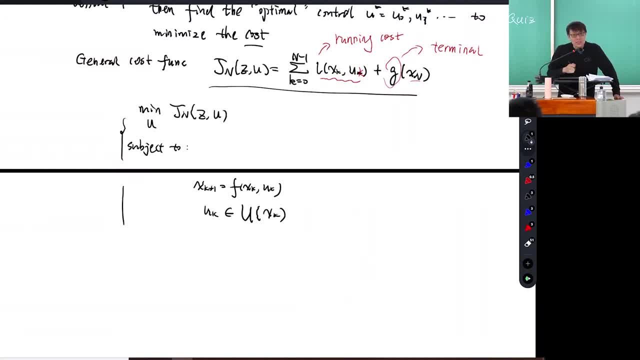 At the least particular time, the available control action you can take. That's the set. I think I gave the examples. If you're close to an obstacle, your available decisions are limited. Right, If tomorrow is the exam, today, your action choice is different. 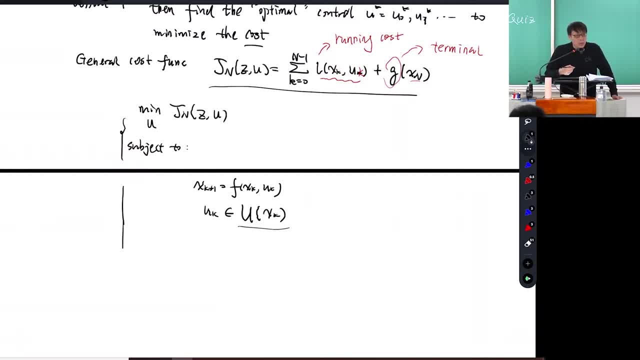 You can only memorize a few formulas without going through all the notes. So that's exactly what this means. And also xk also has some kind of a state constraint. For example, maybe temperature is your state. you hope your temperature will not be too large. 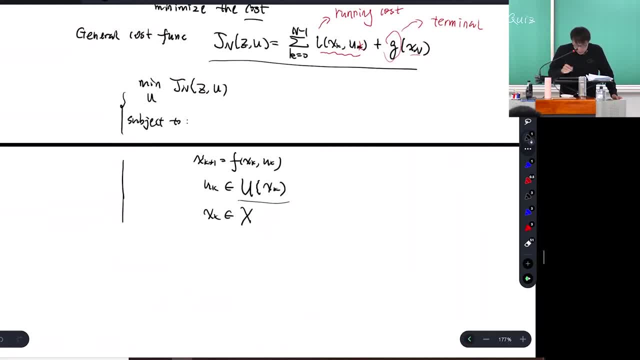 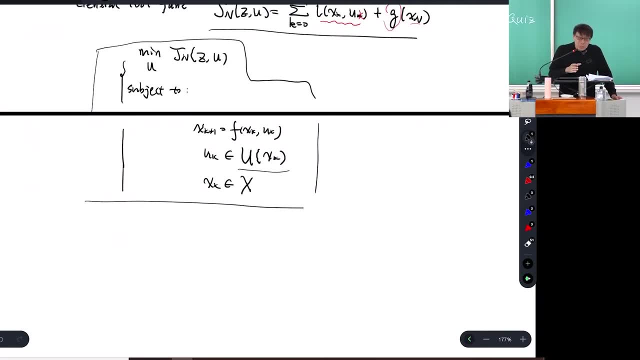 or your velocity cannot be too large, things like that. So that's overall. You can think about them as a high-dimensional optimization problem or we can view that as an optimal control problem. Optimal control problem can be viewed as an optimization problem of dynamic co-systems. 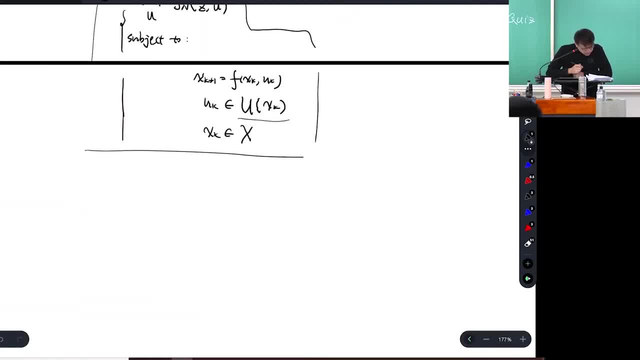 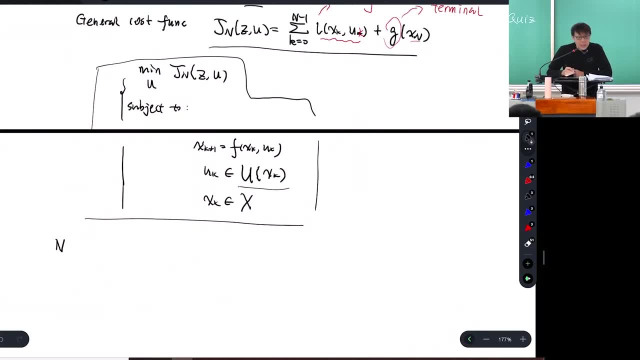 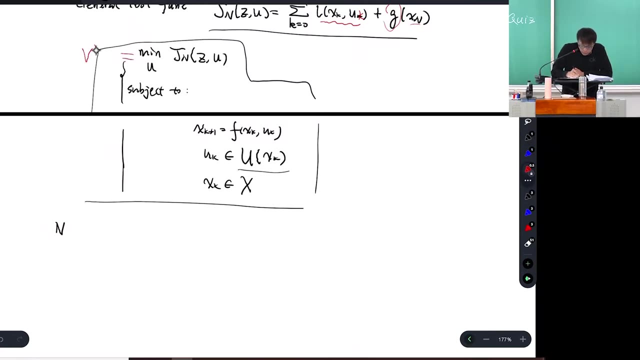 So to do this, we introduce the so-called what DP, dynamic programming, right? So you should know, the solution of this is called V, star or V of Z, and this is called a value function. What does this mean? The optimal cost. 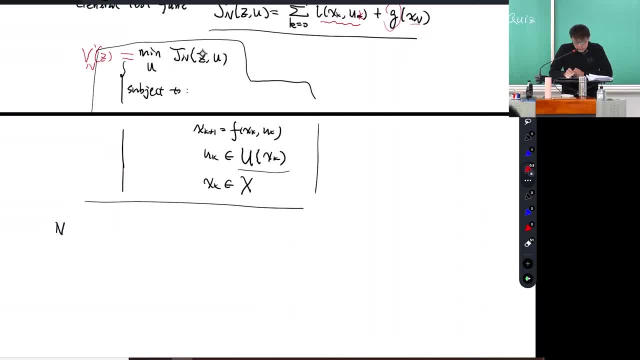 Because this is the value function. This cost function depends on the initial state and the control sequence. If you minimize over the control sequence, this guy will be chosen to be the minimum or the best one. You substitute the best one that becomes only a function of initial state and that is called optimal cost. 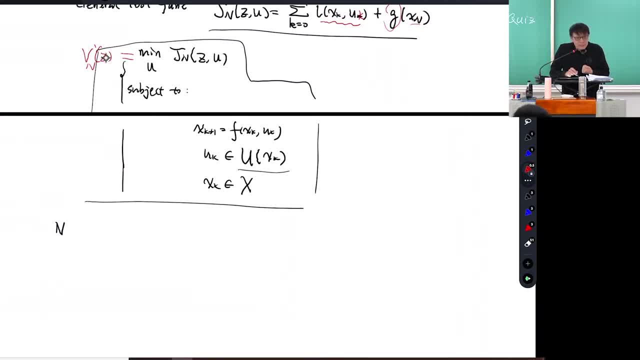 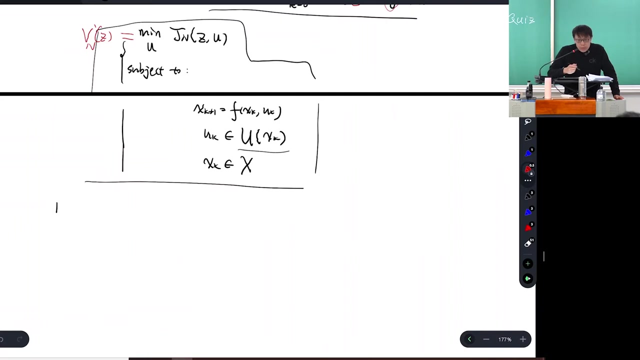 goal or value function. What is the meaning of it? If there's n horizon and my current state or initial state is Z, then the optimal cost cost, not the contraction, the optimal cost is this Vn of Z. We gave an example before In order to solve this n horizon problem. we can do better iteration. 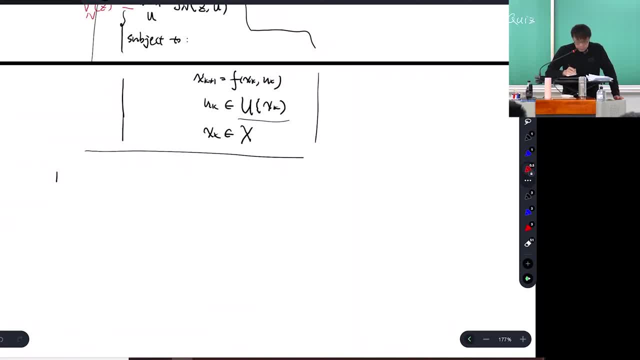 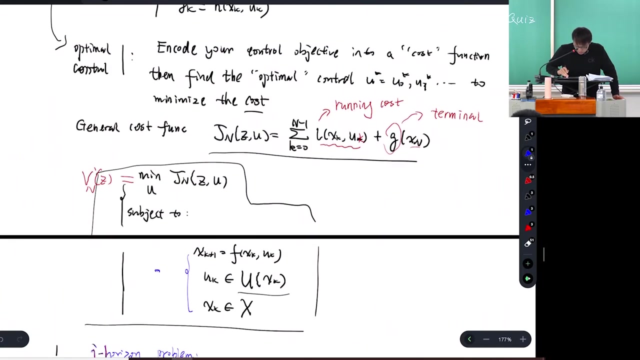 and the key is to determine what We start from. zero horizon, one horizon, two horizons. So in general we have, say, J horizon problem, that's called J horizon problem And I can call this part my equation. hold on, I can call this constraint equation C. okay, 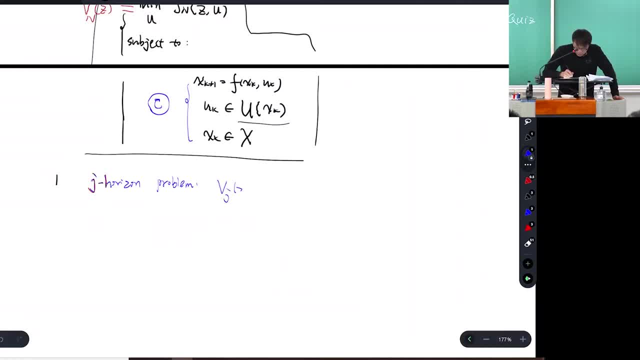 So I can define this as VJ of Z, equal to minimum, over U of JJ of Z. Also have U. In this case it's U. if I want to write more explicitly, that will be U zero up to U J minus 1.. Okay, The first action you take is U zero and then 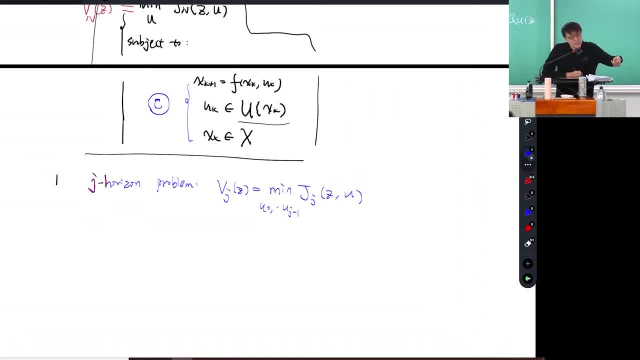 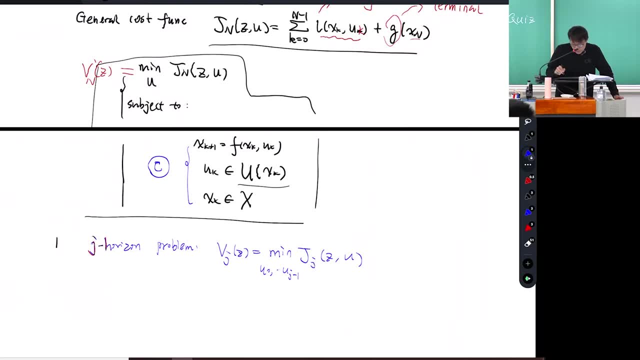 the last one you take is J minus 1, then you move to J. Okay, That's the cost function, If you just replace this capital N with this J. That's the cost function structure, And I don't want to write down everything. 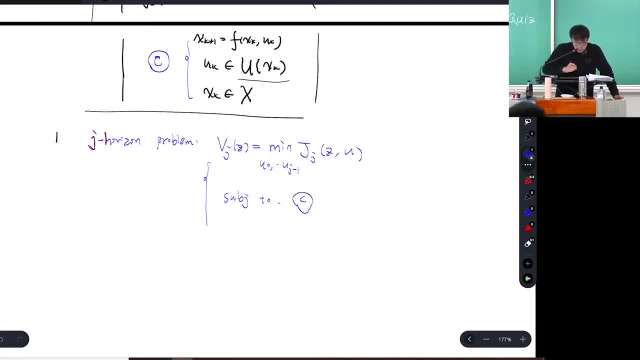 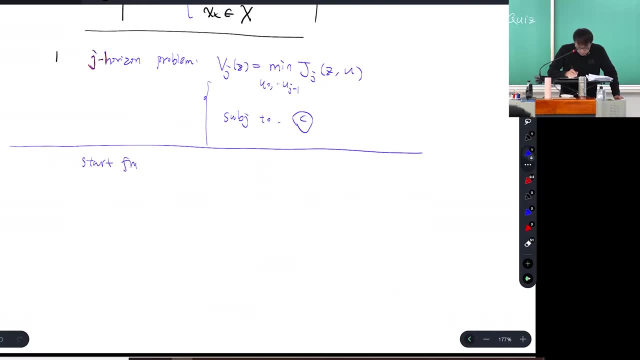 that's subject to what The constraint, Equation, constraint, the same, The same, same constraint is. So we can start from start, from J equal to zero- right, That's called the value iteration. And the V zero, of Z equal to. 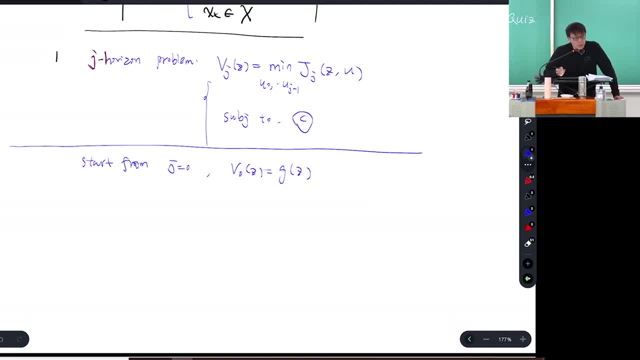 as we derived last time, that will be G of Z, the final terminal cost, Because you're already at terminal There's. you didn't give any choice. You just at the beginning is your end. The beginning of your life is the last day of your life. 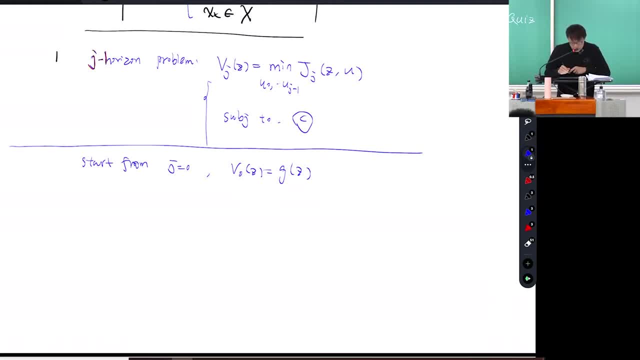 It's things like that. You have no contractions, all right. So that's the terminal cost. It will be your zero horizon optimal cost. okay, And like any induction, you just need to move from J to J plus one. 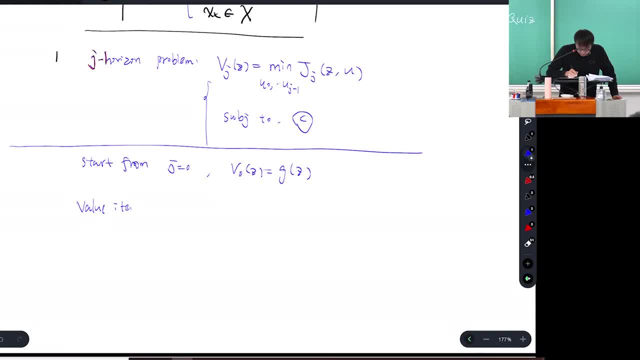 As we mentioned before, this is called the value iteration. Okay, So V, J plus one of Z is what is it? Minimize over all the possible control action you can take, at least state at current state. So U beyond this, U is one. 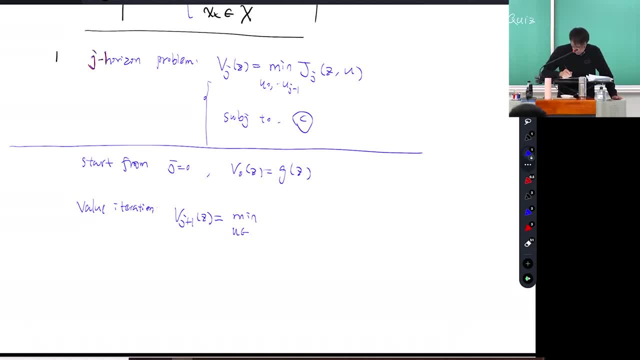 it's just one shot, one time. step U okay, Capital U of Z, That's at this particular state. you have this amount of choice. You can have two choice, three or infinite number choice And for each of these choice, 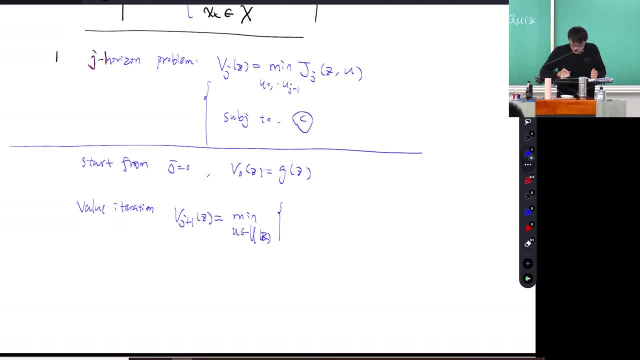 you want to pick the best one. How to evaluate the best? Of course you can do the running cost. Of course, if you apply this, if you apply this U and you're counting like Z, you have a immediate running cost at one step. 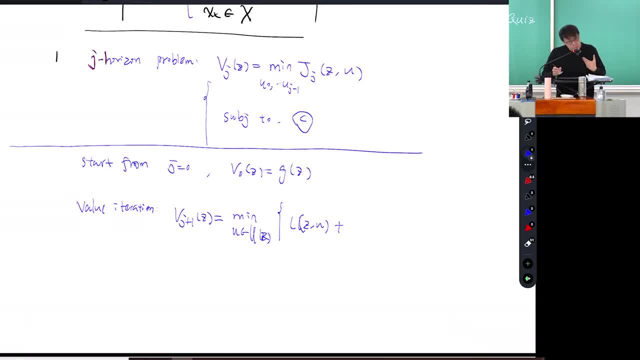 But at next step you will take the optimal one, starting from next state, So that will be V- J, because time horizon is shorter by one. You move one step further, which is F, Z of U. I think we explained this from different ways last week. 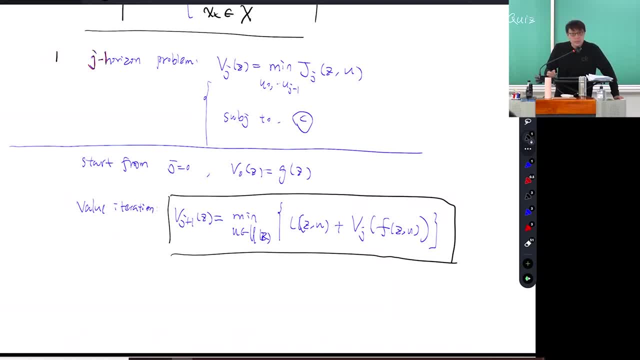 Any questions so far, This is called the value iteration. That's everything. There's different words describing this. This in the CS community, this is called the Bellman. I think they call it back word Propagation, things like that. okay. 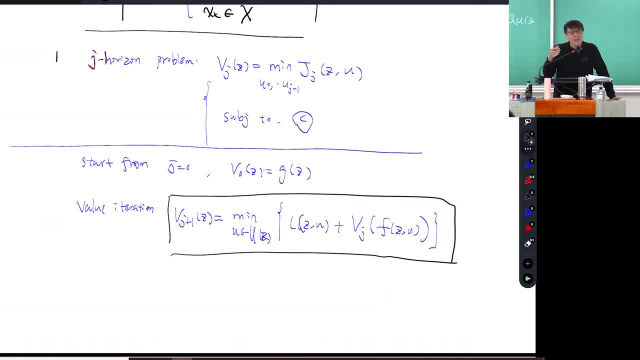 So what's? I think before I talked to a CS candidate, faculty candidate in the US, and they talk about this back word. I don't know what that means. So then I argue with him a little bit, then I find out this is different terminology. 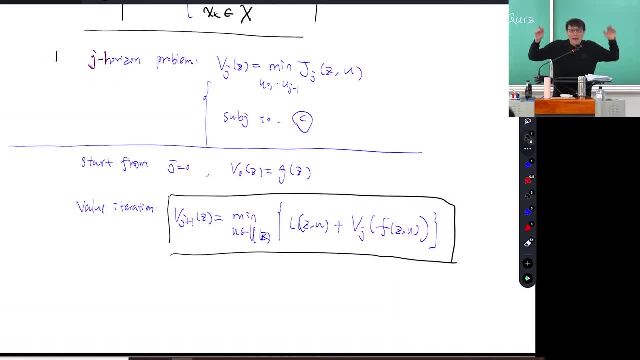 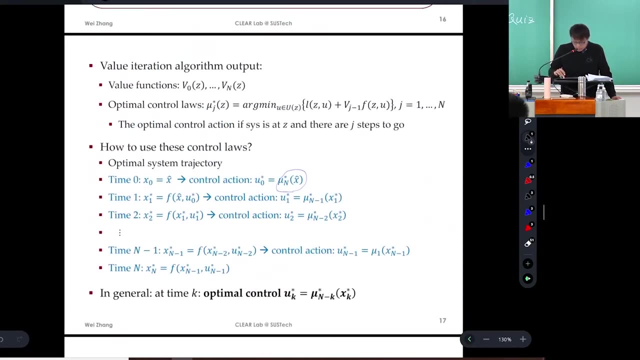 between different community, But in essence, the math is the same right? Math is the common language across different domains. I think that's okay, right? So I think last time we discussed this, This is how we derive it, right? 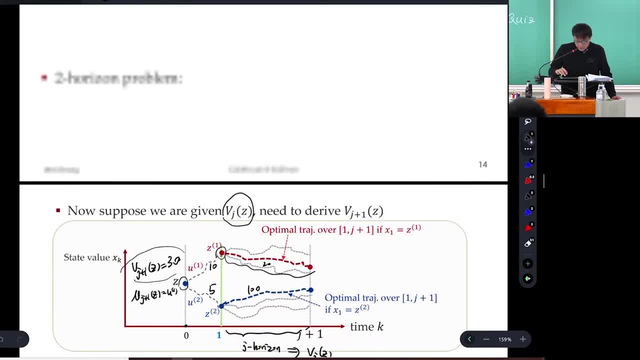 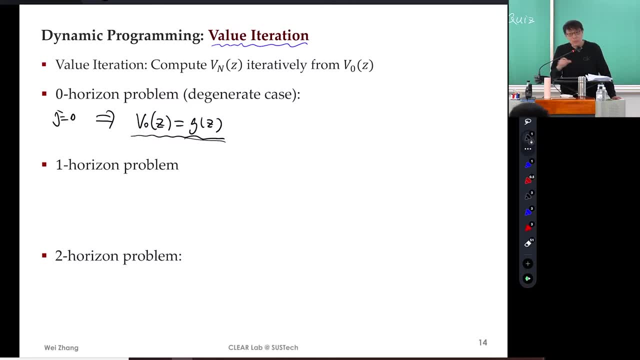 Through figure, And today I'm going to derive it a little bit with math, pure math. I don't think either. some people prefer this way, Some people prefer figure way, Some people just don't like proof anyway. So but I have to let you know that this can be. 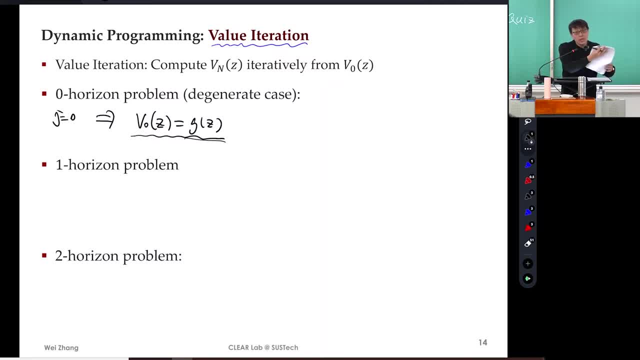 this is very common science. actually, It doesn't need to. you don't need any advanced math to understand this. The starting point is still the terminal cost. The zero horizontal optimal cost is this: And then we talk about one horizontal optimal control problem. 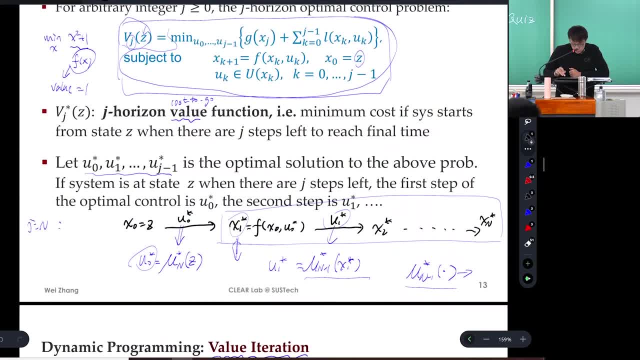 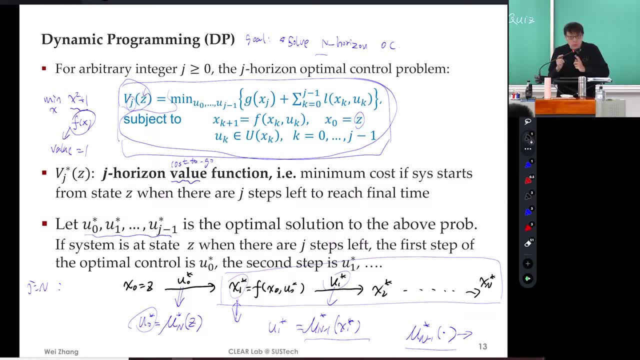 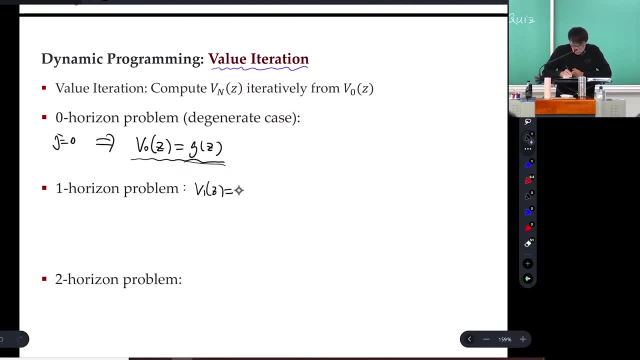 What is it? You just plug in J equal to one, now, right. Then you have an optimal control problem, right? You have one horizontal optimal control problem, And that optimal control problem is, I would say, V1 of Z should be minimized. 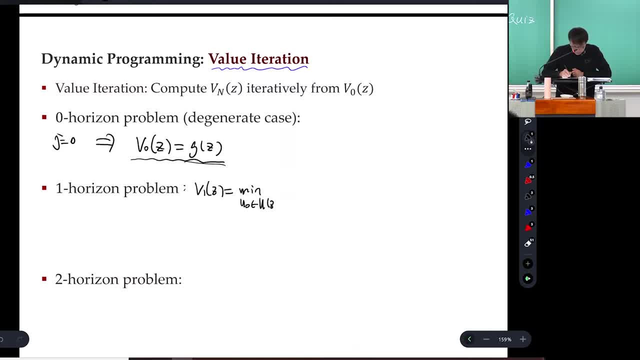 over my current U zero. Currently I'm at Z right. Available control is capital U of Z And it's one horizon. So the running do I have a running cost? So I have running cost X zero, U zero right. 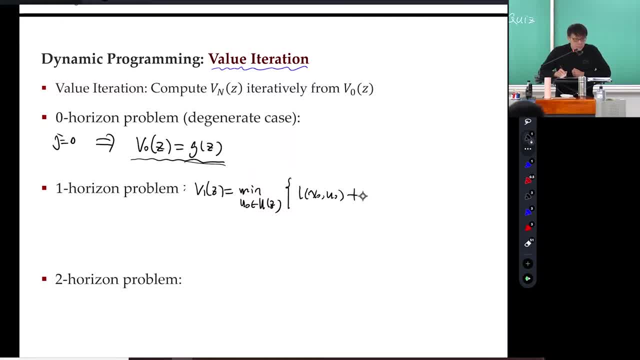 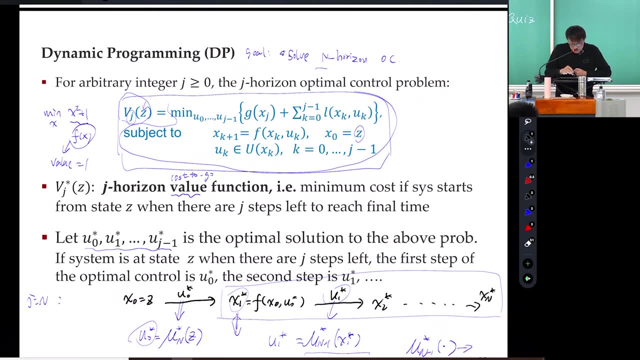 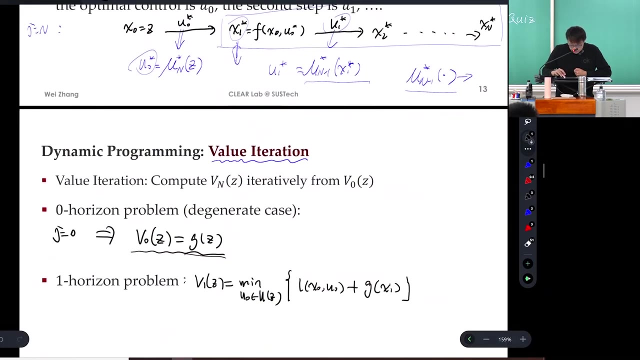 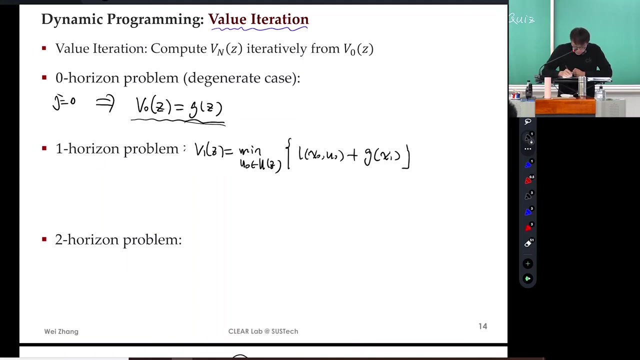 The next state. it's already terminal, So it would be G of X one. This is okay, right? This is the plain introduction. sorry of just somehow restate this. rewrite this formulation when J is equal to one. Okay, so if I want to write dynamics, that's fine. 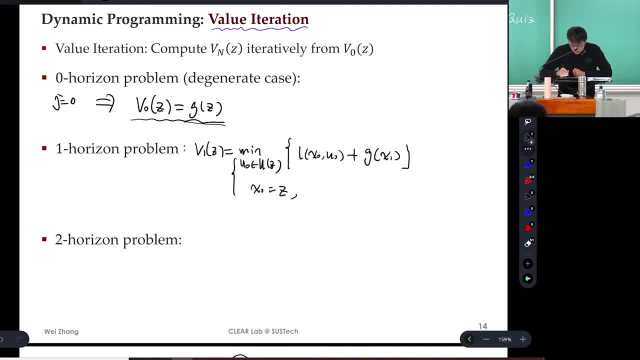 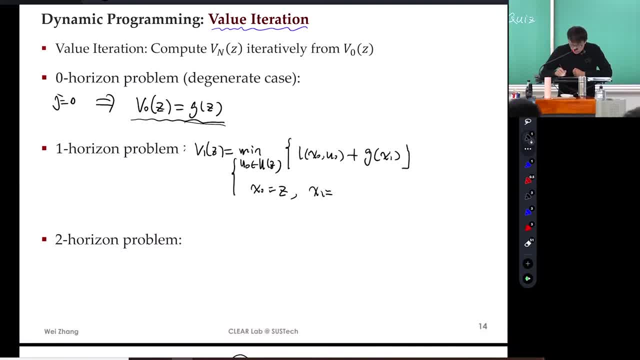 And X one relate to X zero and also relate to U, So that will be F X zero with Z times U zero. Okay, So that's then you have all the relations. So it's only a function of Z now, right. 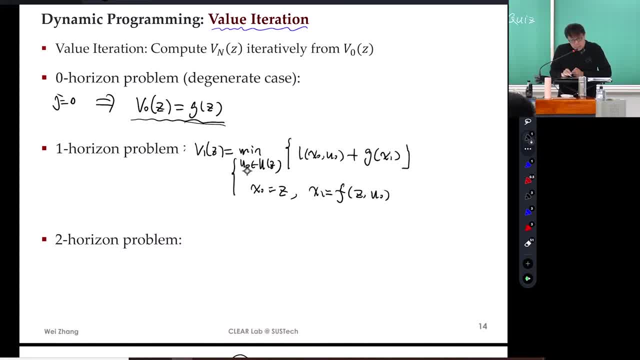 Because U zero is something we want to optimize over. If I fix U zero, then I know I know this guy is z. u0 is fixed, x, y is also fixed. Okay, so I can enumerate all the possible u0 I have. 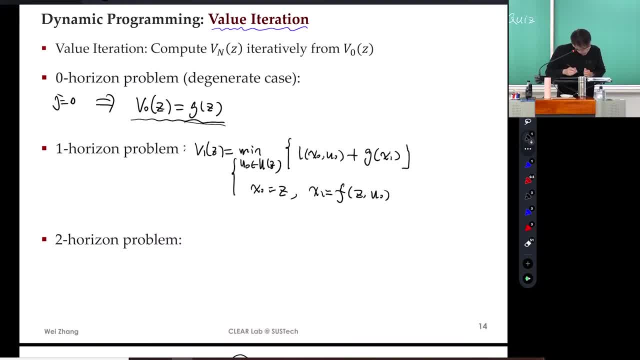 and find the best one. Okay, so this equal to you can immediately see, in this case that will be m. oh sorry, min over u0 belong to uz. This is l. Let me put it into general form. I know x0 is z, so I'm just like z u0,. 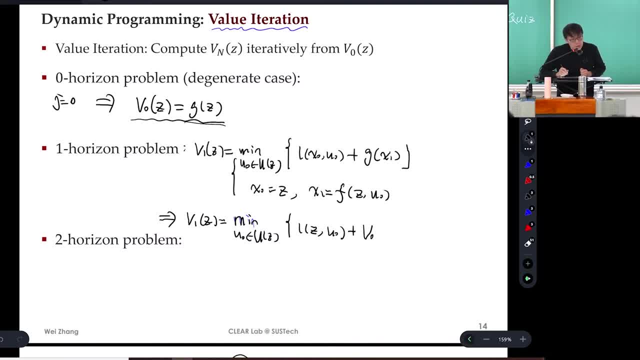 plus g is v0, right G function is u0.. I plug in x1,. x1 is the next location, which will be fg of u0.. I need to write down everything in terms of initial state and also the control input. 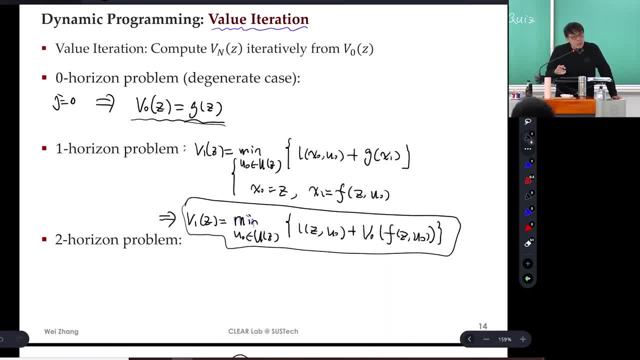 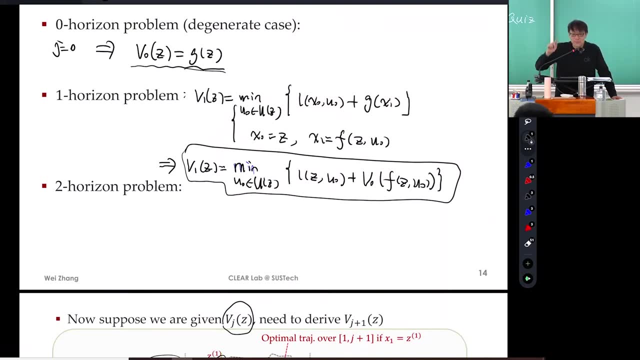 This is the value iteration, right? This is the value iteration. That's too simple. that's one step. Any questions, by the way? No questions. very simple, right? Let's look at two. Once you know how to move from one to two, then, 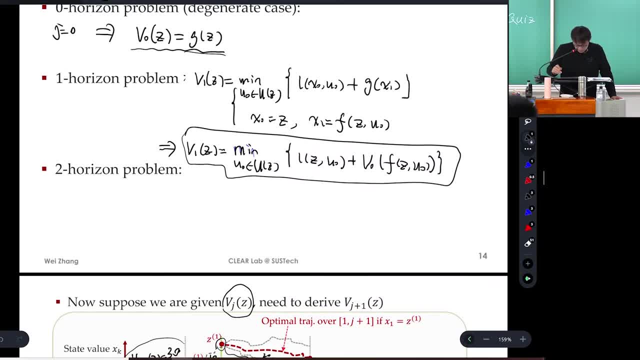 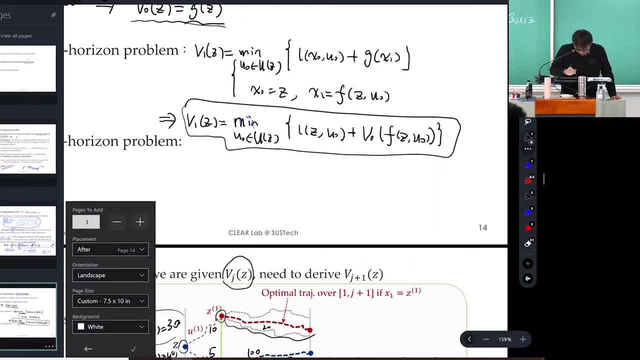 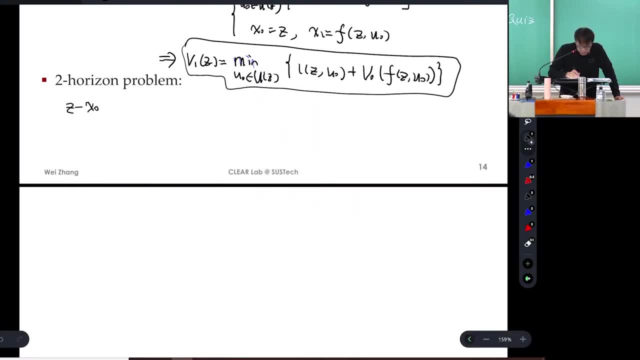 you can move from anywhere. That becomes a trivial problem. then I think I need more space. Let's see Two-horizontal problem. So first of all, I start from z, x0, right, Then I will be applying u g u. 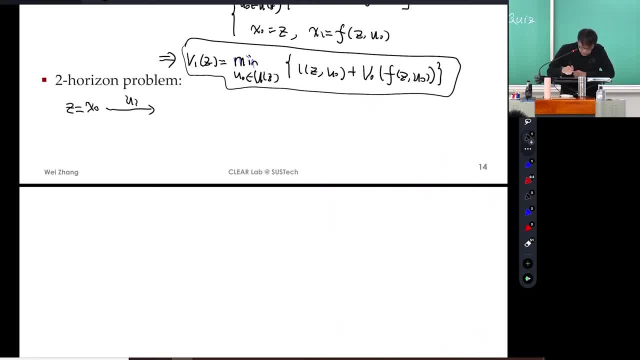 My pen has some problem, I will come. this is u0, I will go to x1.. Then I have u1, I will go to x2.. That's two-horizontal problem. How many control decision or control action I need to determine now? 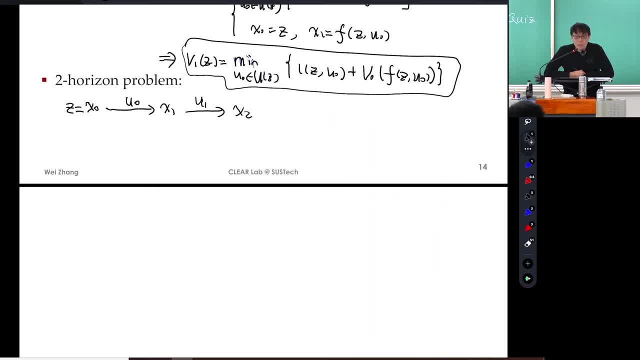 Two right, Two-horizontal. I have two control action I need to determine. One is u0, the other one is u1.. Okay, Depending on what I pick, my cost will be different. I want to minimize over my cost, okay. 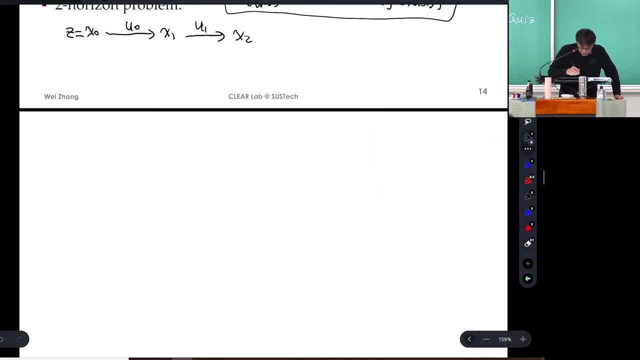 So let's write down everything So that will be two-horizontal optimal control problem. Minimize over u0 and u1.. Okay, if I write more carefully the available control action I can take: u0, belong to capital U, this control constraint. 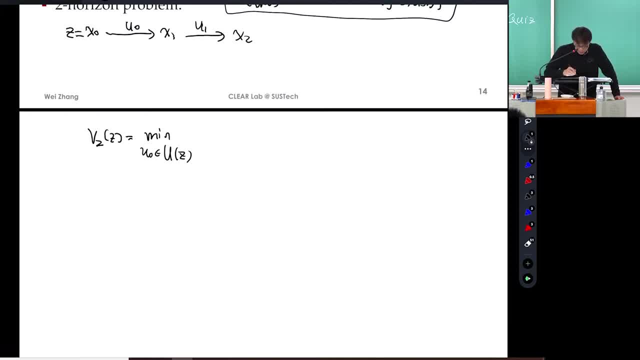 But depending on initial state in general. okay, But u1 depends on what X1, okay, So this X1 depends on u0, you see that? So this is more like complicated now. all right, I need to pick among them what. 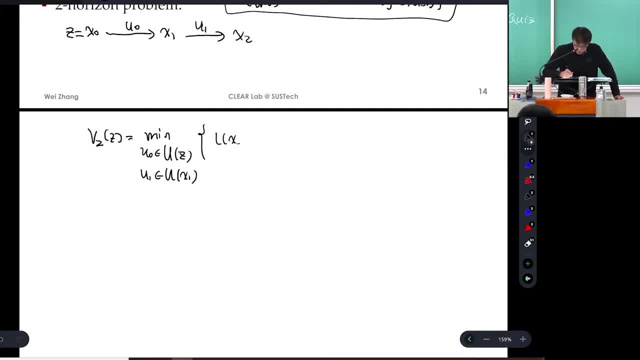 Running cost first. So I'll x0, u0,, plus I'll x1, u1.. Then I have terminal cost x2.. That's the most general or most direct way of writing the two-horizontal optimal control problem. 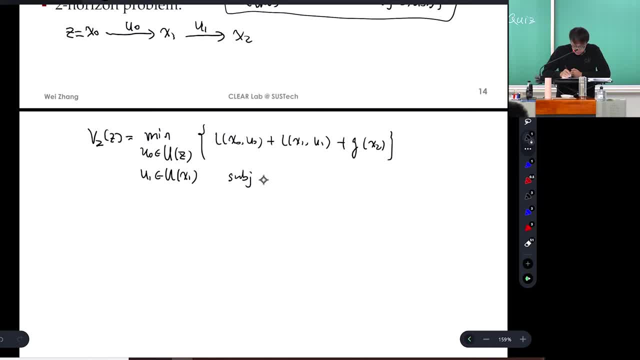 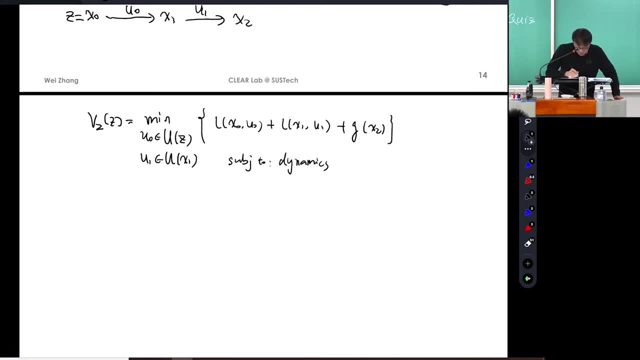 Of course, subject to constraints- right. Subject to constraints- dynamics. let's say I wouldn't want to write them down. A key is that let's write this down. Let's write this slightly differently: Min over u0 belong to u of z. 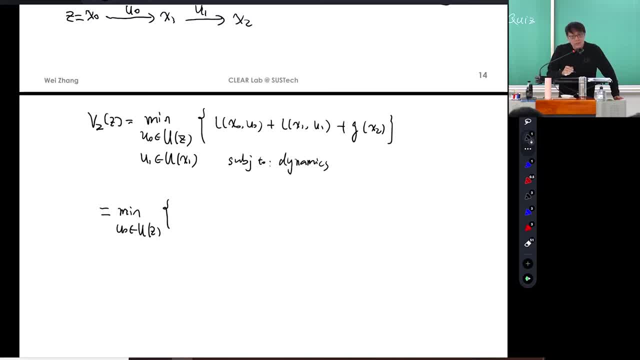 U1 is a causal system, right? Your tomorrow's action would not. so your today's action doesn't affect your yesterday's dynamics. It's like that You see time moving forward. Okay, so then u1 doesn't affect this. 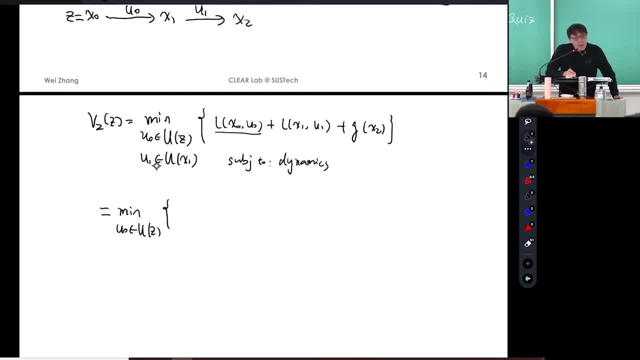 So the x0 and the u0,- this cost does not depend on u1, right, So I can move this inside. X0, u0, and plus min over u1 belong to ux1, okay, And these two terms depend on. 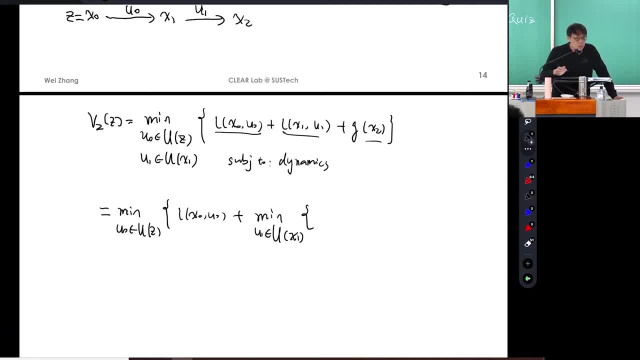 well, depends on both u0 and u1, okay, So that's x. I will say x, lx1, u1 plus g of x2.. If I substitute dynamics, then that will be f, Z or x1, no. 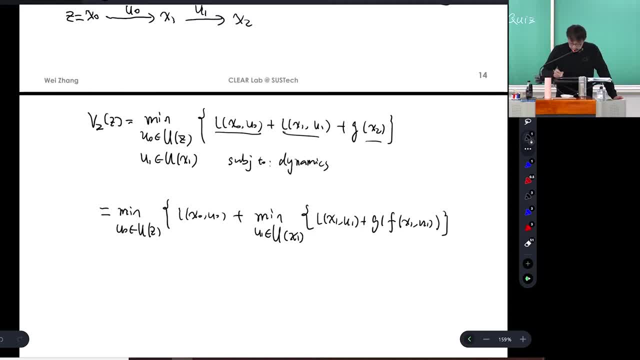 X1- u1, okay. Do you see what I mean? Now, if you have, let's say, minimize x and y, you have x squared plus- oh, x1, u1 plus g of x2, okay, Do you see what I mean? Now, if you have, let's say, minimize x and y, you have x squared plus g of x2, okay. 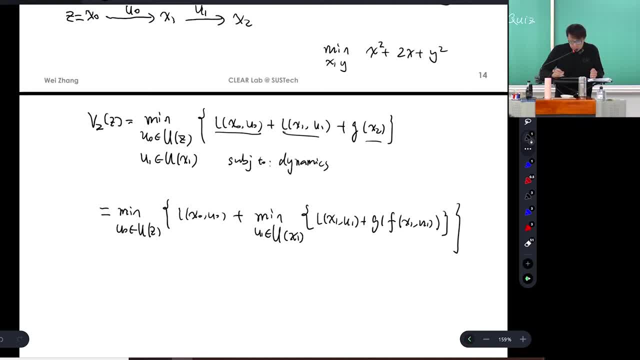 Do you see what I mean? Now, if you have, let's say, minimize x and y, you have x squared plus g of x2, okay. Do you see what I mean? Now, if you have, let's say, minimize x and y, you have x squared plus g of x2, okay. 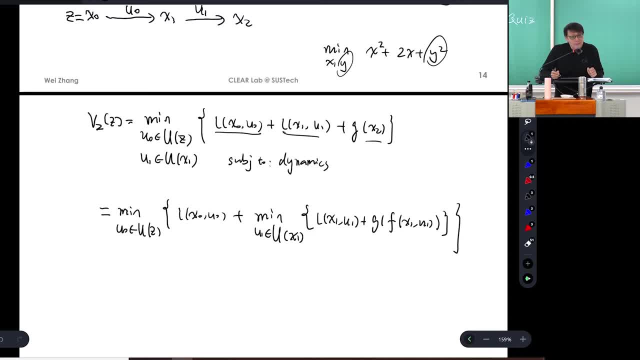 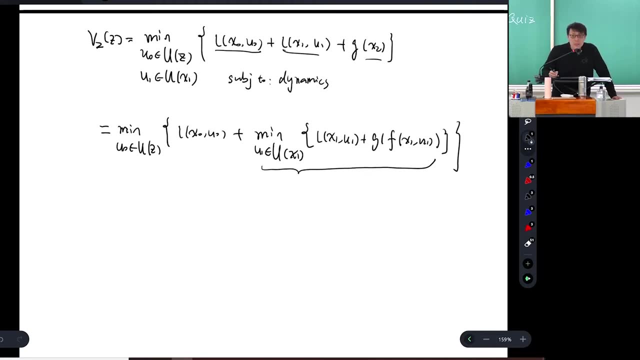 You can do things that this term only depends on this. You can maybe this times x is fine, You can separate them, all right. That's essentially what this is. So this term depend on what Depend on both u0 and u1 and z. 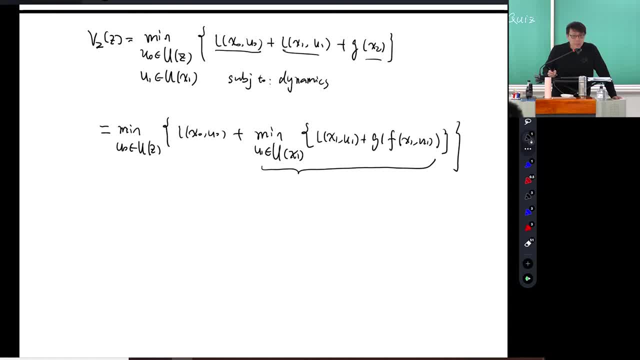 Depend on both u0 and u1 and z. That means x1, or x0.. That means x1, or x0.. Because it depends on x1 and also depends on u1.. x1 depends on x0 and u0. 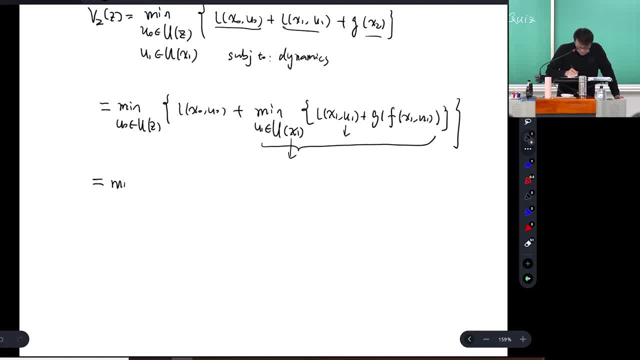 Okay, So that will become u0. belongs to u of z, And now I'm going to change right, Because x0 is z, right, I will say z, u0.. So, plus, I'm going to tell you that this one is nothing but this guy. 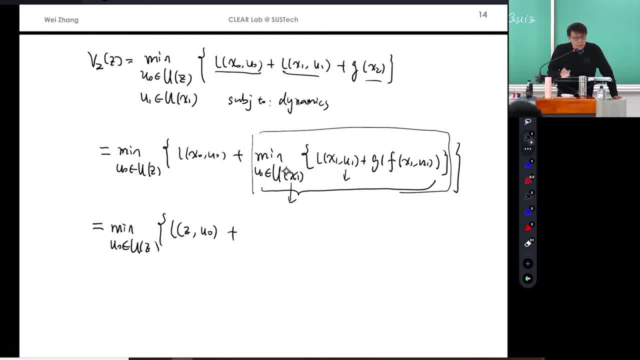 Okay, This depends on x1, right? If you parameterize this problem with x1, it's nothing, but this is what v1 of x1.. Okay, If, let's say, if you substitute this z with x1. 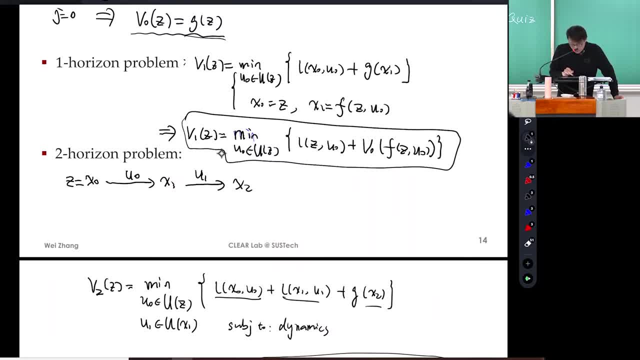 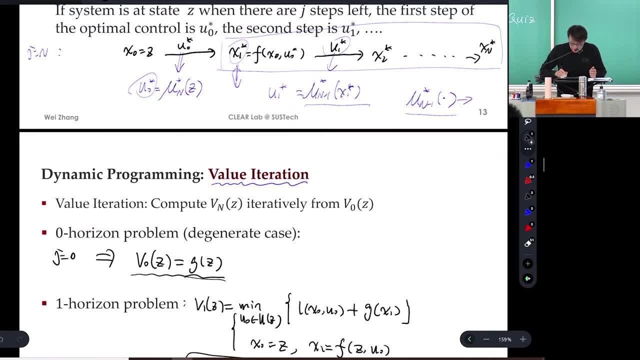 Okay, If you substitute this z with x1, then everything is the same. Of course, this u0 is a dummy variable, Right? It's like if I so minimize over x, x squared plus e to the x, Then I say this one is minimized over z, z squared plus e to the z. 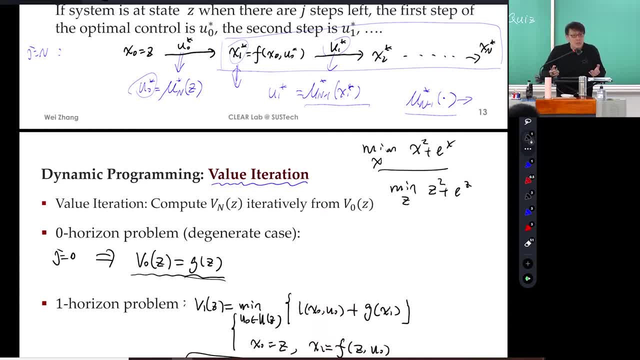 A change variable right. The function doesn't change, It's just a dummy variable. Is this two optimization problems the same, Right? Are these two optimization problems the same? Exactly the same. I can pick whatever q, alpha, beta, whatever I want is dummy variable right. 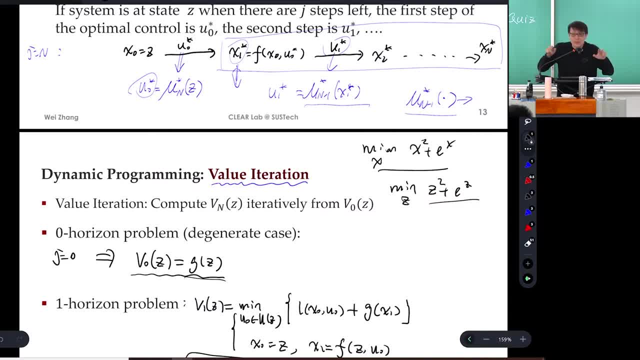 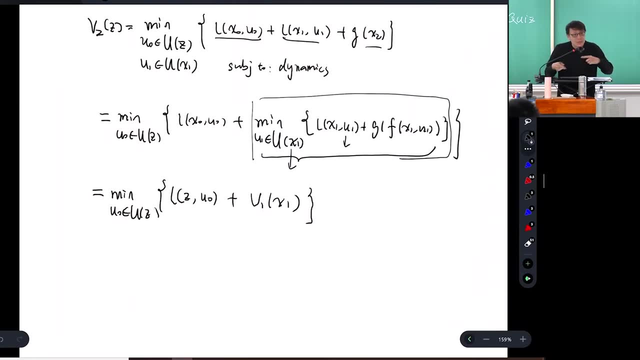 It's a function, The form or the structure of the function. It's the key, Instead of the variable I pick. I like z, you may like other variable, That doesn't matter. Okay, So if you change with a little bit change of variables, you find out this is exactly this. 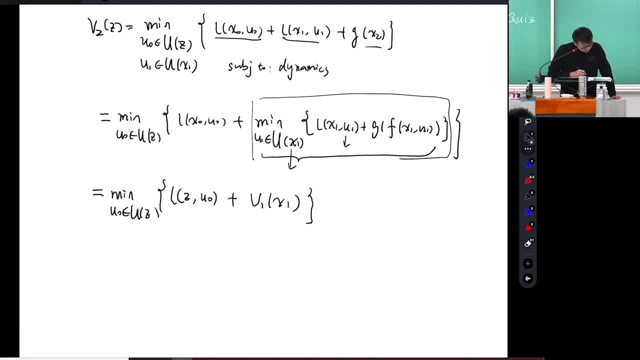 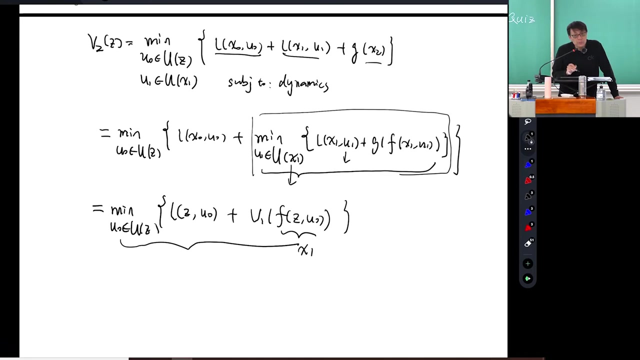 Right, So that's also value iteration. Okay, If I write it down like this, that will be x1.. I know it's fz of u0.. Right, This is x1. So it's the same. So I have, from v1 to v2, follow this value iteration formula. 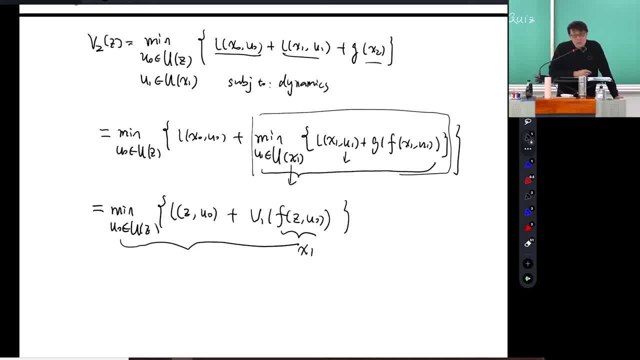 This is a pure algebraic manipulation. Sometimes it's you know everything makes sense but you don't have intuitive way of understanding things. But I want to make sure you convince you that, both intuitively or algebraically, these values, it's not hard. 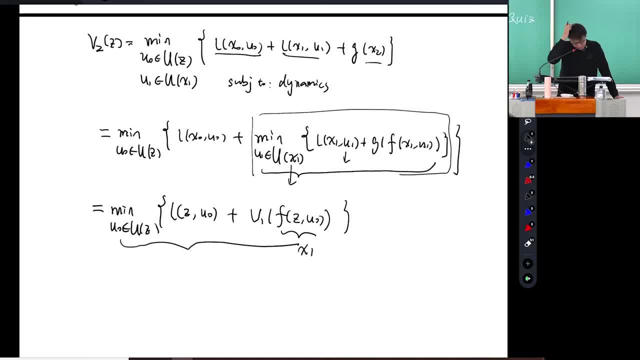 You just need to know what's going on. Any questions? No, I think I have complete derivation of value iteration for you and it works for the value. iteration works for all dynamical systems. Did I assume f is linear Or anything? I don't impose any conditions. 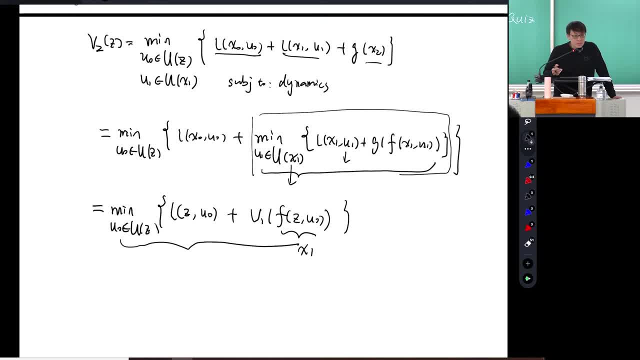 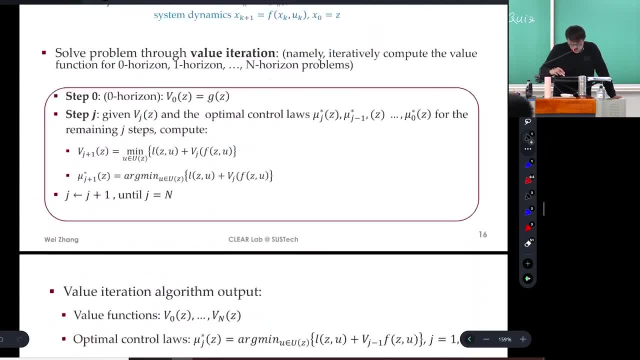 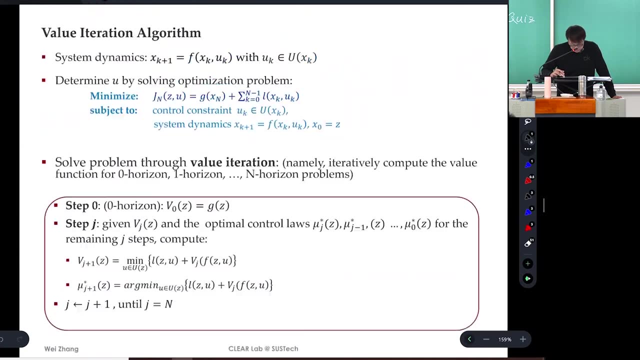 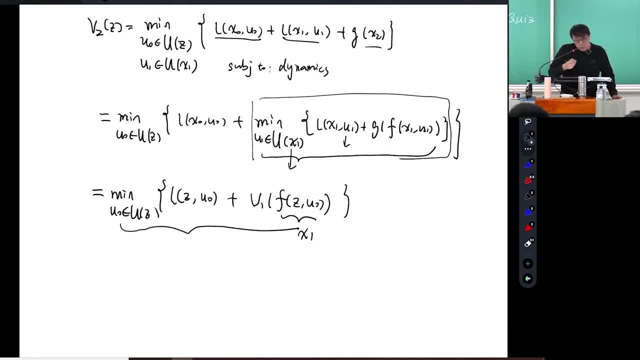 So you do the minimization, you have a cost function, but I typically want to know the minimizer, and we call this minimizer. This guy is called mu one star. mu one star of z equal to arg min u of this l z of. 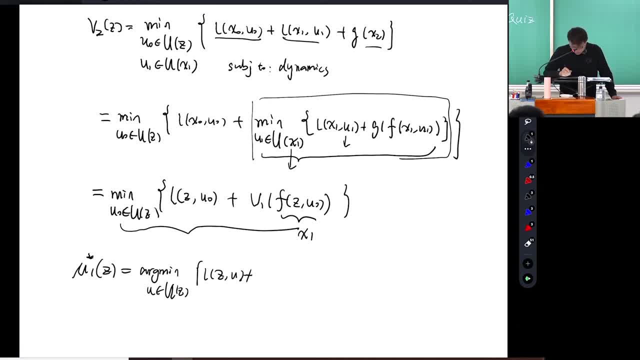 u, u, zero and u are the same dummy variable. okay, So plus v, one of f, z, of u. We call this the optimal action, We call the mu, And the action depends on the state z, So it's called a control law. 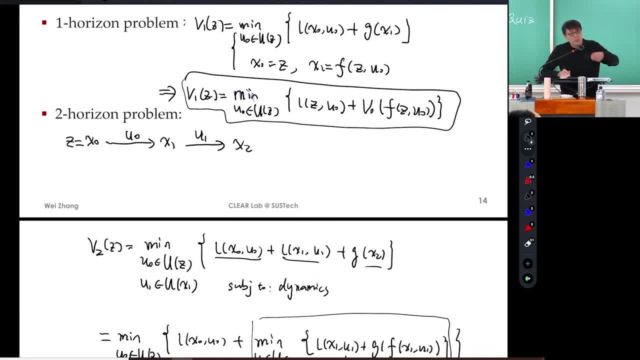 Before we also have this right. So this, any optimization, you optimize it. you will have arg min right. this guy, So mu zero z star will be arg min of this as well. the whole thing You optimize, you find the optimizer and also the optimal. 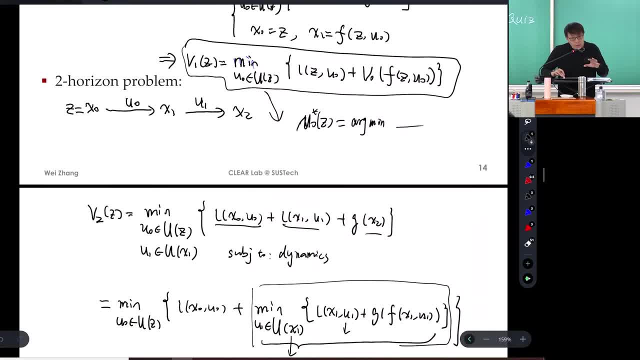 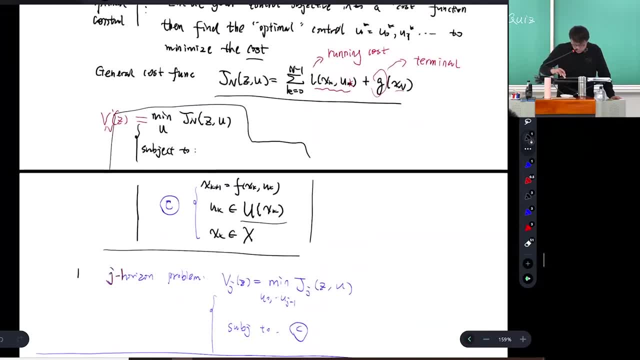 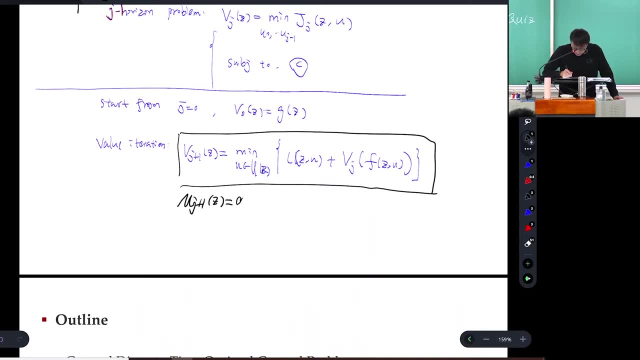 So that's the value. Overall you will have mu one, mu two, mu three, mu n, star right. If I go back to our review part, this will be our mu j plus one z is arg min. That's our control, optimal control, action. I want to pick. 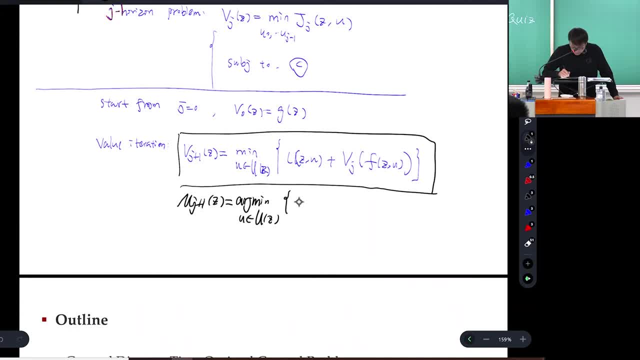 Of course u belong to u of z. This is l z of u plus v j. This is arg min. That's our optimal control action I want to pick. Of course u belong to u of z. This is l z of u plus v j. 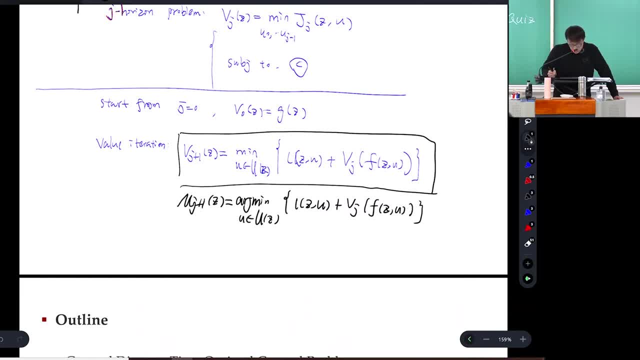 This is arg min. This is a value of i z of u. That's arg min. What does this mean? I want you to speak it out, okay, not the equation. What's the meaning of mu? let's call it star, okay. 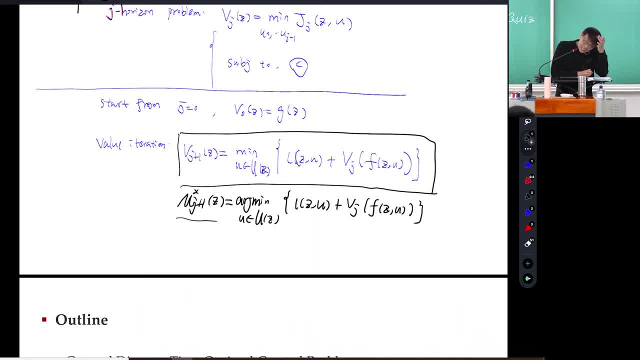 What's the mu- j plus one z. The optimal control action you need to take if there are j plus one steps left and you are currently at state Z. You know the difference between J and Z, okay, Hopefully my pronunciation is clear enough. 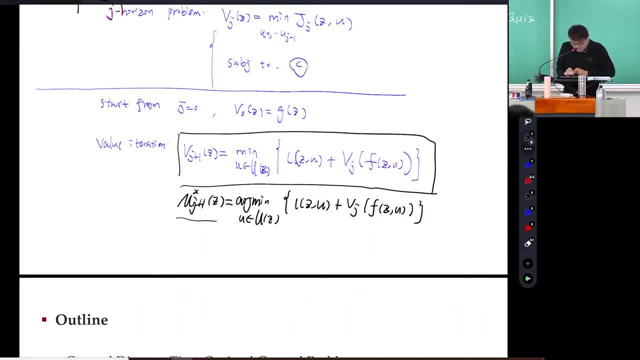 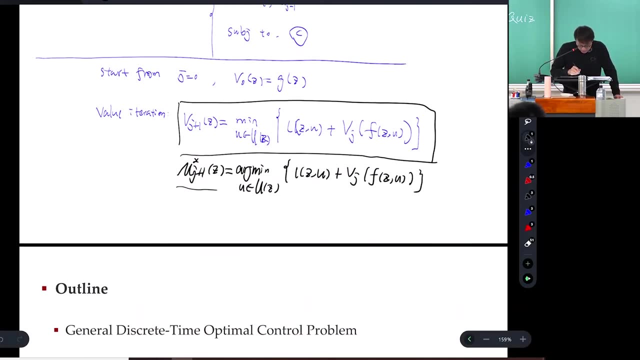 that you know. this is J, this is Z. okay, J and a Z. it's hard, All right, you see the meaning. Okay, now let me test you a little bit. I think I tested you already. So X, zero, you apply the optimal control action. 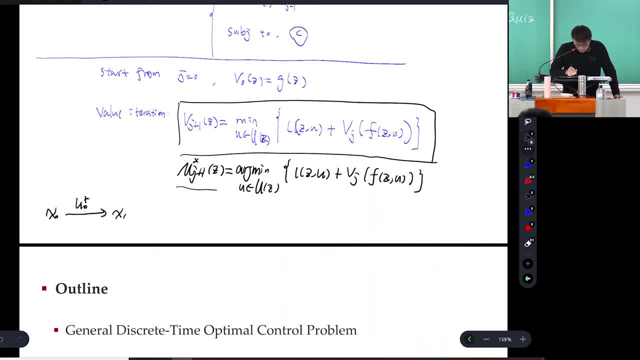 U zero star, suppose n steps right. You move to X, one star, then you apply U one star, you go to X, two star, keep going And I can tell you that this U zero star. that's the control action. 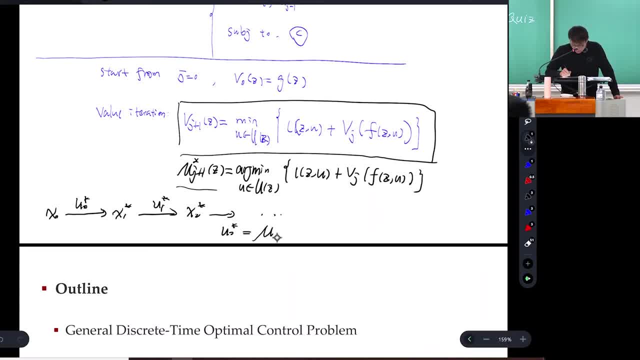 is equal to mu, n star of X, zero. Why? Because it's the optimal control action you need to take if there are n steps left and you are currently at Z, which is X, zero. Okay, and U one star is mu, how many steps you left. 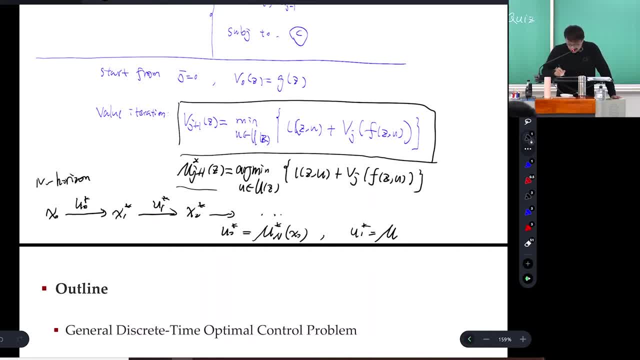 Suppose n-horizontal problem: okay, N minus one star. what X? one star right. Depending on your state, depending on where you are, your contraction is different And this mu of that is a function that means all the optimum contraction is a law right. 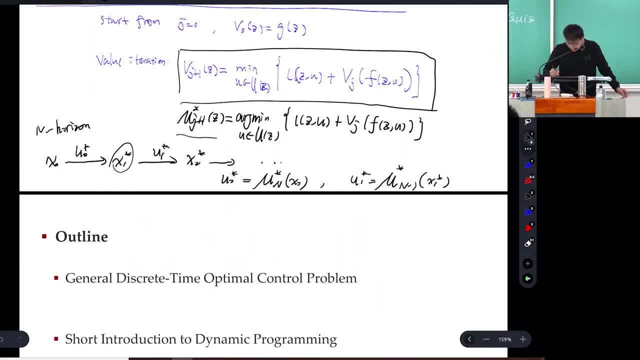 It's basically a function. If I say mu of n star of X zero, that's a control law right. That maps state to contraction. I can tell you that if my control law is mu n star, this is function right. 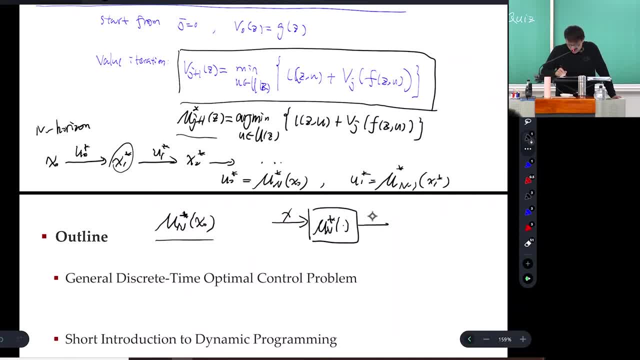 Whatever control, whatever state I put into, I will apply a contraction, and then that's my system. If I do this, this is MPC. Okay, that's exactly MPC. I don't think I have time to go through the details. 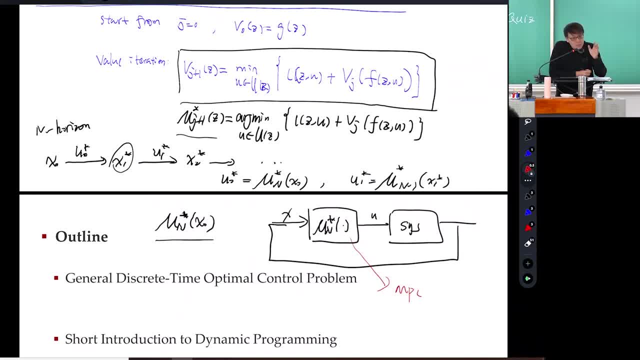 but that's exactly MPC And you can analyze its behavior. You see, if you want to apply the n-horizontal optimal control, your control law keep changing. Did you see the difference? The first one, you apply n-horizontal, The next one, you apply n-1-horizontal. 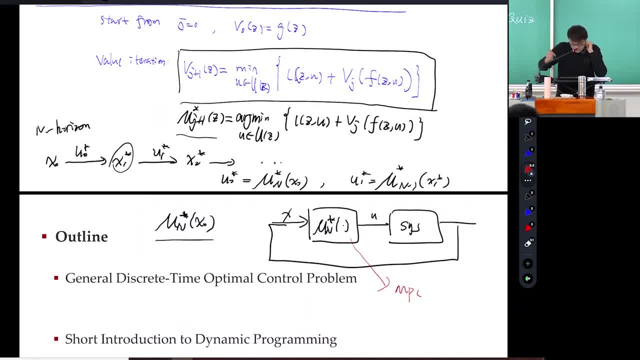 because your horizon is shorter one time. You're given a finite time. But if I keep applying the n-horizontal- I didn't change the horizon size At any given time- I think I have n-horizontal into the future. okay, I keep repleting this optimal control law. 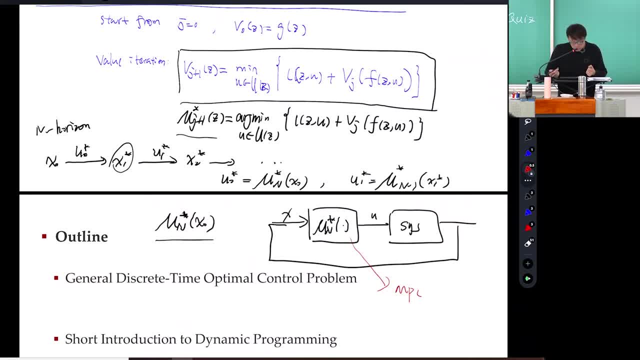 then I have a MPC model- predict control- Because once I apply this, then I have n-horizontal. Then I forgot about u1. now I just redo that again. So this is the optimal control law. We can analyze its behavior, even analyze stability. 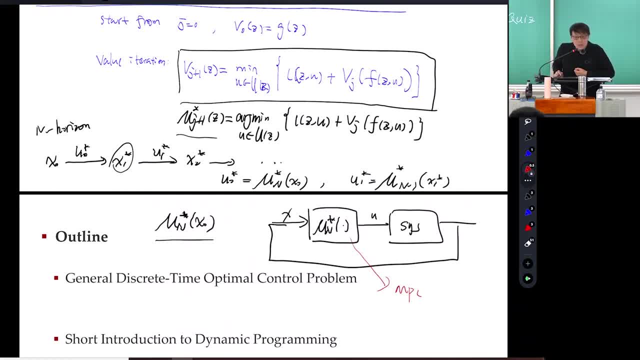 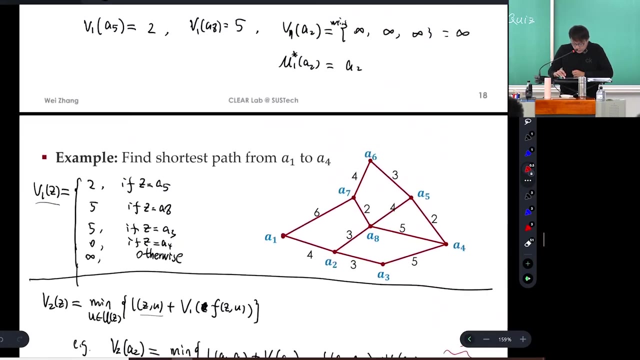 closed-loop stability under MPC controller. I think next semester I'm going to talk- Well, I don't think you can take it- I'll talk this in the more details- about, hopefully, everything about MPC next semester. So that's enough for the review. 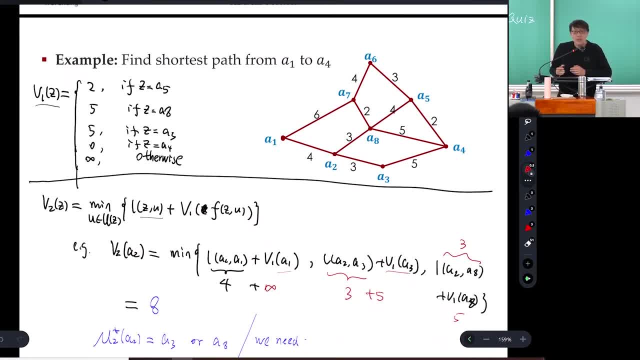 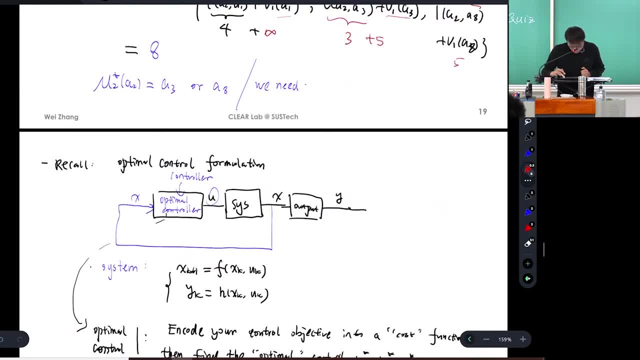 and a little bit more in-depth discussion. Let's go back to our example. As I mentioned, if you don't write code, you don't understand. Okay, let's see, This is a. we didn't write code before, right. 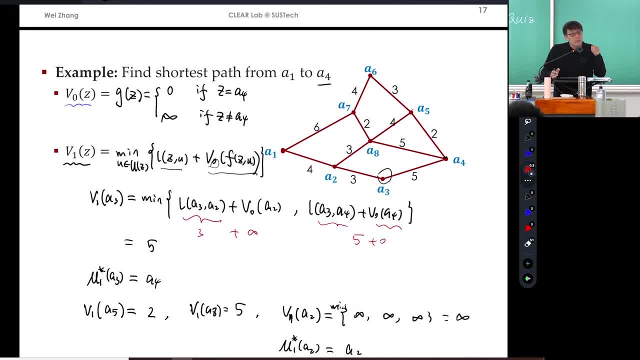 So this shortest path problem, almost trivial to solve, but we need to know or we need to derive solutions as if we are the program. okay, We designed as if we are the program. Okay, We designed as if we are the program. 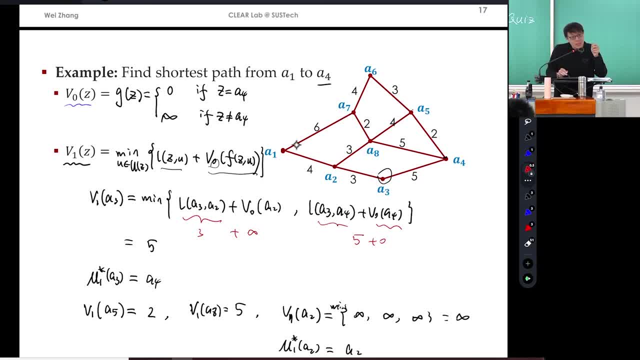 This is a terminal cost. We did our running cost, which is the length of its link. Then we do the value iteration. Did you remember? This graph can be really large, right In the example in the homework, the last homework. 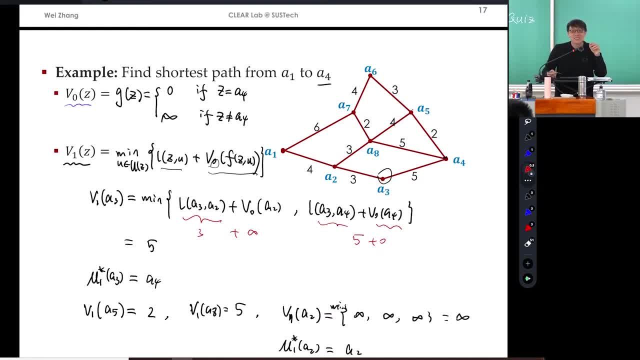 you were asked to do. you forgot about homework. You need homework. I think You will love it. I think because without it, you may not know what to review for the exam. final The error fair problem, that's the homework right. 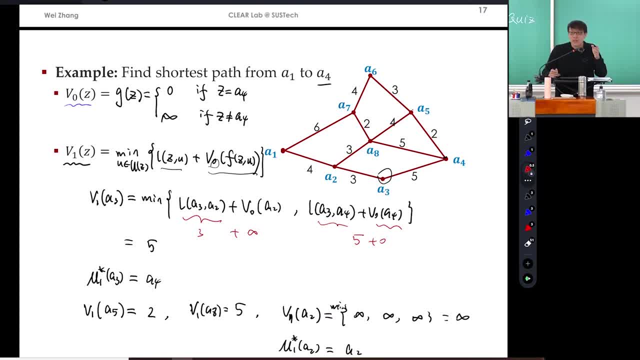 Today I'm going to write a code for you as a starting point for you to solve homeworks. Let's just- I never done this before, okay, Let's just write a code to solve this problem- DP. How hard a DP problem is. 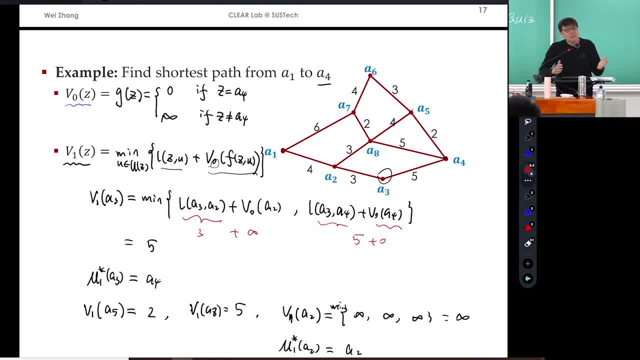 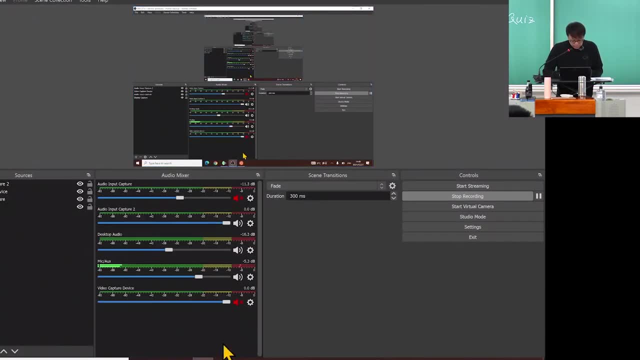 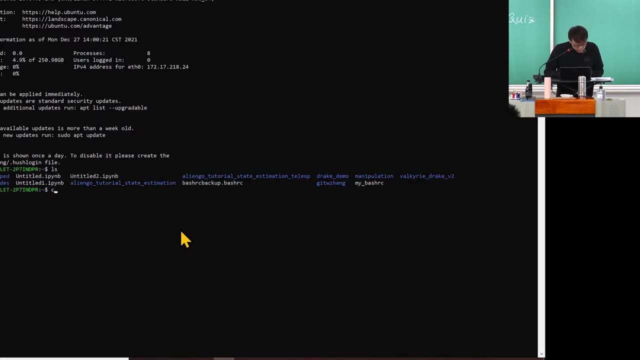 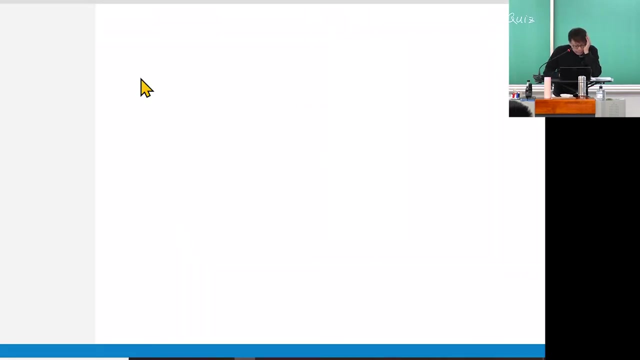 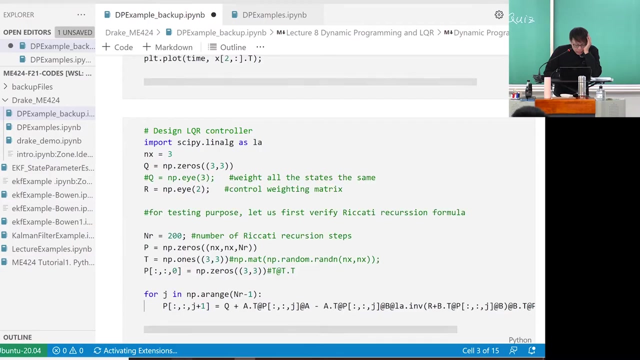 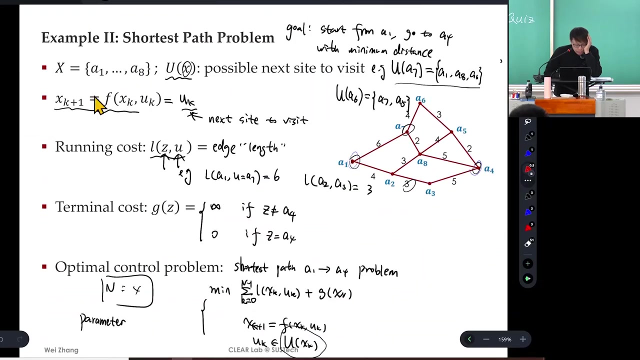 What are the coding? A few lines of code. If you know, everything is a few lines of code. Let's try to write these few lines of code. Let's see, let's ME. Let's try to write. Did we formulate this problem before? 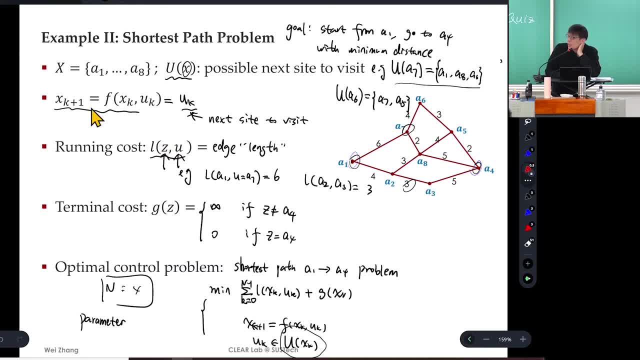 as an optimal control problem. Right, That's our reformulation. That's the state uptake equation, That's our state space. right, Running cost, terminal cost and optimal control problem: All right, this is running call, terminal calls and this, right, how do we write code that's? 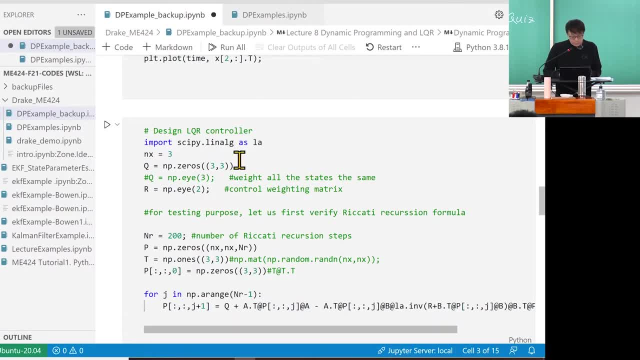 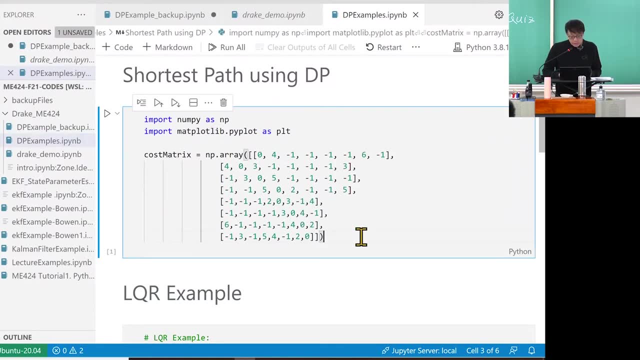 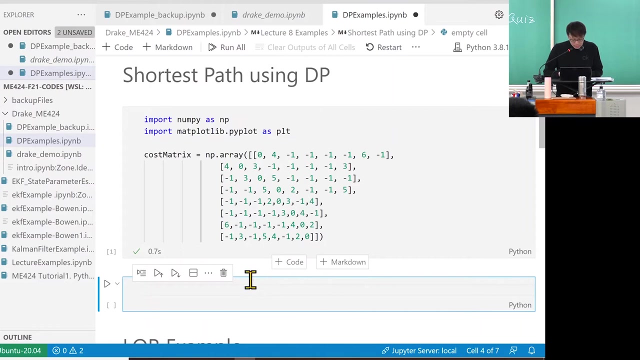 really important. I think let's hold on, let's do this. I already. it take me some time to type in all these numbers. I'm not sure whether it's true. that's 8 by 8, let's let's see. okay, 8 by 8, let's print cost matrix. 8 by 8, it's symmetric. 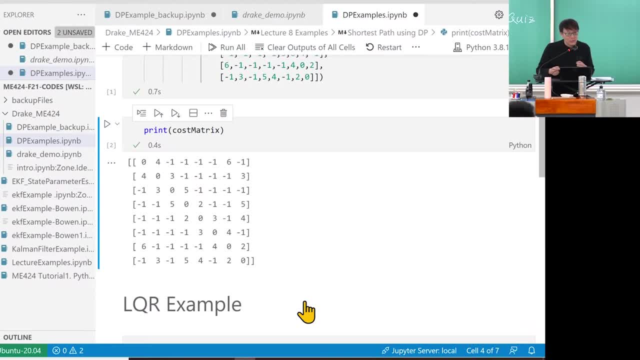 because the link, I think, is undirected graph. okay, from one to the other versus the other. from one is the same cost, right from this means if you stay at zero, zero cost. if you from not zero, one, okay, let's say one. one, two, two is four. 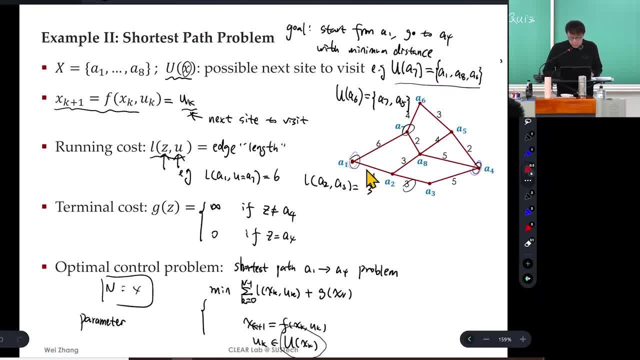 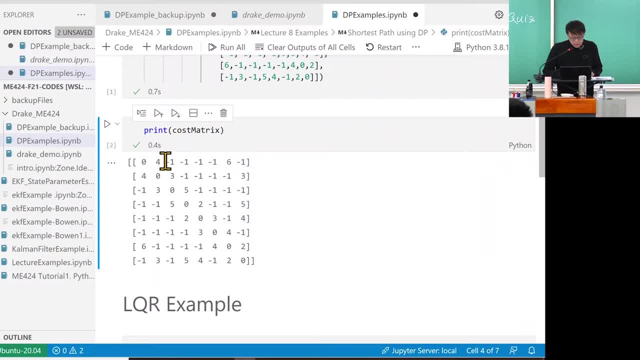 right, okay, let's look at our one two two is four. one two, seven is six. one two, seven, seven is this one. all the others are negative one. I just use negative one. two means big, big, big, large infinity, whatever. okay, I can assign this cost to be different things later on, but for now it's just the negative. one means: 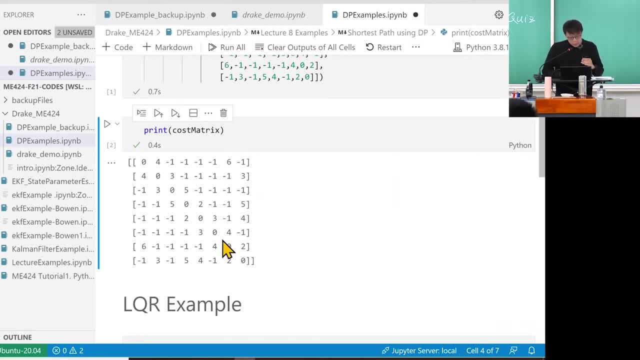 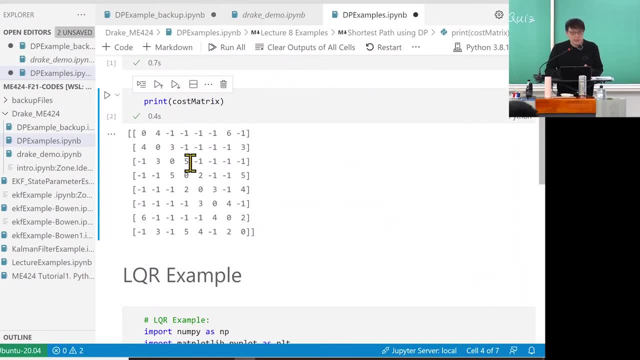 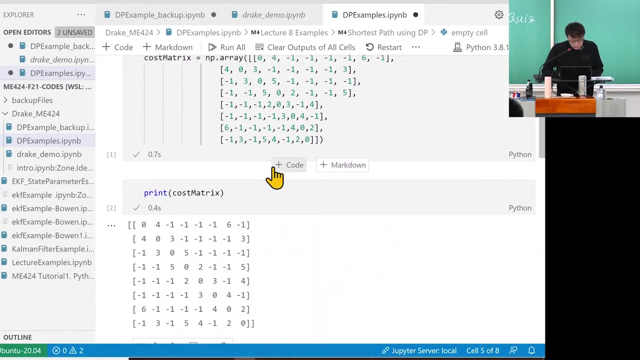 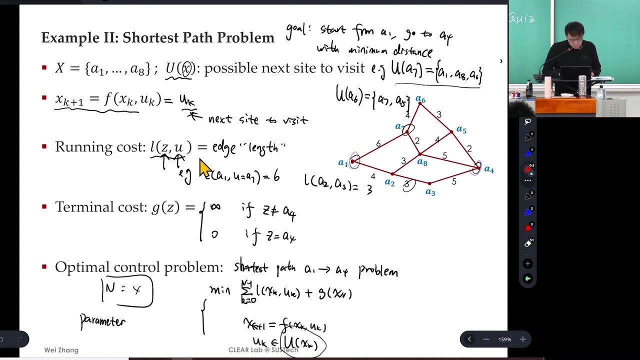 infinity in this cost matrix. all right, hopefully you trust my. I think it's right. okay, that's the cost matrix, that's the graph. okay, now we are trying to. let's see, hold on, now we are trying to solve the problem. first of all, how to get started. 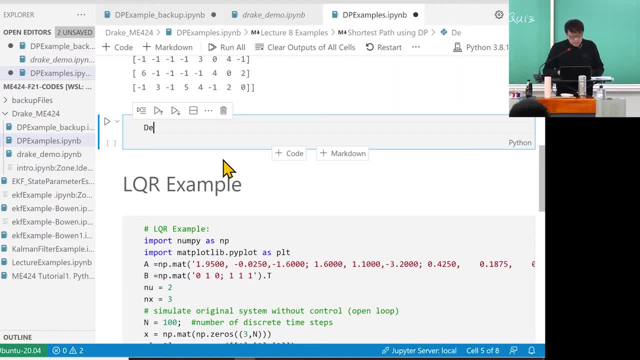 okay, okay. So the first step, um, we want to come out of the talvez. let's uh about different people define different. not I like to do the value retracement first. okay so, Bobby TBI, define how to do, define, define like this: so: defined value iteration. okay, the 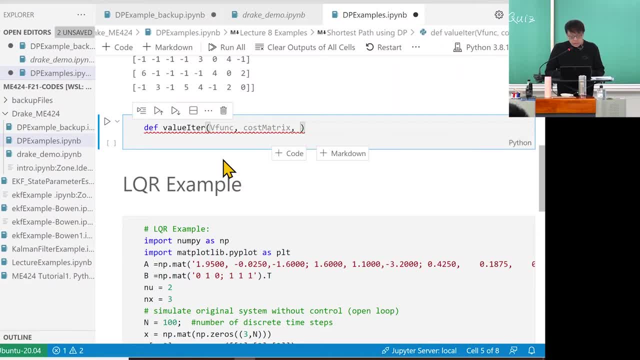 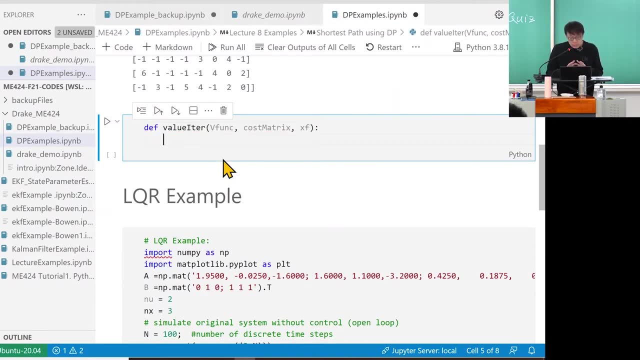 thing I need is the, the function. I also need the cost matrix and for the valorators, I also need to know, let's say, terminal state. Okay, I need to know terminal state. So what we need is, each time I need, let's say, J. 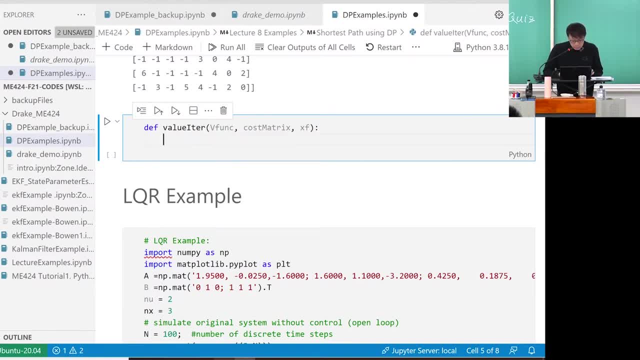 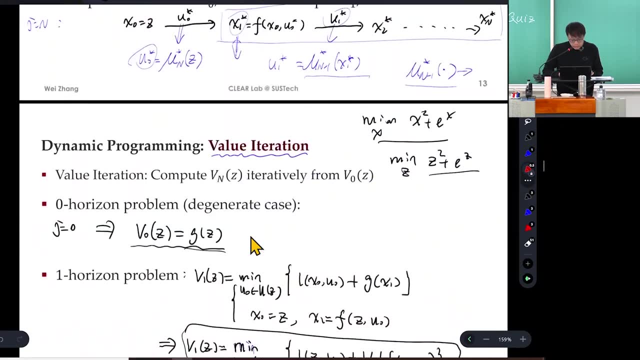 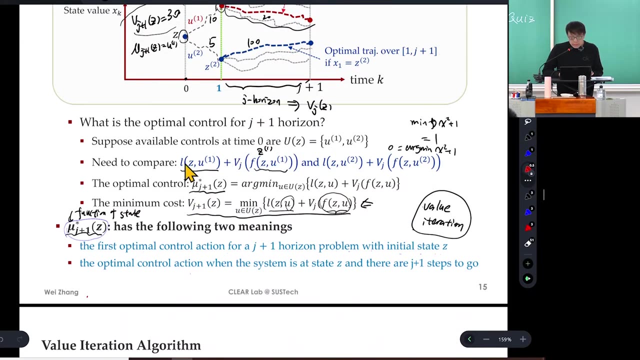 Oh, let me think This step. let's try to map to the map. okay, So each given time, we need to compare a few things. What are the things we need to compare? Yeah, yeah, that's okay. 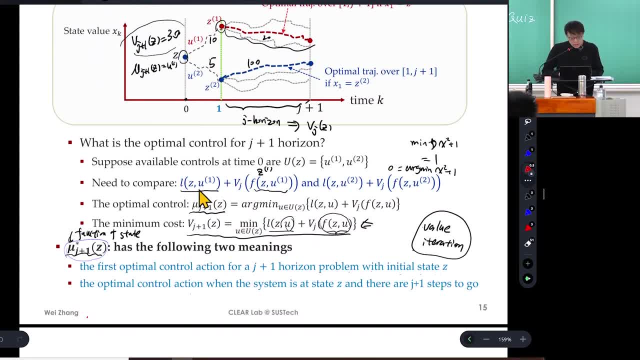 Let's follow my notes. okay, Let's just map the map to code. So this: for each U you need to compare running cost per DOS plus the next value, function cost right, And for different U's you need to pick the one that's. 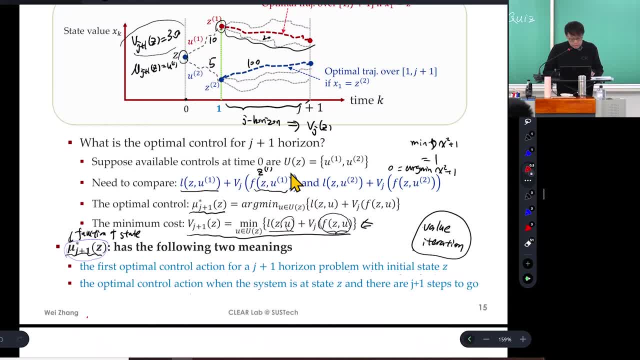 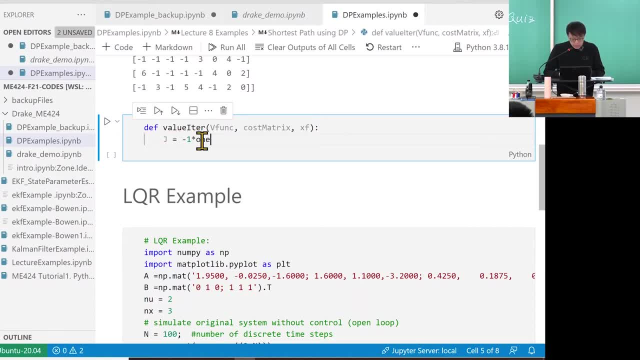 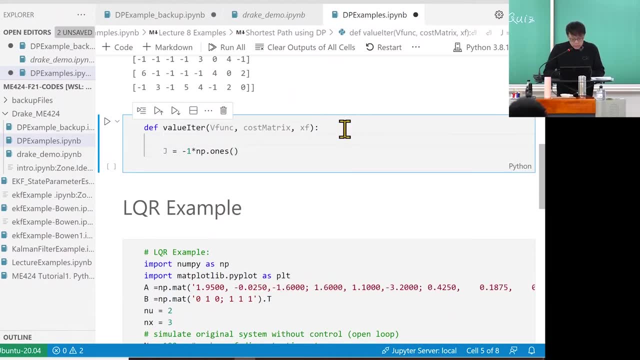 the U, that's minimize all the possible actions, right, So I will call this J of U equal to. let's initialize this. Let's neglect U one one, NP, dot one. What's the dimension? Let's do a little bit general N equal to. 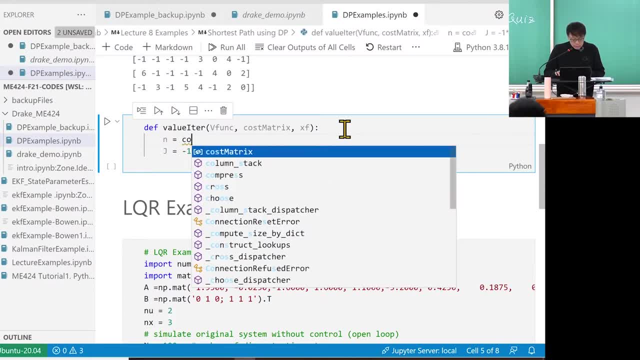 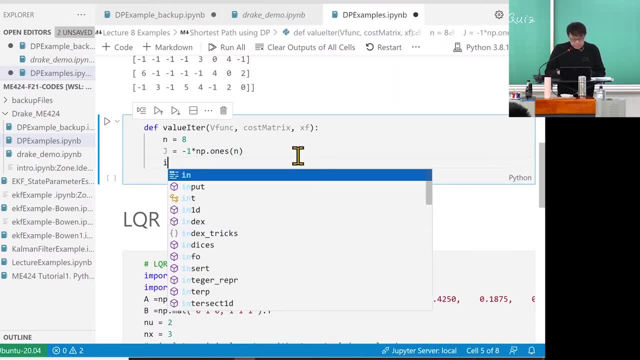 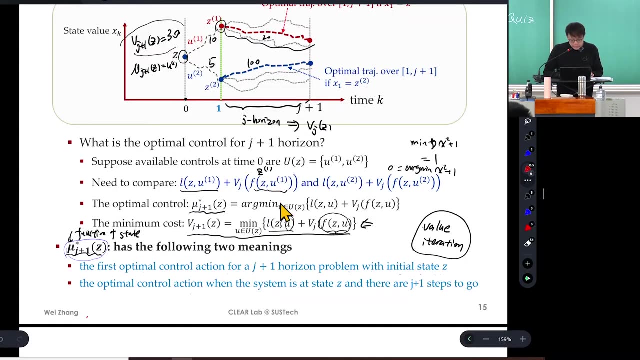 Cost matrix. Let's get really hard to code it. sorry, Eight. okay, This is N, Okay. the value function, which is the value, let's say v. next What we are doing: value iteration from vj to vj plus one. 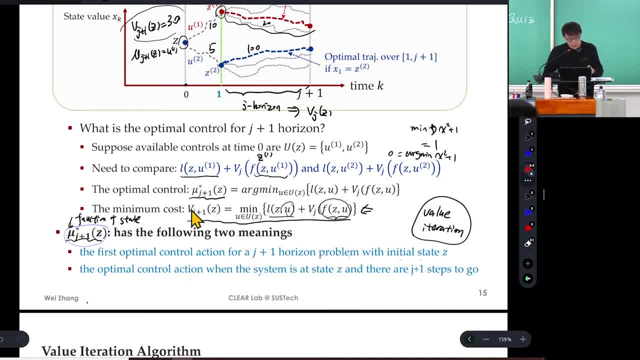 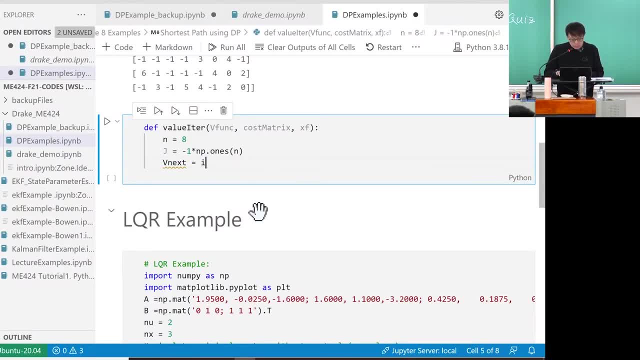 Let me repeat: I need to. you gave me vj. I need to tell you what vj plus one is And also I tell you what's the optimal control action I need to take. V next is also: whatever initialization is fine. 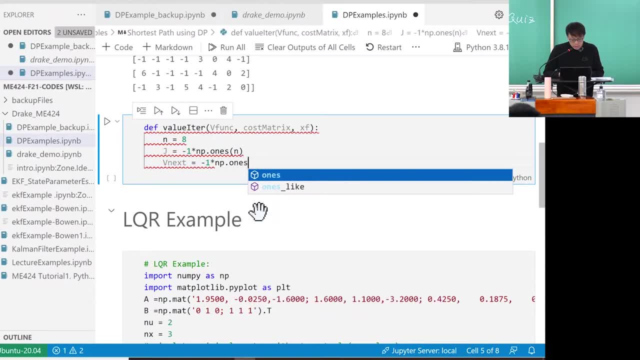 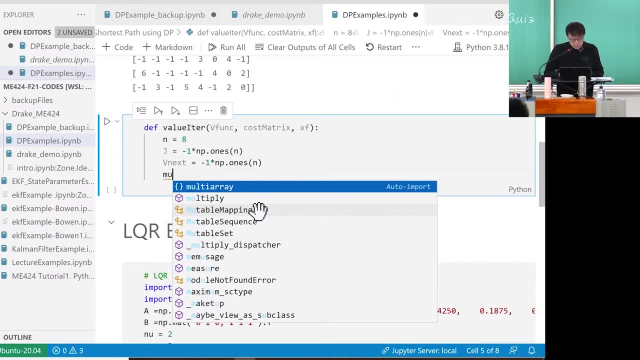 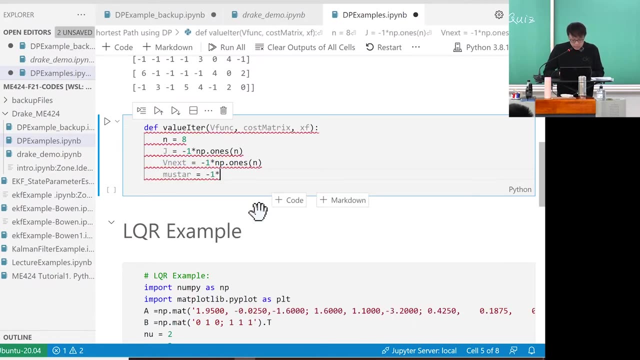 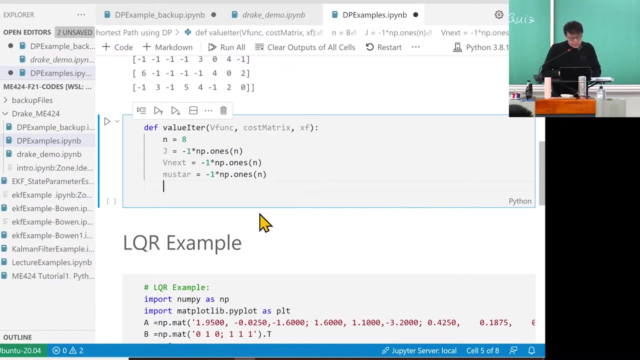 let's just say next to one times np dot ones and what else I need. I also need mu Mu star. mu star is next to one times np times np dot ones. and okay, that's some initialization, Then I can start for each state. 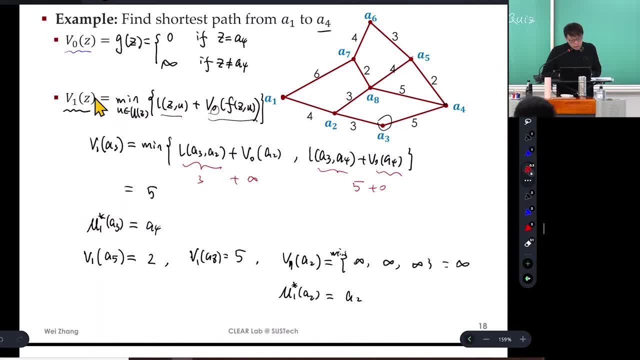 look at. I mean, just need to repeat what we did here. For all the z, you need to find a function that means for all the possible state z, you need to compute the value and also compute the optimal mu star right. 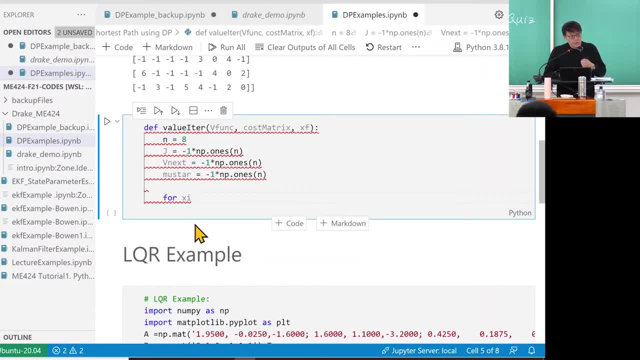 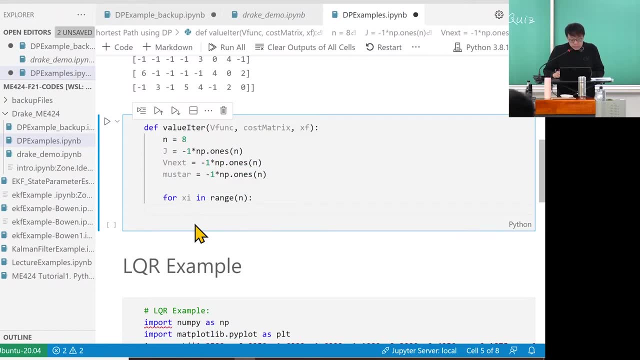 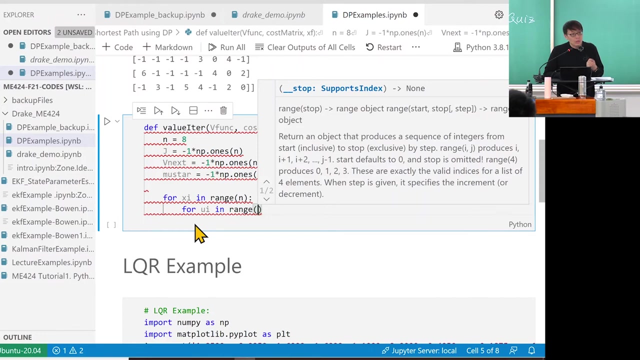 So if you have a for loop, that for, let's say, xi, that means the index for state in range, n Hold on, that's fine, and for ui, ui in range because u also control action that I can take in general. 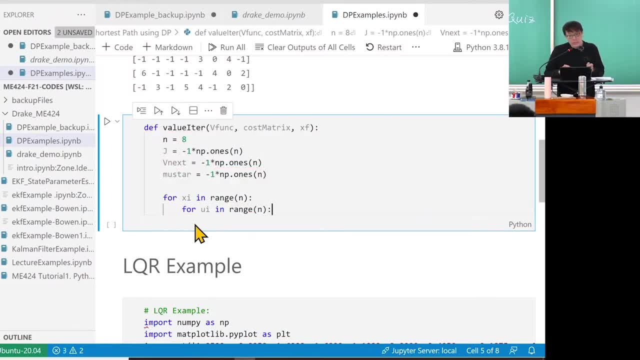 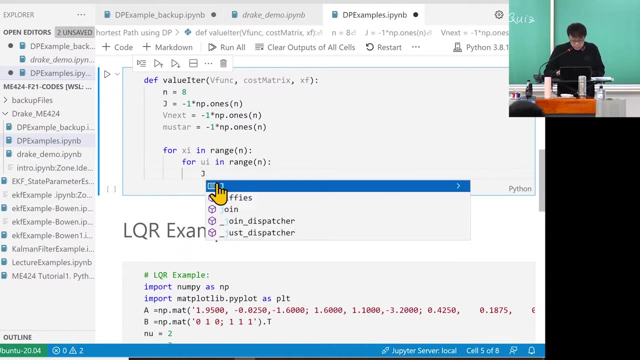 I don't know what I can take. let's say this and all the state I can, possible, but some state are next to one. that means impossible, right, And this is what is it. I need to compute uj of ui equal to. 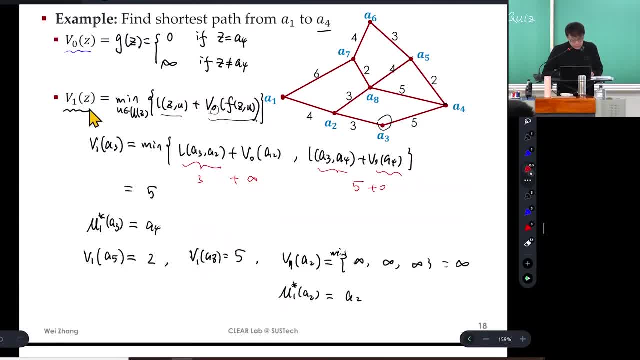 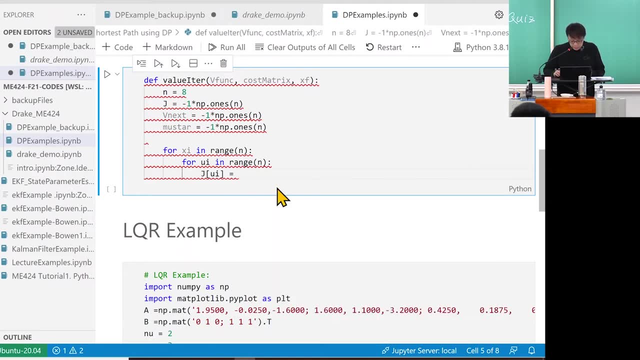 for each state. look at this: okay, V is the minimum amount is two, right. So for that means for each u, Each u is running cost plus the next, the previous, okay, So that will be a cost matrix. 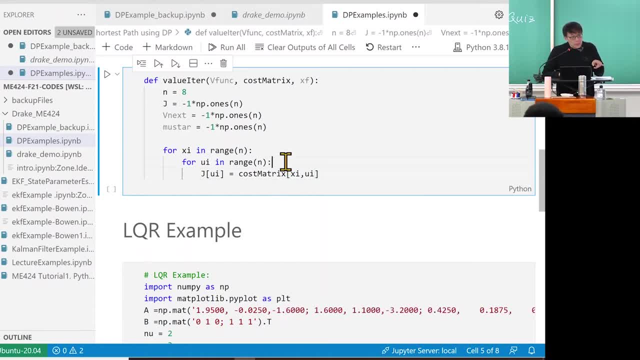 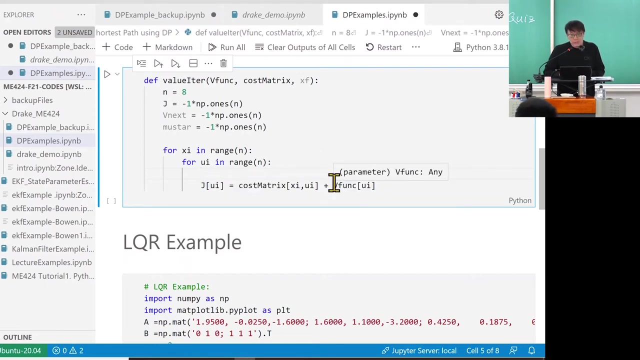 From xi to ui. yes, right, That's my cost. Okay. And plus plus the v function of. suppose it's also n dimensional vector next, right Next is ui, No v function, J plus y is v next. 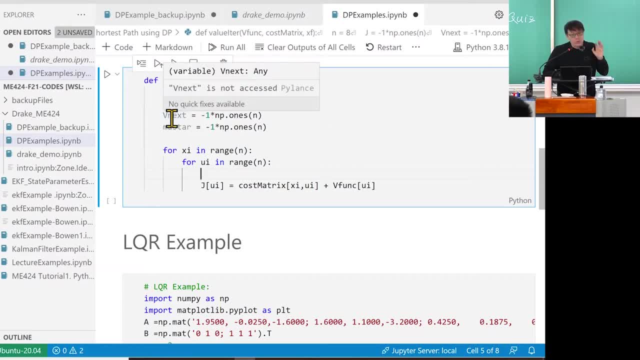 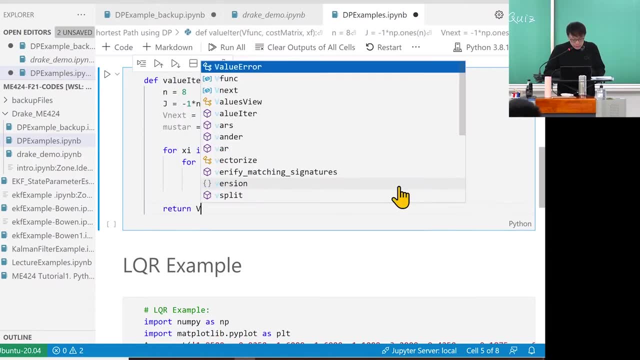 V is v is the current of vj. This is vj. I need to compute v next Right. If I want to do this, I need to return v. next that's vj and mu star. That's my return of my value iteration. 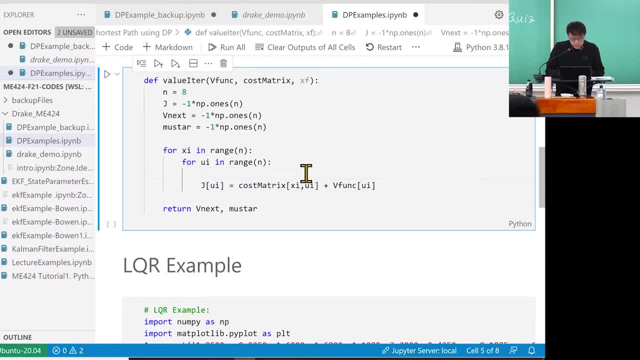 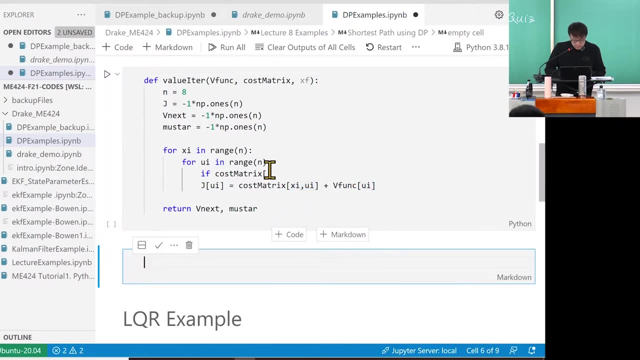 That's it. Of course, you need to make sure that- no, sorry, I'm gonna do this cost matrix. If cost matrix here, ui, no, no, no sorry, this guy, This guy ui, is equal to next one of this infinity. 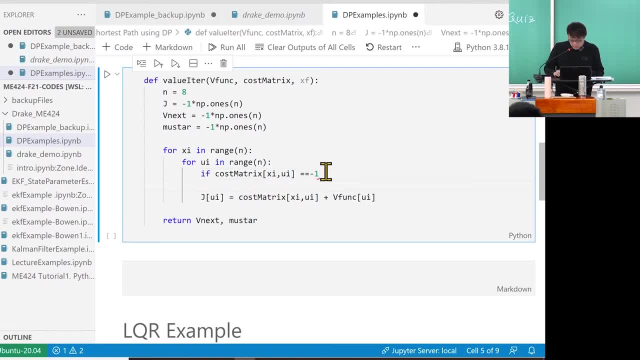 I cannot do the traditional sum right. I will just say here that will be my j of j of ui equal to. that's a very big number, okay, All right, that's almost like infinity. And this guy is this. 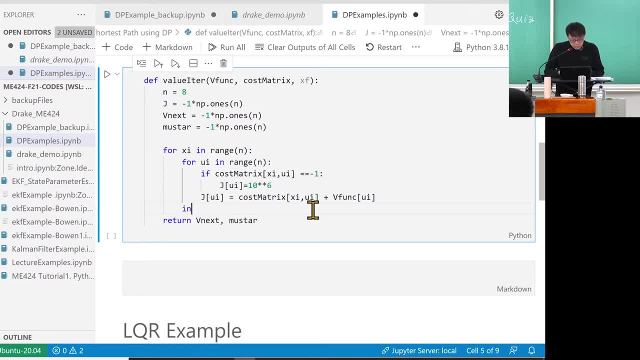 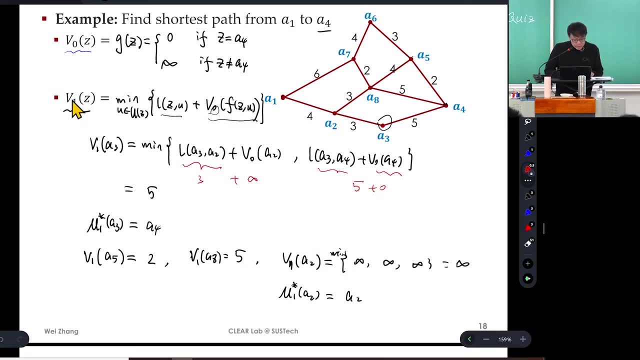 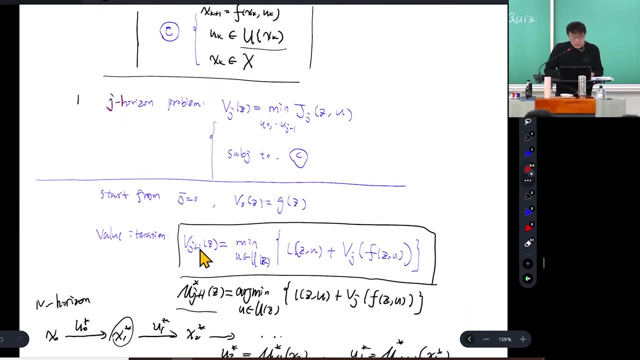 I think that's it. Then I need to do, and then, of course, of course, V of xi. what is it? V one? or, if I look at my formula, let's look at this formula. okay, That means vj plus one is v next. 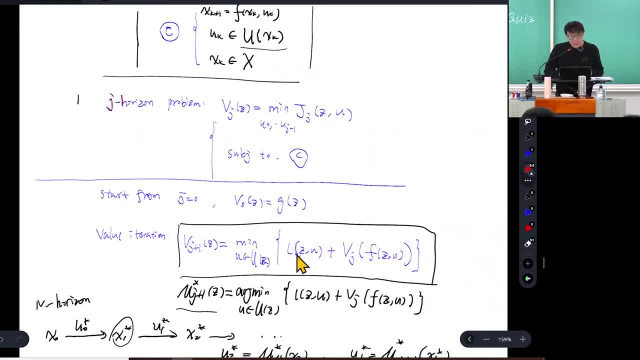 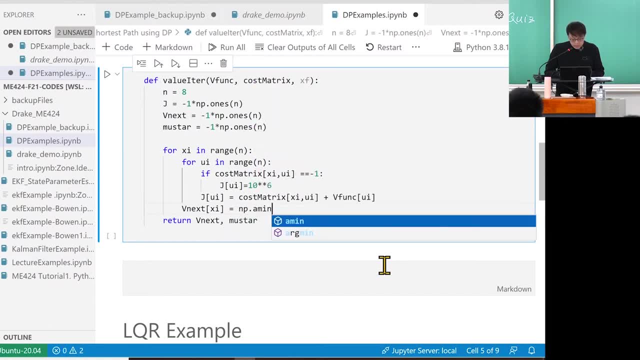 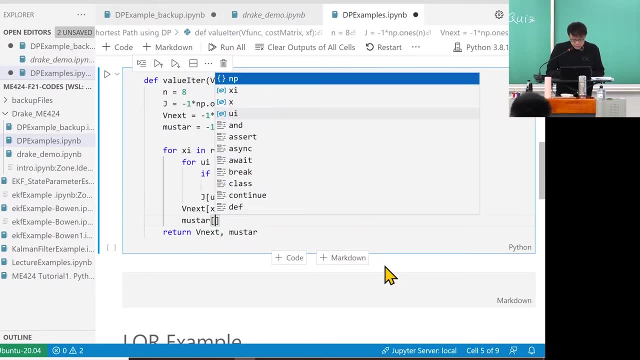 V, next, of this state, equals to the mean of this right. So that's the equal to numpy dot. I mean j okay, And this mu star of xi, which one Is this one? Mu star x one is equal to. 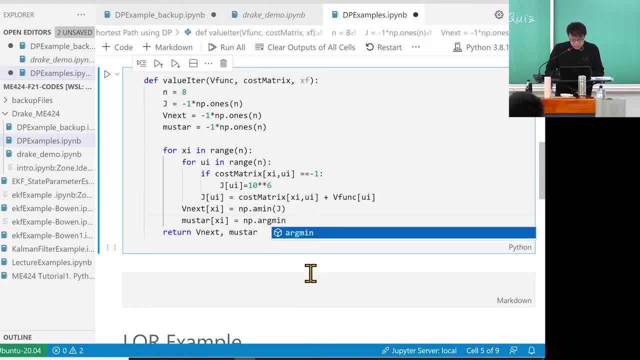 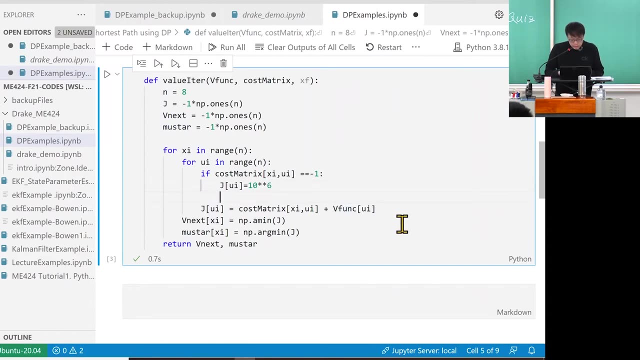 np, dot, argmin, j And that's it. Okay, I think that's roughly. I think there are even errors for if or how. Oh, okay, This will be Okay. yes, IELTS, Okay, there's no bug. 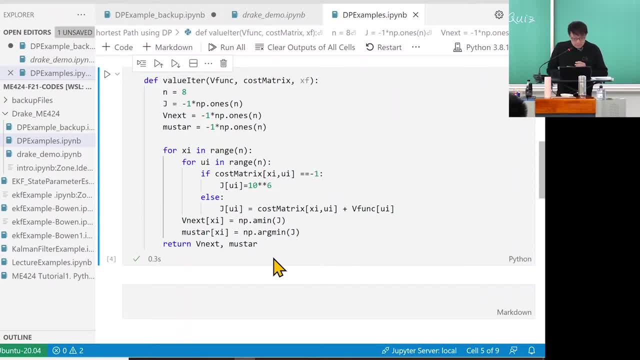 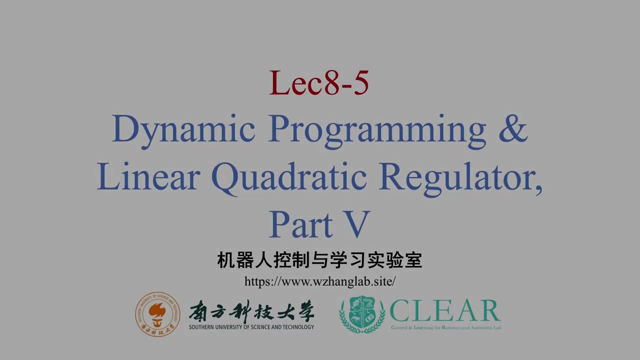 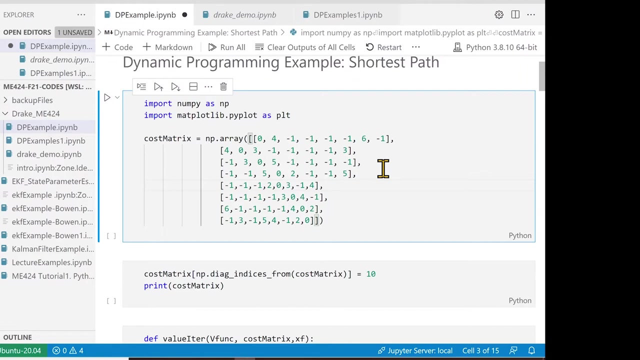 That doesn't mean it works. We'll continue next, next class. okay, Take a break. Take a break. I modify the code a little bit So before my diagonals are all zero, that means I can stay. I can stay at a current state without incurring any cost. 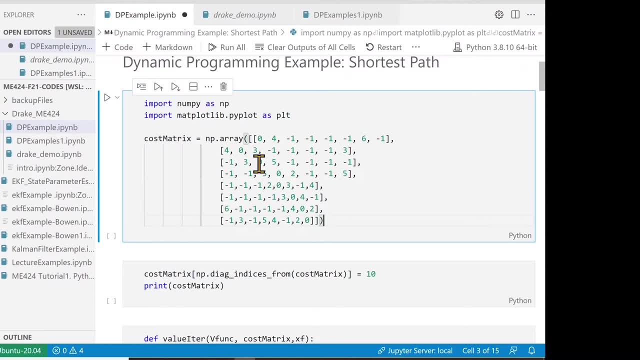 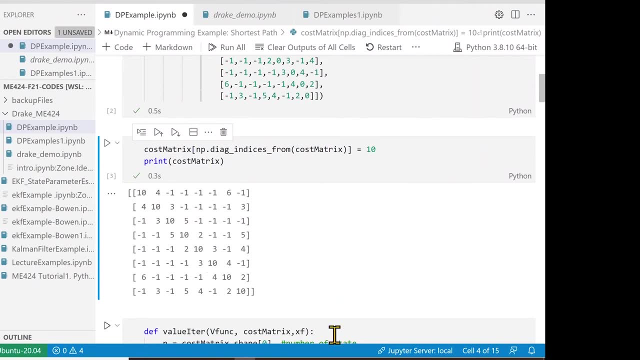 Okay, I don't like this behavior. I want to encourage them to move. So I change it to: I change the diagonal to be 10, okay, So you have to move, otherwise it's not like, otherwise they will keep. 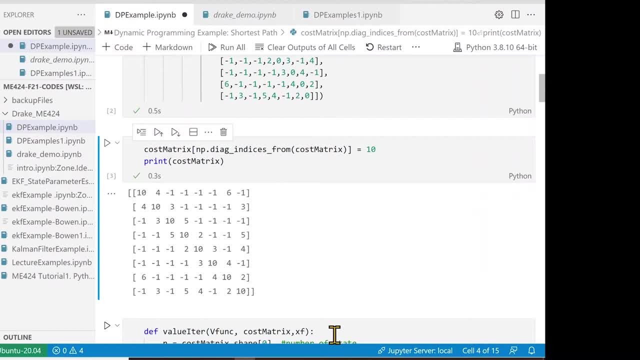 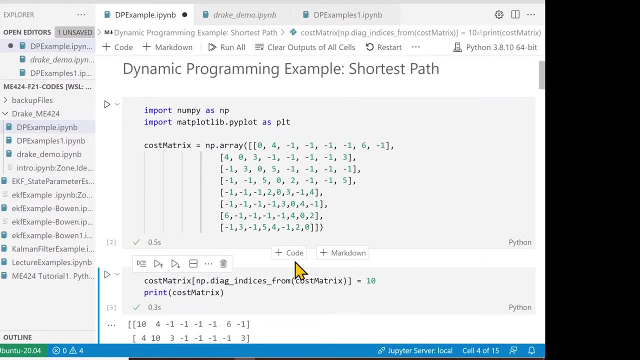 I would like them. let's say, if you have more, suppose you can get to the final state in four steps, but I gave you 10 steps, Then previous call structure. you can stay at the beginning, waste six steps, then move right. 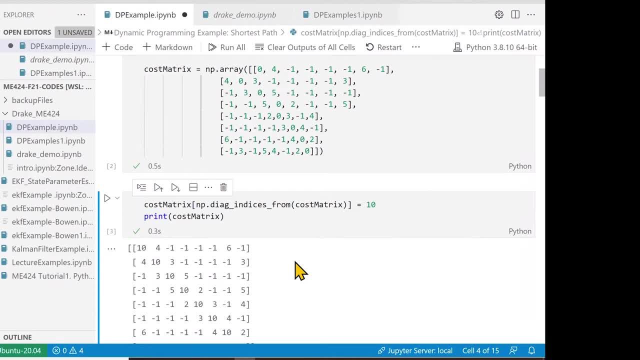 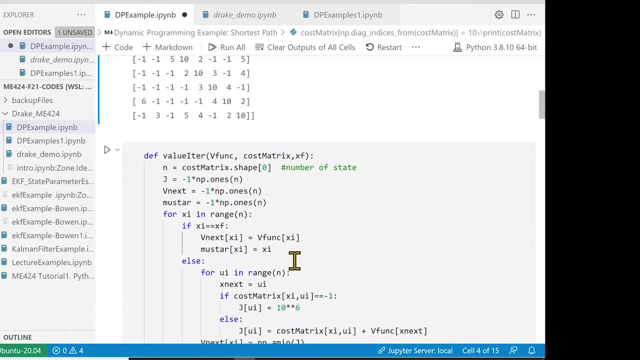 But now I want to make sure you just go to their end state, wait for the end of the time horizon. So that's how I change the call structure to reflect my objective. You see what I mean. Nothing is given for sure, it's just how to encode your objective into cost functions. 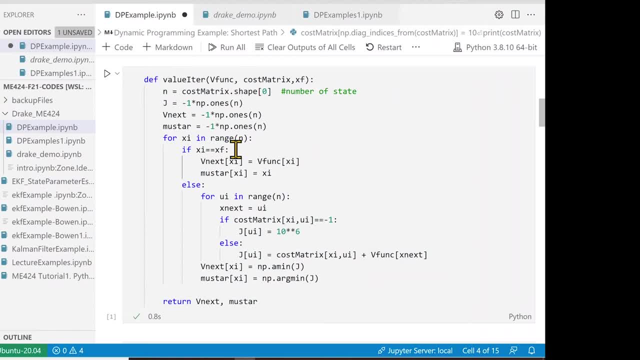 And then this one is now. it depends on the initial state. I think that, sorry, the terminal ones, if you're terminals, I already did decide the optimal cost. optimal control is just state. If you're terminal, your optimal control is state. 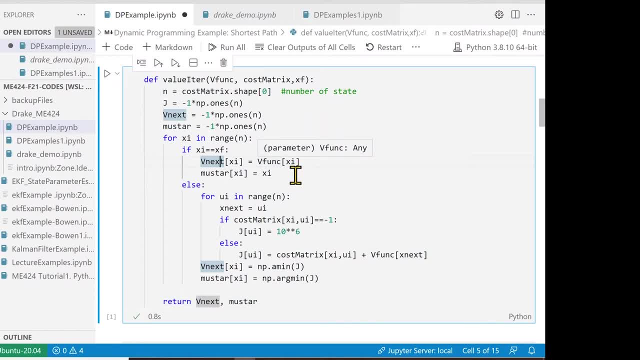 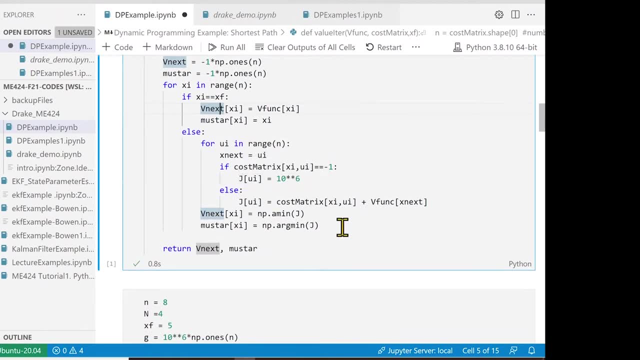 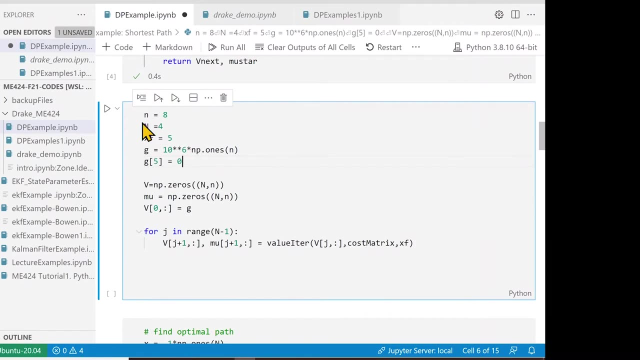 and the optimal cost is nothing, because there's no running cost. you stay there. If not in the final cost, then it's just what we wrote down just a few minutes ago And that's our valid version. Then we can start okay. 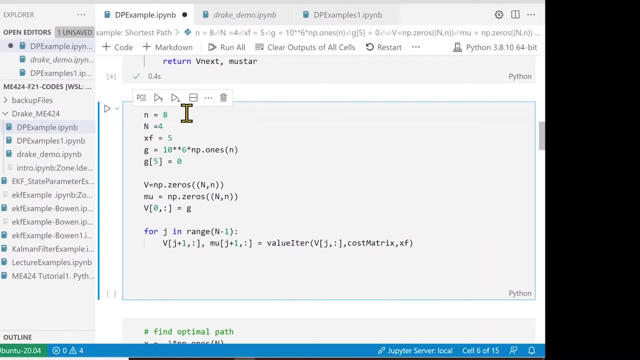 This is I have end state, eight cities right Eight sites. horizon I gave is four- I can give more, by the way, And terminal I want to go to in the lecture note where we want to go. 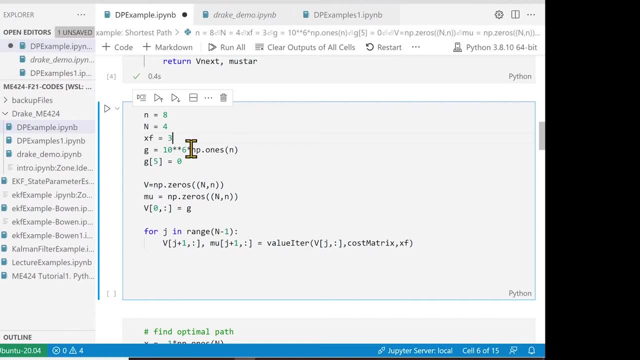 Four, right For the index, this would be three, okay, And I mean the terminal state is this, So I can assign a terminal cost g function, Which is all, all infinity. this is infinity, all right, Except. 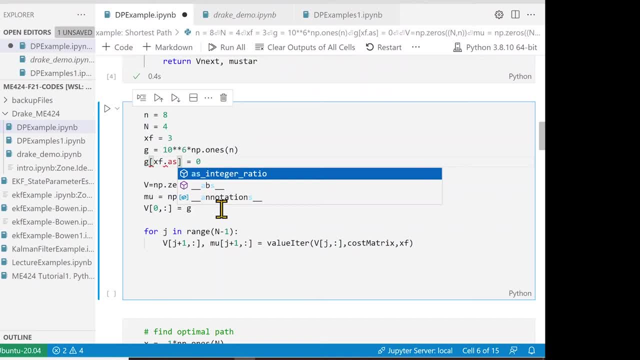 I will say x, i've dot, i type int: okay. So except this thing, If I- I'm not sure whether it's floating or not, but anyway I want to use that integer to index it. So g of the terminal state is: 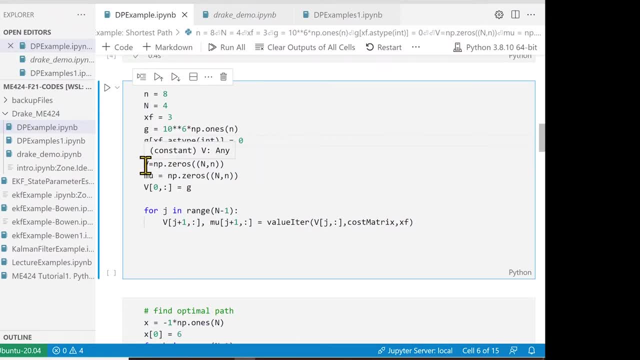 zero. Okay, Then I start my value iteration. Okay, The first value iteration is: I have an origin, and every horizon, every time step, I have a. this is v of all the states, right State is small and and mu is also the same thing. 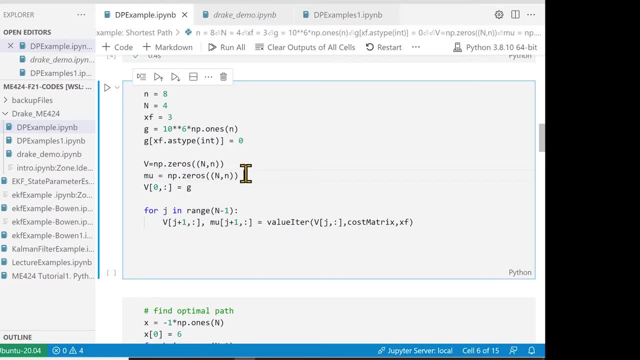 it's a mu, one of z, mu, two of z is a function, And so that's. in this case it's rho is a function. all right, And that's it. And initially the first row is G V, zero. 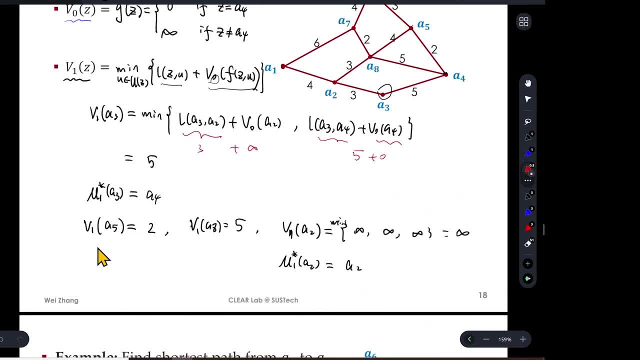 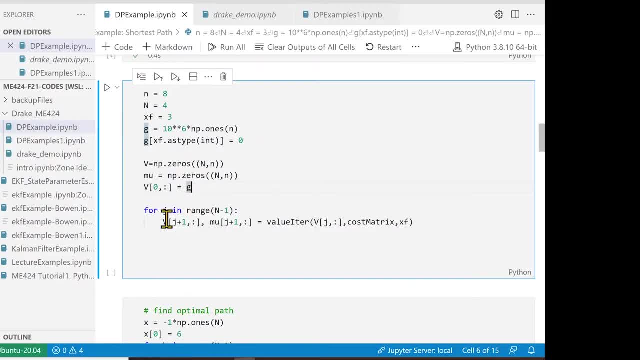 that's exactly the math here: V zero. what V zero is this? Okay, so that's it. Then I do value iteration. there's one line of code, that's it. I solve it If I run it. hold on, run it. 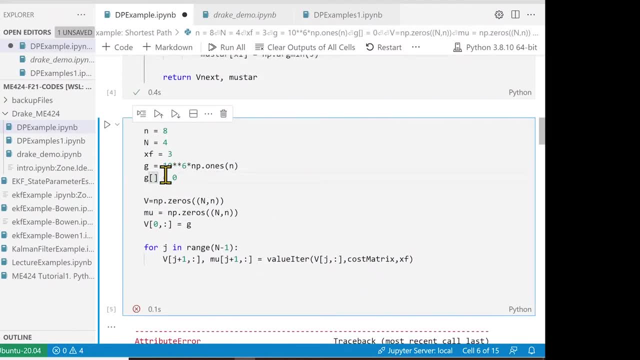 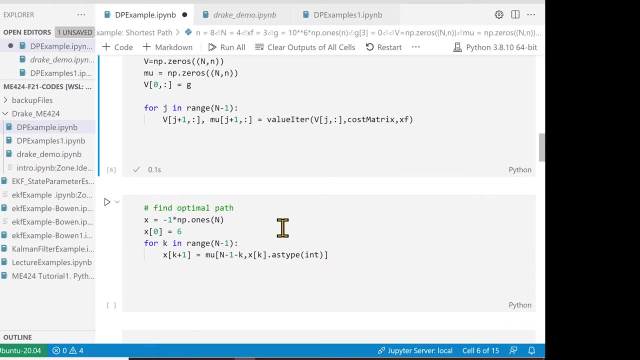 It doesn't work this way. let's, Let's just hard-code it for now. Okay, it works. Now I need to find the optimal path. I solve it. what did I solve If I want to print V function? 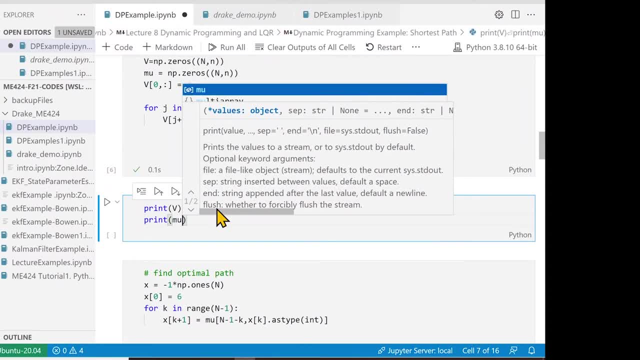 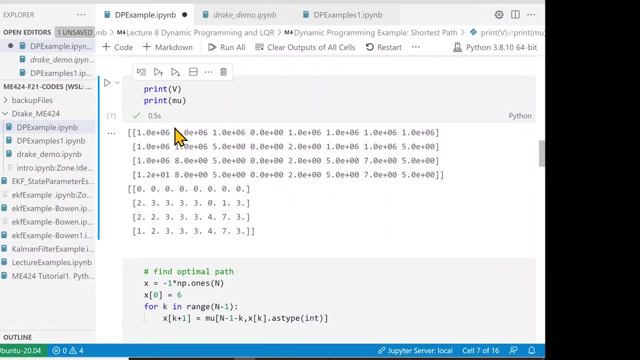 and let's say print mu function. okay. So those are the functions. each row is V, zero One. let's say this one: the first row is what The zero haور is: an optimal control cost, which is exactly G. 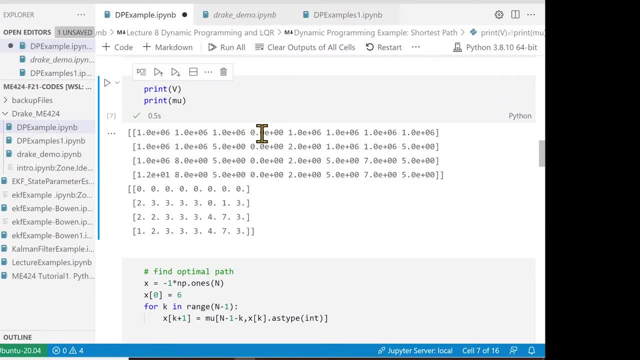 Everything is infinity, except for the fourth one, which is the three index right, Index three. We don't have U zero because we start out to have some action to take. as I said before, at least you have one horizon right. 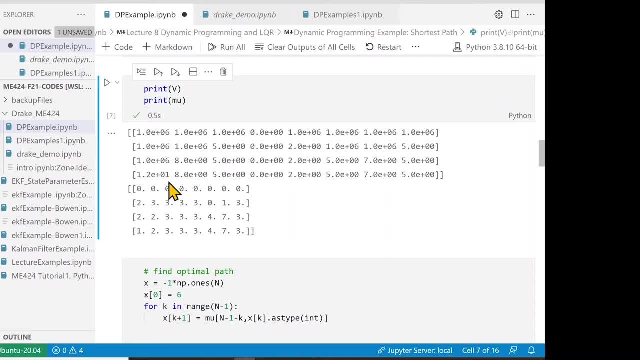 If you have zero horizon, there's no contraction you need to take. So this is the initial values, All right. the second lines, second rows, or optimal one horizon cost, okay. For example, this one means if I have one time horizon. 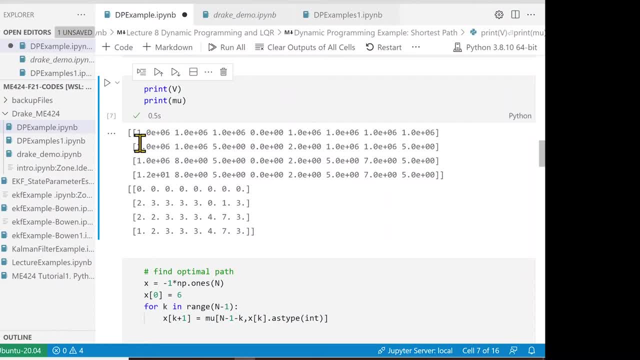 if I start from three, this is three. that's right. that's two to three. right The second row, third column, that's two to three. the optimal cost is five Right one horizon, Sorry, no, no, no. 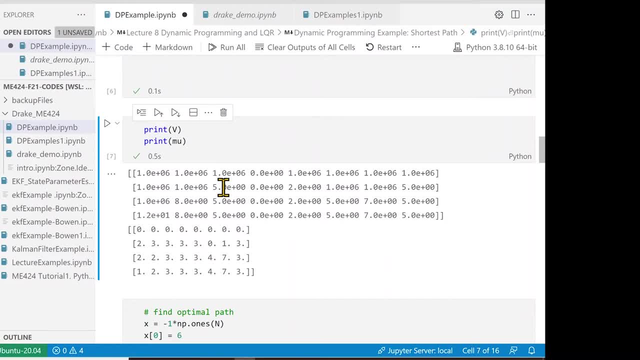 This is from three, right? So if I have one horizon, you start from three, A3, that's the third city- then the cost is non-trivial. now, It's not infinity, it's five. If you look at this figure, 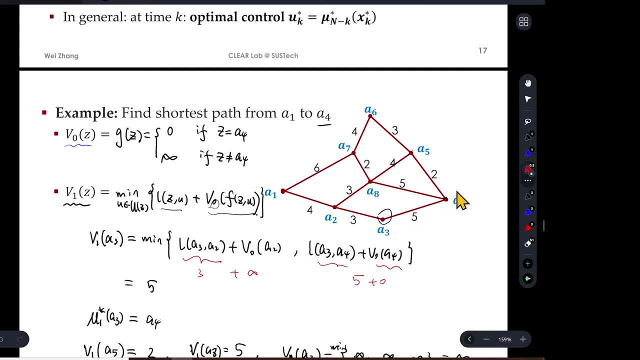 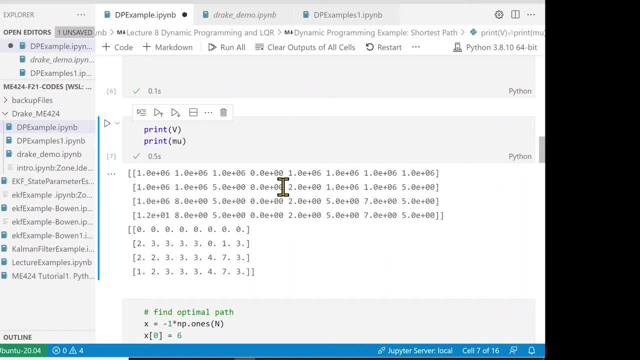 if you start from three, yes, you can get there in one horizon. It's no longer infinite, it's five. Okay, that means that. So anything, that is not, if you're at one horizon, you're still at, you're already at the four. 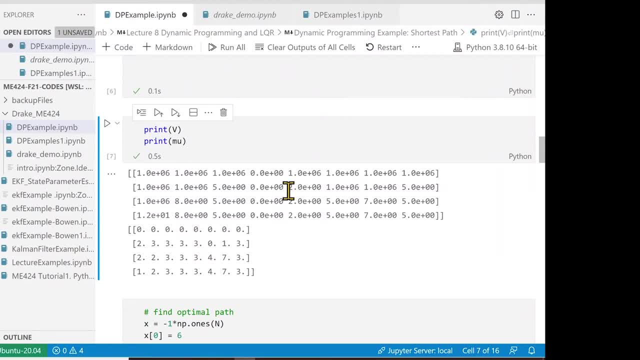 then you stay there. there's zero cost. Then this is from one, two, three, four, five, from A5 to A4, right, A5 to A4, the optimal cost is two like that, all right. 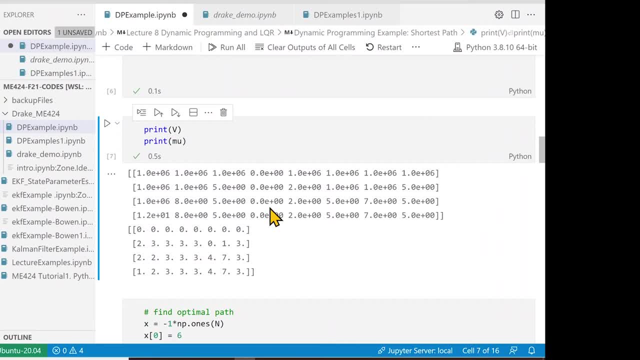 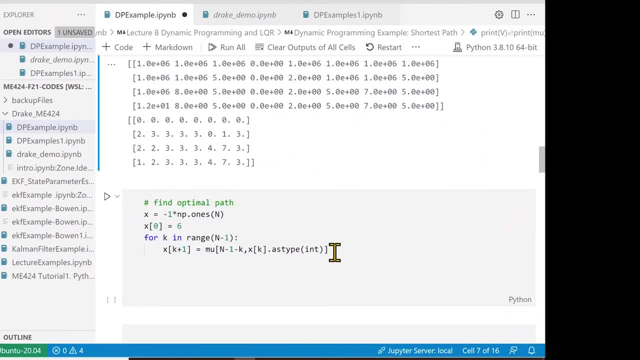 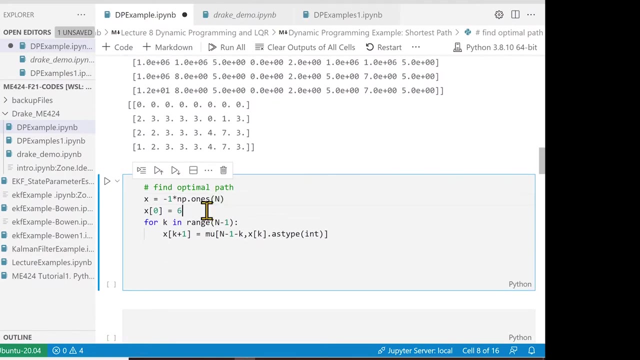 Of course you can see it, but you want to make sure your code, your code, can do it. then you can arbitrary generalize the problem to arbitrary complexity. So that's the meaning. Okay, so we have a control function, control law and also optimal cost function. 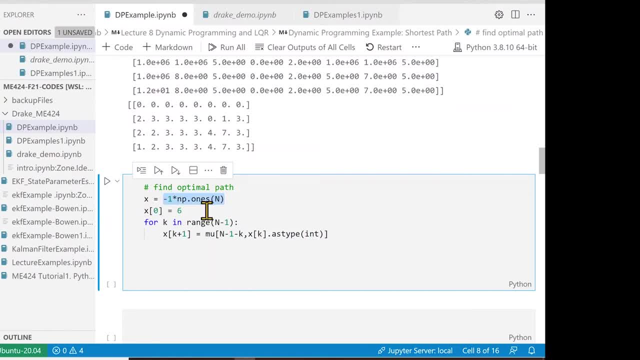 The way we started is like say I want to have the optimal control path. Let's say we start from. either way is fine. let's start from one right Start from one. one is zero. right Start from zero. okay. 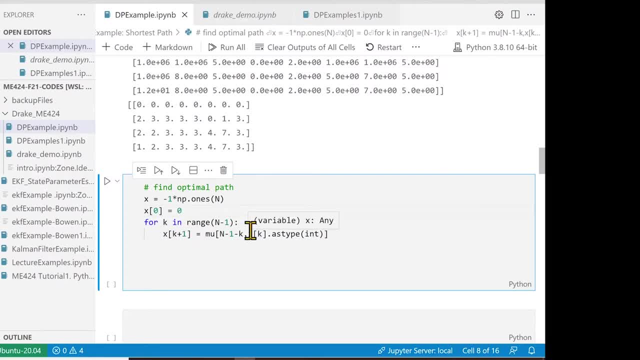 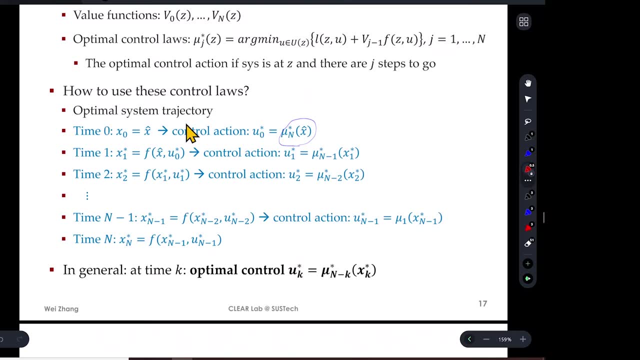 Start from zero, the first- then you need to apply your optimal control law. If you look at the math, the optimal control law right. You start from time zero. you apply the n-horizon optimal law. that means the optimal control action you need to take. 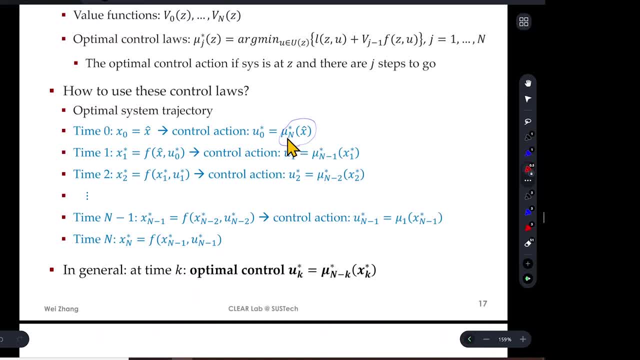 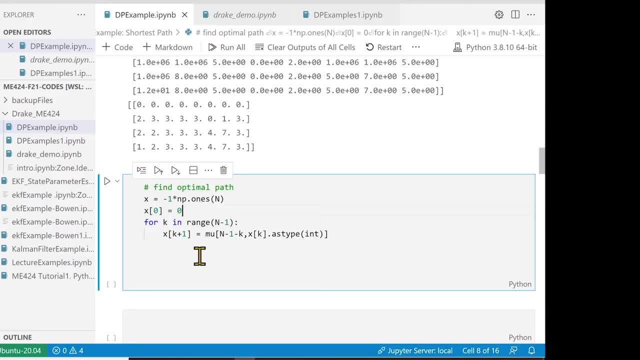 when you're at this state there's n horizon left, Okay, and then you apply that. then you go to n minus one horizon left, things like that. You apply this. so that will be because our f is just u. 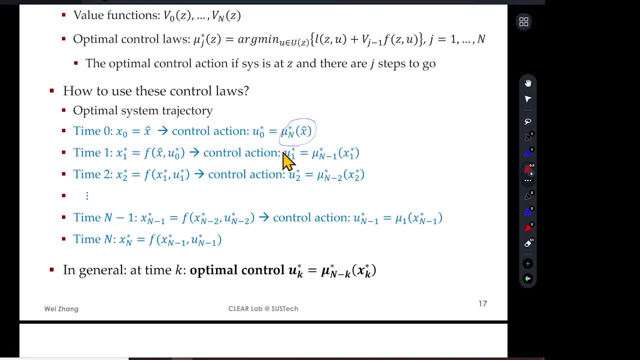 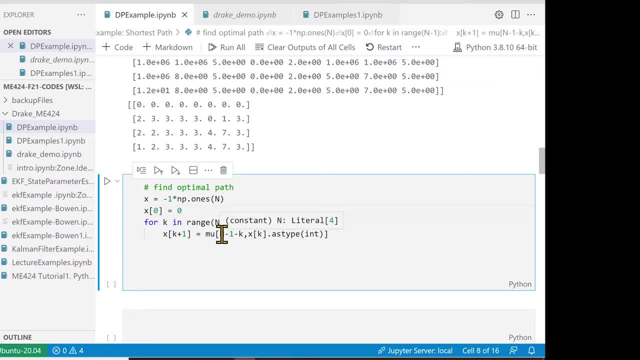 our f function is just: you directly control your next step, next control state, next state. So that will be mu k plus one. sorry, x k plus one is mu n minus one minus k. that's the. if you check, you can check, okay. 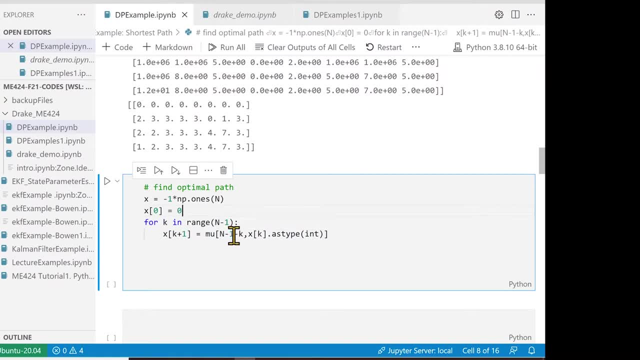 if k is zero, that means you have n minus one, that's n, right. So Python has index. that's start from zero. So that means n. So you have n horizon left. then at this time you are at xk, at least xk. I think I need to use this. 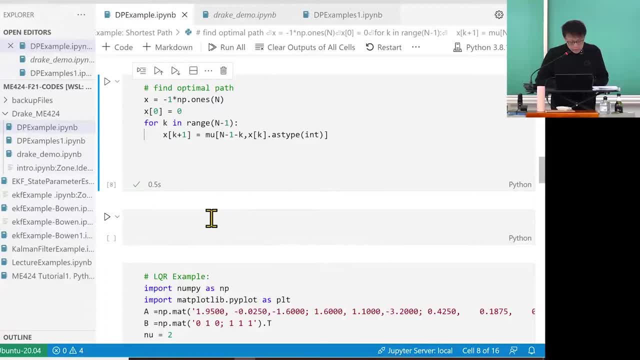 Right, let's state So: I apply this, it works. then, if I print my optimal control trajectory, what is it? Okay, zero, one, two, three. what's the optimal path? One, two, three, four, that means right. 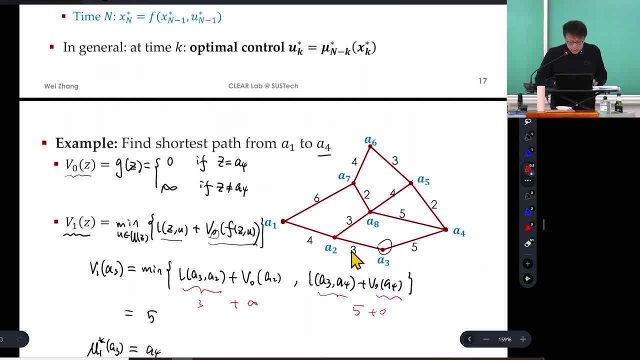 So that means one, two, three, four. this is what is it- seven, 12.. If I can go, there's also 12, right, This number is bad. Hold on if I change this to six. 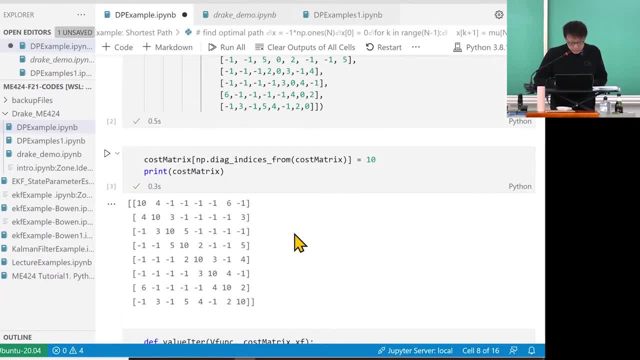 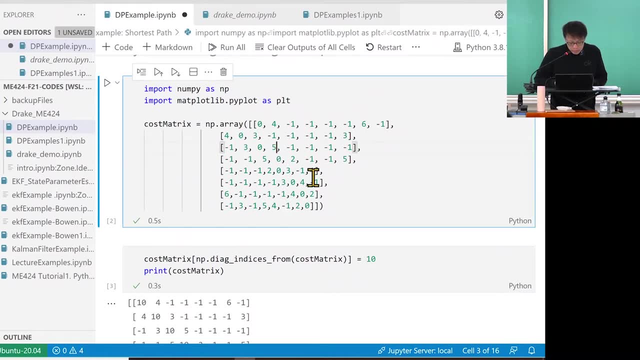 three to four to six. let's change that right, Let's change it. Can I do this? One, two, three, four. that means six. One, two, three, three to four. it's this: one, two, six. 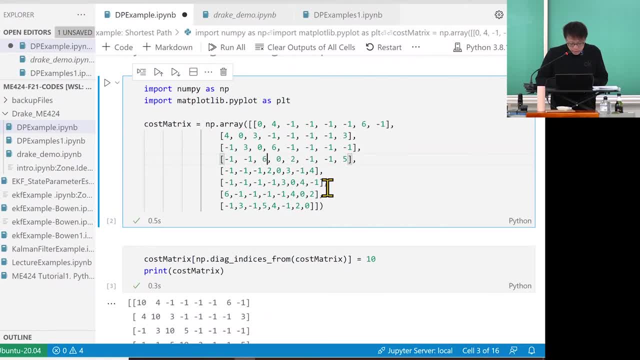 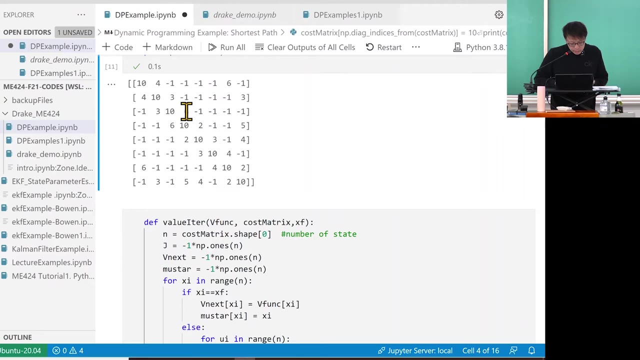 and four, two, three, this one right Six, Isn't it? Yeah, Symmetric, Symmetric. Okay, if I run it. if I run it, let's see: Three, two, six. three to four is six. 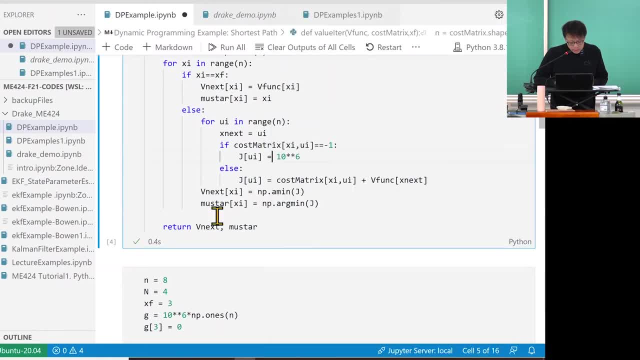 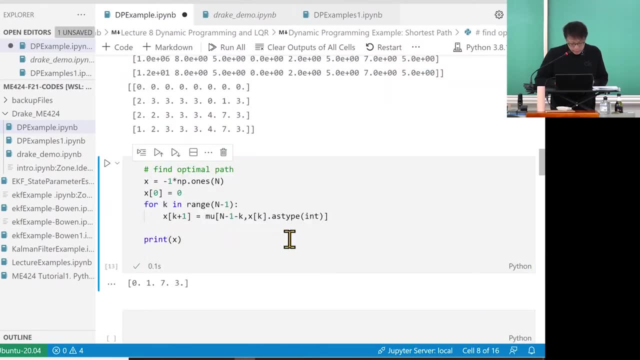 Four to three is also six, right, I don't need to rerun this. I don't need to rerun this And this guy. then I have different sequence now. I don't like 0,, 1,, 2,, 3.. 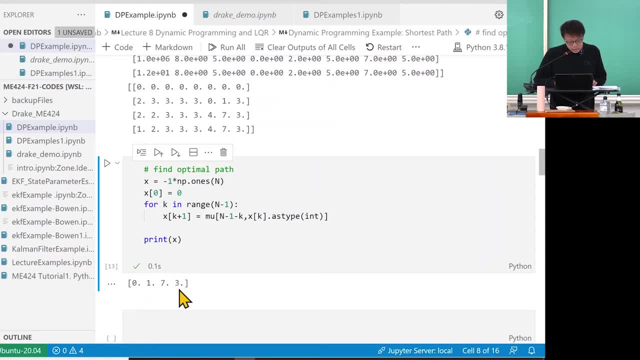 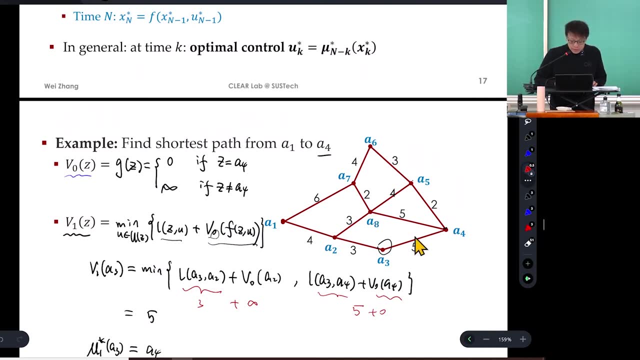 It looks like cheating. So 0,, 1,, 7,, 3, why is that? 0, 1 means 1,, 2,, 8,, 7, right Three, because this guy is six now. 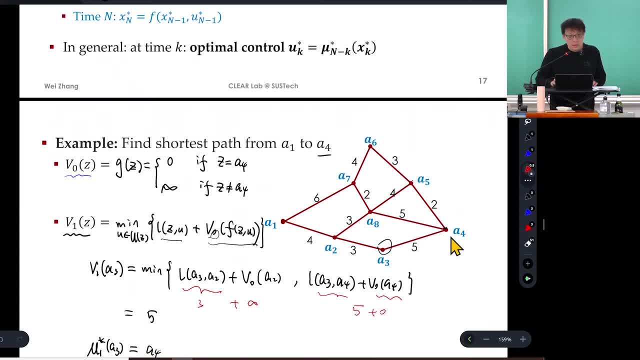 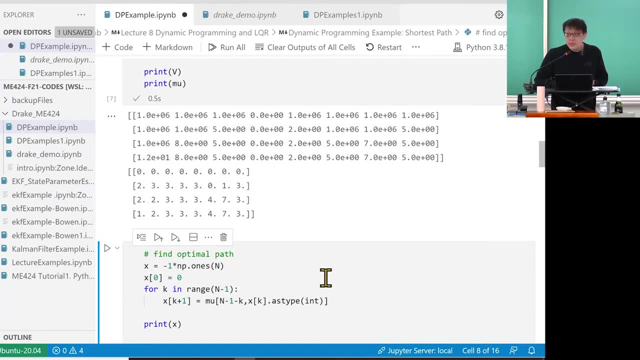 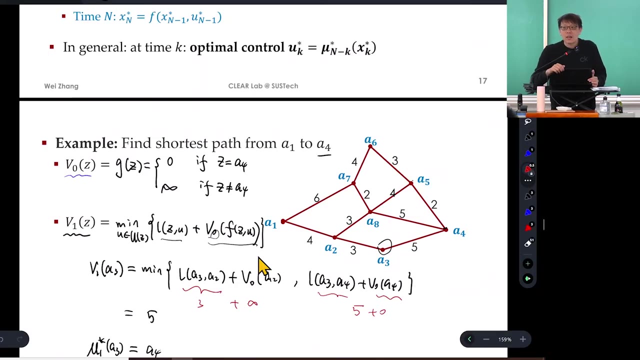 The optimum path is this: They'll automatically find this. I think this. I can upload this code for you and you almost have your code base for your homework. I want to save your time. Any questions? No questions. okay, Let's try to learn the LQR. 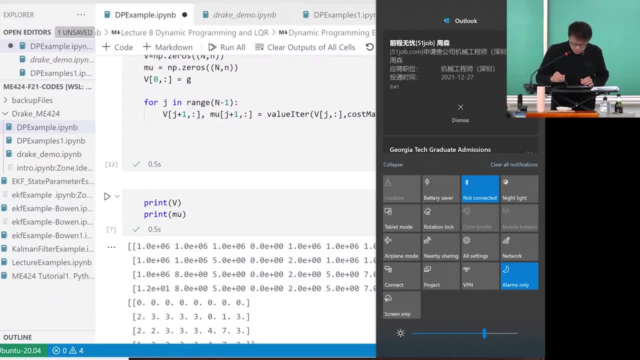 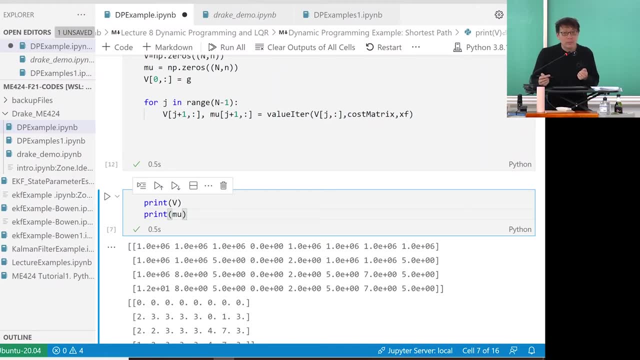 And it's very important, almost one topic, It's the most important topic for after a common filter. all we want to do is LQR, but it's similar to common filter. I spend a lot of time. do the background then become common filter, become just linear Gaussian? 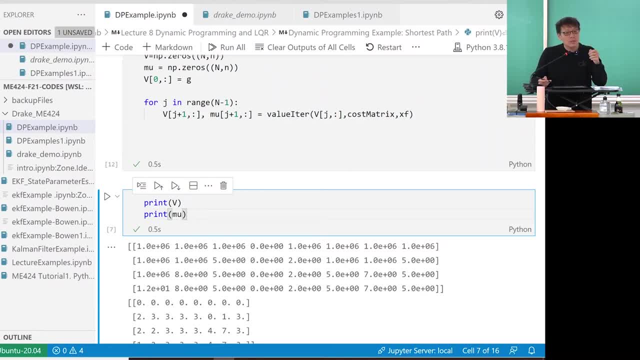 estimates and minimum in square. If you know all these foundations, common filter, you can derive very easily- And similarly in LQR we're just trying to know a special case of DP. Nothing changes, all right, It's just. the I function is linear. 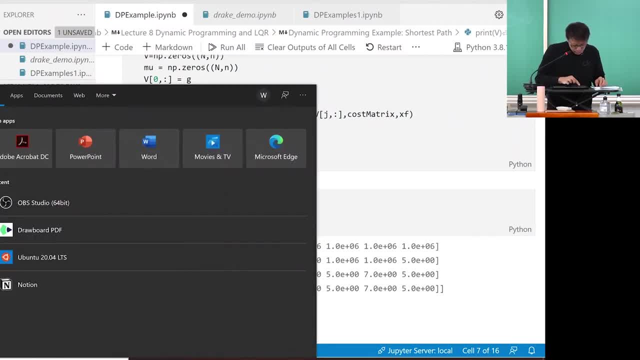 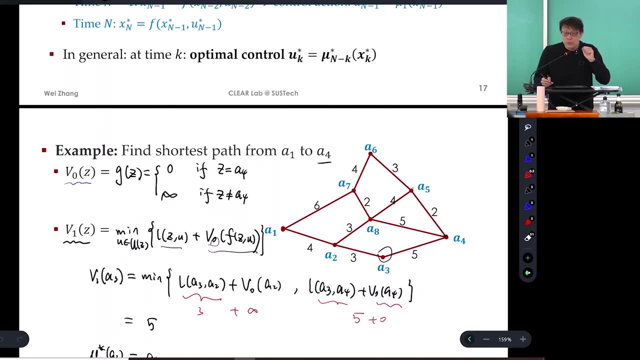 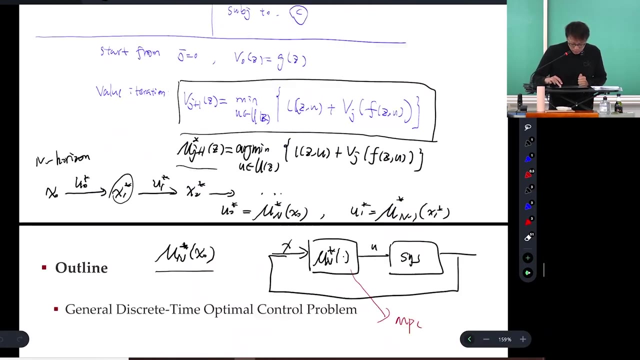 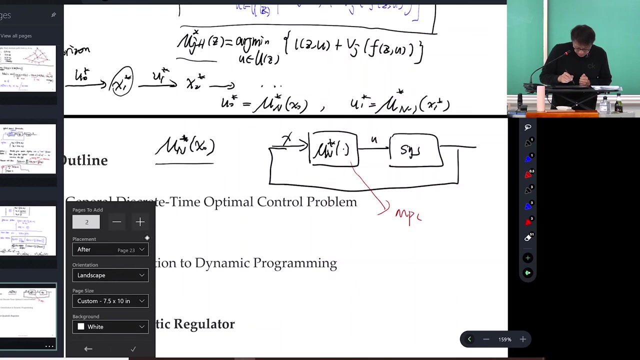 And Oh I. function is linear and also cost function has a special structure. so you have a analytical form for the bad iteration. okay, If I want to repeat or I have to add to this point, I need more space, Do this. 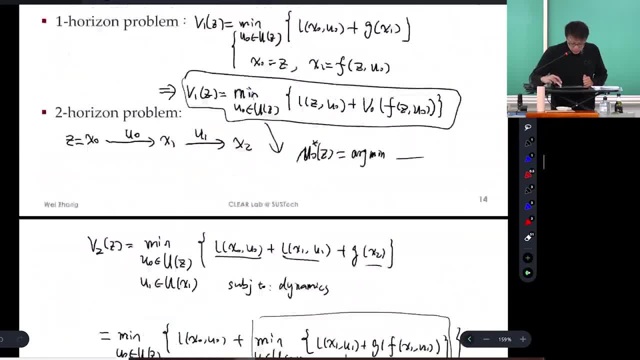 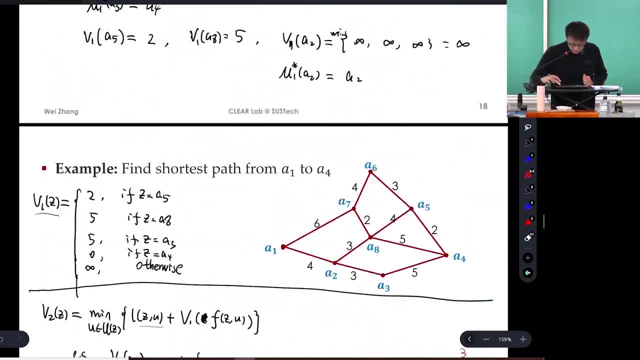 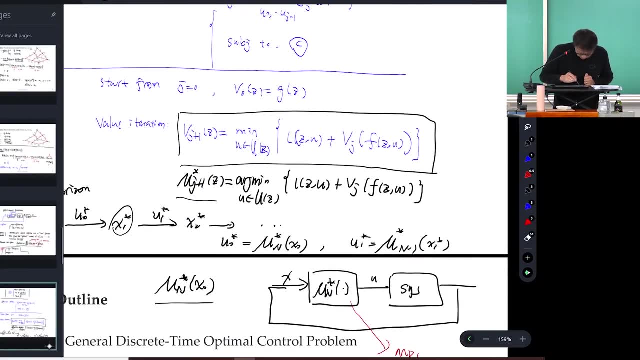 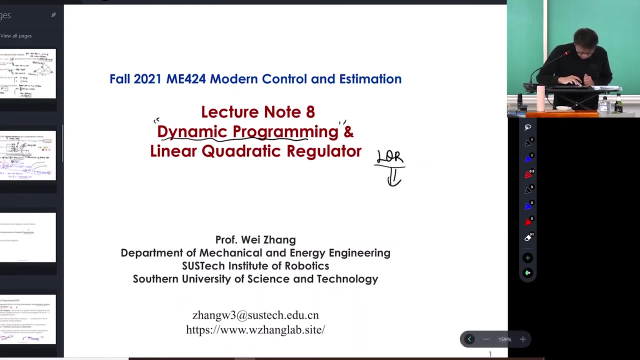 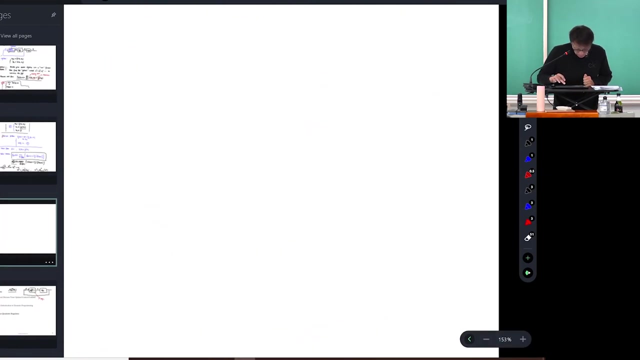 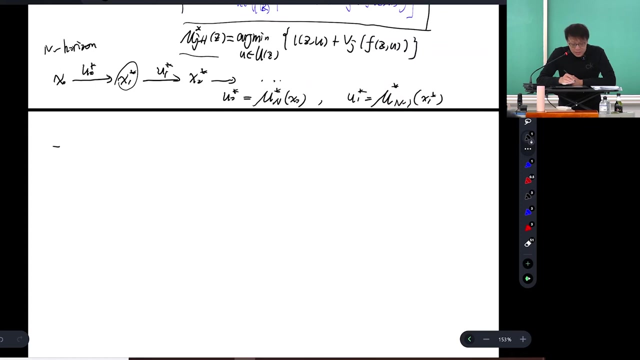 Where is it Okay? Hmm, Here. Okay, Hold on Insert page. Okay, DOециMENT. So based on our coding, you can see that for that case I need to enumerate A1, so it's 1,, 2,. 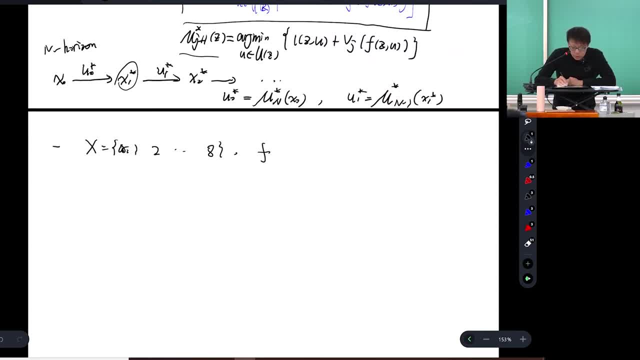 all the way to eight numbers, right? So I need to do our for loop to enumerate all this, right? But if I have, let's see, I have a line, This is a binary, okay, So for each line, this is a filter. 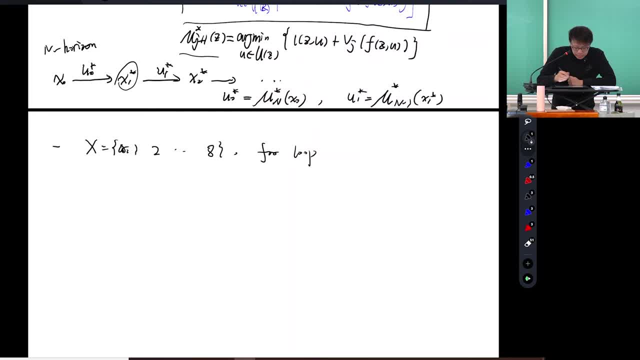 Hey, this is my translation, Sorry, excuse me, Sorry, excuse me, Sorry, Sorry. This is discrete, this is small cities, right? So if I have a line, let's say my state space is r. Let's say not r, my state space is temperature. 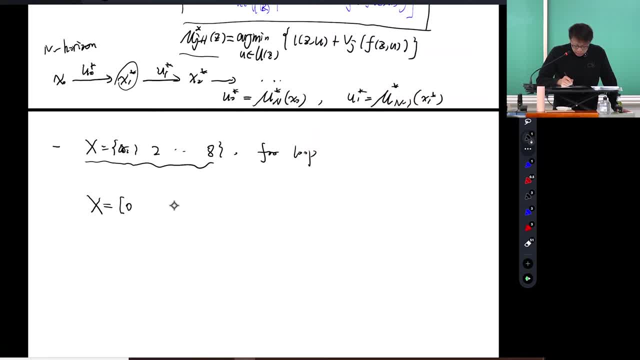 St John temperature. let's say today is pretty cold. Zero to 35, that's not true. Zero to 40, okay, Suppose that's my state space, suppose. okay, This continues. how many states I need to enumerate? 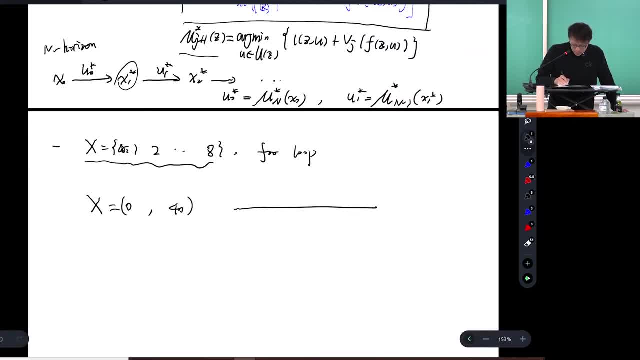 Infinite. Typically, you would do what? This is zero, this is 40.. You would do some tiny grading. this is called grading right, Suppose. I want to make sure it's pretty accurate. I'm grading with size, with grid size. 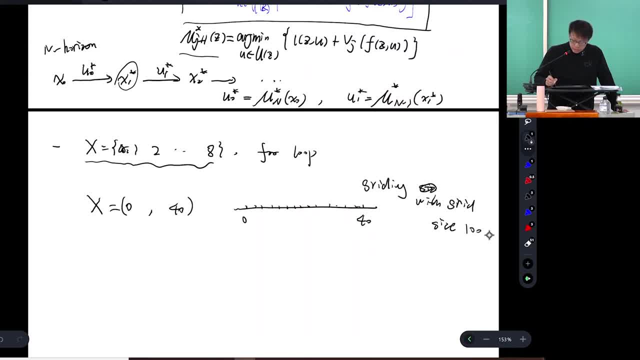 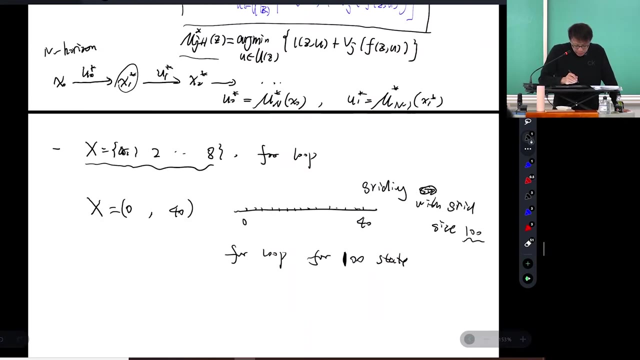 Grid size: 100, right. Then I need to do four loops for a hundred states, Values right From zero to 0.4, and so on and so forth. okay, So that's case, but this is 1D case. 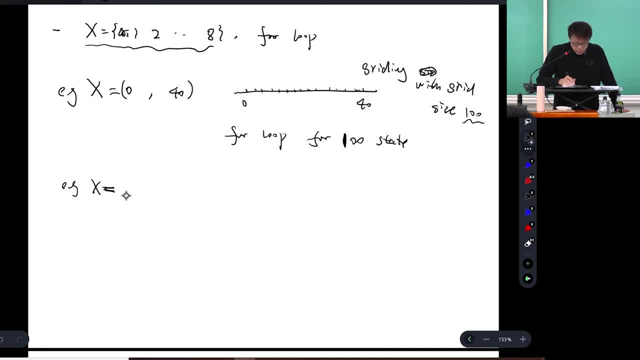 But if my state is St John, Guangzhou, temperature, maybe I can say: this is X1 and X2, two-dimensional right. X1 belong to zero to 40. X2 also belong to zero to 40, then I need to do grading right. 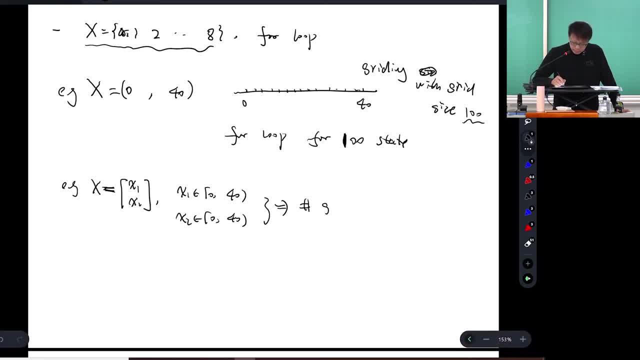 How many grades I need? Equal to 100 squared, which is 10,000.. I need to do four loops in 10,000.. Although I can solve- did I say that I can solve everything using DP or optimal control? 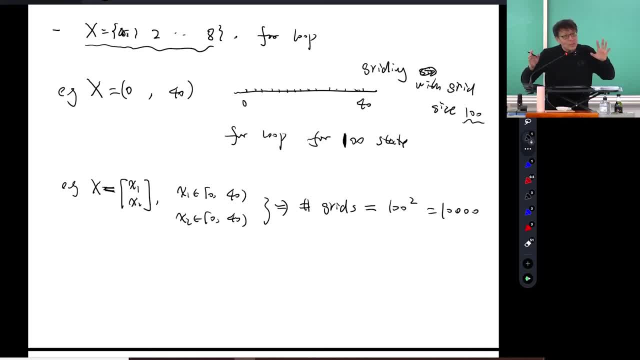 That's true, all right. The problem is that theoretically I can write everything in terms of optimal control problem, but when the state dimension is higher, complexity grows exponentially. Suppose I have X1, X2, X10.. Suppose I have 10 dimensional. 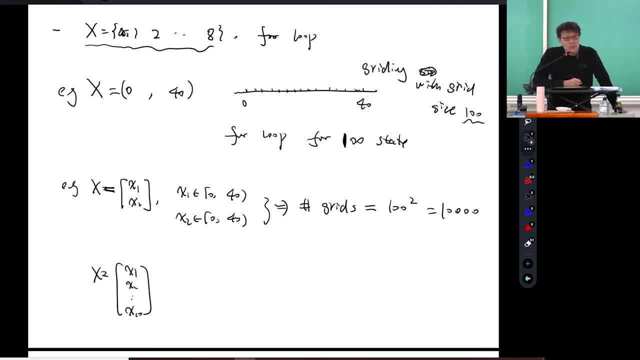 maybe a very simple aircraft or a simple dynamic robot, dynamic model. Then number of grades point. I need to do four loop. it's 10 to the 10.. 100 to the 10,, sorry, 100 to the 10, we cannot do it. 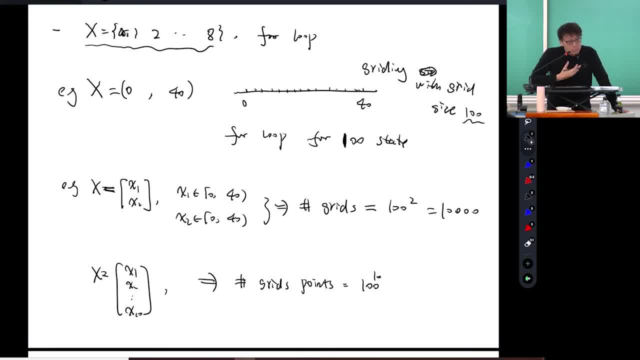 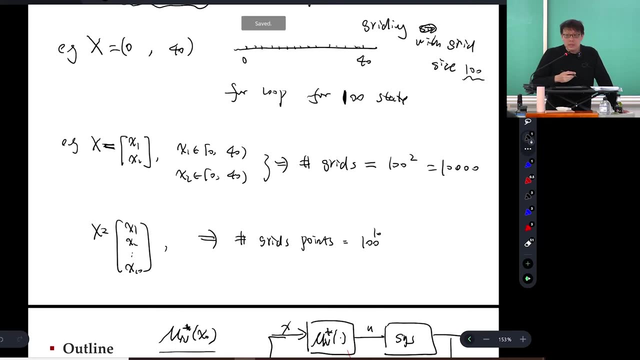 All right, I think current computer can do maybe up to five or six, But you still need to do it in a smart way, and this can only be solved offline. Okay, so you see the catch. It's not, of course, everything can be formed in this way. 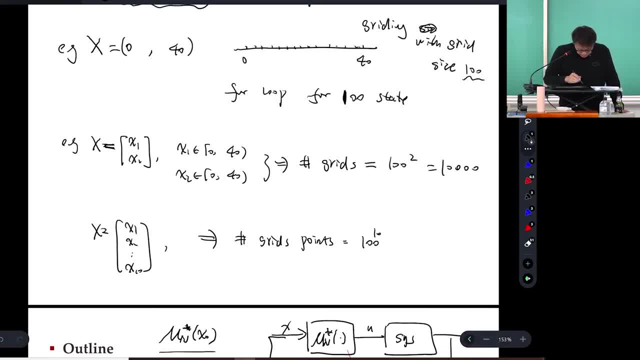 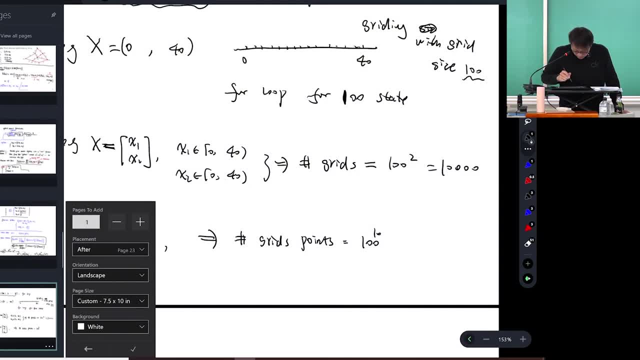 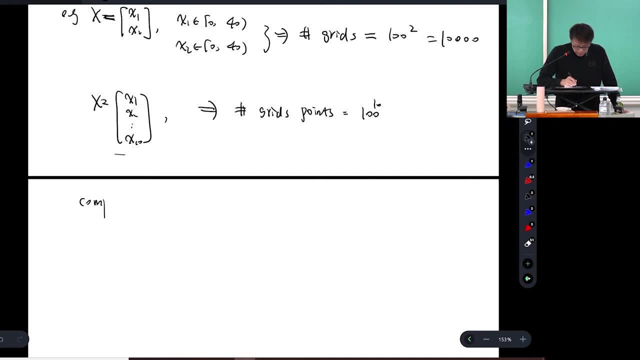 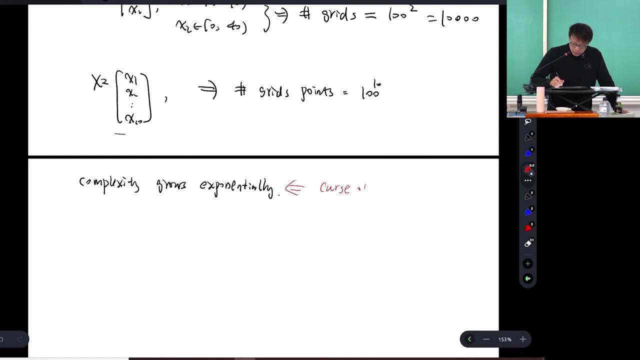 but we cannot solve it, Unless, unless- so it's this is called, so the complexity, I would say complexity- grows exponentially. Okay, this is called commercial and this is a famous term called. this is called curse of dimensionality. 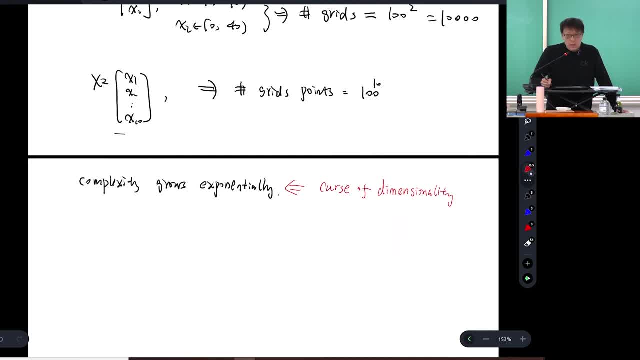 You have to know All the optimal control problems: reinforcement learning, Markov, decision process learning. they suffer from the curse of dimensionality problem, just like this: Okay, you cannot do high dimensional things because they suffer from, Okay, curse of dimensionality. 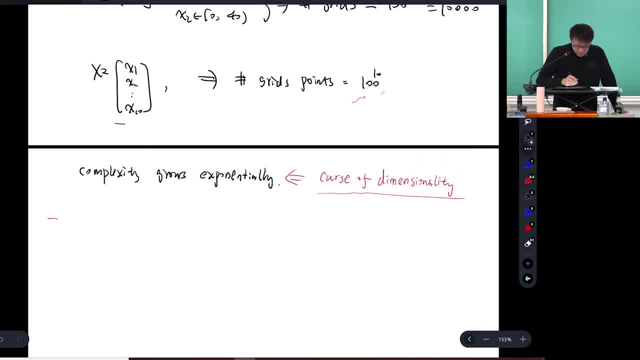 Okay, One last exception. So what we can do is, of course, discrete problem, that you may have 10,000 or 20,000.. Okay, computer can handle it, Just do four loops and code. write your code smartly. 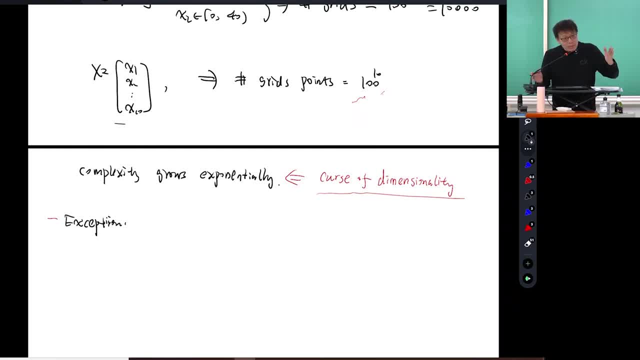 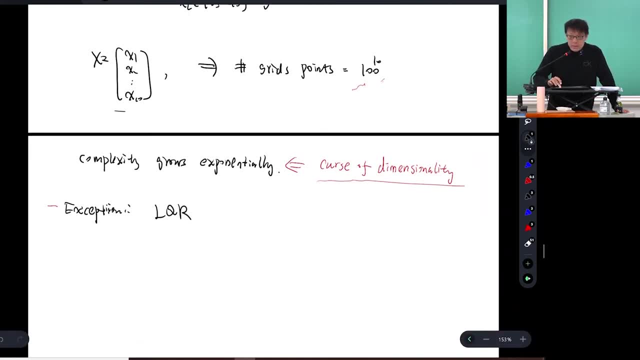 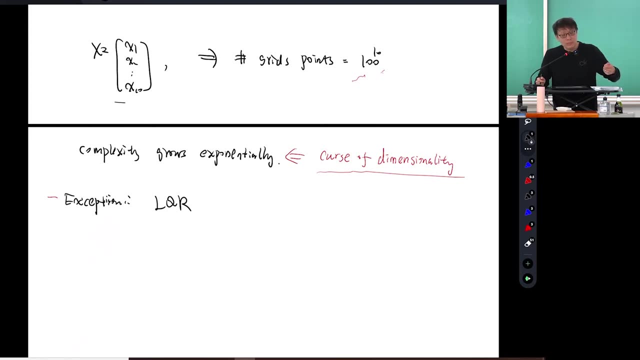 You should be able to do it. But in general if you have high dimensional state space, it's hard. Exception is LQR. That's an exception, It's not a standard long theory. I'll say this exception to curse of dimensionality. 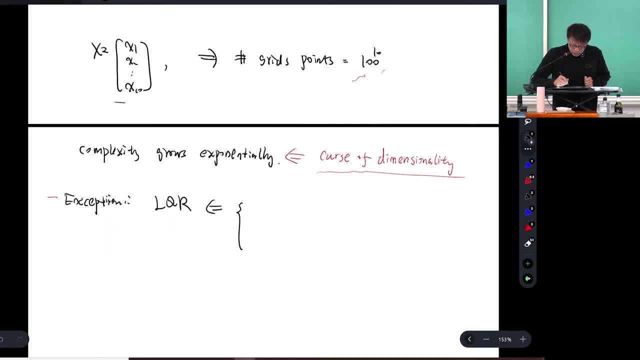 because no need to do grading. We have analytical form for value function and mu J star. Okay, the reason we want to do four loops is that we need to enumerate all the possible state and tell you, or compute, the optimal cost to go and optimal control action I need to take. 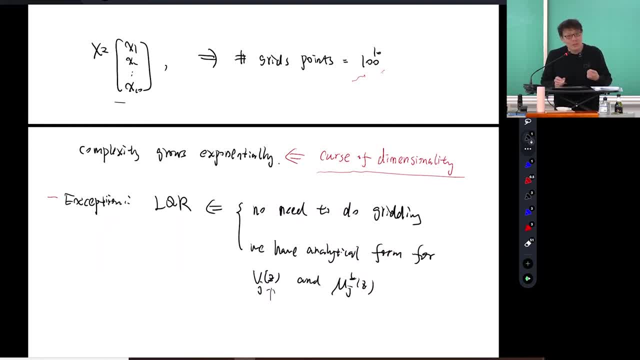 Exception means I don't need to do it. I can derive a formula for it, So I don't have to do four loops. Okay, that's LQR, And we are going to use 10 minutes to cover it Once you know. DP. 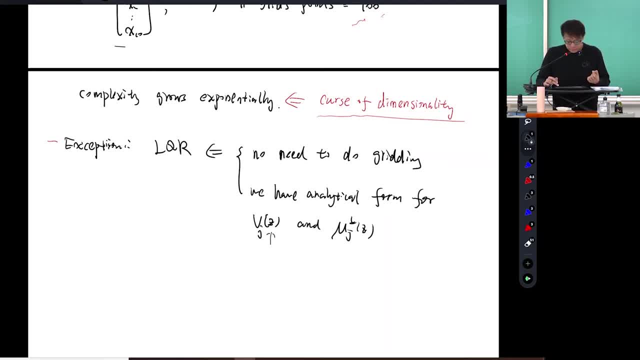 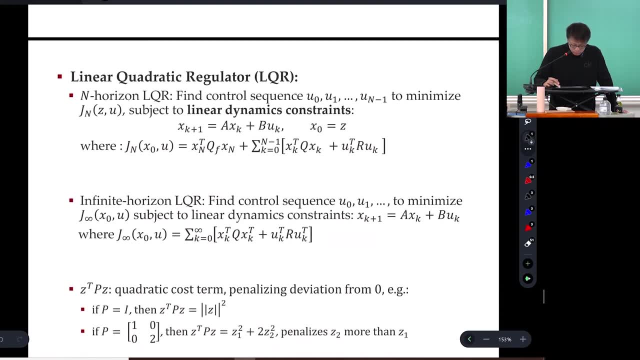 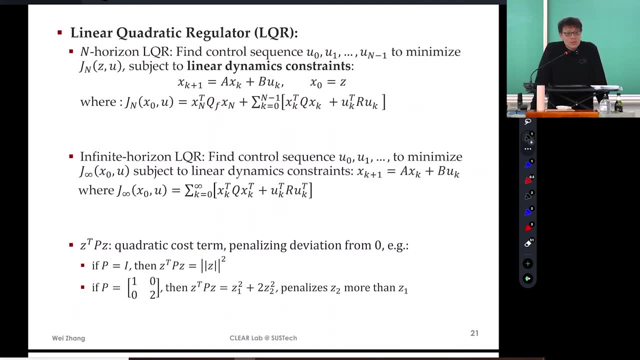 that's just the exercise. Okay, I hope that logic is clean. now Let's start our introduction to well, IOQR- linear quadratic regulator- Very, very important nowadays. When I was student, nobody use it Now because computer is faster. 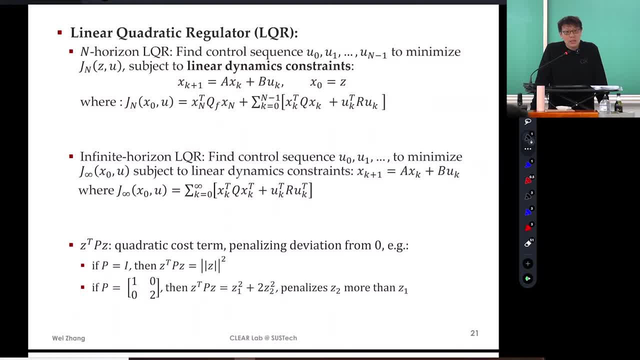 and the robotics people like to use it and it's become a standalone thing that everyone have to know, especially people in robotics. Okay, and first of all I want to emphasize: IOQR is the same as Kalman filter. The formula are the same. 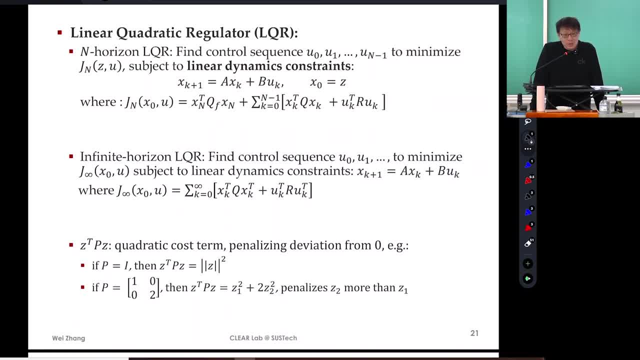 The optimal feedback gain is Kalman gain. It's a dual problem. Okay, it's like a. controllability versus observability is dual And LQR is the dual to Kalman filtering. Okay, we wouldn't cover that, but the formulation is like the following: 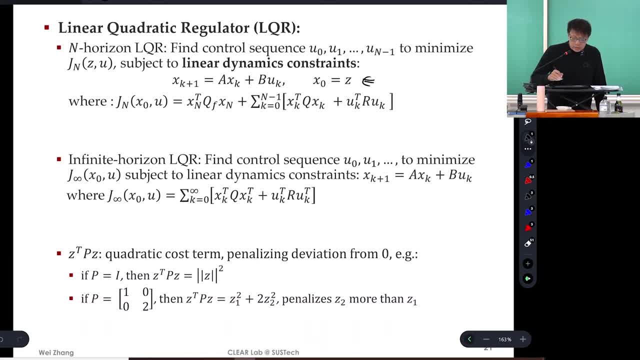 Before we have reviewed optimal control problem right. So before we have general optimal control problem like this. now the difference is what The? I have become AX plus BU, that we focus on Simple, right, Deterministic and also linear In both control and the state. 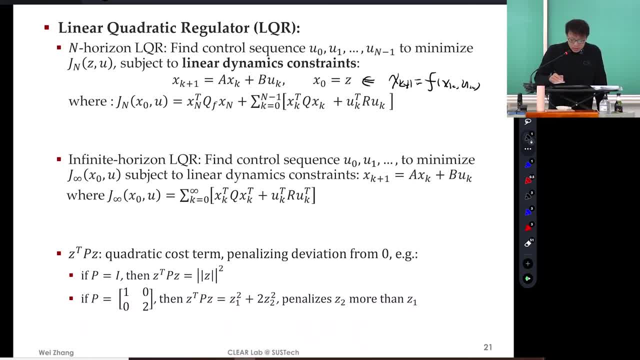 And before the cost function is arbitrary. This is my running cost now. It's a quadratic function of state and the control. Any questions? What does this mean? So this is running cost and also terminal cost. This is my G of XN. 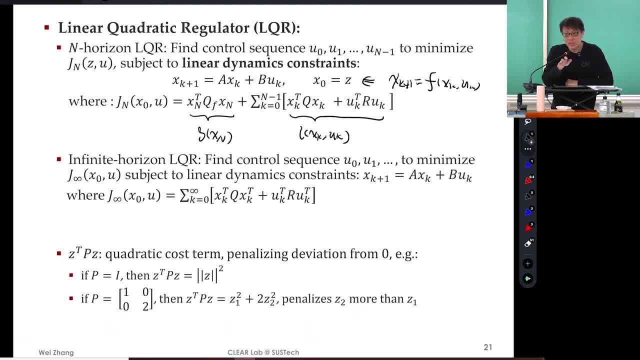 So LQR is just a special case of non-linear control. sorry, optimal control, of course. So this is G of terminal cost. Terminal cost is a function of it's a quadratic function of the terminal state. Why we like quadratic function? 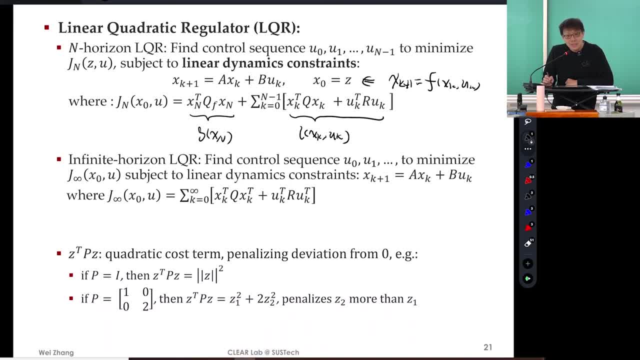 Because we can solve analytical form for it. It's like a least square Okay, So it's no Y, okay, It's just. this way Can capture our objective to a certain extent And also the benefit is that we can have analytical form. 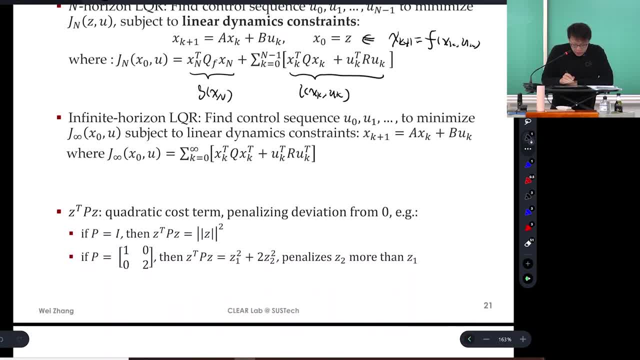 for the optimal solution. Okay, So quadratic function. I think I can just briefly mention it again. So this is Z transpose P of D is a function from RN to R. If you give me a state, I give you a number. That number is a so-called quadratic cost terms. 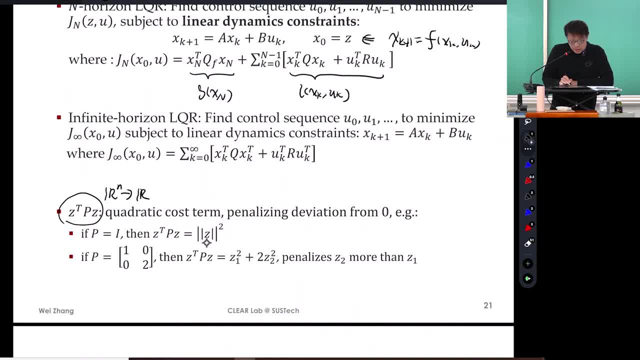 So if I choose my P to be identity, then this is nothing but the norm of the Z. Okay, If I pick it, this is just norm. Why I want to minimize the norm? Because I don't want it to be large. 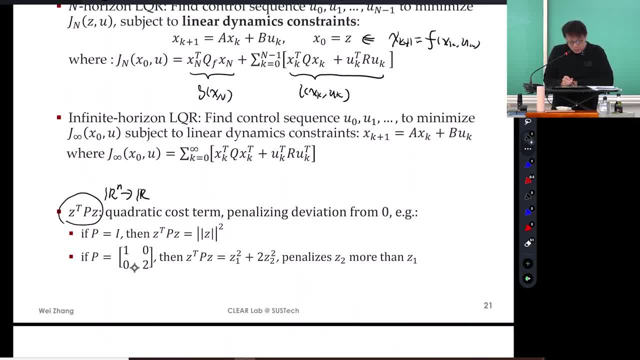 Okay, If I pick it to be diagonal, but one coordinate is bigger or smaller than the other, then I have. the form is like this, If you just multiply things out. So Z is Z, one, Z two. right, If Z transpose P, Z. 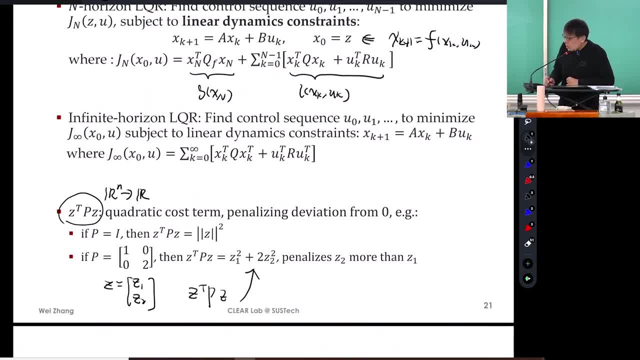 will be just this. So what does this cost? means? or indicate You penalize X two more, twice at the large as X one Z one. So the second coordinate is more important. I want it to be small, Okay, So that's all it means. 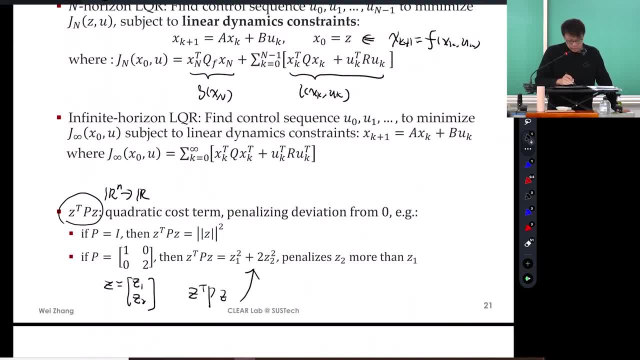 We allow you to. in general, it could be just anything that is positive, semi-definite. It will be valid for a quadratic cost function. Okay, So I want to. so the goal you can see from this LQR, the goal is to use small. 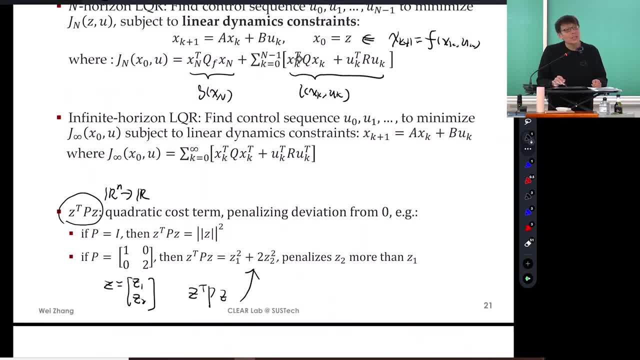 control, action or effort to make your state convert to zero. That's why it's called a regulator And a state in general. as we mentioned before, we want them to go to zero. That zero is a code, and code zero means your desired position. 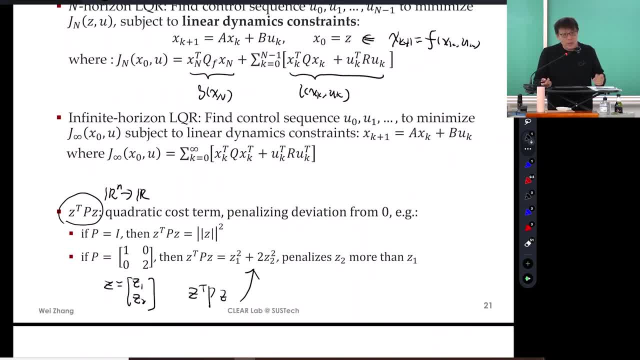 your 60 miles per hour. your set 25 degrees of degrees, Okay. So that's whatever desired value you want. You call that A the origin, then X is D, B- Okay, So that's the division from that, Okay. 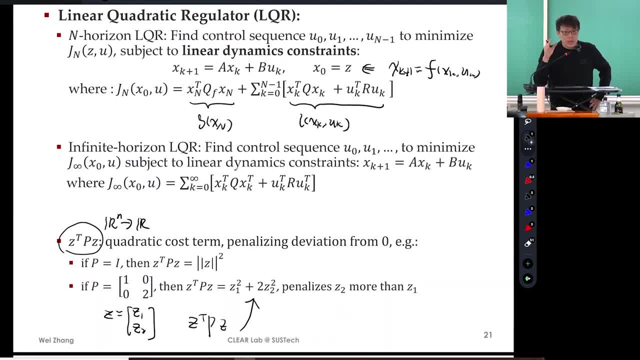 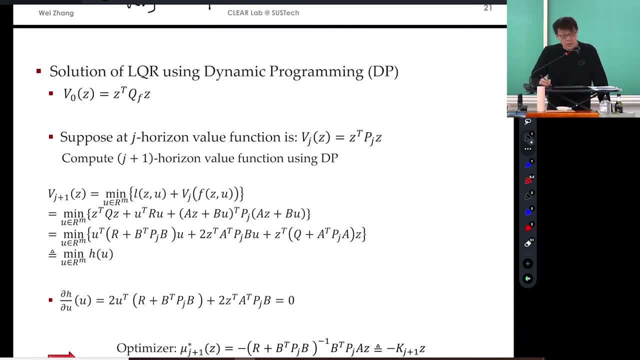 Any questions? We have the same formulation. It's just a specialized in linear system and the quadratic cost. That's why it's called linear quadratic regulator. Okay, To solve it, what we do is D P. What is D P Internally? 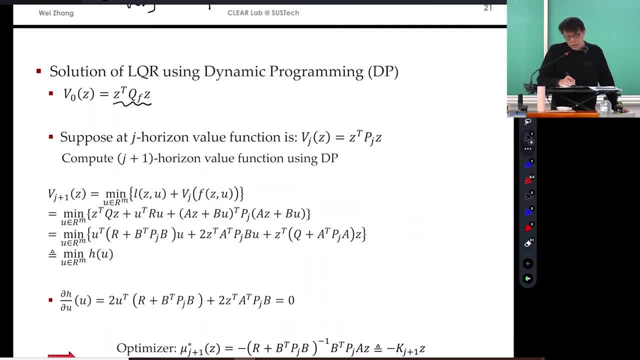 initially, what we have is terminal cost. What is the terminal cost? G of X, N right G of Z? Z is a dummy variable. Okay, It's representing the function. So what does this mean If you have zero horizon? 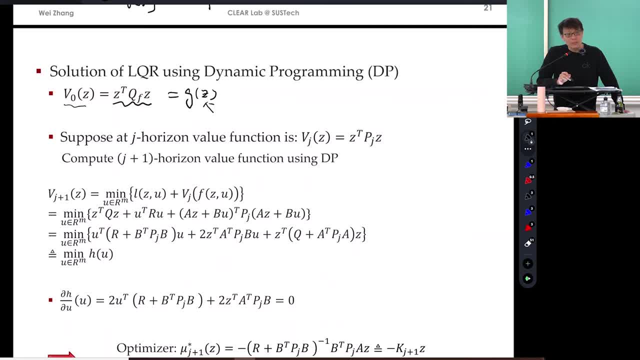 that means you don't have any time to leave. Then you are at Z. that's your cost. Okay, Terminal cost. And now we need to do value iteration right Before we just do value iterations through four loops. But now for linear quadratic regulator. 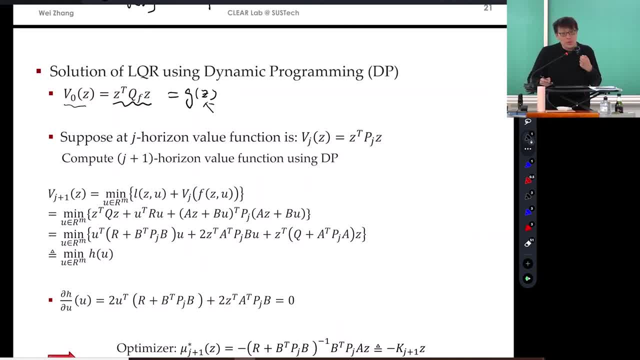 we somehow can find the optimal solution analytically, because it's just nothing but a minimization problem, And in this case we have an analytical solution that's similar to least square. I think right And I make a conjecture. It's not, I make a conjecture. 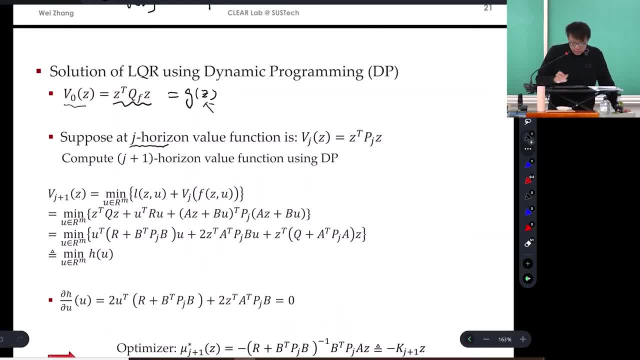 Let's assume first of all the J horizon problem is of this form. What is this form? A quadratic function? Okay, Suppose my J horizon cost function is a quadratic function. It holds- For now we know- for J equal to zero already. 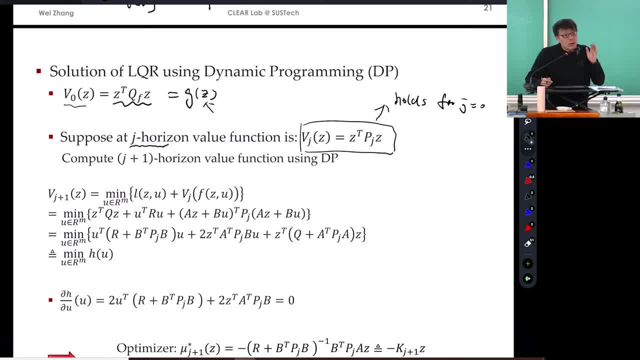 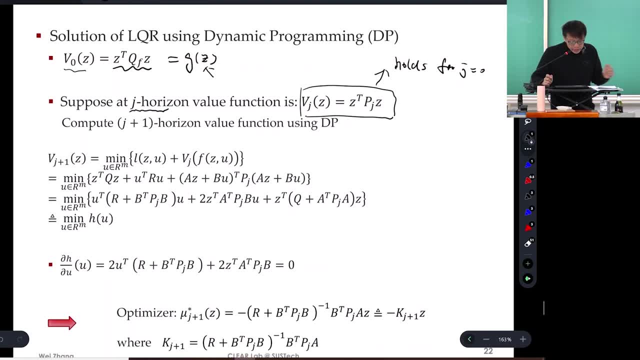 Right, Let's assume it holds for J And we want to prove J plus one is also a quadratic function. Okay, So now let's derive it. So let's say VJ plus one, Z is of this form. So what does this form mean? 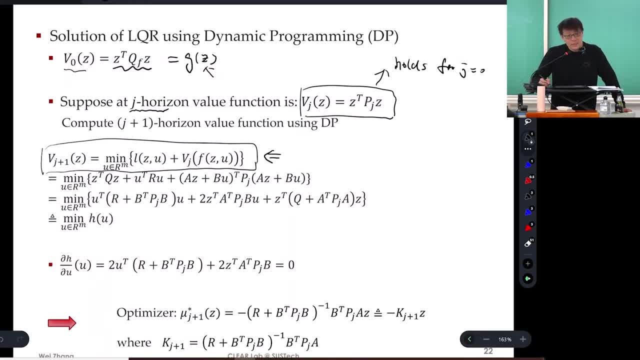 What is it called? Is this something special to LQR? Is this DP Similar? How similar? The same right. This is called value iteration. Okay, This is value iteration, Exactly the formula I gave you before, Because now L is what. 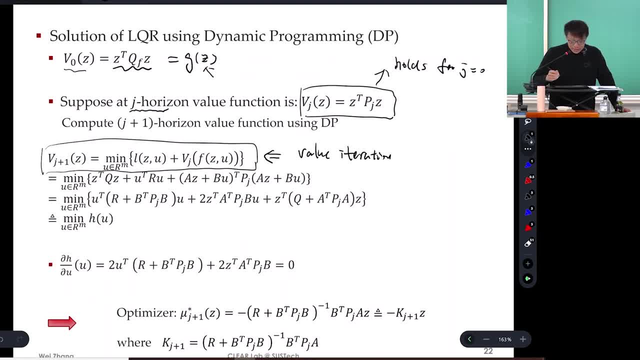 L is the quadratic in Z, quadratic in U. This is the running cost, Right, As I mentioned before, this is my L. L is X, K is transpose. Q is X, Y is X, Y is X, Y is Y. 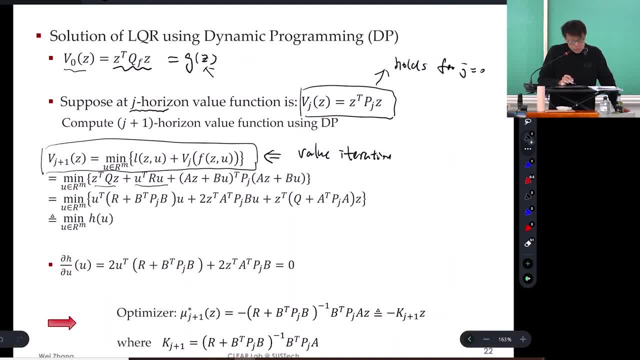 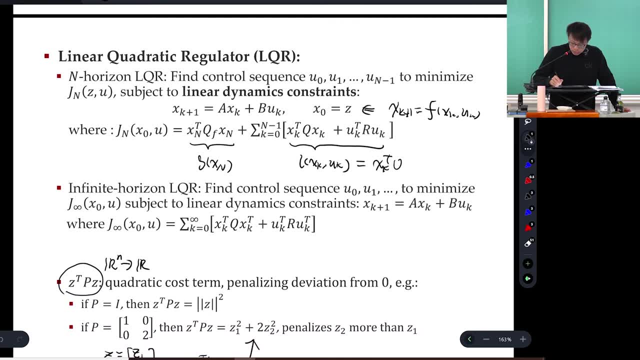 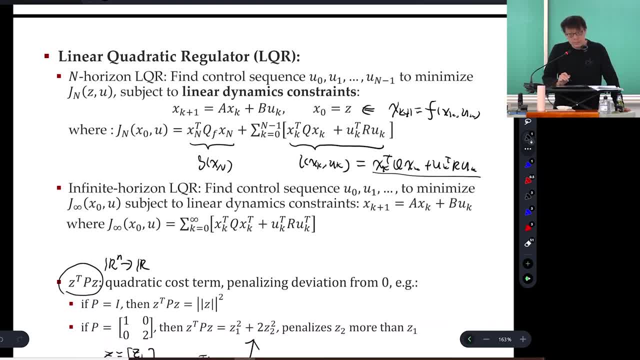 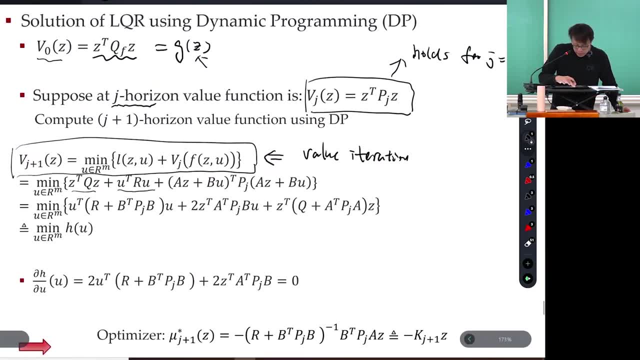 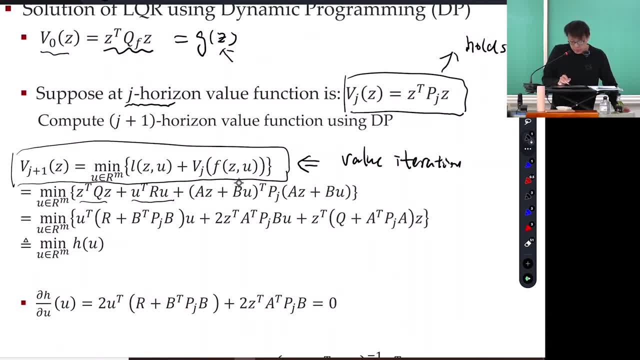 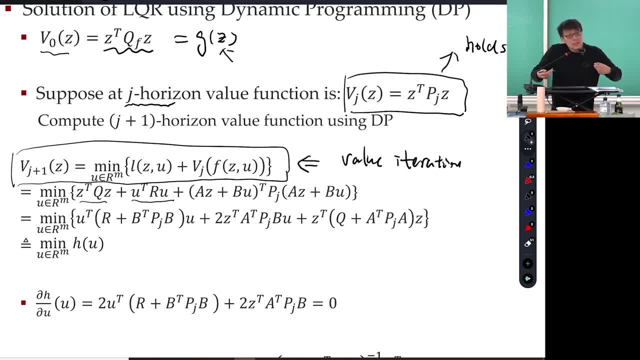 Y is Y, Y is Y. Assume at least from Jira we can do this right And plug in this. then I can group terms: Hopefully I think you can verify at home- And group terms. I can write it like this: okay, 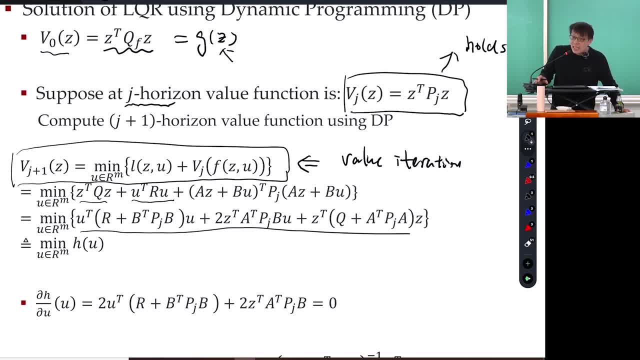 It's a quadratic function in both state. z and u control u And what we want to optimize, We want to optimize with respect to u, So I write it in terms of a quadratic function of u A. z is some kind of a parameter or constant in this case. 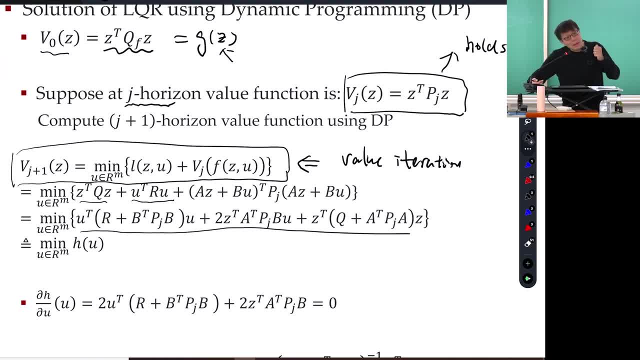 because we only optimize over u. We want to pick the best u such that this function is minimized. Okay, so this f x, u is just each u is just this function. In this case, what we should do is this: 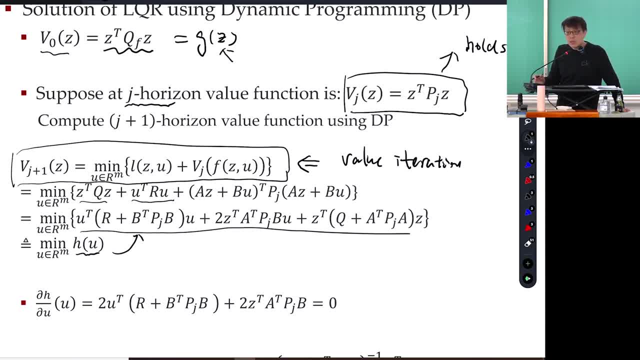 I think this is, in essence, is the same as this square. now, right, What you need to do is take derivative with respect to u. Okay, this function, h is from rm to r. It's a quadratic function, It's. you can write it like: 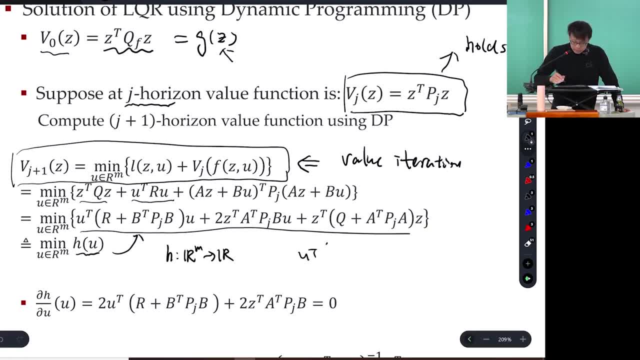 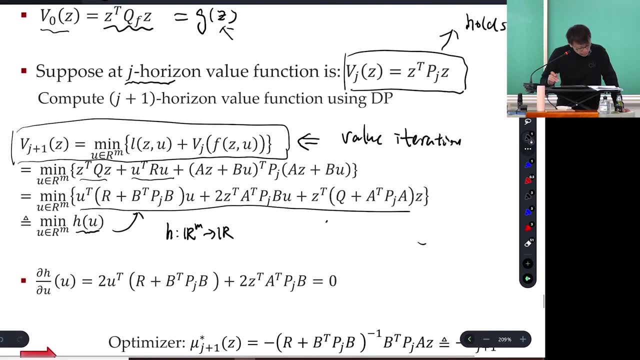 u transpose a quadratic function, That's a capital R? u plus something, a linear function of u. So anyway, that's this. You take derivative, it will become this, and let it equal to zero. You can solve for u right. 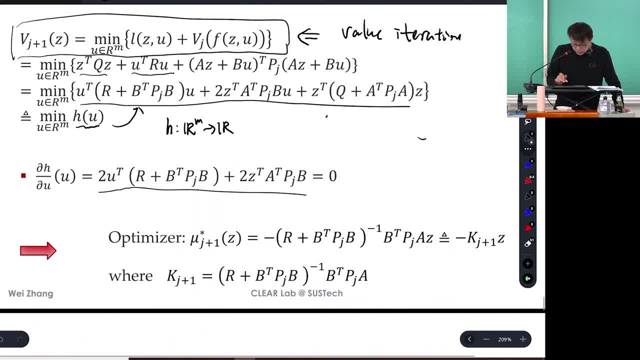 That's your take: derivative, And you solve it. That means you invert it over all you have. Okay, so you get this. So that means the optimal contraction at this time is some matrix, a lot of matrix, multiplied together times z. 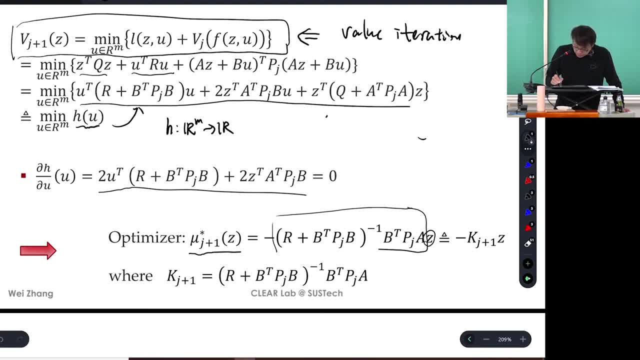 And I will call this guy k of j plus one. If you look at nature, it is a linear function of the state. Okay, it's a linear function of z. That's my solution When I solve this optimization problem. it's a linear function of the state z. 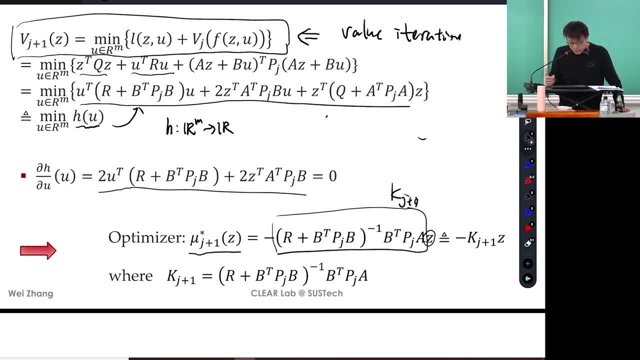 then that's my solution. Okay, you can go back to check. And this is I define it as a gain. This is a Kalman gain. Okay, This is the Kalman gain. It's like Kalman filter gain, it's the same thing. 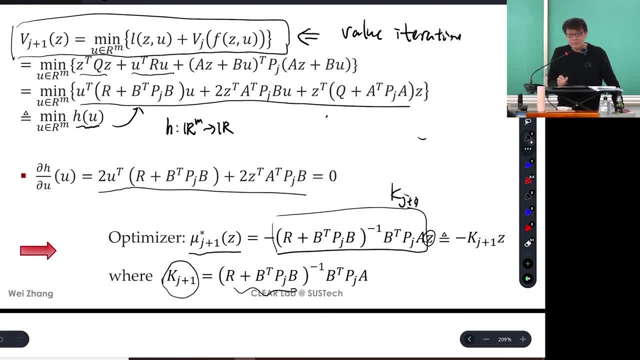 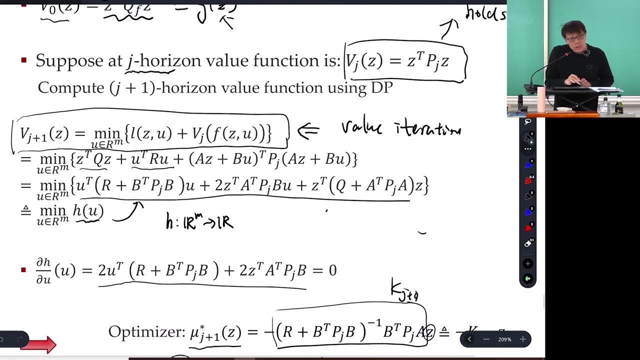 This is the covariance inverse, right? You remember? Okay, very interesting. Okay, any questions. That's your optimal one. Then I plug in this guy, right? So this is my optimal u, What's my optimal cost? I need to plug in my optimal u to have my optimal cost. 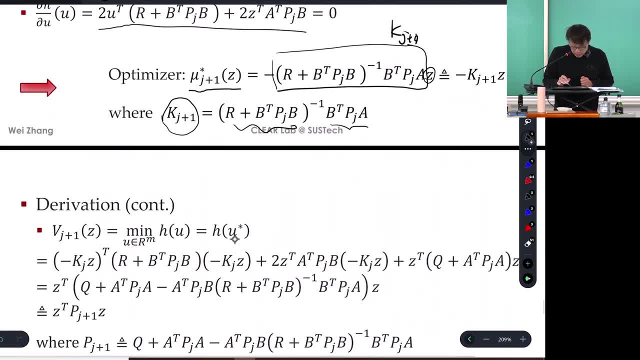 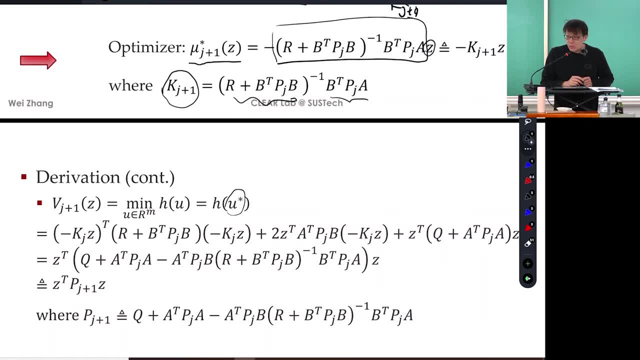 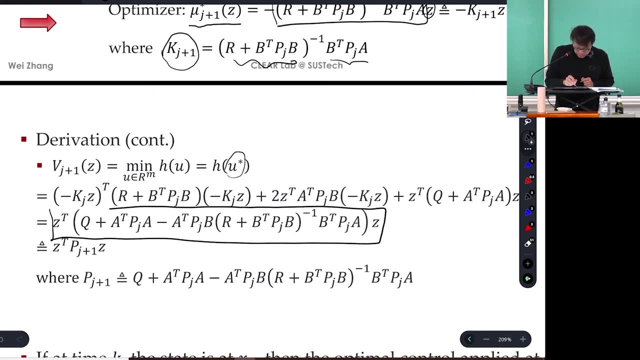 The optimal control. I plug in this, u star becomes this. I mean, after some kind of manipulation of those symbols, I find it out This is nothing but of this form. Vintia, is this a quadratic function? Yes, 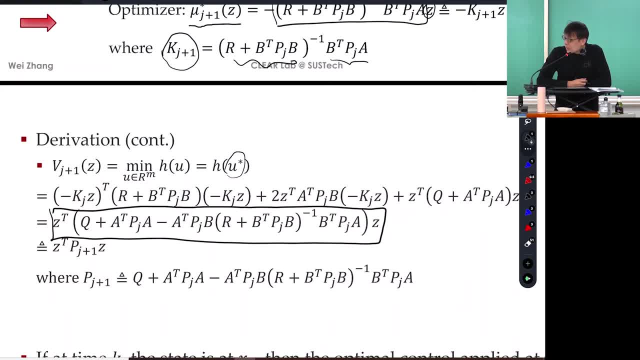 Of what Of z? Okay, although it looks complicated, I'm going to ask you: is this a quadratic function of z? Yes, It's of the form of this, And I can call this animal, this very complicated animal, my pj plus one. 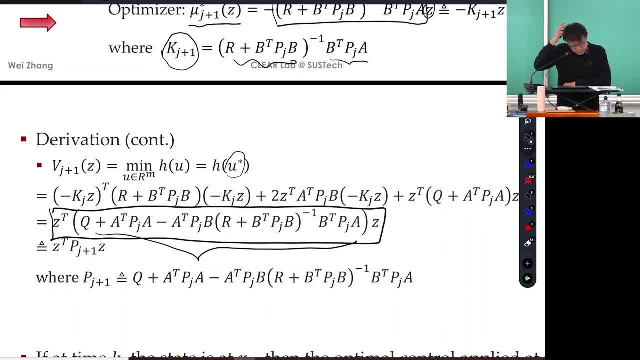 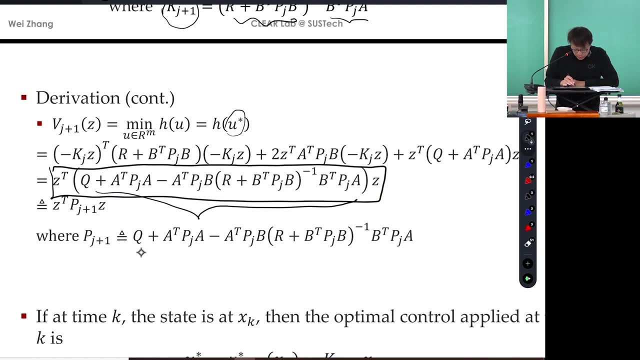 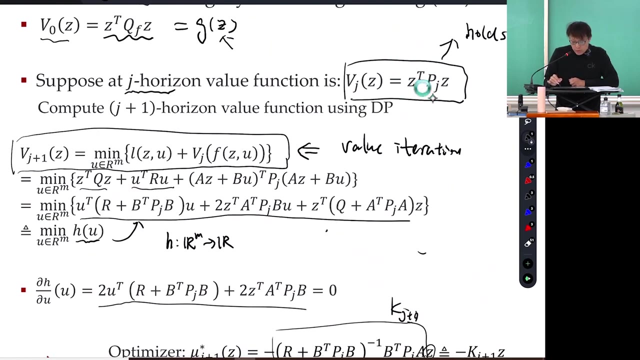 Okay, That's my pj plus one That relate to pj related to ab And also my cost function structure. And so this is now I, I I buy pj plus one. Validated my proof right. So if I start from a quadratic function, value function, next time 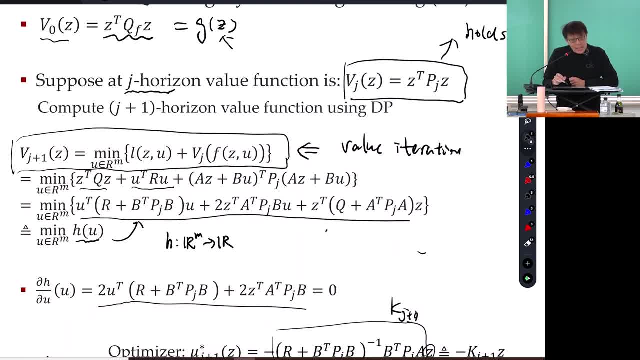 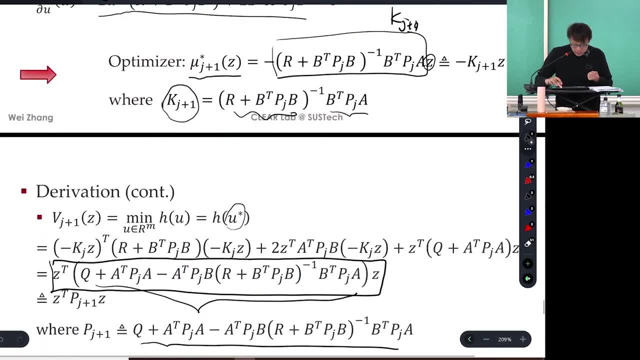 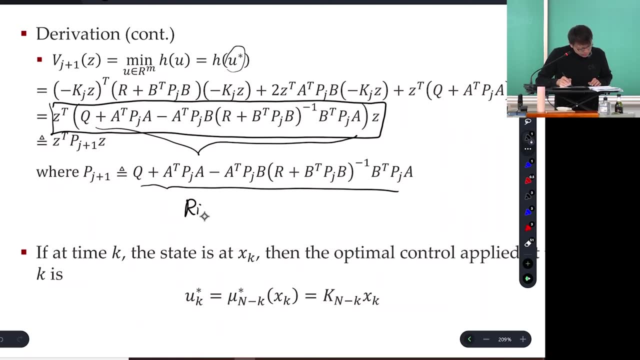 I will also be quadratic function and next, next time, I will also be quadratic function. It just this P Changes, right? How does that P change over time From this recursion formula? This is called Riccati, Riccati recursion formula. okay, It's not a Riccati equation, yet It's a Riccati recursion. 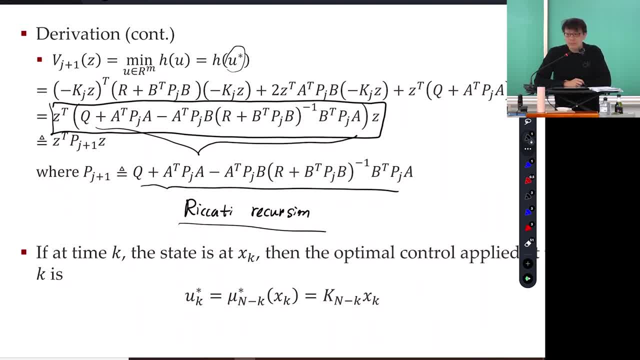 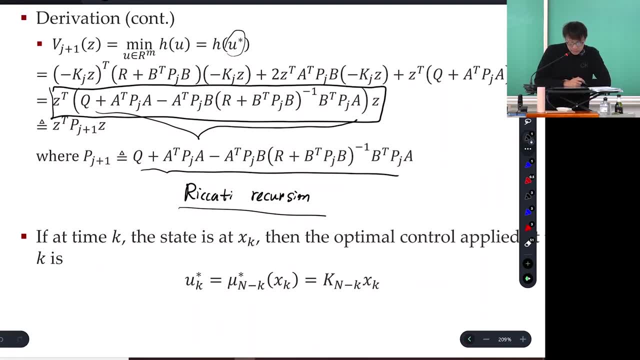 Riccati equation or the Riccati recursion is very Famous term in optimal control and linear robotics as well, And this update formula should be the same as common filter. the covariance gain, Covariance matrix. update equation is the same. Okay, if you pick your notation. 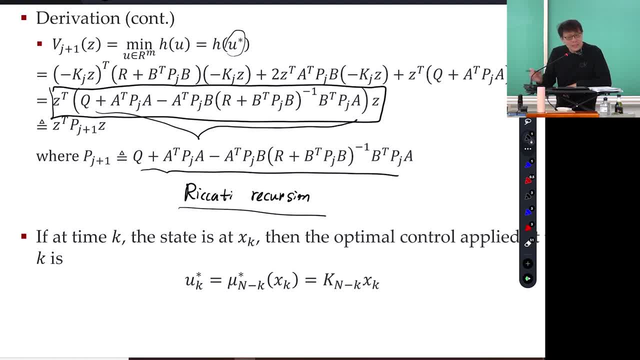 And they are the same. It's just like a B's observable, almost like right Controllable and observability, things like that. A B observable is a transport, B, transport of sorry, a B, a, C observable means a transpose C, transpose Controllable, things like that. All right. 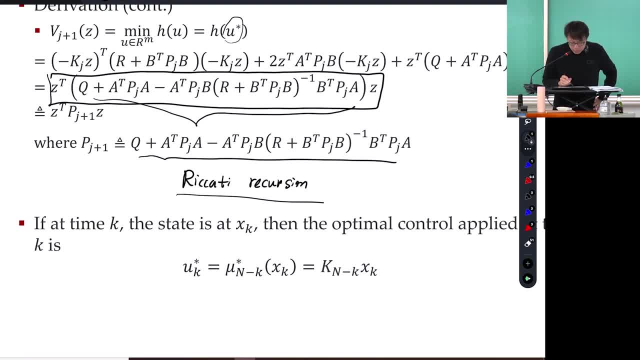 So The optimal control action you need to take, it's, It's just off this formula. It's- again- I think it's there should be a negative sign here Again- times the state. so it's optimal contract is linear and it's gain can be computed. 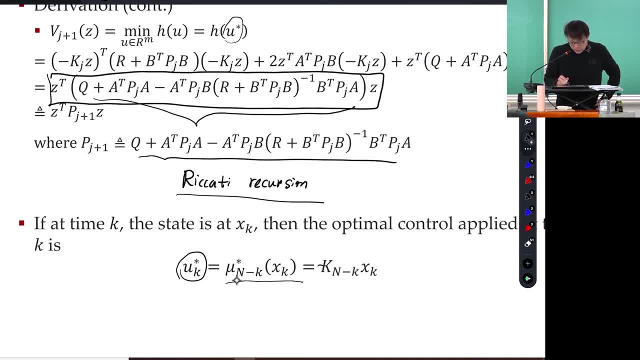 Okay, and this, this is so the meaning of this is the optimal control law you need to take, once there are N minus K steps left and you're at X K Right, and this is the optimal gain you to apply. and to compute this, you need to compute the Riccati recursion formula. 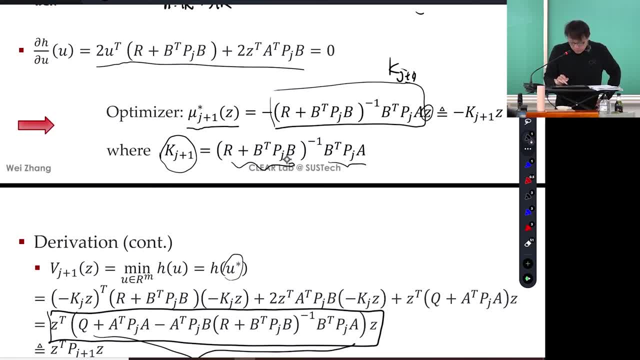 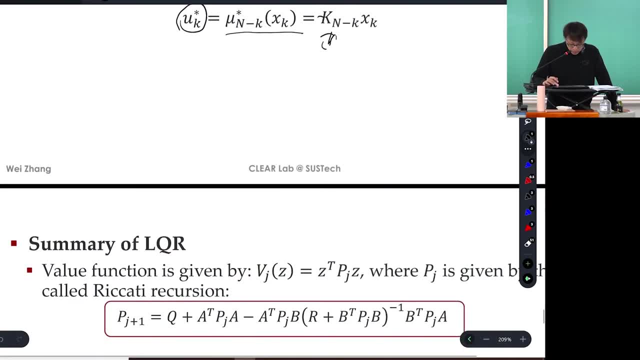 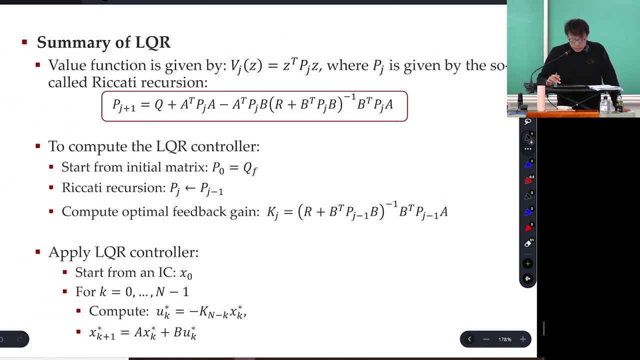 Which is J, You need to PJ. once you compute PJ, you can define K. Once you define K, you know what often I actually need to take. That's a summary. I wouldn't want to go over it in details, but how to solve it. by the way, 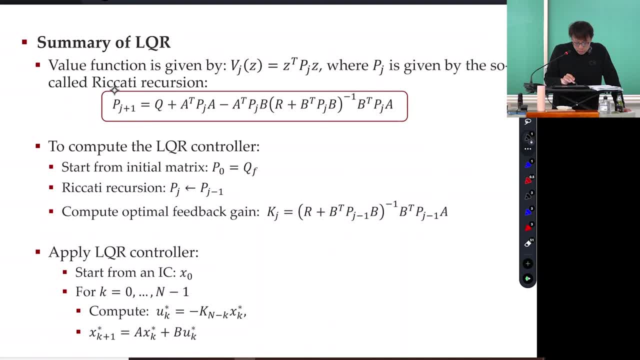 you just, You just do the Riccati recursion. you start from P zero. Okay, whatever P zero is fine Terminal cost. that's your Terminal cost function. Okay, P zero is nothing but Q in. You can pick arbitrary positive Simon and matrices and then you do the recursion. you have P zero, you have P one, you have P. 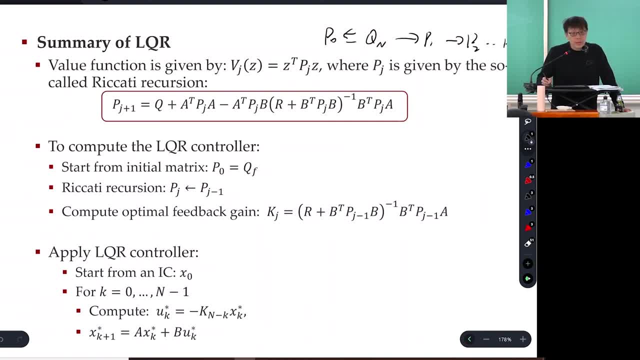 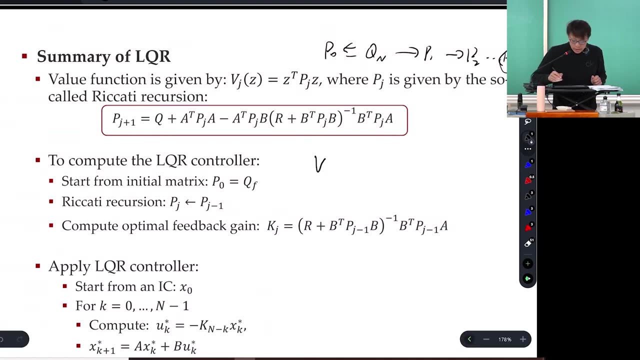 Two, all the way to P in. Okay, what does P and means Why we care about P? because we care about V. Okay, V, J of the. I Mean by the iteration. right, We do the shortest path problem. We do by the iteration. All we want to do is compute this guy. 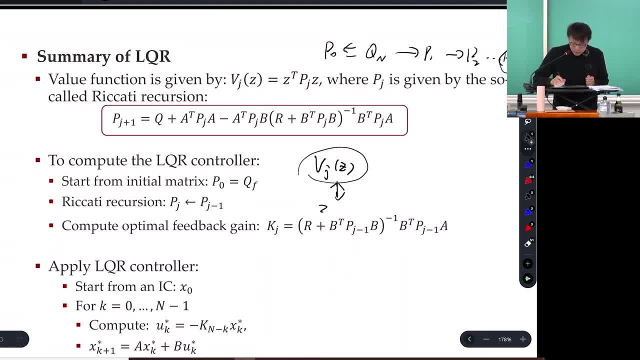 Right now. in this case, this guy is nothing but J, transpose P of Z of J. It has a prime tradition in finite state, the finite Dimension. I don't need to enumerate all of the, I just need to find a matrix. Okay, so once I find this, I know V, J and also know 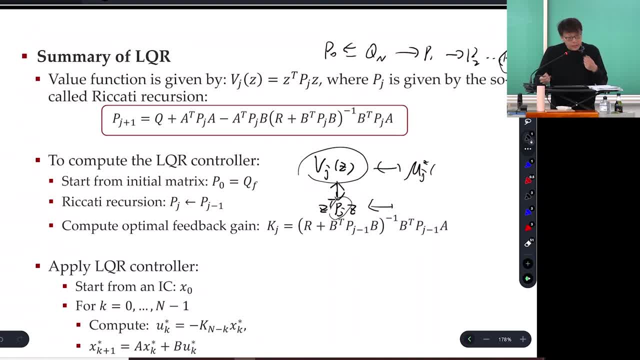 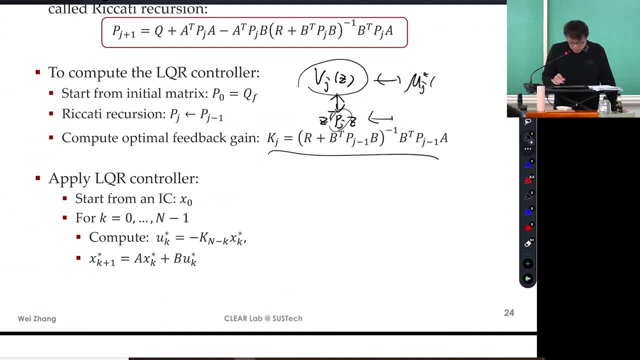 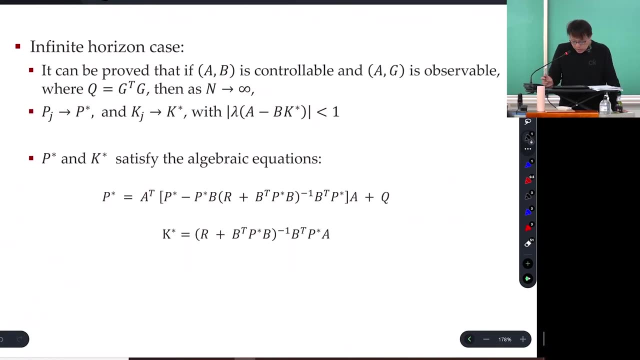 Corresponding mu of J star, which is a common gain related to it. All right, that's it. So our controller is just you at any given time. Once you find this, you find the K and then you just move your system along the optimal path, right and the infinite horizon case. 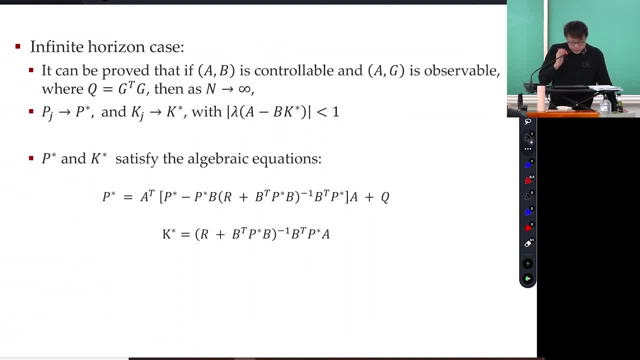 I Have 15 minutes. Okay, even a hard, in case It's. it can be proved that a B is controllable. a G is observed over there. cheese Q is G, transpose G. okay, you could decouple G and then the Valerie tourism converges and 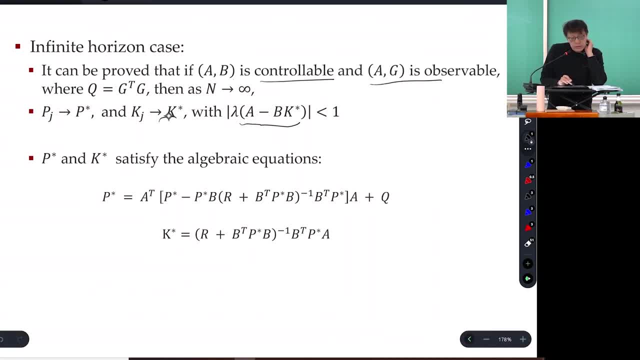 the Wednesday converged the optimal gain. it's: it's, it's all, it's a stable. your system is stable, exponentially stable, and And this satisfies the algebraic Riccati equation right. So when the update doesn't give any changes, it converges. 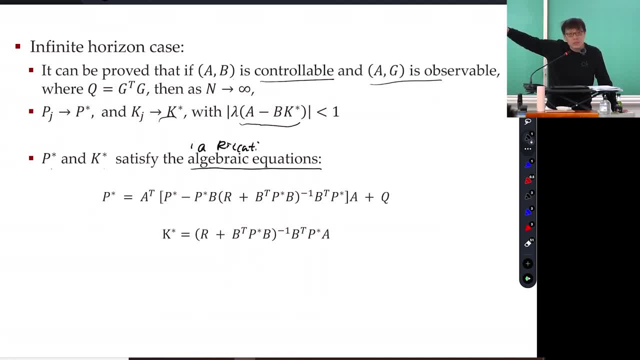 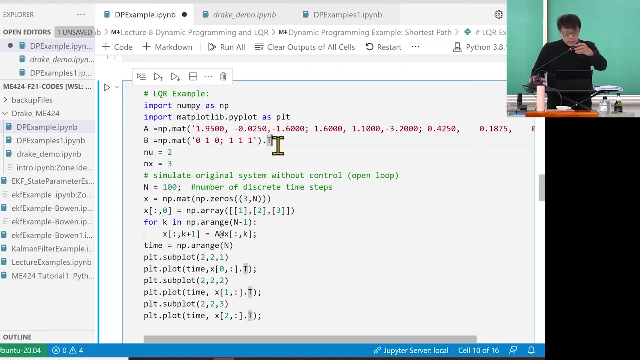 The value function converges, okay, then the gain converges as well. You don't need to have so many time varying gain. You have a stationary gain to apply. that's optimal gain. okay, Let's look at the code again. This is the LQR problem. 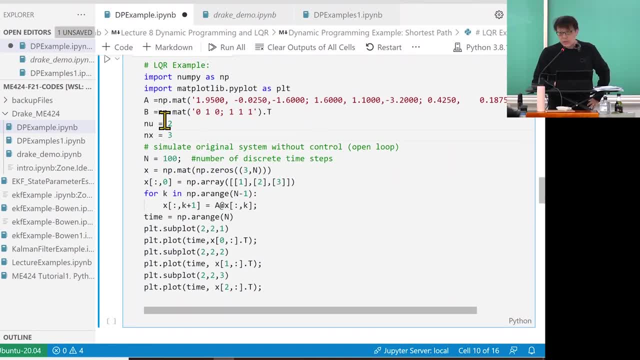 We have this AB matrix. AB is two dimensions. now, Before we did our pole placement. typically we can do pole placement for one dimensional U by hand and the high dimensional. I want you to use place function in MATLAB or in Python. In this case, that's a state. 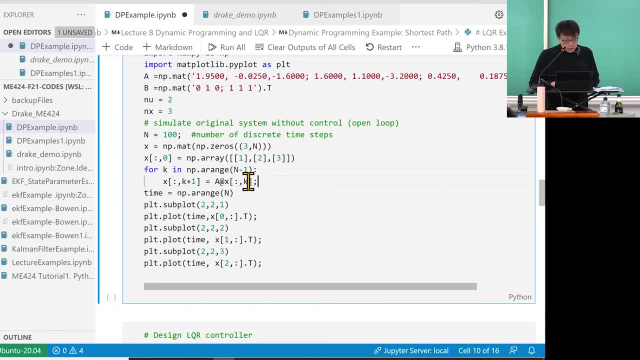 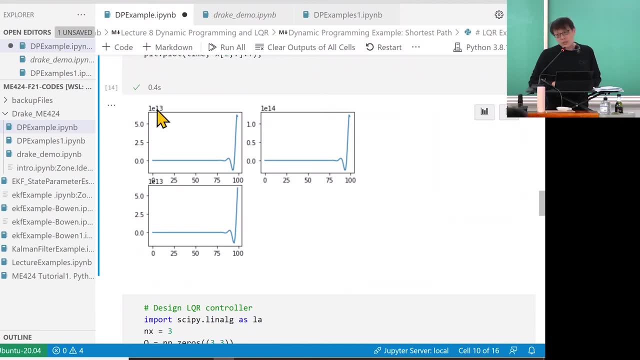 So I can plot without now, without any control, suppose I don't know how to control. the open loop system Is one. So 10 to the 13 is unstable, right, diverse. The system is open loop unstable. I have to design my controller carefully. 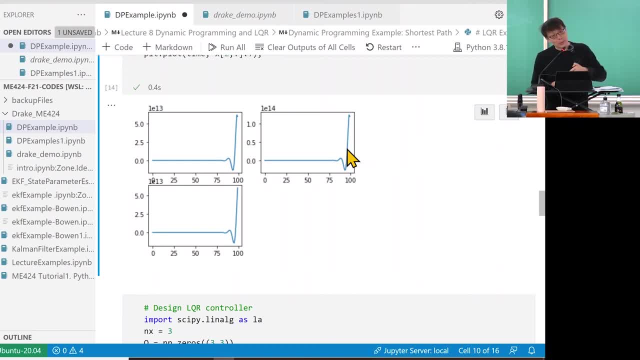 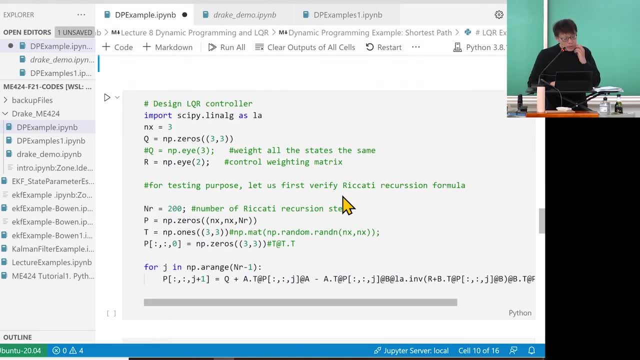 If it is open loop stable, then I can apply zero control. it's still stable, I don't need to do anything. it's good, but I can do things to improve its performance. Now we can design our LQR controller. Design LQR controller. 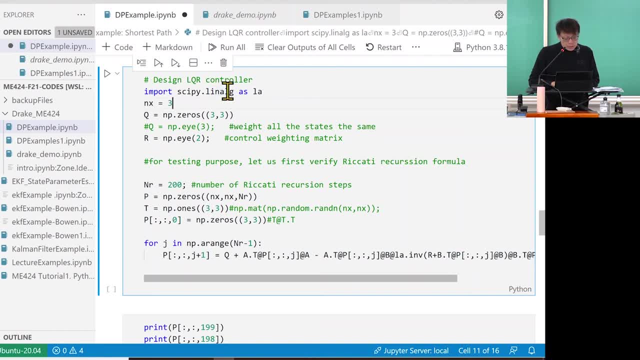 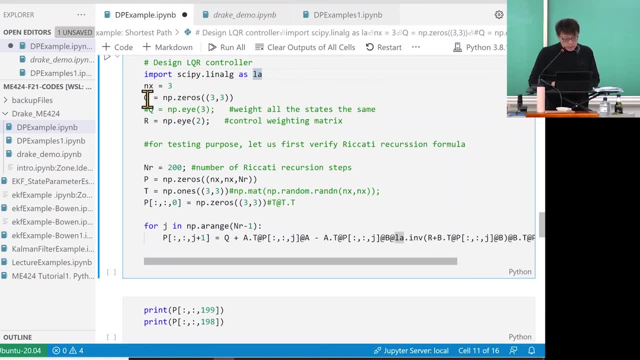 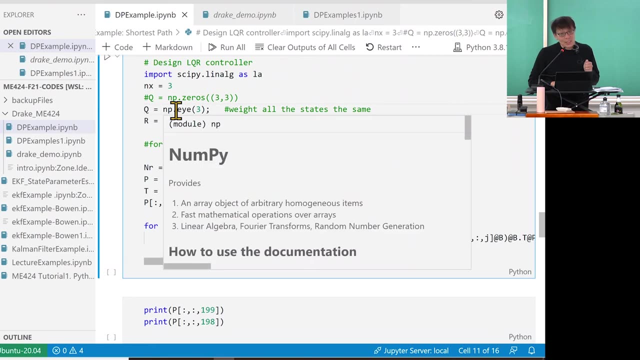 Okay, Okay, So now we have our LQR controller, Import this linear algebra package. then let's not use zeros. The terminal, this is the weighting matrix. So that means this identity means I weight all the states the same, okay. 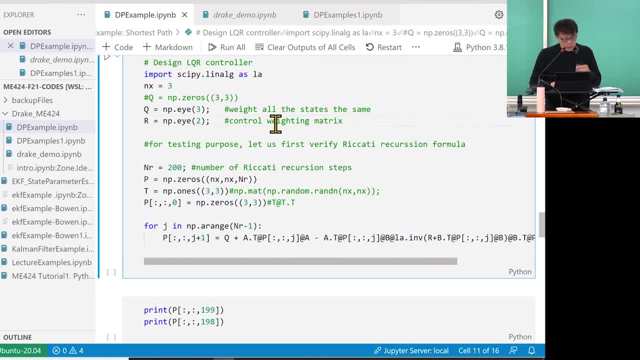 And R is the also identity. the control weighting is: I'm just trying this first, okay, For testing purpose. that's first the verify record recursive formula. And R is the also identity. The control weighting is: I'm just trying this first, okay. 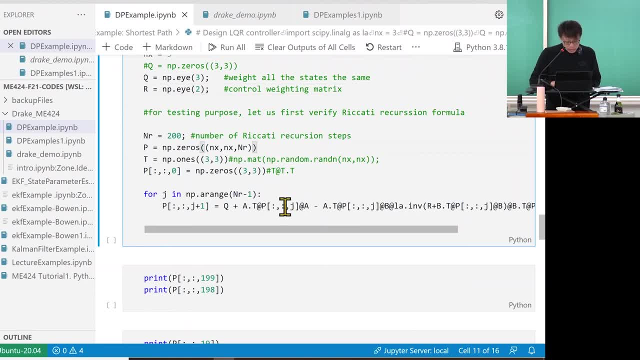 For testing purpose. that's first the verify record recursive formula. And R is the also identity, the control weighting. The control weighting is- I'm just trying this first. okay, For testing purpose. that's first the verify record recursive formula. 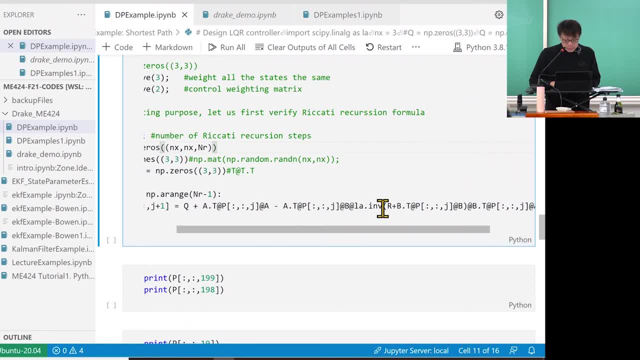 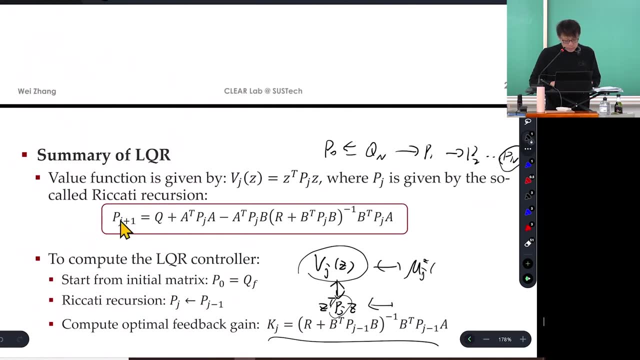 And if I run this, by the way, it's just one four loop. The long equation is, I think is just I typed it down, this recorded recursion: okay, q a transport p a minus a transport p B or whatever inverse. 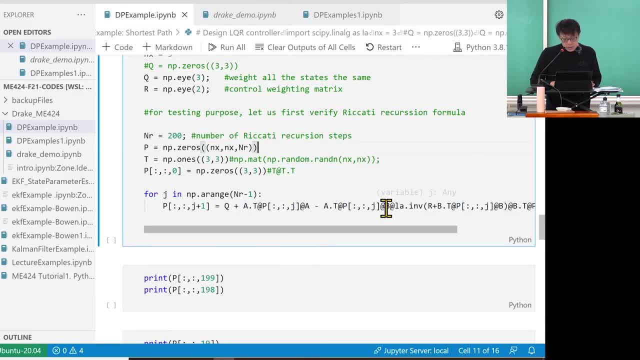 So q a transport p minus a transport p B. inverse of this is exactly typing down the recording deals. So here you smooth stuff out, Hardly recursive formula, And what we are computing is the optimal value function. Okay, the optimal value function is represented by p. now 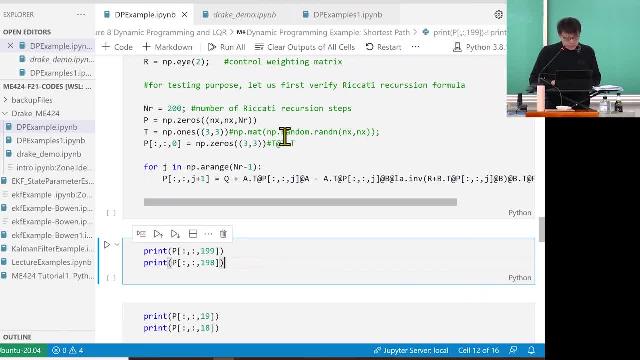 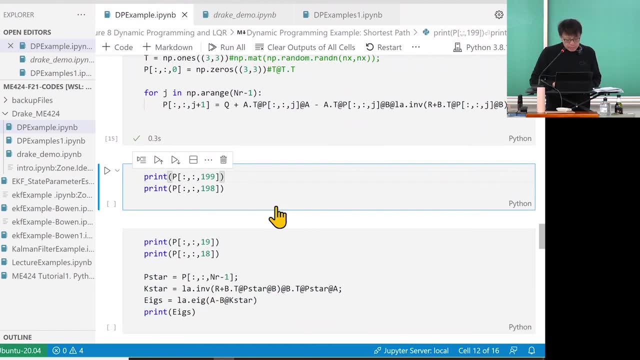 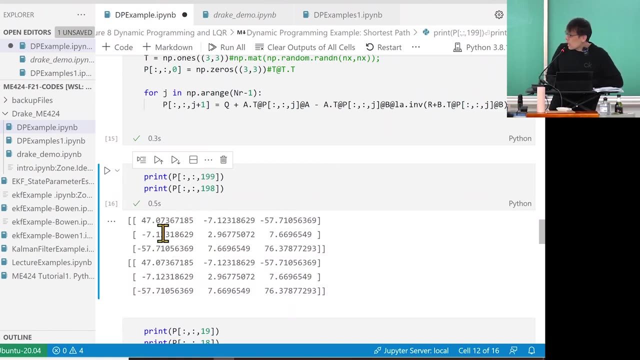 Okay, it's a quadratic function, So I do the formula for 200 steps. If I plot this 200 steps, they are the same: It's 199, 198.. The last two matrices are the same. Actually, I don't need 200.. 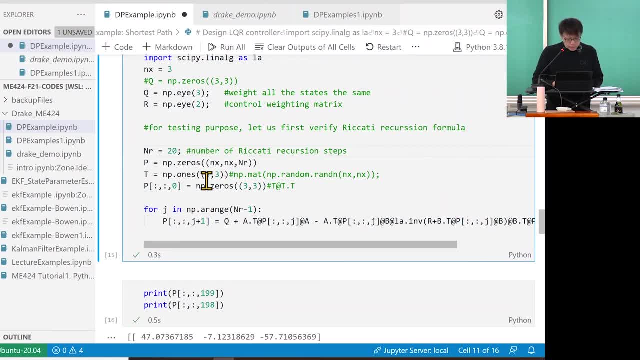 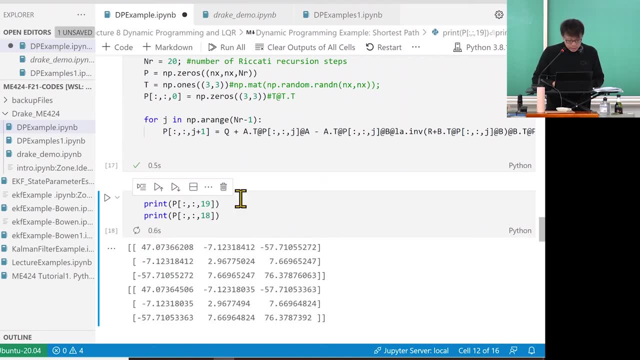 I think I need it will be convert pretty quick. 20 is fine, But I don't have it anymore 19.. Okay, it's already converged. It's exponential, converges very fast. I think 10 steps or 15 step will be converged pretty fast. 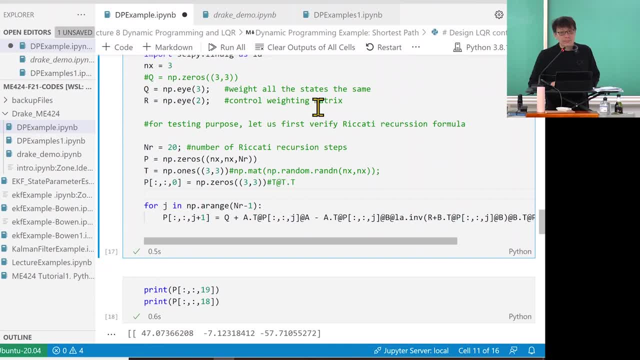 Why the converge With 10 or y? It's like, okay, think about this. It's a value function, the optimal cost, right? So if the system is controllable, that means you can drive it to zero. Of course you cannot drive to zero. next step: 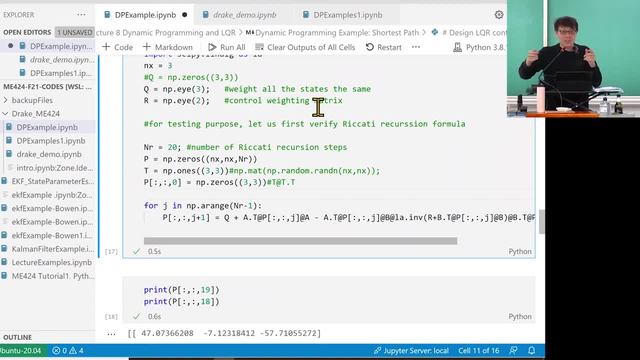 Maybe you're given four steps, or let's say 10 steps, You already can make it very, very close to zero. But if I give one more step to you, the cost doesn't change any much, right? You cannot reduce the cost further. 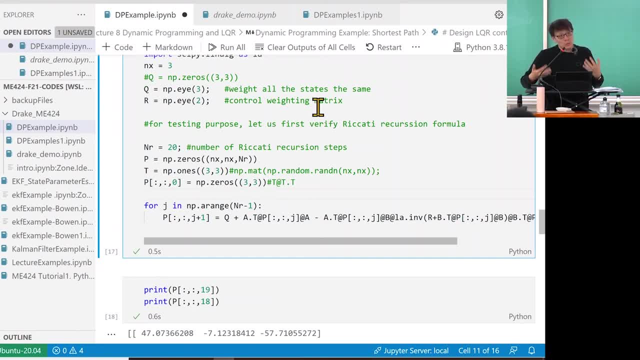 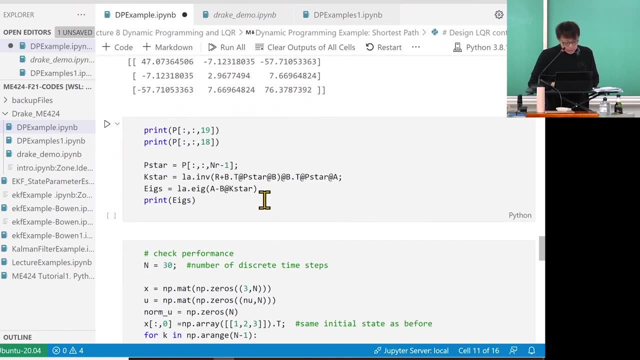 So once I give you enough time, horizon, you are able to do this right. So then that somehow, after the horizon size is big enough, then it doesn't change anymore. Okay, now let's see, let's check. This is K star. 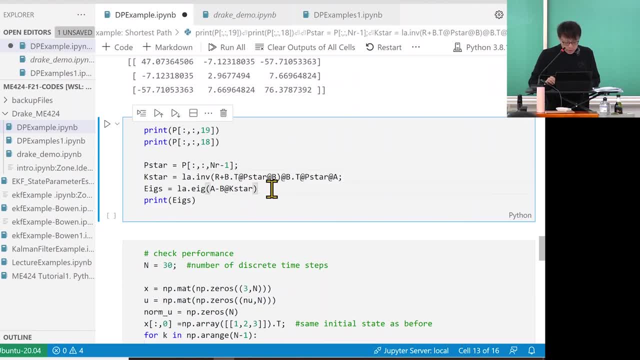 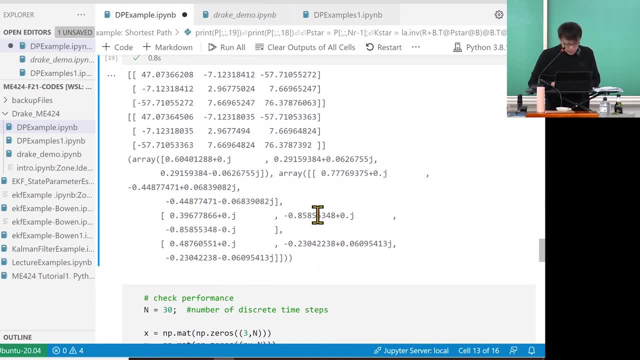 This already converged. I just use the K star. Look at the K star. the angle values is wow, where is the angle value? It's hard to see. These are the angle values. I think they're all close to zero. 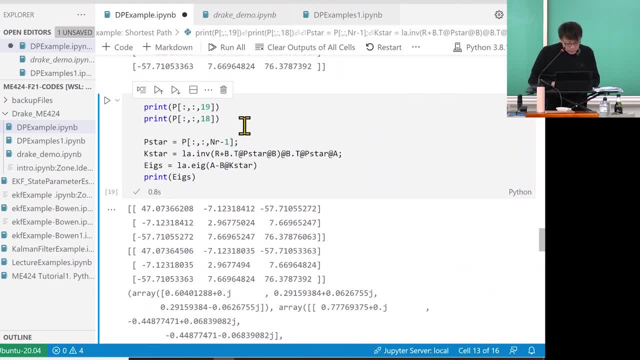 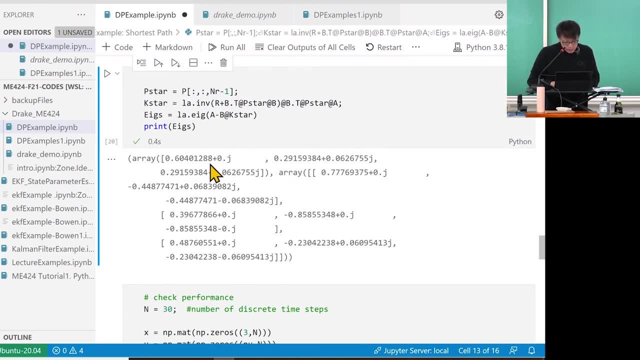 Oh, sorry, it's lost- stable at least. Okay, I print too many things. I don't need to print these two anymore. Okay, these are the arrays. These are the first array is the angle values. Okay, Those are angle vectors. 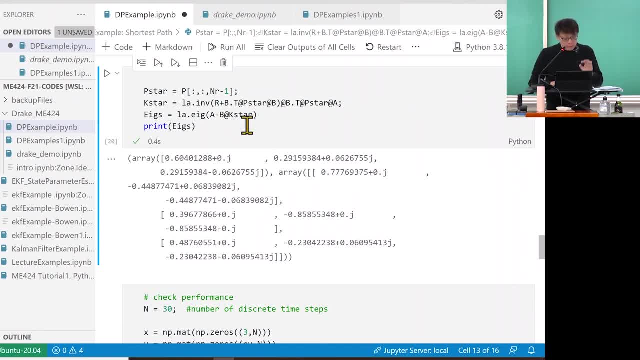 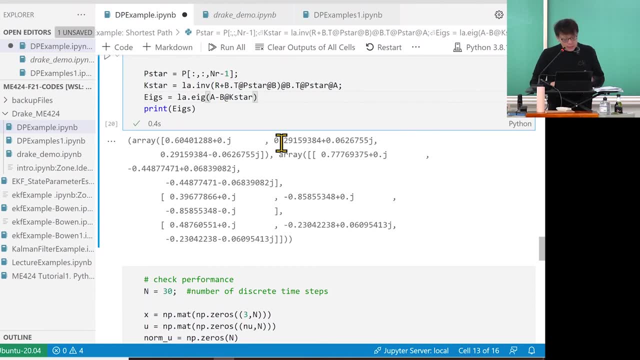 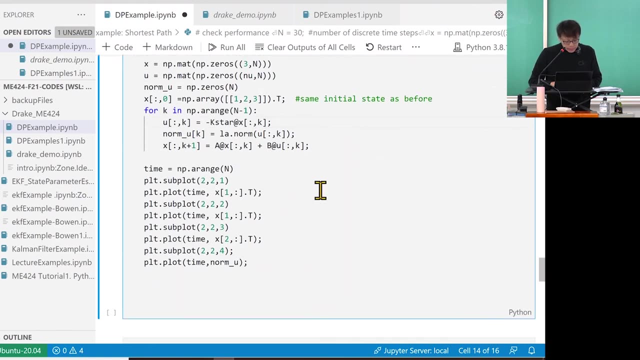 There are before it's open loop unstable, but all I want to make sure is that the converged one is stable, Okay, and then I can keep applying this controlled, this stationary control action. Now let's check the performance. How do I check the performance? 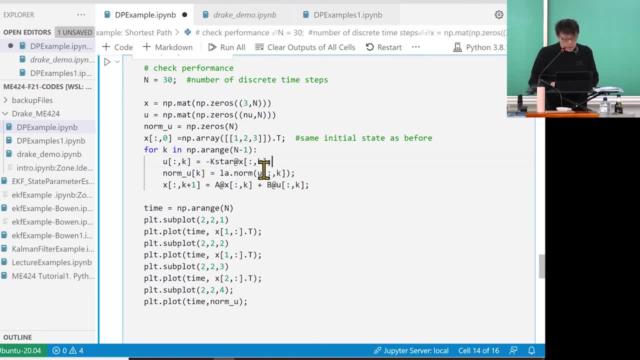 I need to simulate the system under this optimal control. How do we do it? We start from some initial state: One, two, three, the same initial state as we did before for the open loop: one. But now I, instead of using zero control. 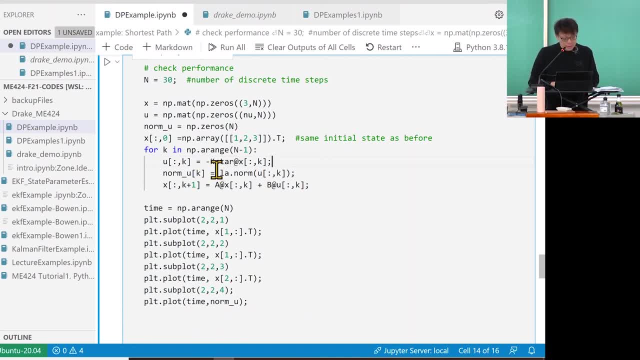 now I use optimal control. How do I compute optimal control? In this case, I just keep using K star. sorry So I didn't do the time-barring. It's KJ, right, It's K. first you need to apply K20,. 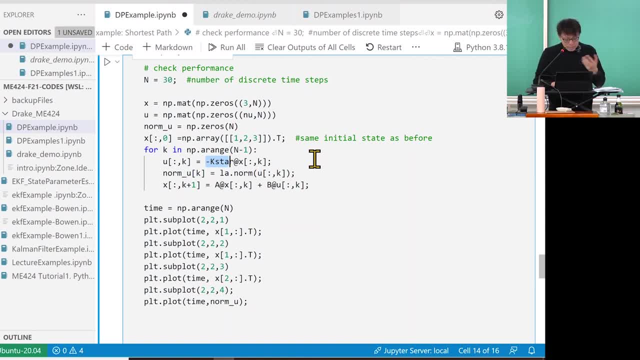 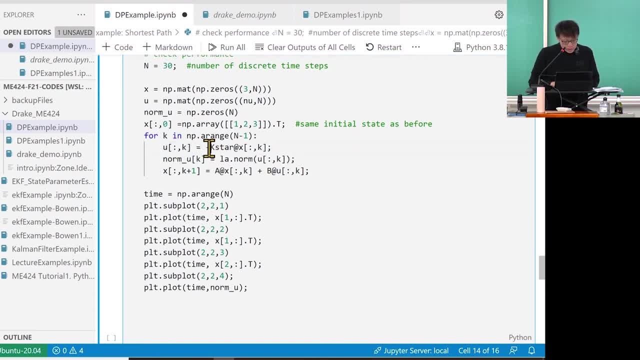 I mean the performance will be the same or similar right. I mean the performance will be the same or similar right. UK is K star again times this And I also compute the norm of U and then I evolve my system using this U. okay, 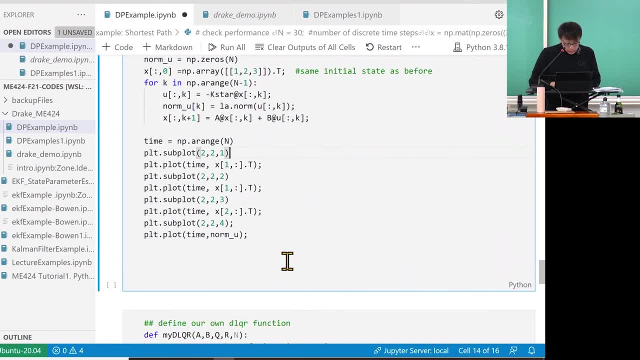 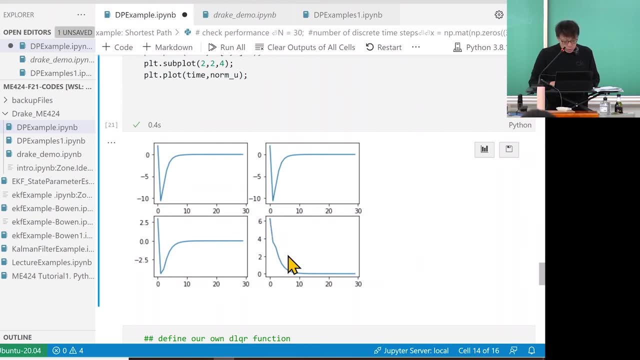 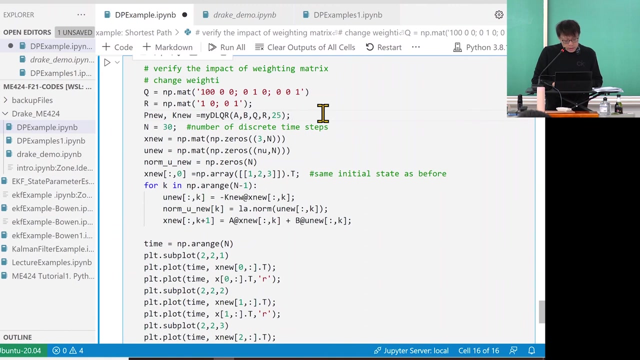 And then I plot it Before it diverts. now it converts. So there's X1,, X2, X3, this is the U norm. You see, U also converts to zero. So that's how it works. Now let's jump to the next one. 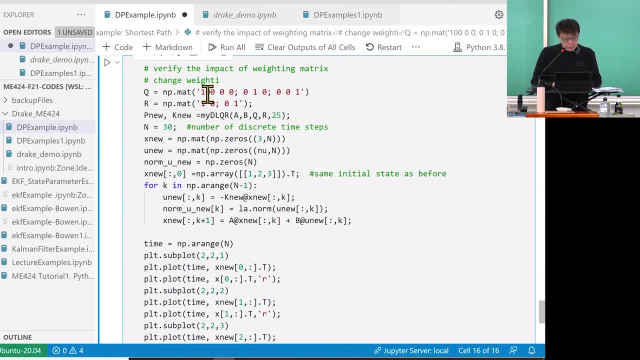 If I change it, let's say I change my cost function. okay, Before I have identity, right Now I make my Q a hundred. The first element is a hundred. What does this mean? The first element is to be more stable. 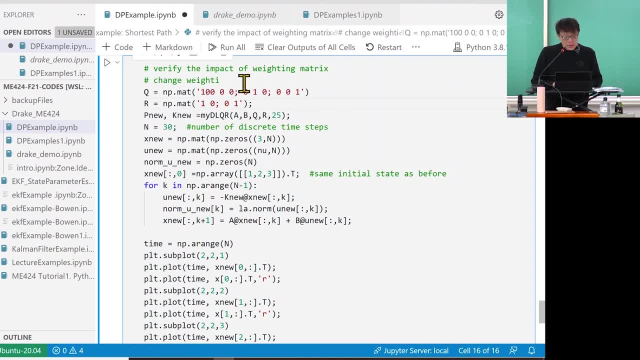 Stable as faster, much faster. Okay, So that means X1, I want to penalize X1.. I want it to be smaller, right? I think it's a hundred percent, a hundred times more important than other states. I changed my U. 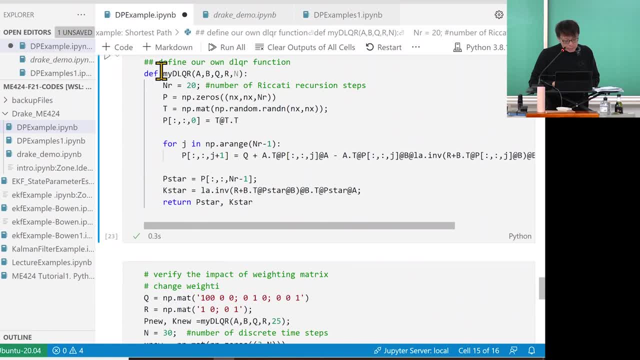 Because typically I don't want to rewrite this, I just have my own I O Q R. By the way, if you call D I O Q R in MATLAB, the Python, I didn't find it, I just I called it by myself. 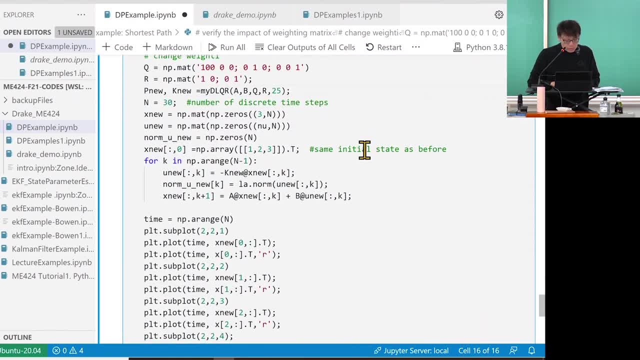 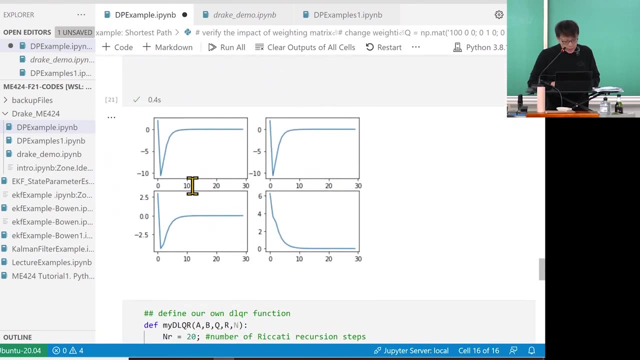 It's just this. No, then this is: let's see, I find the optimal value, function p and gain k. Then I have this is new, right Before I called it x. this is x And this I changed the cost and that becomes new. 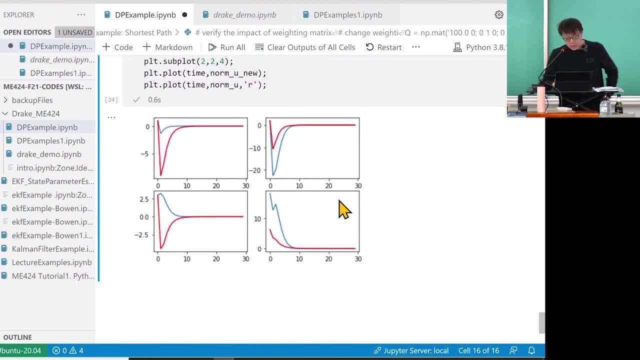 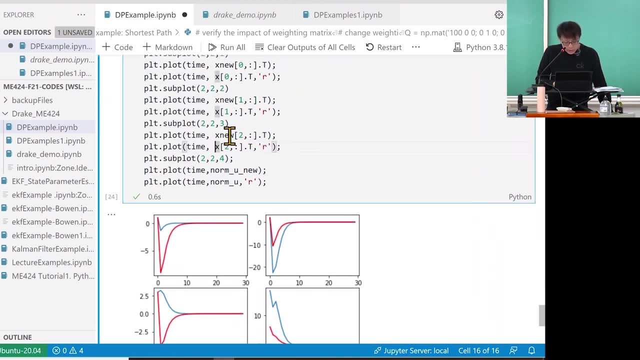 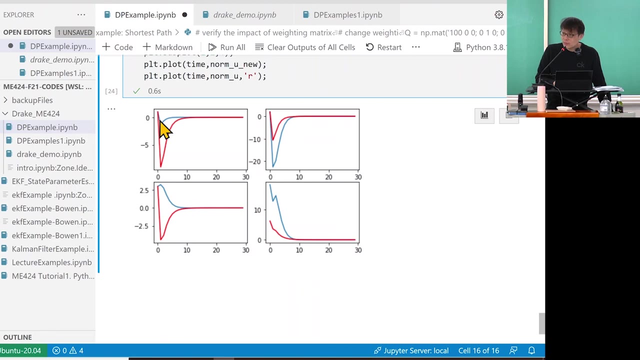 I compute them together: The red one is the previous one. I think Red one is the x. The blue one is the new. okay, What did I care more before I care more x one. The blue one becomes dramatically smaller. okay. 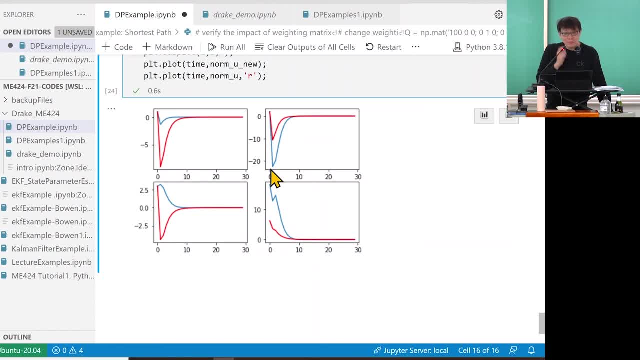 But there's no free lunch. X two become bigger, Right. This is the blue is the new one, right? X two is bigger than before because you care more about x one now, okay, And the control action is also bigger, right. 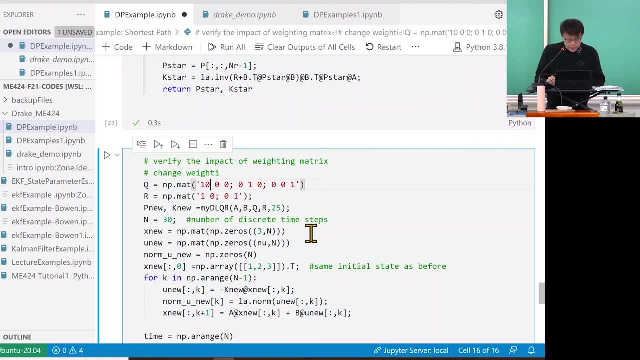 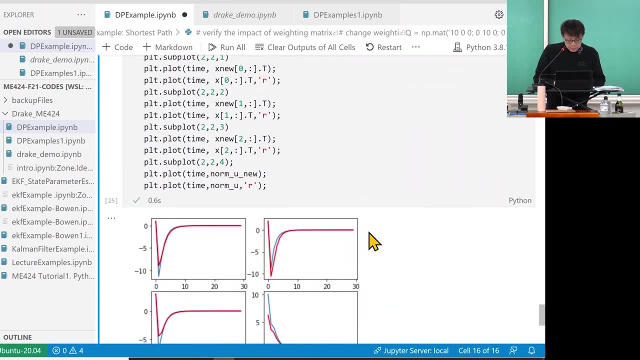 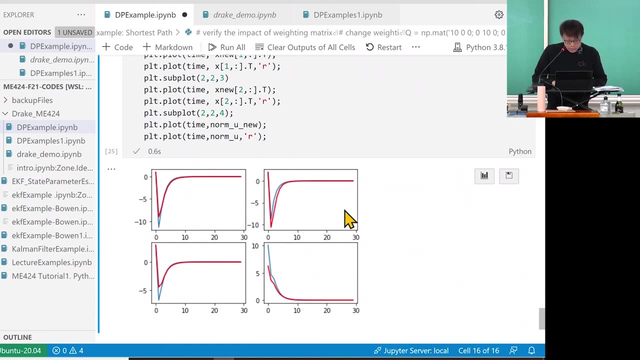 And you can play with it. If I care. this guy and this guy- x one, x two. both are more important. I can see that doesn't work well, that much X two is more. it can be handled. Where is it? 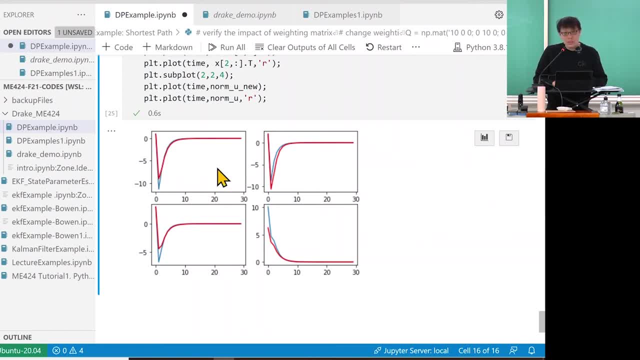 Okay, x two is smaller than before, and then sacrifice a little bit. There's no kind of a strict constraint. If you add more constraint that you wouldn't be able to derive the formula analytically, then you have to use MTC. 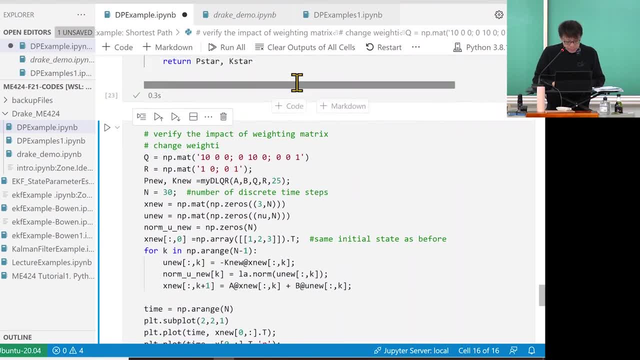 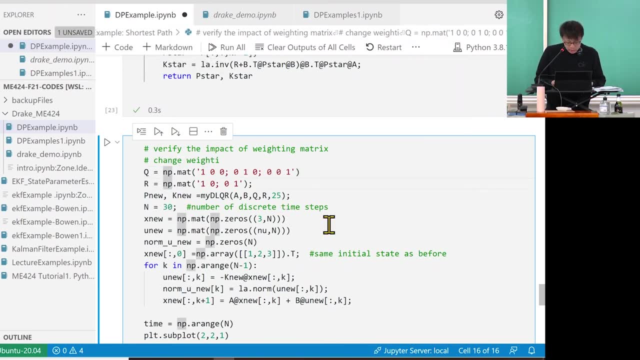 You have to do it on the runtime. I can penalize- let's say this is one, This is one. I can penalize my control action more, Let's say a hundred times more. So I don't want to waste my control energy. 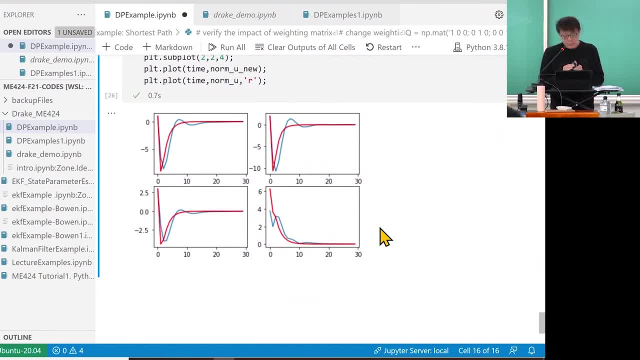 And you can see that the case. Which one has a bigger control, action or energy, The blue or red, The red one, right, The total energy is the one underneath the curve. Okay, That's the total energy, The energy underneath the curve. 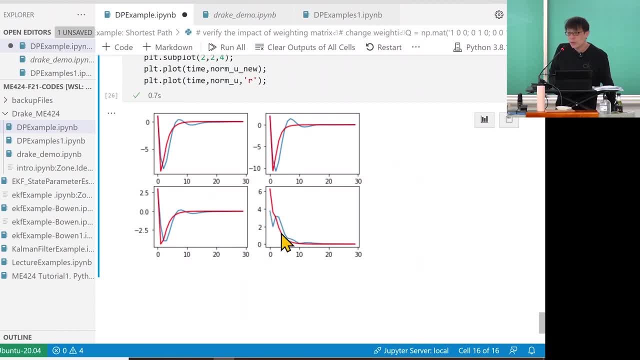 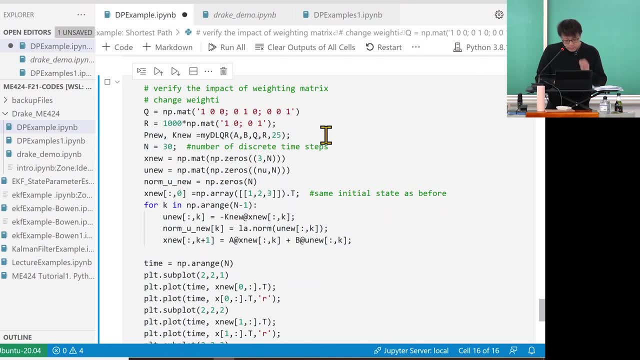 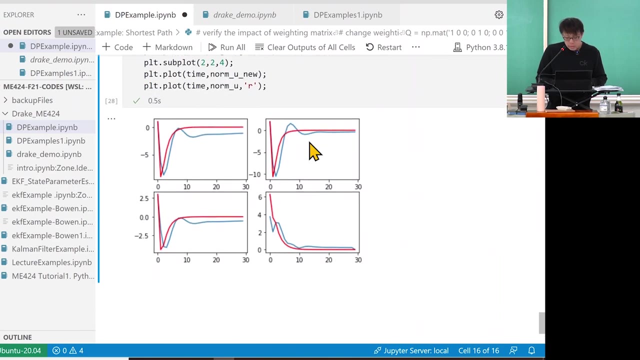 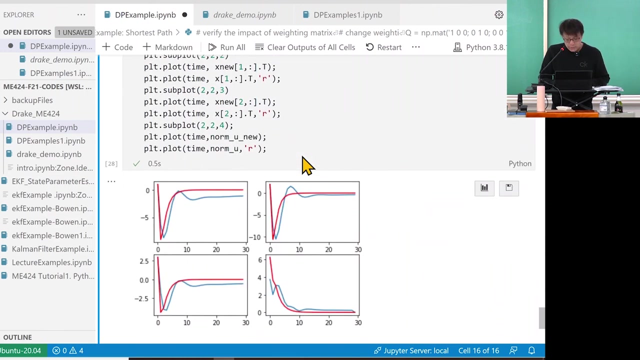 I think the blue one is smaller, That's the new one is smaller. If I take more extreme, it doesn't work. It's still. it's almost like a. I don't know why it doesn't work. No, it doesn't behave like the way I want. 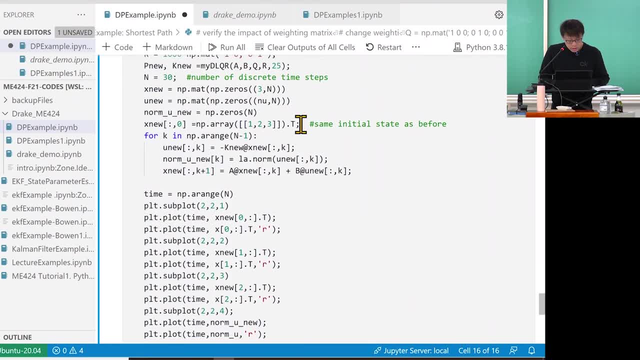 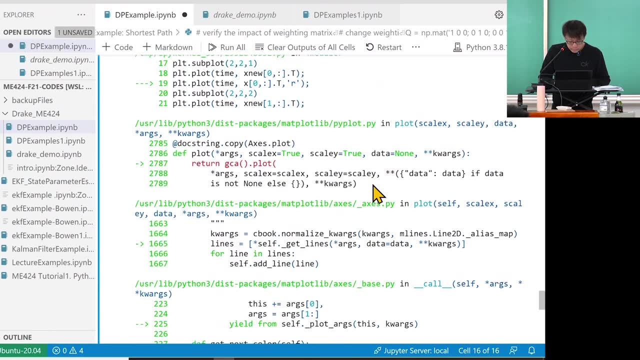 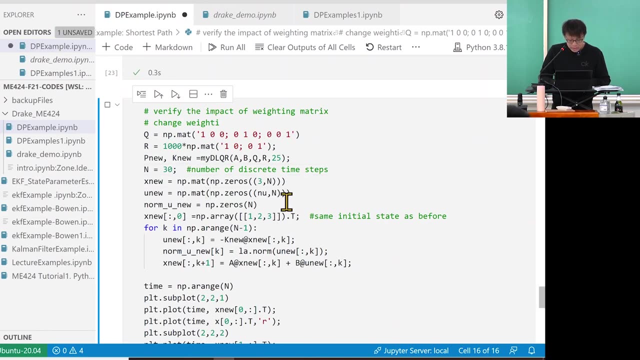 It's not working. It's almost the best I can do. Maybe I can make it more. The other one is only 30 steps. I don't think that we can see that much difference within 30 steps. That's why I want to change. 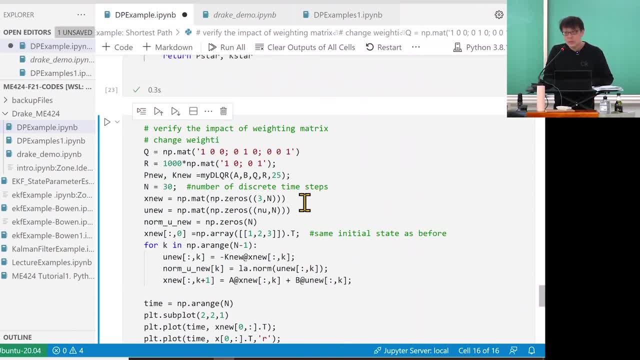 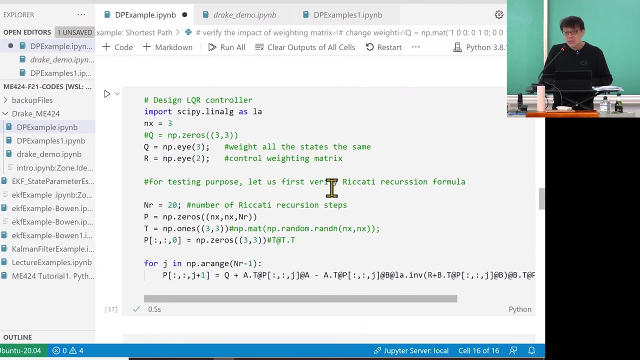 Anyway, I think you can play with it. Okay, I don't think we have time for quiz today, Do we? Four minutes, Four minutes. I have a really hard quiz for you, but Okay, that's almost the end of our QR. 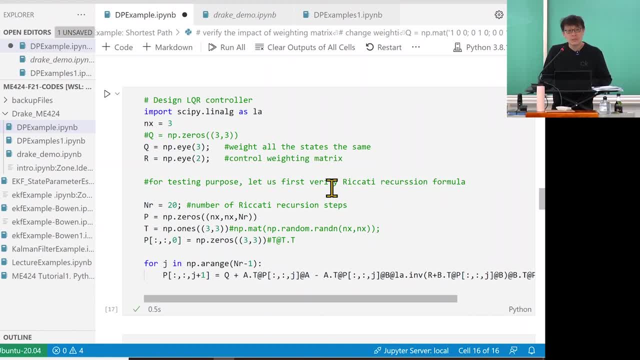 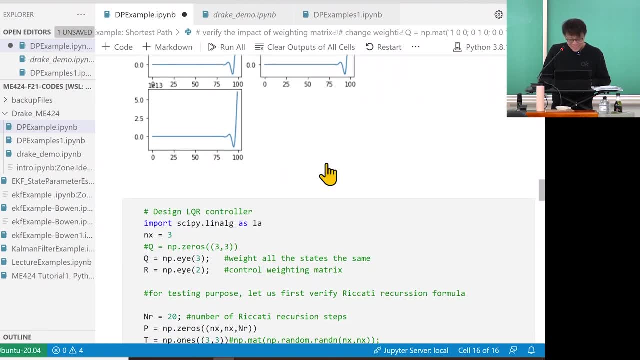 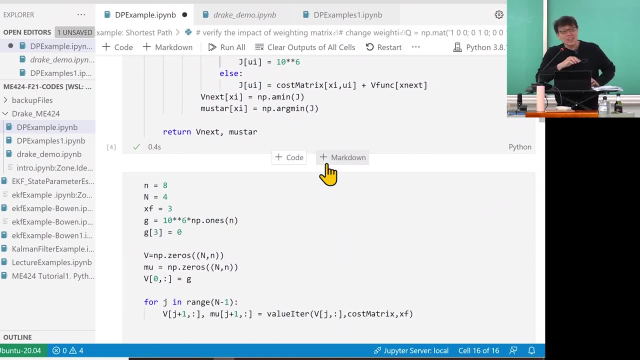 And the end of everything for this matter. Next time we're going to review: Huh, What's wrong? You want to learn more. You want to learn more. I was going to talk about MPC, but I don't have time. 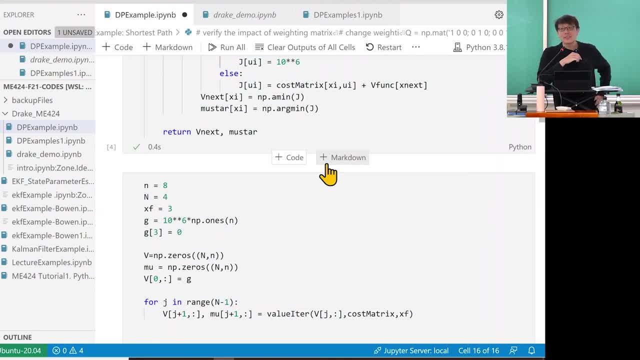 Okay, I was going to talk about MPC, but I don't have time. But I feel like a lecture can probably go over a little bit. It may not be very meaningful. I might as well learn this from us. Actually, you've already been in touch with a lot of things. 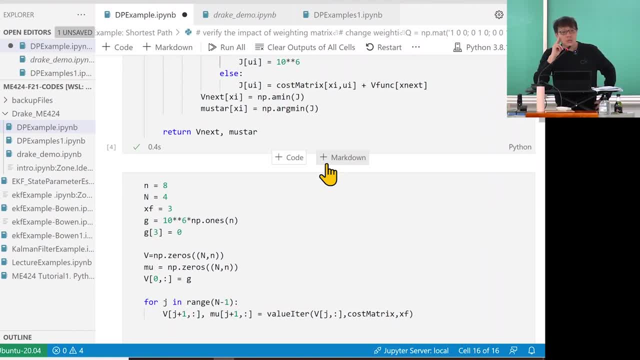 It's almost time to read some information. Uh, we can just take what we should learn and learn it a little more deeply. It's better. In the next class we will review it more deeply. All right, We have this semester, including the beginning. 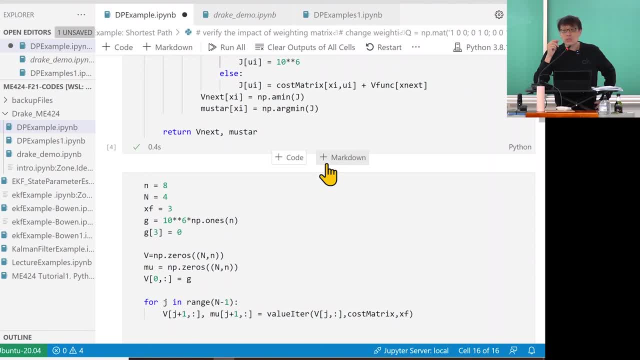 All right, And then I hope you guys do a little bit of review beforehand, All right. Otherwise, if you forget what I'm talking about, the results won't be as good. So in the last couple of days before Wednesday, 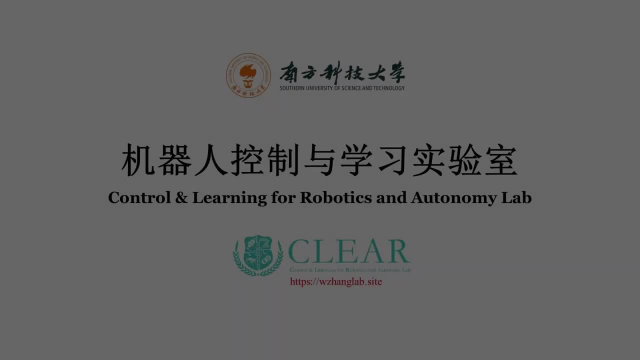 you should do a little bit of review, It will be better. 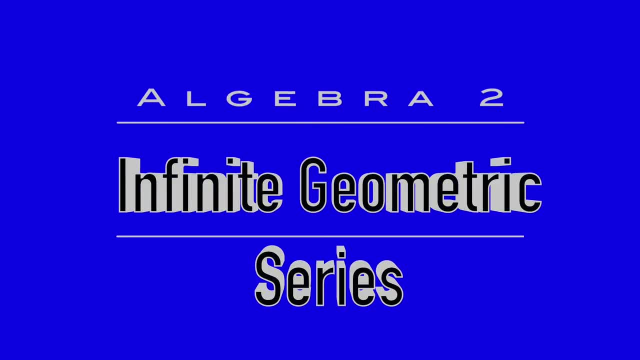 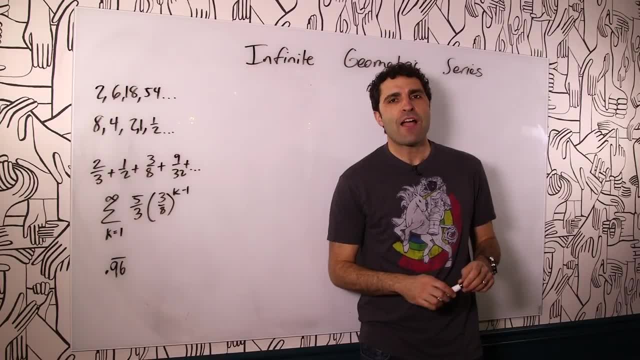 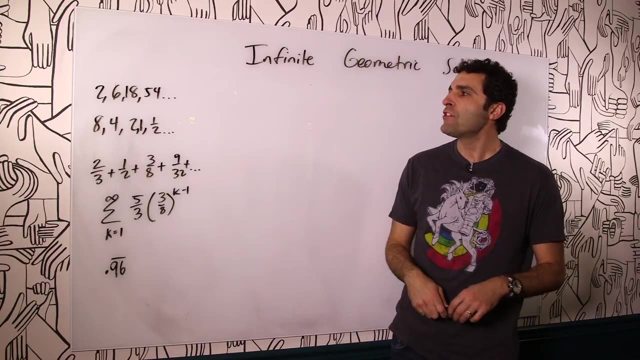 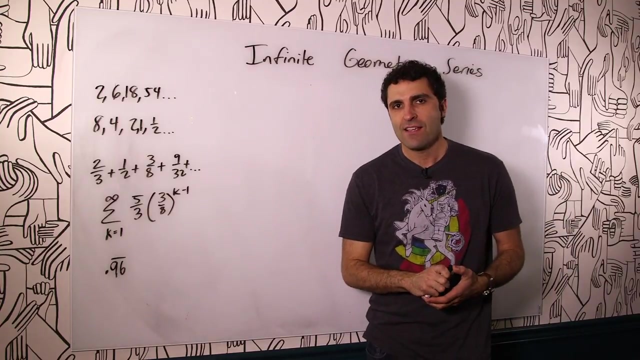 Hello, my name is Robert Adut and welcome to yaymathorg. This is called Yay Math in Studio, where I bring to you, first and foremost, from the first person perspective, how to do these high-level Algebra 2 topics. Today's topic for Yay Math is infinite geometric series.